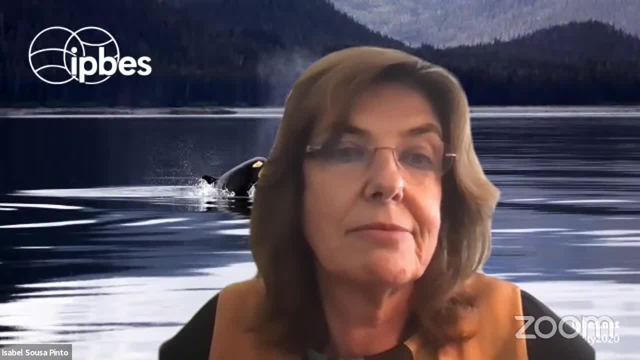 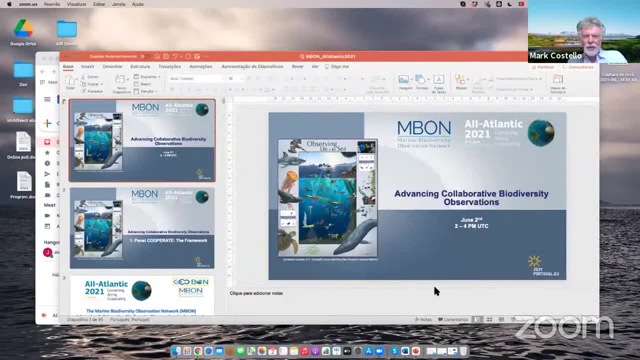 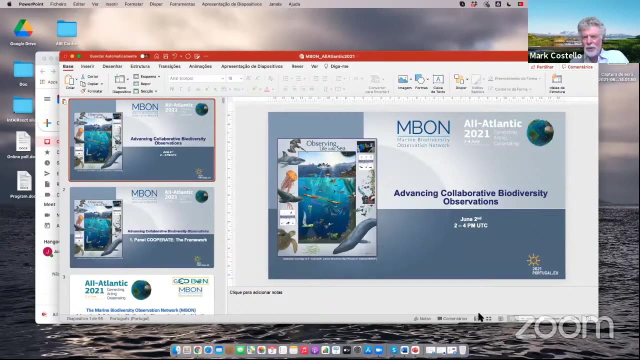 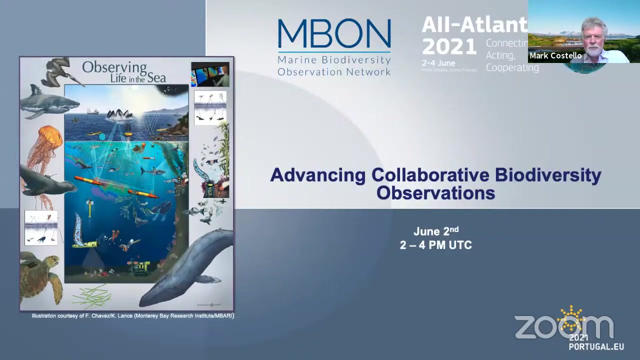 Welcome to the All Atlantic 2021 conference and we're going to have some introductions to the Marine Biodiversity Observation Network by Isabel Sousa-Pinto and Frank Muller-Karger and others. And who's going first, Frank? It's me, It's you, Isabel, sorry, Okay, You. 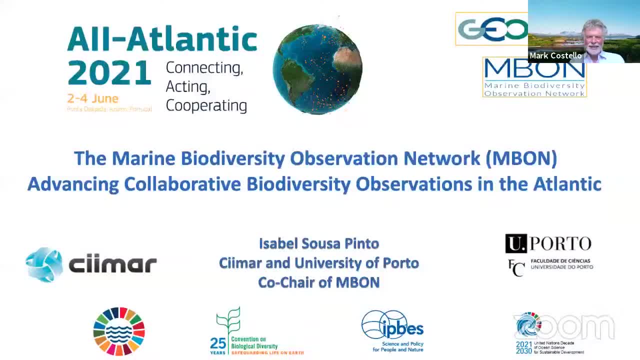 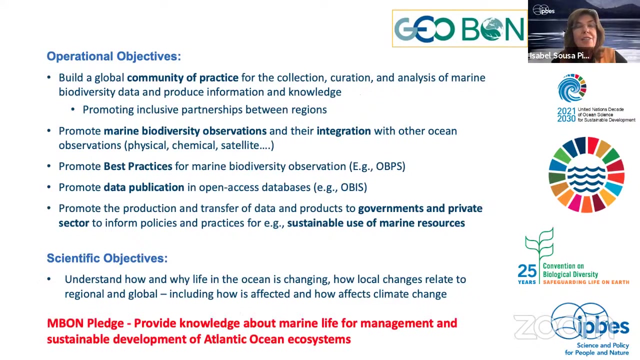 have the floor. Thank you Well, good afternoon to everybody. So I'll be starting with this M Bonn and Advancing Collaborative Biodiversity Observations in the Atlantic Next. So I think I'm going to start with you, Isabel. Next slide, please, Joanna. So the M Bonn. 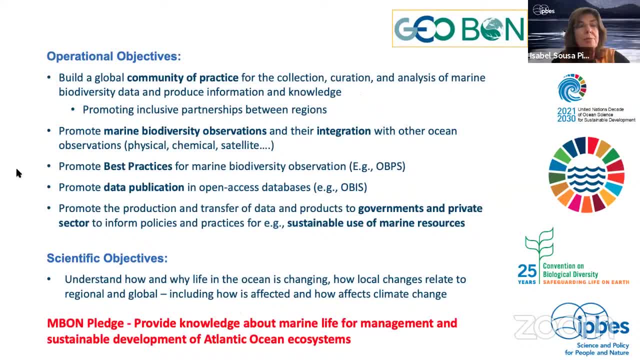 the operational objectives we have is really to build a global community of practice to really collect, create and analyze marine biodiversity data and produce, hopefully, useful products and knowledge to support decision making. We also promote very much inclusive partnership between the different regions, So that's very good for this Atlantic. 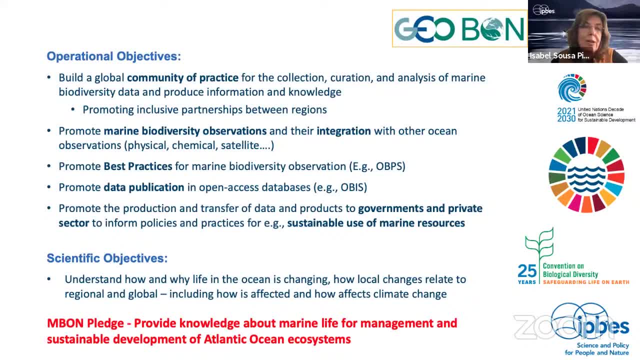 cooperation. So we also promote the marine biodiversity observations, because we believe we need more of those, but also their integration with other ocean observations, for instance physical, chemical and other observations, in the framework of GOOSS and all these regional, group and national GOOSS programs. 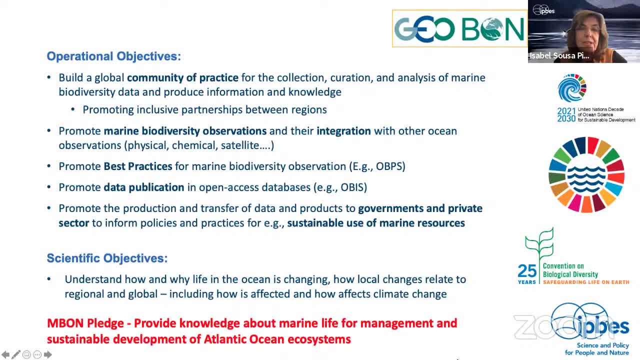 We also promote best practices for marine biodiversity observation and we do collaborate very closely with the ocean best practices system. We promote data publication in open access and work very closely with. We promote also the production transfer of data and products to governments, to civil society, to private companies and all the 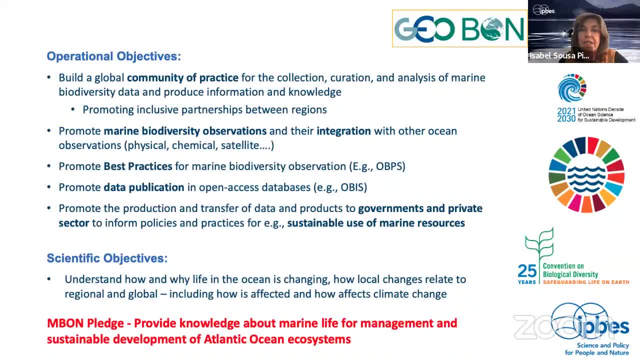 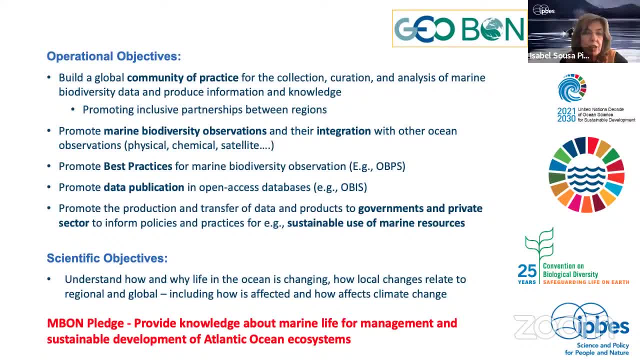 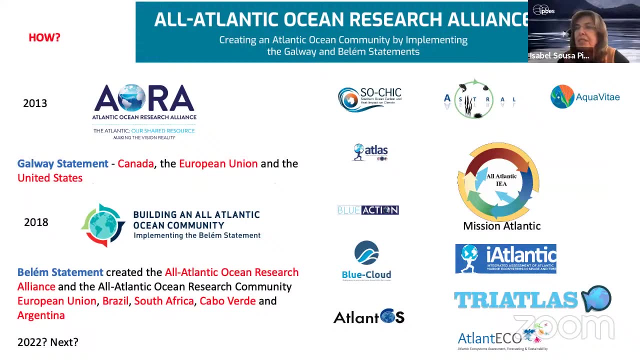 we have a firstひさуб and we have this project with the young women's research organization And we've done, you know, a lot of Джiba going for this and English research 저�. so we say thank you. 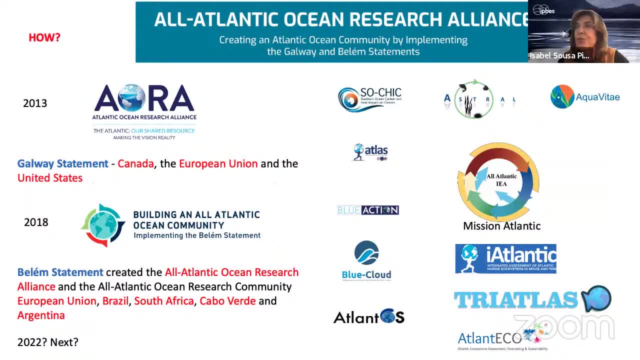 Thank you, Let's go. Let's go over there. There you go. the united states really sign an agreement to do cooperate in research, in marine research for the atlantic, in the mostly in the north atlantic. it was followed by in 2018 by the belen statement. 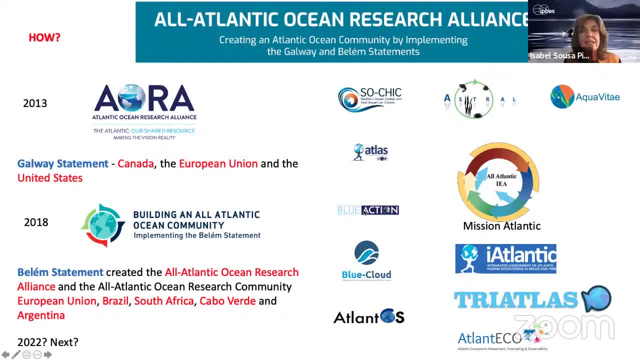 that created the all-atlantic ocean research alliance and the this anchor. this project is trying to build this all-atlantic ocean research community. this statement and this was assigned by european union, brazil, south africa, cape verde and argentina, but also brings together many other. 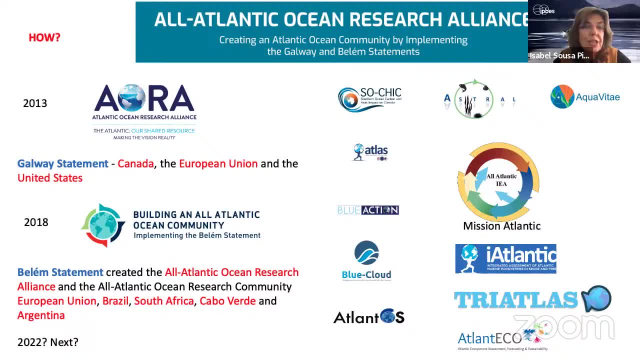 countries that are boarding the atlantic. so this um, this um activities really brought together a lot of working groups to work in in many issues as a culture by the rest and so on, but they also brought funding for a number of projects that really bring together partners from. 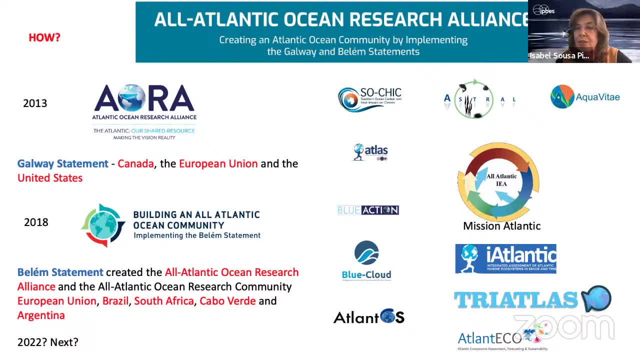 the, the all sides of the atlantic, and i would like to um to signal these four, please next, this four here that are now, uh, ongoing and they are collecting really data, new data on biodiversity in the ocean, they are modeling and really creating products are very much in line with what we would like to do with embon next, please. 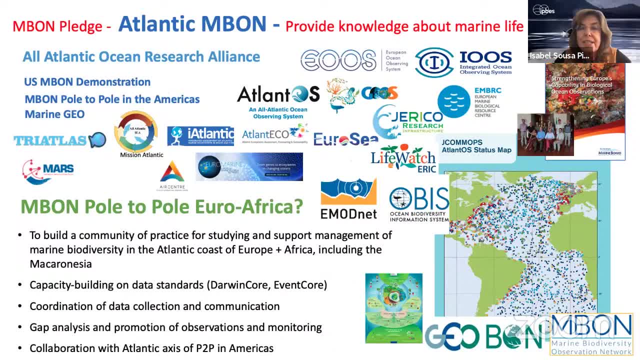 next, um so, uh, this is a little bit um, uh, the building blocks that we have, some of the building blocks we would have for this we could call the atlantic embon. we have already all these uh initiatives that i referred to before, but we also have the us and bond demonstration. 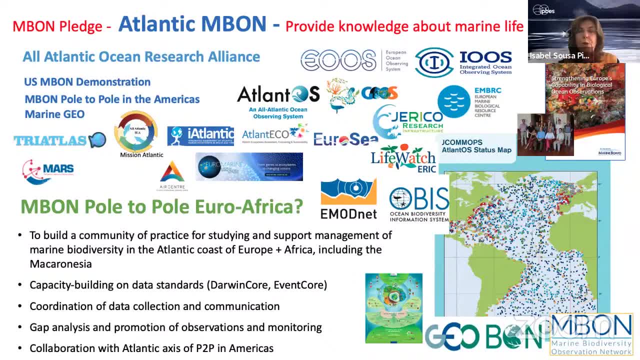 that in the in the us, tried to really move forward in this understanding how to bring together observations for knowing better marine biodiversity. the, the marine protocol, will be also presented and marine geo will be presented later and we could, for instance, also create this embon pole to pole that is going to be presented for the americas, but we could do it also in europe. 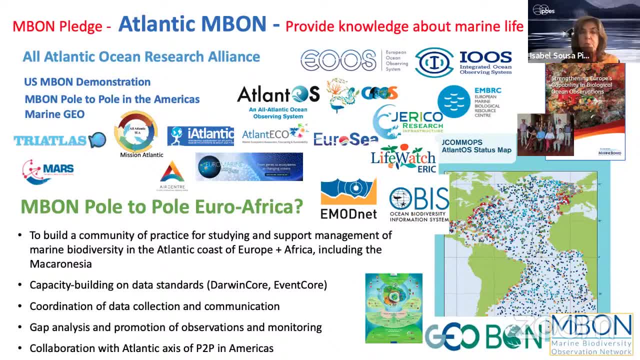 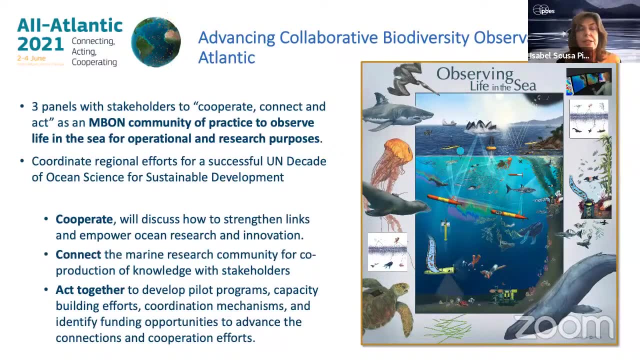 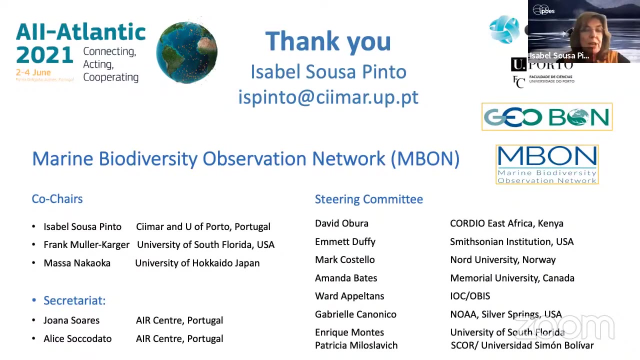 africa and really create a community, whole community, of atlantic biodiversity observation. so we would like to take a look at the, the different types of methods that we will use, and also to see how the support looks like and, um, how can we be a part of this? uh? 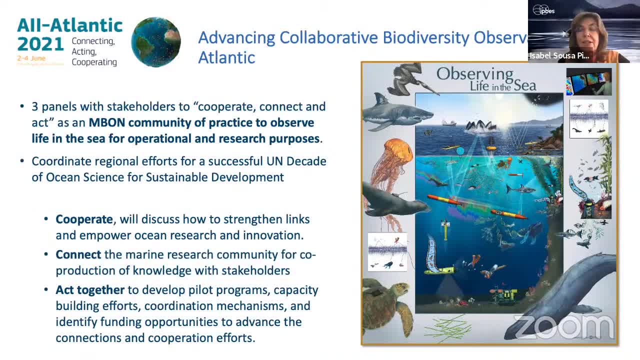 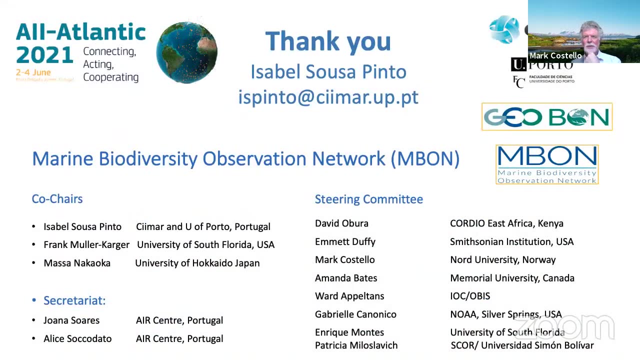 next, okay, next, so, uh, we are here, then, to really cooperate, uh, create uh, cooperate- now it was a little uh, cooperate uh- and to act together and so to create this community for marine biodiversity. And I think now I end here. Thanks very much, Isabel, because each speaker has just about five minutes, so we have 10 minutes for discussion. 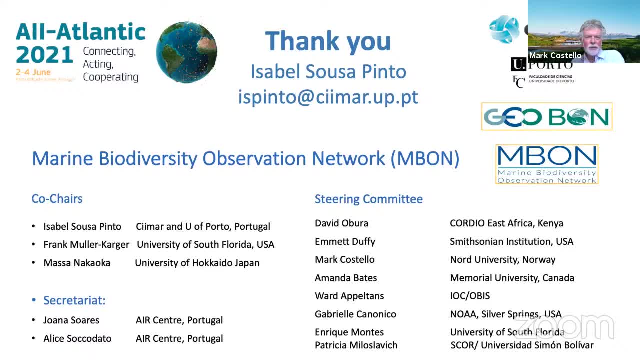 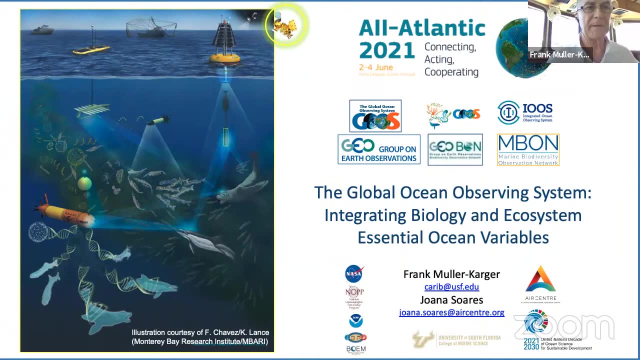 Thank you. So two of the Marine Biodiversity Observation Network chairs are based around the Atlantic, Isabel and Frank, And the next presentation is from Frank Muller-Karger. Thanks Frank, Thank you Mark, Thank you Isabel, Thanks everybody for participating today. 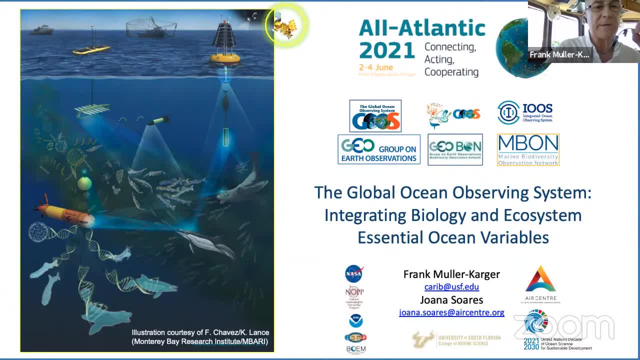 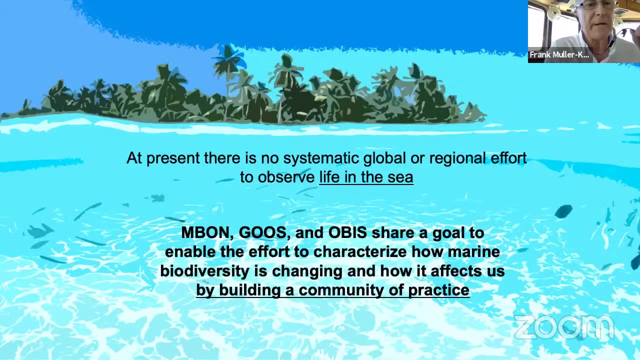 I'm going to talk to you a little bit about how we're trying to organize the community around essential ocean variables to produce the necessary information that we require to track what's going on in the ocean. Next, Many, many ecosystem services. Many, many ecosystem services depend on life in the sea, And the problem that we have is that there's no systematic global or even regional effort to observe life in the sea. 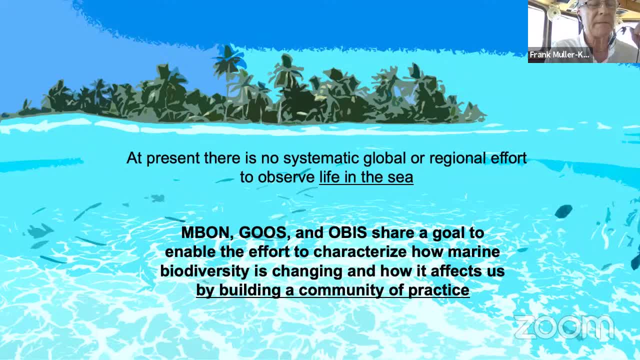 And by that I mean a well-coordinated, community-based set of standards that we can use to share the information so that we can build appropriate indicators, And that's essentially the activity that we're talking about today. How do we collaborate to reach that? 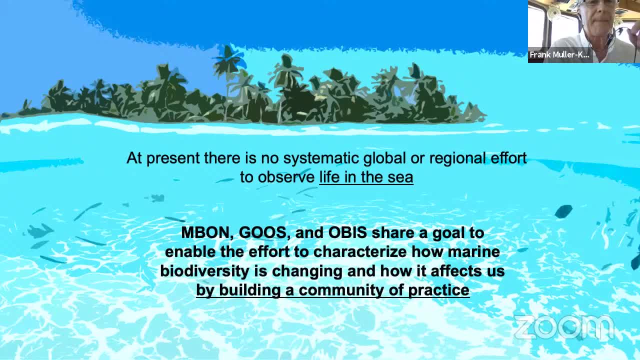 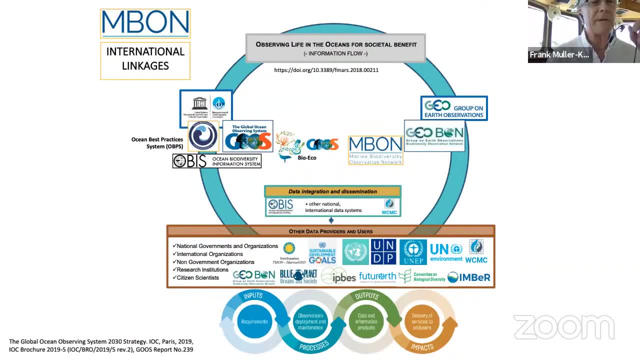 So for that next Next slide, Thank you For that- we're working with international organizations. These are governmental organizations. On the right-hand side, here you see the Group on Earth Observations that Isabel talked about and others are going to talk about today, under which we have the Marine Biodiversity Observation Network. 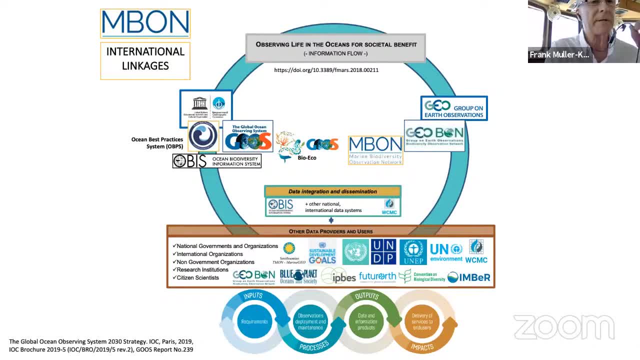 But one of the main pillars of the activities that we're conducting is housed under UNESCO. This is the Under Intergovernmental Oceanographic Commission And they have several programs. One is the Global Ocean Observing System that has physical, biogeochemical and biological and ecosystem panels. 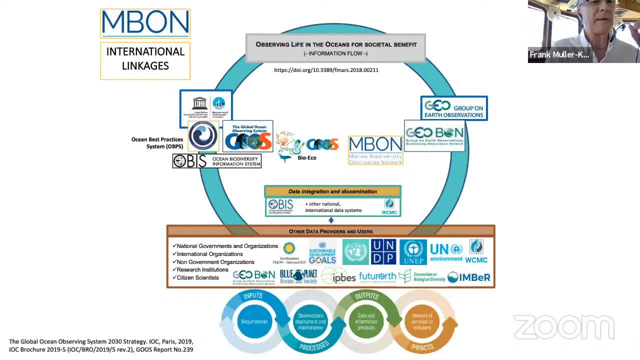 And we also work with the Ocean Best Practices System, the Ocean Biodiversity Information System, or OPIS, and the Ocean Teacher Global Academy. All of these that we link together across these different organizations to develop the standards and the frameworks to develop information for the agencies that receive the loan. 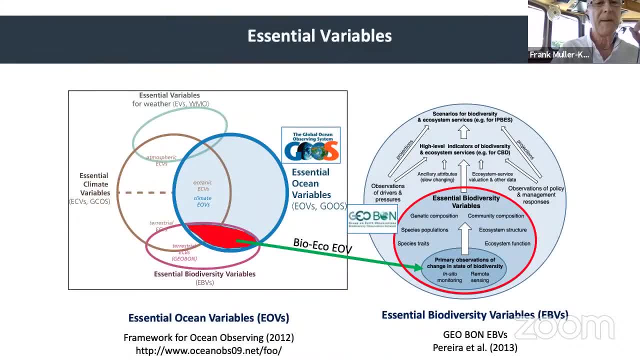 Next, Next slide. So we have this concept of essential variables. This was started by the essential climate variable: people, the Global Climate Observing System. There's a number of efforts that have developed kind of in parallel. One is the essential ocean variables and there's also essential biodiversity variables. 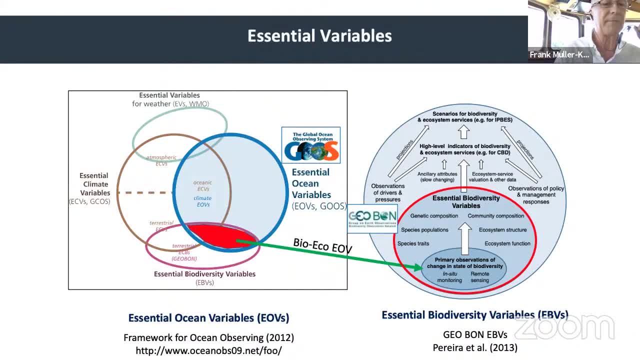 For for. in order to construct the biodiversity variables, we need fundamental taxonomic and other types of information about life. Those are the essential ocean variables for biology and ecosystems And that's what's shown in red in the left-hand side graph. That feeds into the primary observations. 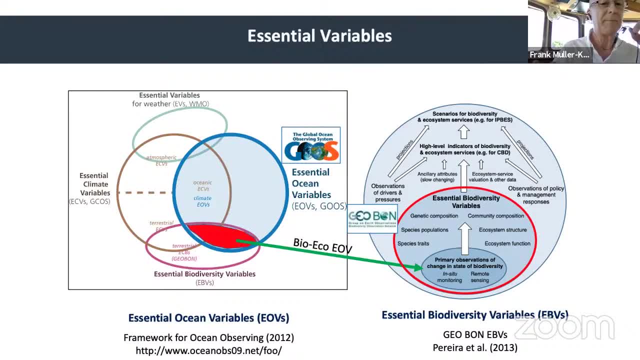 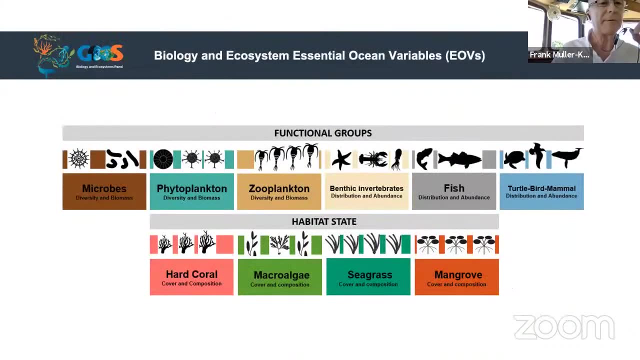 that then build up to the essential biodiversity variables. EBVs- essential biodiversity variables- are like maps that change over time, So they have to be, you have to be, you have to have the independent individual observations. Next, The essential ocean variables for biology and ecosystems. 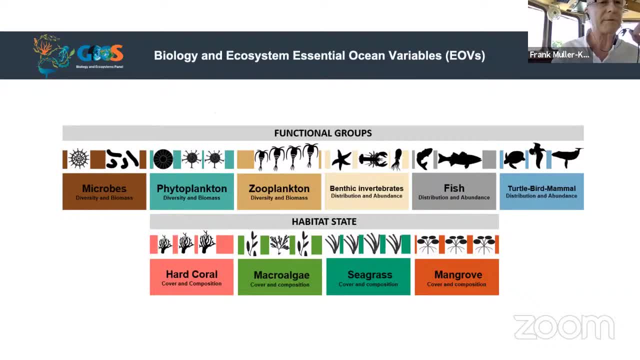 are organized this way. They can be found under the Global Ocean Observing System webpage, And they're organized by functional groups, for example microbes, plankton, invertebrates, fish, turtle spirits and mammals, but also by habitat. 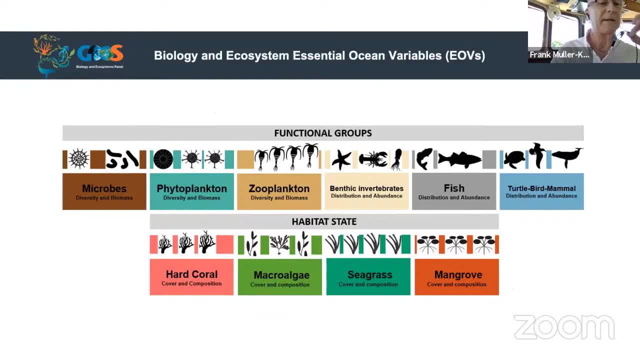 So we have hard coral microalgae, seagrasses and mangroves, And they try to go at a very fundamental level. What's the coral cover Then? what's the species of these organisms And how are they distributed? 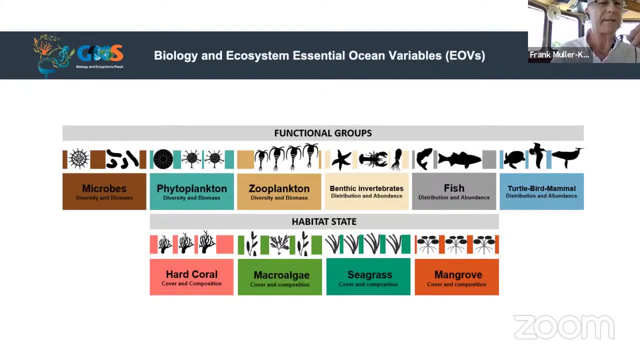 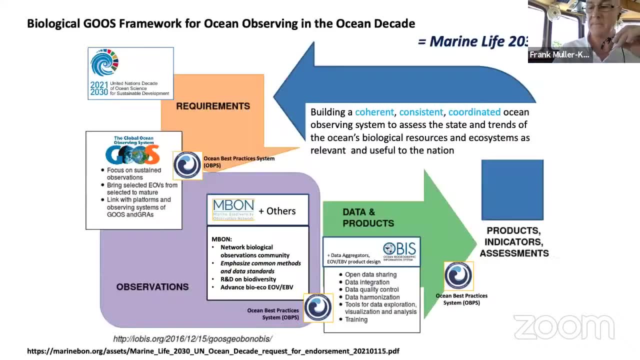 So these very fundamental levels of observations that we have to collect and organize using certain standards, And that's what the community is all about Next. So to do that, we have partnered with these different groups: the Global Ocean Observing System, AMBON, OBIS. 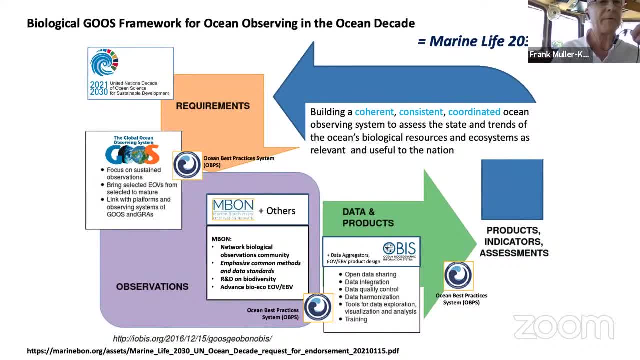 and the Ocean Best Practices System to try to develop a framework for the ocean decade that we call Marine Life 2030. So Emmett is going to talk about Marine Life 2030 later, But basically what we have is we have to establish the requirements. 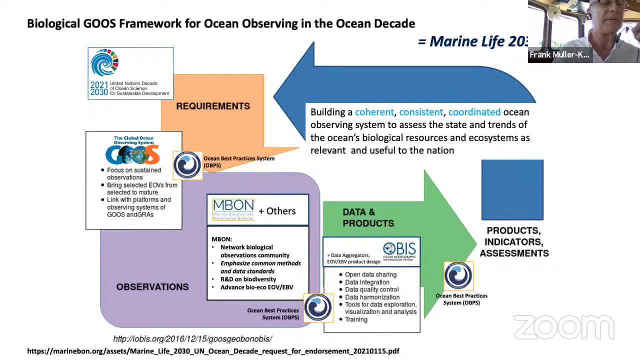 that society needs to understand the ocean for the economy, the blue economy and human health and so on. So GOOSE develops these requirements under these essential ocean variables. They follow best practices developed by the Ocean Best Practice, kept track by the Ocean Best Practices System. 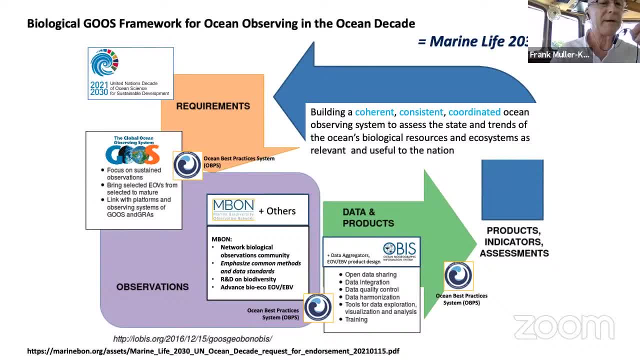 AMBON helps organize the community, developing standards and training programs, and works with OBIS, the Ocean Best biodiversity observation information system, to try to produce the uh, the database that people use them to generate the products. and you have this, this continuous loop, where you have a feedback. 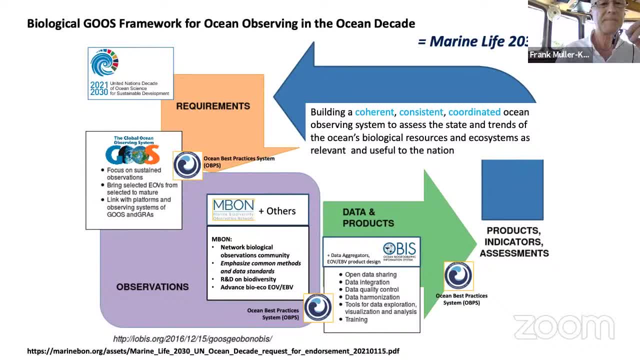 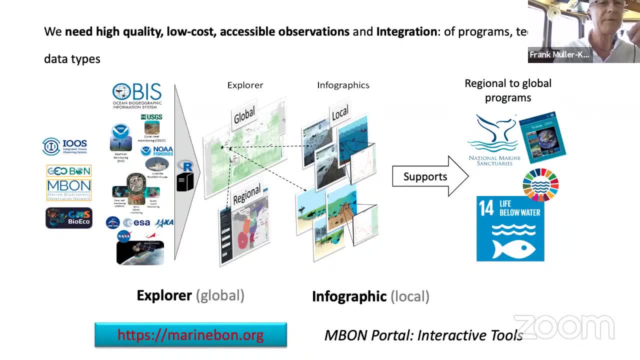 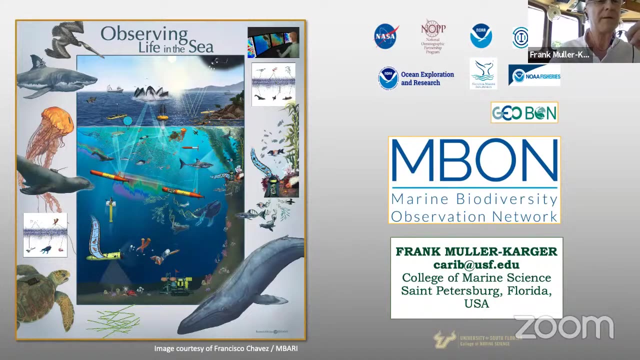 trying to understand how you improve these products. next, the whole point is to organize the community, as you see on the left, to generate products, integrating remote sensing and local data to generate products as you have in the right next place. so please join us. uh, contact us if you want. there's my email on the screen. you can write me. 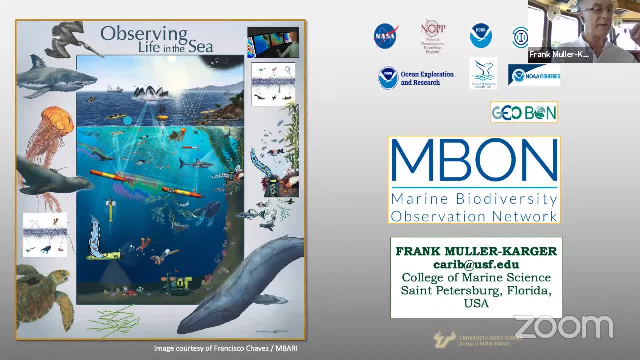 you can also join through the uh. geobon and enrique is going to talk about that later in the session. thank you, thanks very much, frank. i'm very impressed that you're actually really are at sea. looks like you're sitting in your boat. um, i guess we have to keep moving um. 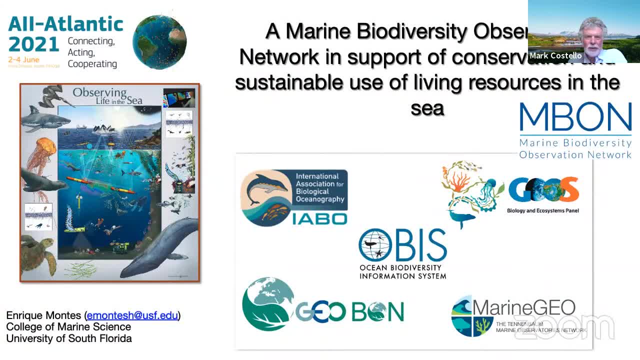 our next presentation. we have two presentations now: one by enrique montes, who's done a really um outstanding uh, networking across the americas, uh, that isabel mentioned earlier. we hope to try and replicate on the europe and africa. so the floor is yours, enrique. 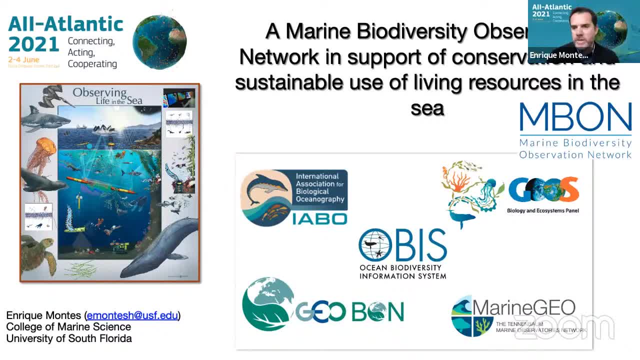 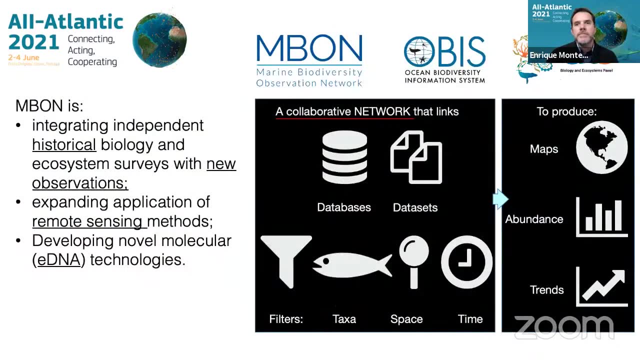 thank you, mark and uh. i will be briefly showing you some examples of of the kind of uh tools and implementations that the global emblem has been putting together over the past several years in this presentation next, please. so if you, if you ask anyone what, what emblem is? it's, in essence, a community of practice that. 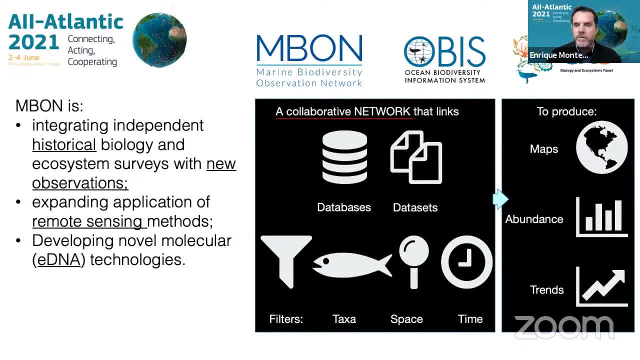 is dedicated to understanding how biodiversity is changing over time and space around the world and different ecosystems, habitats, etc. and he's doing that by uh focusing on these three key actions: uh integrating- integrating independent historical, bio, biological and ecosystem. and i think the most important thing you have to recognize is the presence of these. 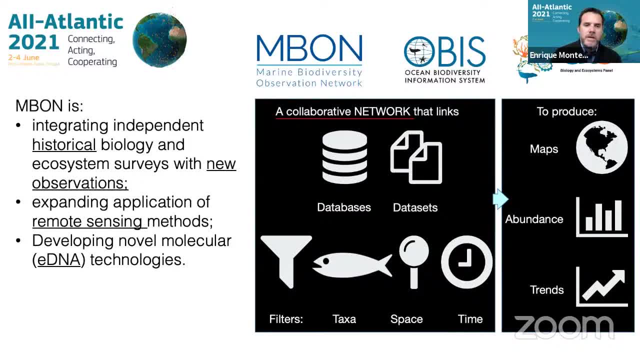 research and research tools. it's. it's something that is just so much more important than just being able to imagine, like an exact frontline scale, a very overpopulated this. this is, uh, a really interesting aspect of the Google lugan. so, looking at data in the space and the space. 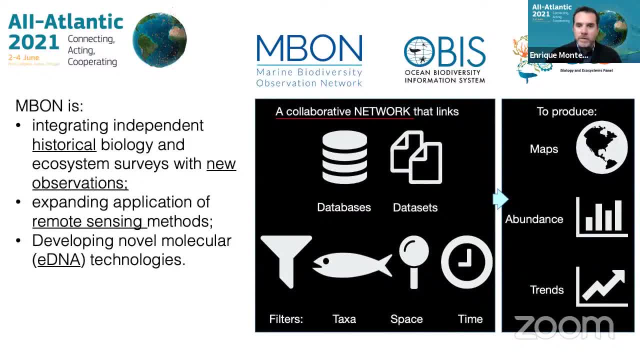 and global. so the data generation and, of course, the scientific research and development are becoming more and more important and much more relevant to the el Jeong and the development of a new set of tools, some of them based on molecular technologies, to start measuring the occurrence of taxa. 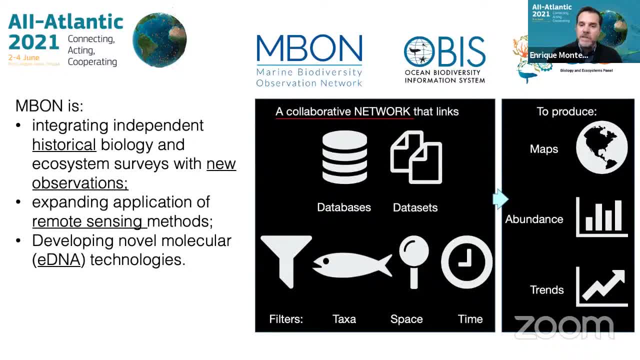 in different places cheaply and inexpensively And with all of this information. the MBON framework seeks to develop organized databases and data sets in a way that we can filter data by taxa, by space and time and be able to generate maps. 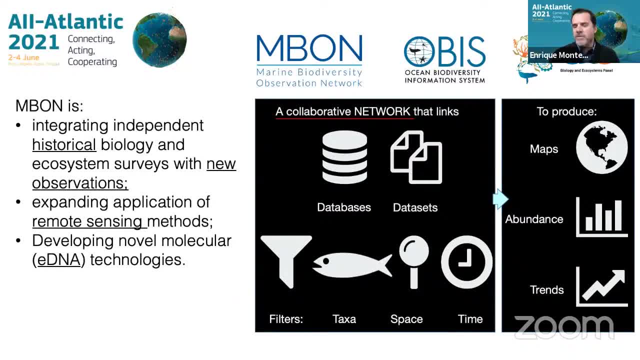 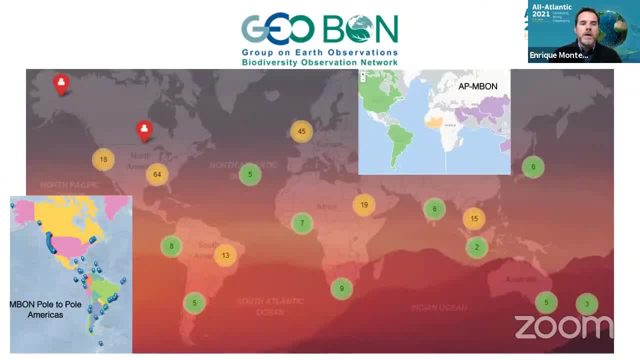 time series plots and understand how all of the different metrics and indicators of biodiversity change over time. Next, As Frank and Isabel already mentioned, MBON operates under the Group on Earth Observation Biodiversity Observation Network. It has many groups around the world. 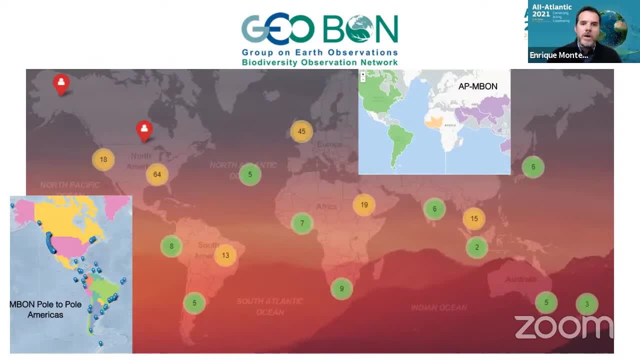 incorporating some of these elements, but I'm going to focus today on a couple of major implementations that are happening in different parts of the world. One of them is the MBON, the MBON Multiple of the Americas, And another large regional organization of MBON. 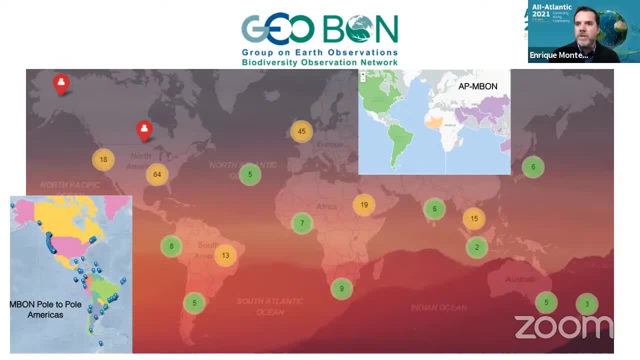 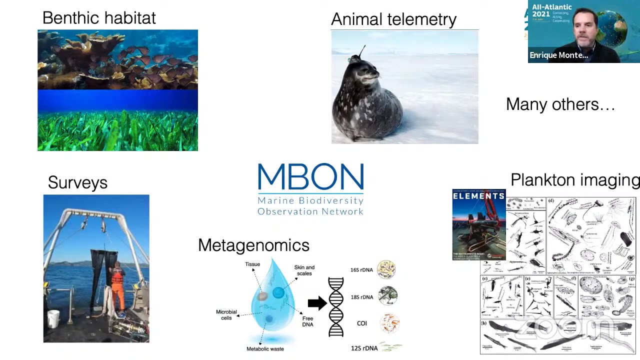 is in the Asia Pacific region that is being led by Mark Costello and others in Japan and other parts of the Asia Pacific region. Next, please. MBON is focusing on many different elements of biodiversity. It's looking at benthic habitat, as Frank mentioned before. 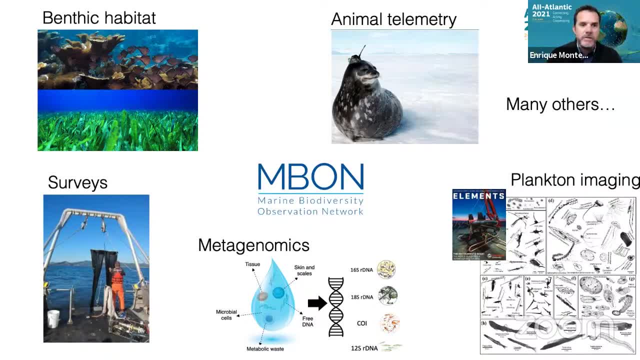 but it's also using information coming from traditional surveys, animal telemetry, metagenomics in the form of environmental DNA, plant and imaging technologies that are collected during field cruises, and many, many other techniques that are being applied and implemented, aligned with best practices. 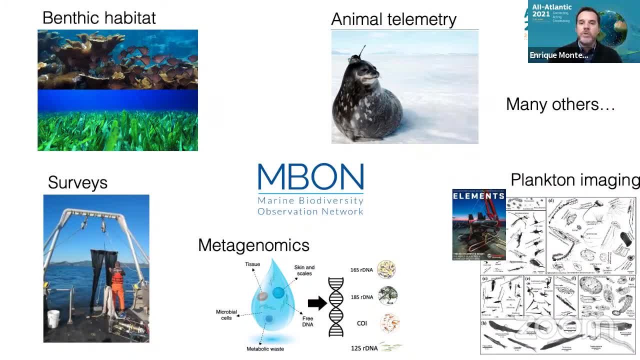 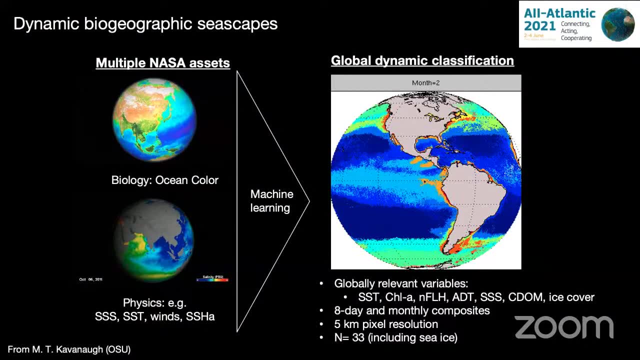 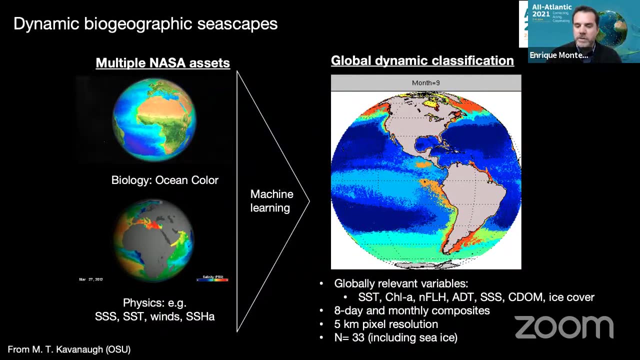 to better understand how biodiversity is changing, how food webs around the world are changing and why. Next, All of these in-situ measurements are being integrated with satellite remote sensing and, specifically, we're using the satellite seascape classification methods, which is, in essence, 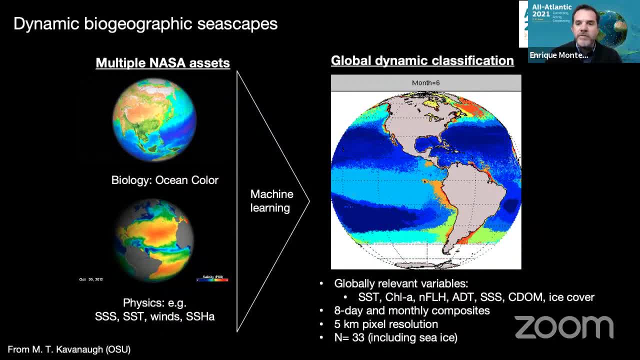 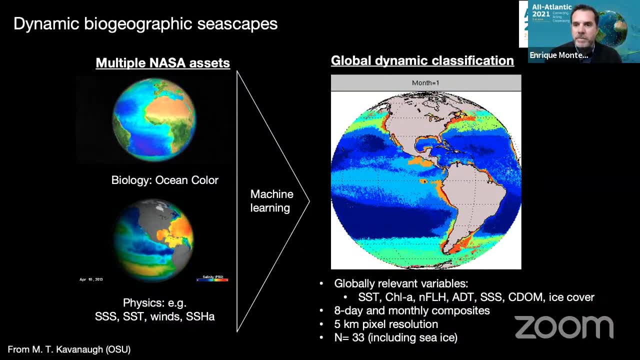 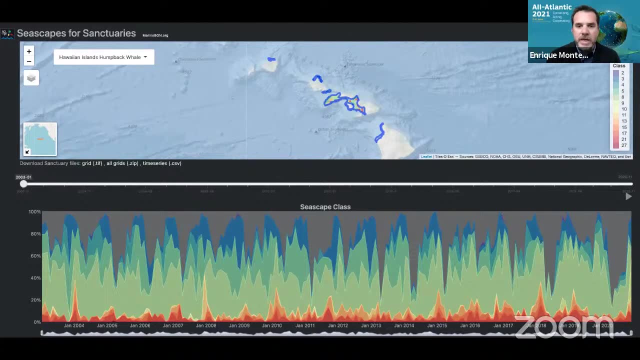 machine learning classification of different types of satellite data to understand how surface habitats, fluid habitats in the global ocean change over time and space. Next, These type of classification, for example, allows us to understand how the biogeography of a region of interest changes over time. 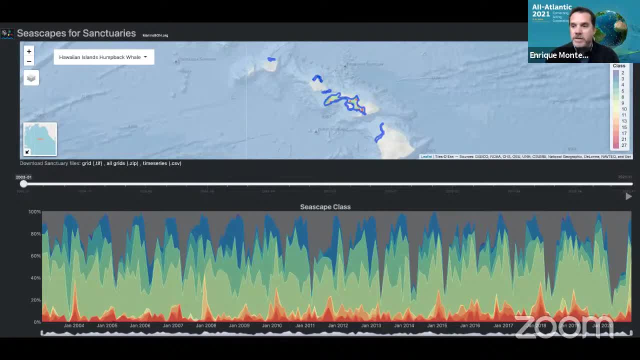 and see how each of these different classes that are being generated by this classification method expand and contract, And that, in turn, lets us understand how the biota that lives within those classes is changing over time in specific spaces. Next, The program is very focused on 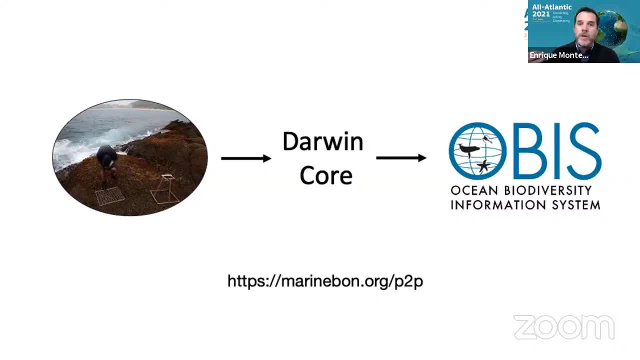 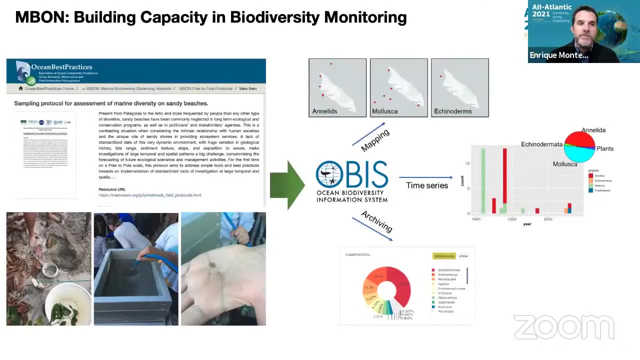 translating information that is collected on the ground to the Darwin core schema, so that it can. so these observations can be shared through the ocean biodiversity information system, And I'll show you a couple of examples of that. Next, The tool, for example. 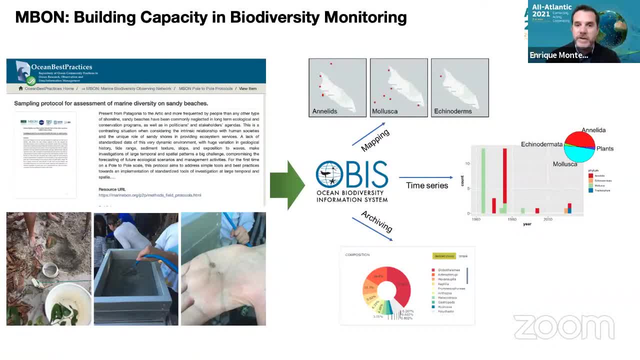 the EMBOM pole-to-pole program is developing field protocols that are standardized, that can then be, can guide data collectors in a way that then observations can be shared through OVIS And from there data can be mapped, can be represented as time series plots. 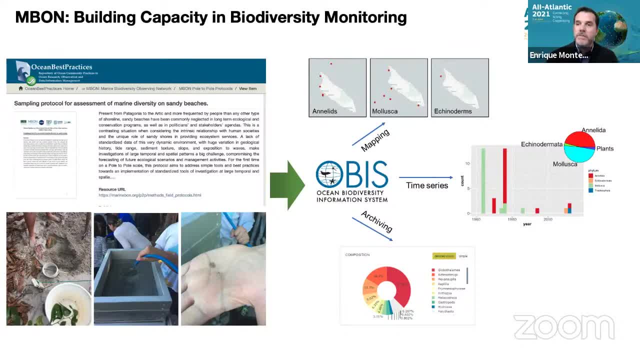 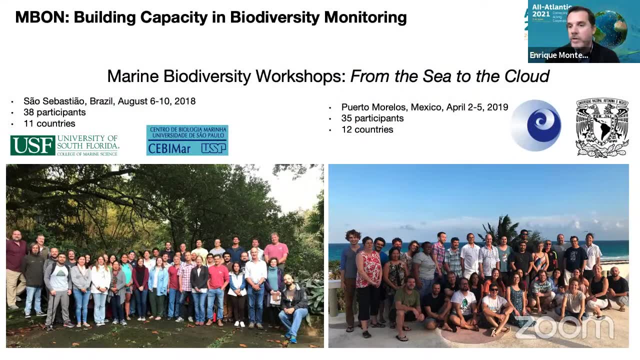 and then are permanently archived and curated in OVIS. Next, The EMBOM, pole-to-pole and other programs around the world are implementing capacity building workshops and bringing together coastal ecologists and managers to train people now how to apply these different tools and approaches. 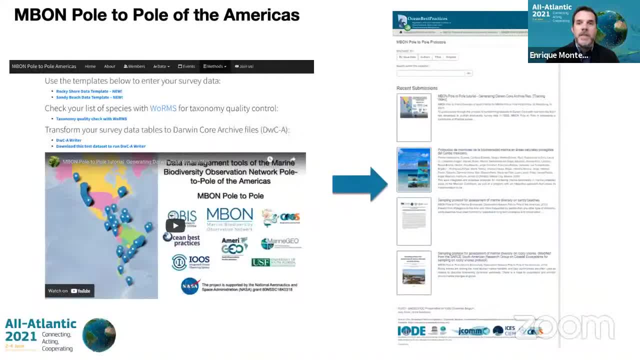 Next, And finally, all of the tools and outputs that are stemming out of these different EMBOM efforts are being shared through different outlets, but most importantly, through the ocean best practice system, to which Frank was referring to briefly, And this is a permanent repository for protocols. 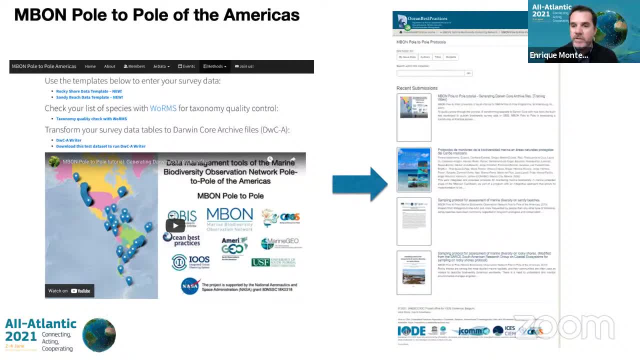 best practices and ways of measuring and looking at biodiversity so that others can adopt these tools and implement their own biodiversity observing program In their countries or regions. And I think this is my last slide, Thank you. Thanks very much, Enrique. You're all very timely. 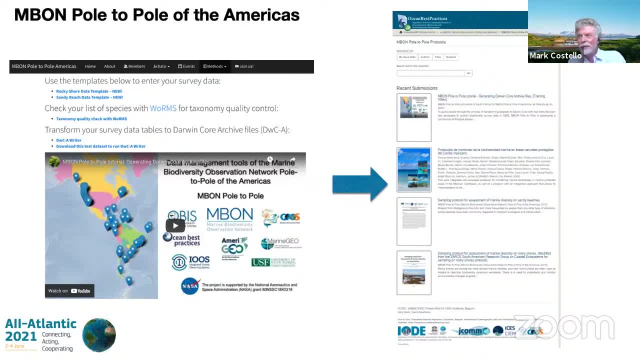 There's some questions in the chat appearing which will interest Enrique, And thank you, Lien, for answering one already. So if anybody else has questions, please put them in the Q&A box And, without further delay, let's go to the last speaker of the session. 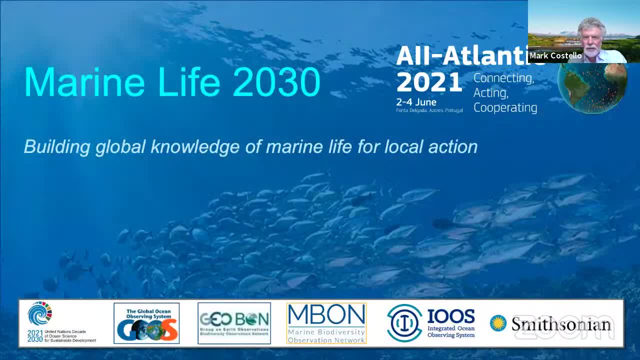 who's Emmet Duffy at Marine Life 2030, a new vision or a new vision? Emmet Duffy, Marine Life 2030, a new vision or a new vision? Emmet Duffy, Marine Life 2030, a new vision or a new vision? 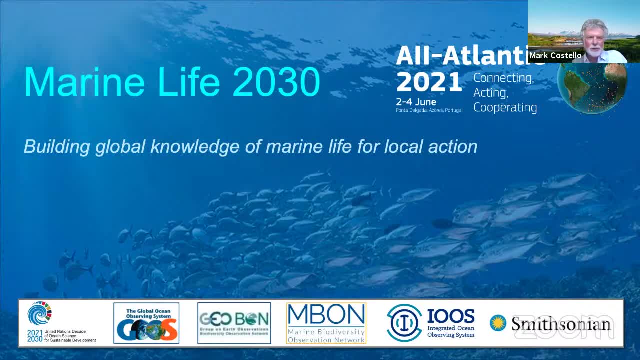 And a new initiative within the MBON community and friends. Thank you Well. first, thank you to the organizers of the All-Atlantic Conference and the MBON site event, and to all of you for joining us. It's an honor to be here. 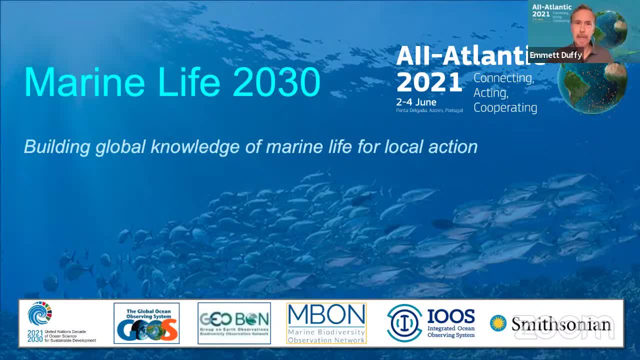 on behalf of the many partner organizations that have committed to Marine Life 2030.. This is an ambitious proposal for a program under the UN Decade for Ocean Science and Sustainability. Our goal, briefly, is to build global knowledge of marine life for local action. 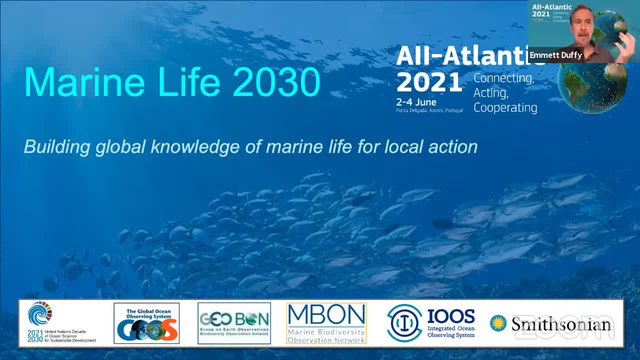 Specifically, we aim to realize and operationalize the concept of the global open access system for tracking marine life at high resolution that the other speakers have talked about in some detail. This system, we believe, needs to be co-designed with and in collaboration with stakeholders around the world. 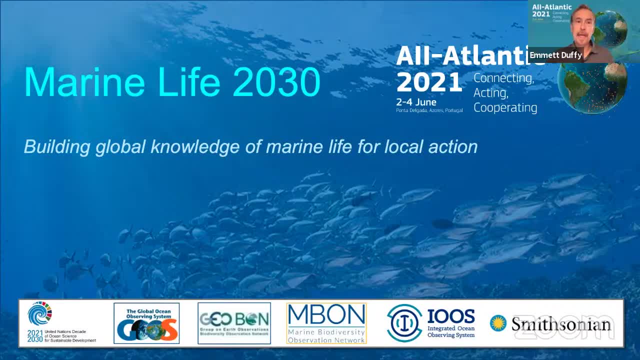 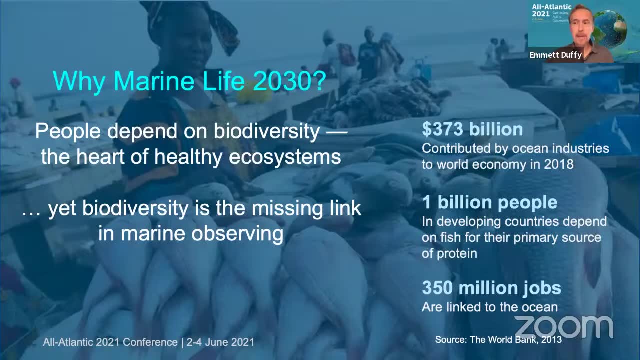 to prioritize knowledge of marine life that addresses needs of local people Next, please. So why do we need this? The simple answer is that biodiversity, the variety of life, is the heart of healthy marine ecosystems that people depend on. And yet, as has been mentioned, 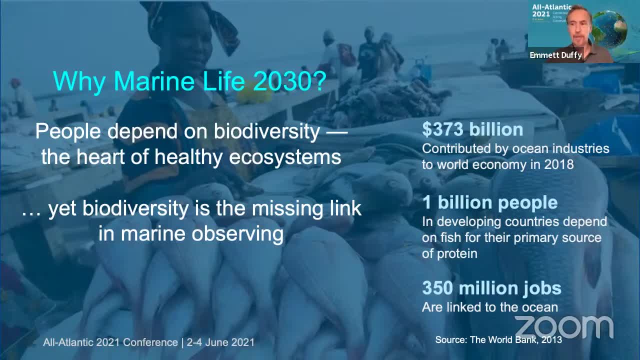 it is a missing link in global ocean. observing Wild species interacting together, govern how marine ecosystems work and how they respond, and how they respond And how they respond to climate change and other stressors. And, importantly, marine life does a lot for us. 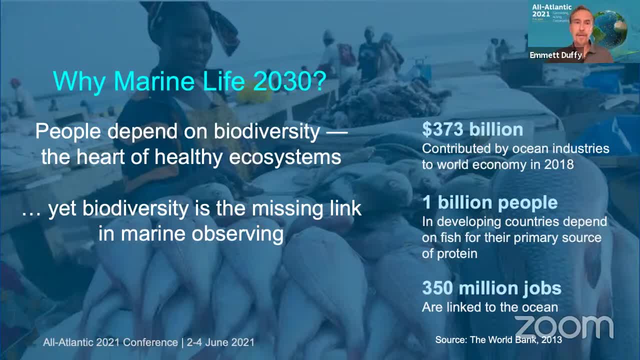 the people who live around the Atlantic and other oceans. Ocean industries contribute nearly $400 billion a year to the world economy. Fish are a primary protein source for a billion people, mostly in the developing world, and provide 350 million jobs, And, conversely, organisms that cause marine disease. 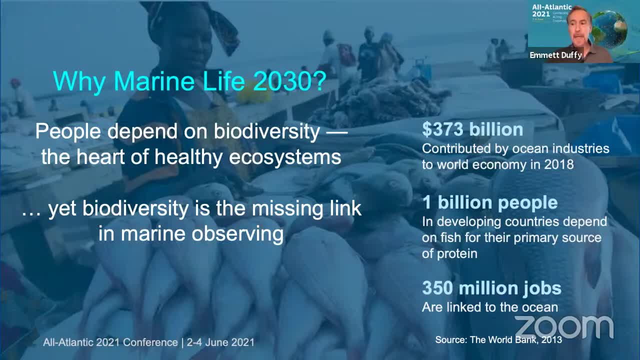 and invasive species pose threats to people and economies, And those marine ecosystems are changing faster than ever now, with climate and other stressors. All of this means that understanding marine species- who they are, where they are and what they are doing has big consequences for us. 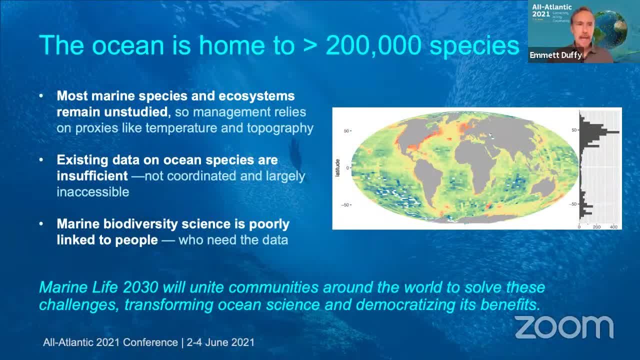 Next slide, please. So why now don't we already know these things? We do know that the ocean is home to at least 200,000 species, different kinds of organisms, from viruses to whales, which play important roles in ecosystems that we depend on. 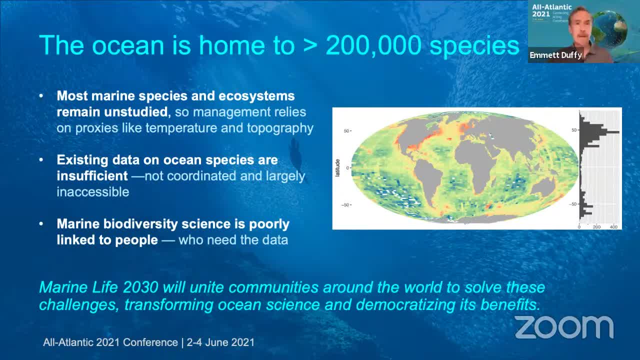 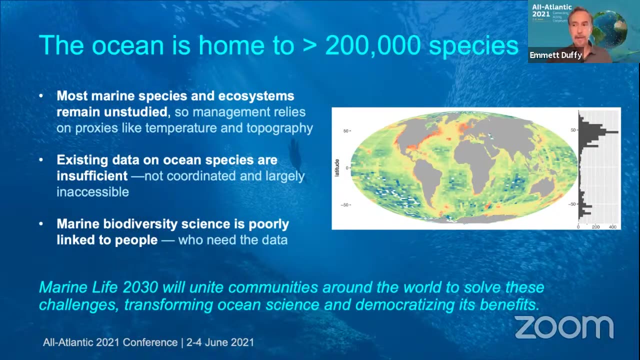 But for much of the world ocean, we know little or nothing about the species living there or what they do, And that is especially true for marine species in the developing countries around the world tropics. Yet this is where biodiversity is greatest and where people most depend on marine life. 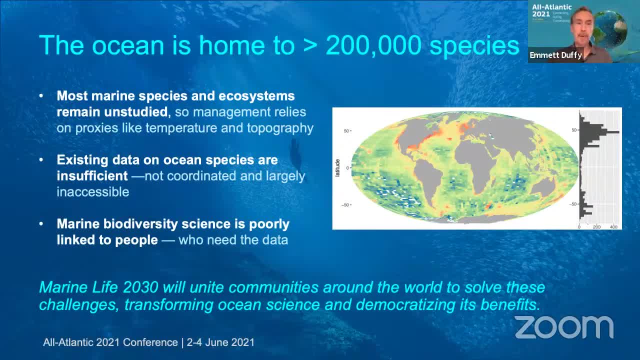 and need that information. Also, the data on marine life we do have is not well-coordinated or accessible. although OBIS and others are making very strong inroads in that direction, Much of it is not collected with people in mind, And so Marine Life 2030 aims to solve these problems. 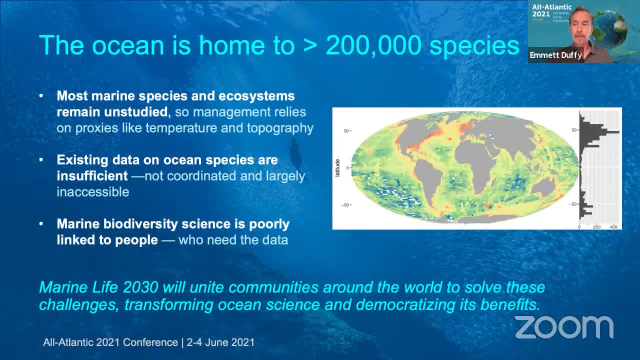 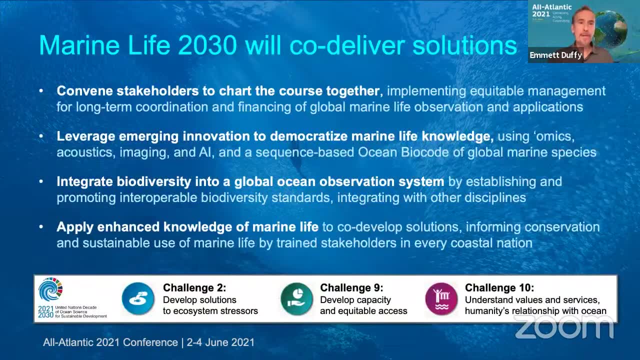 by uniting communities around the world to transform marine science and democratize the benefits. Next slide, please. So how will we do this? Obviously, establishing a working system for tracking marine life and delivering that knowledge to everyone will be a huge job. 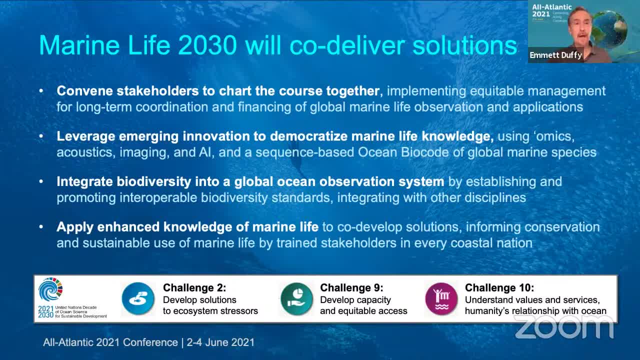 It's already a huge job. It hasn't been done, completed yet, because biodiversity is a lot harder than temperature and physics. It will require commitment of people, organizations and resources everywhere, And that is why more than 80 partners have come together worldwide. 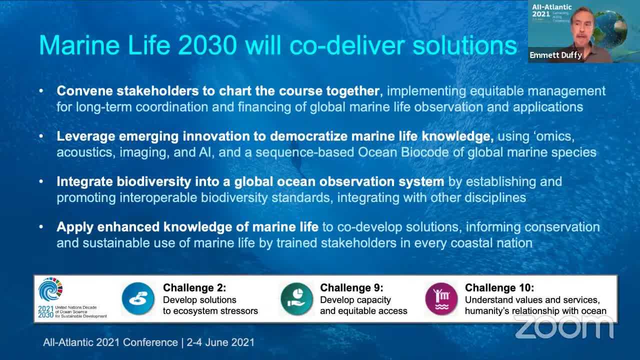 committed to make Marine Life 2030, a reality, So what we aim to do is first get everyone at the same table to design a process to make this a reality. Not everyone in the world, obviously, but we need scientists, stakeholders. 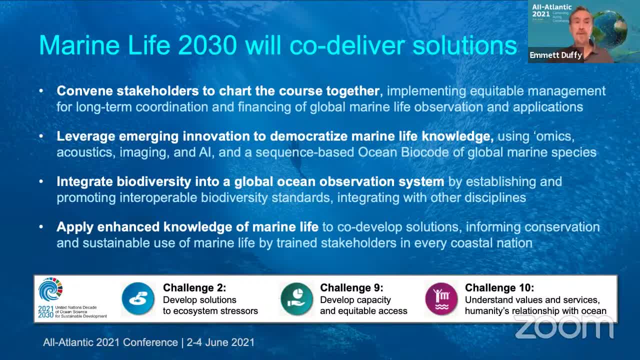 governments, indigenous leaders and so on. We do not presume to know how this will work. We need to hear from people and co-design it. Secondly, we want to make the most of emerging new technologies that reduce costs, increase the resolution and coverage. 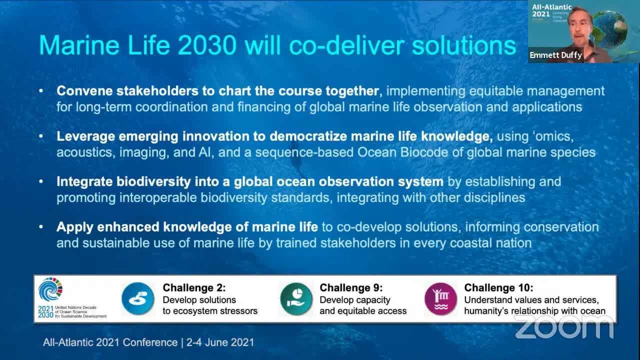 of observing and deliver that knowledge in a timely manner to people who need it. Third, we have, as we've already seen a bit, a robust global observing system for climate and physical oceanography. We need to integrate life into that system better than we have so far. 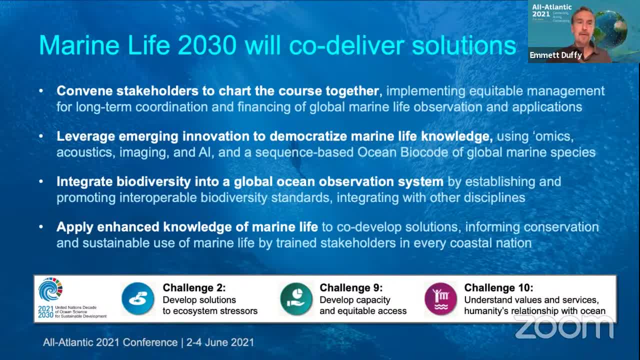 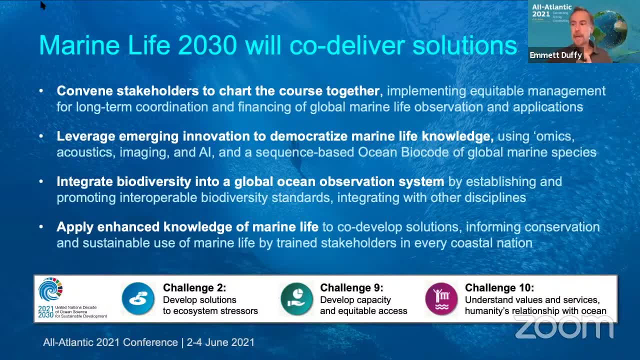 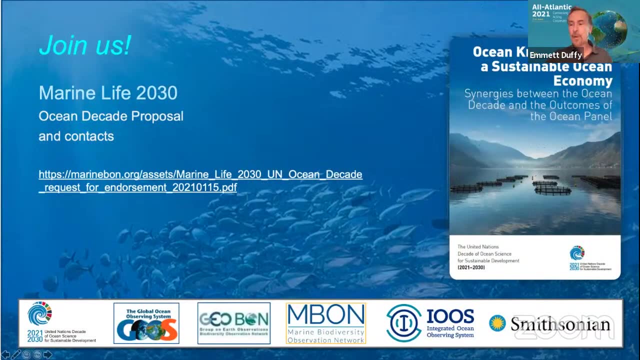 And finally, and in many ways most importantly, we need to ensure that throughout that process, the people who need information on life in the ocean are full players in designing that system And in the course of that we can solve several ocean decade challenges. 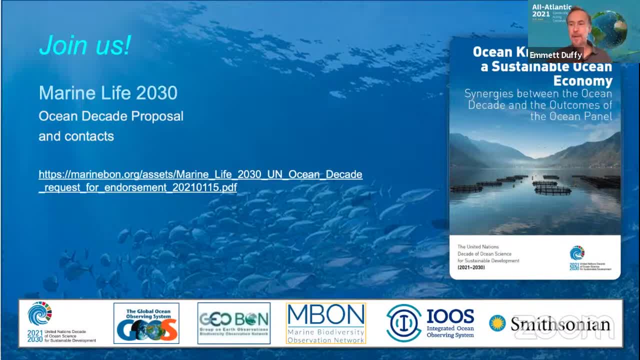 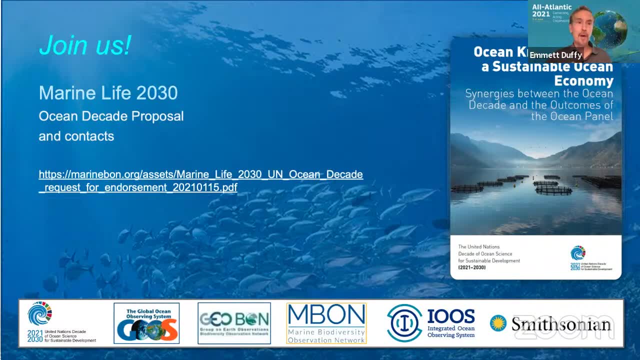 So we hope that you will join us, And I just want to note that the European Union has made major contributions so far and has a historic opportunity to demonstrate leadership through the all-Atlantic region and elsewhere. Thank you, Thanks very much, Emmet. 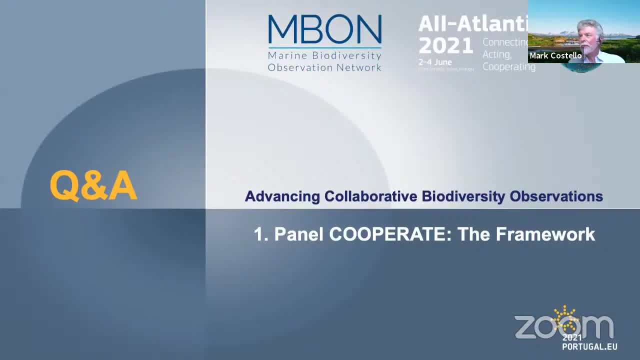 Thanks Enrique, Emmet, Isabel and Frank. We have some good questions coming up in the chat. But, Darwin Core, they're partly answered, But I think there's an extended data schema now in use in OBIS which includes sample information. 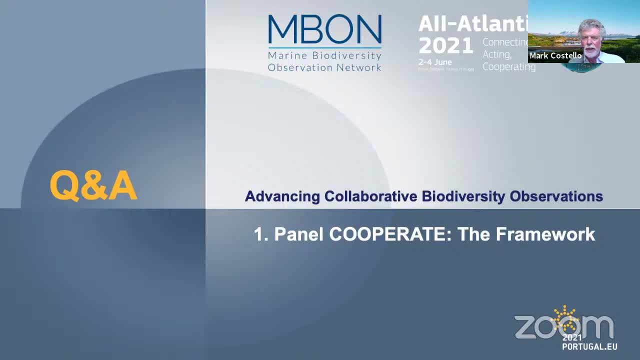 and abundance, And already a lot of this information is in OBIS. And we have a second question from Claude about local changes over time. Yes, they can be recorded in Darwin Core records, And I'm just thinking with our time left. 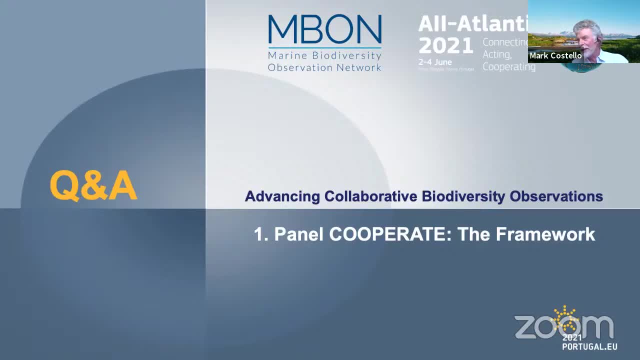 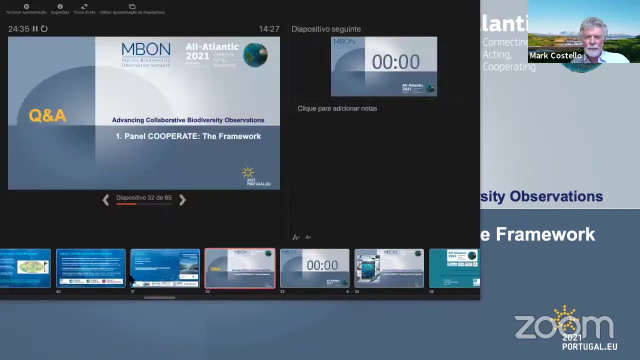 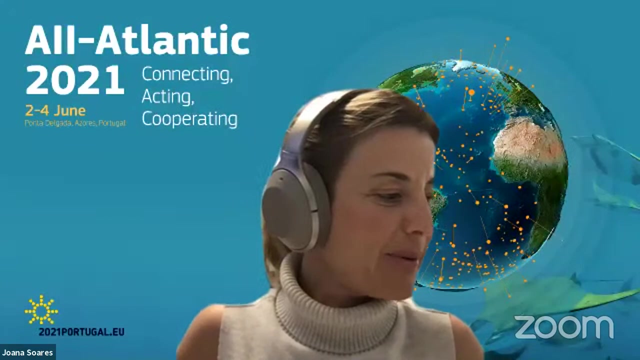 is it more effective to just use the Q&A? Do we have to finish in exactly three minutes, Joanna? Is our time actually ending or do we have a little bit more time? Sorry, I was with a technical problem. Yes, we have until 2.30, at least. 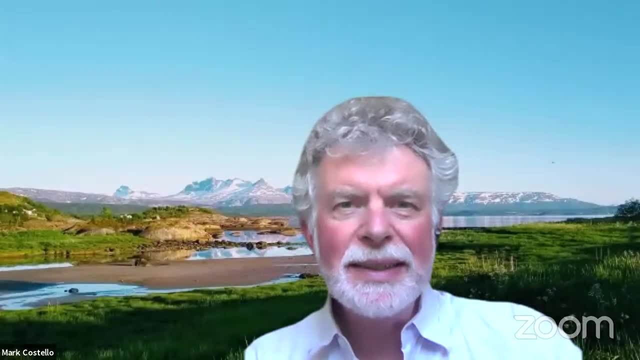 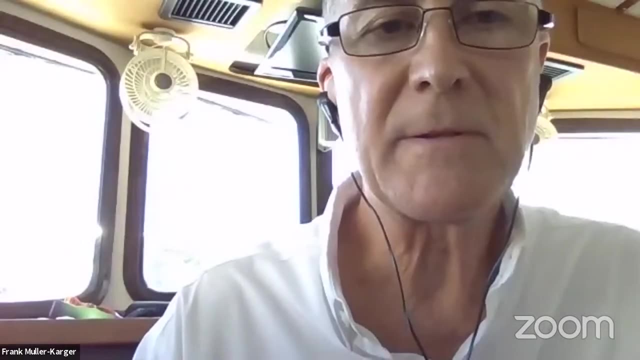 At least OK. So well, we have, Oh, only then. OK, So we have two minutes left. Are there any other questions? Can I answer that question, Frank, on the time? Yeah, I think that the issue of how you record data in Darwin Core. 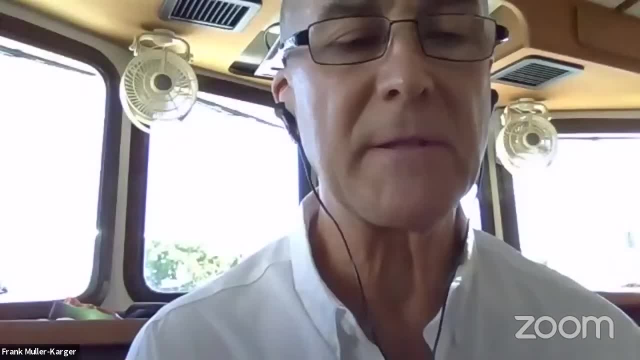 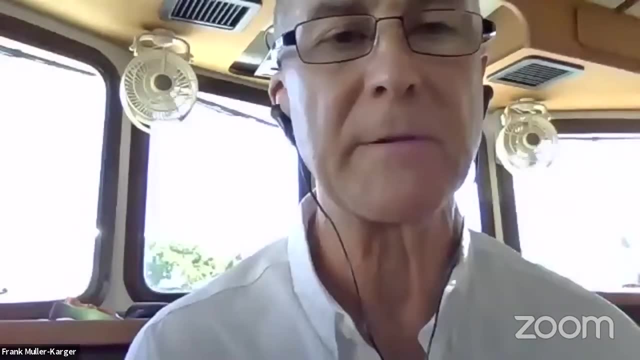 and how you link to other standards is pretty critical. But it's not just the Darwin Core standards, but also the metadata standards. Yeah, Yeah, Yeah, If we. this is part of what we're trying to do is help people understand the different standards. 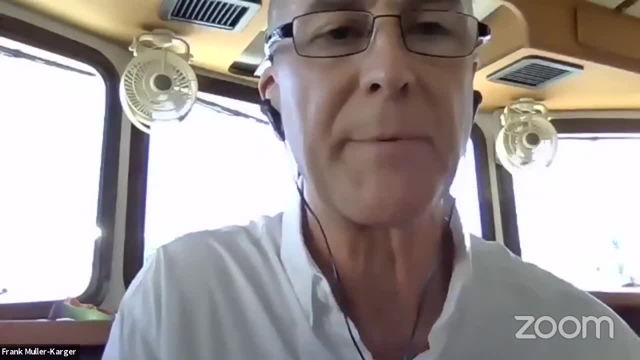 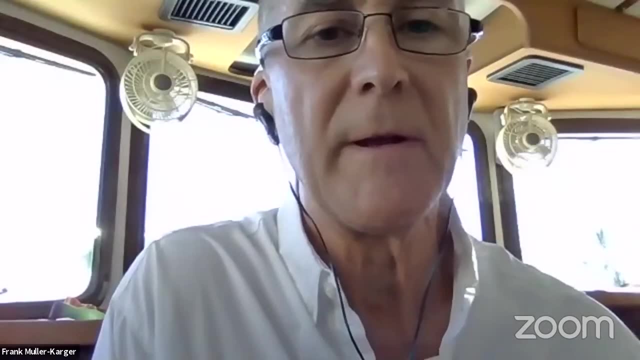 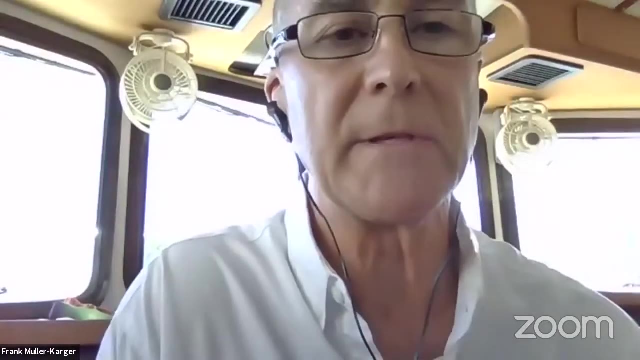 train people on how to record data with proper metadata, Because I think that the person that put the question is completely right: If you don't know the right metadata, how you link to physical and biogeochemical variables, which is exactly what we're trying to do. 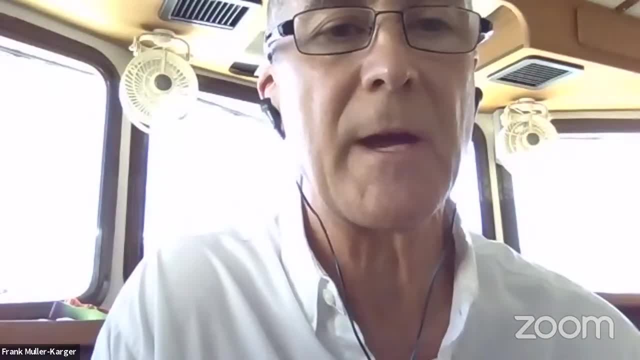 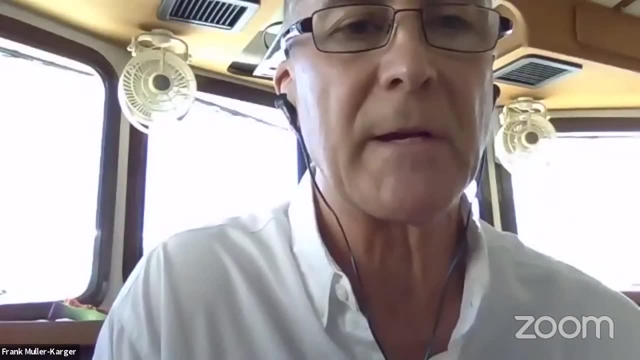 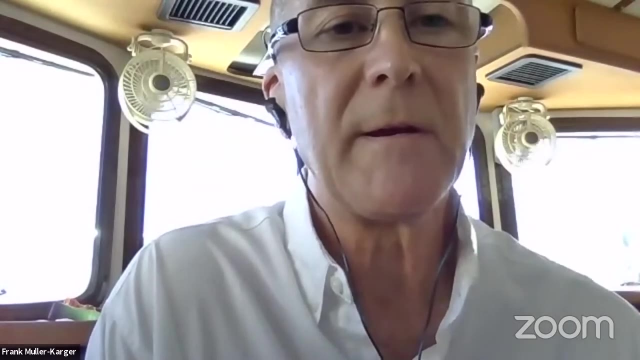 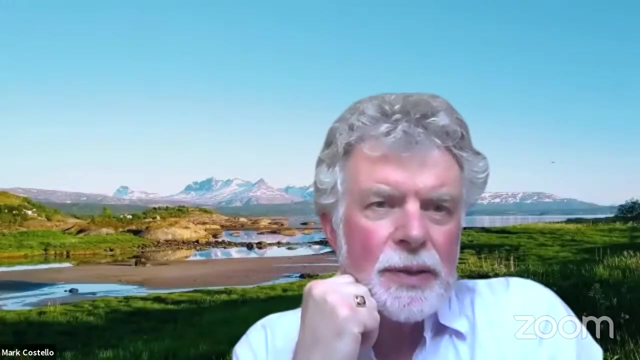 this is not just about biology and nothing more. We have to integrate into the global ocean observing system And to understand whether the changes are due to biological processes or chemical or physical processes or people socioeconomic processes. Thanks, Frank. Yeah, And I think, the key problem that Emmet and Enrique have mentioned. 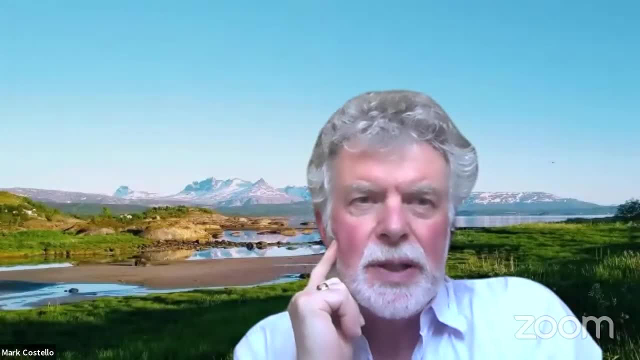 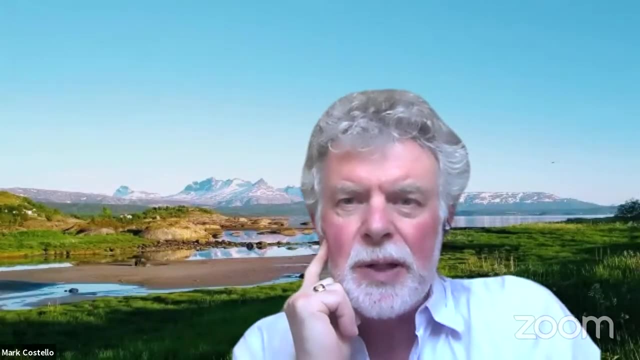 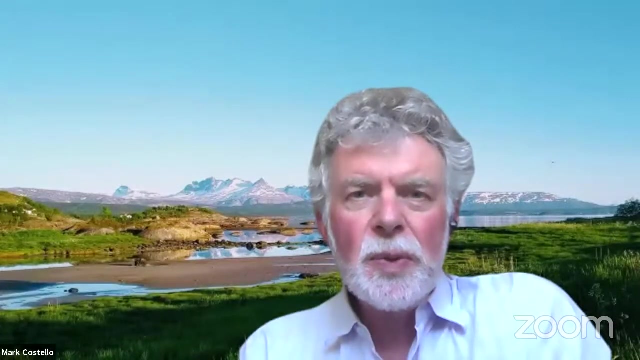 as well and all the speakers- is the timeliness of availability of data. We need to collect more data and make it available faster to be relevant to local communities as well as policymakers. I'm just checking the chat again. I think these presentations will be available afterwards, Joanna. 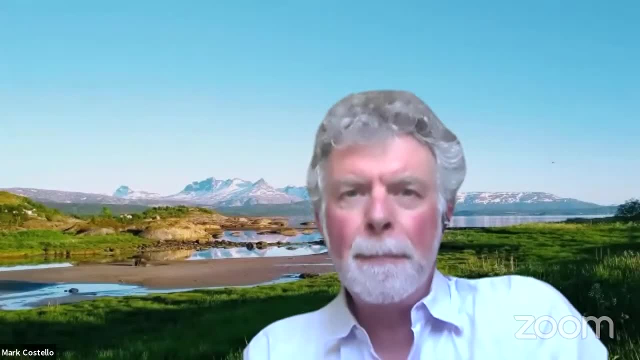 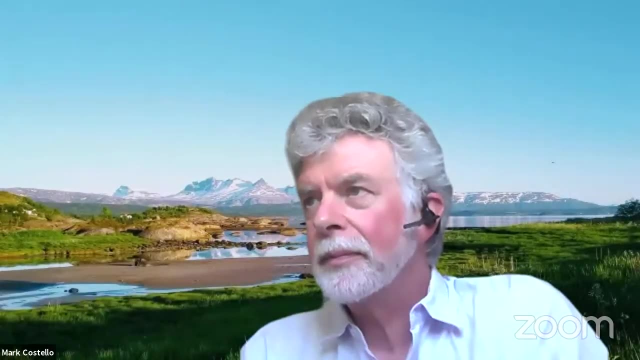 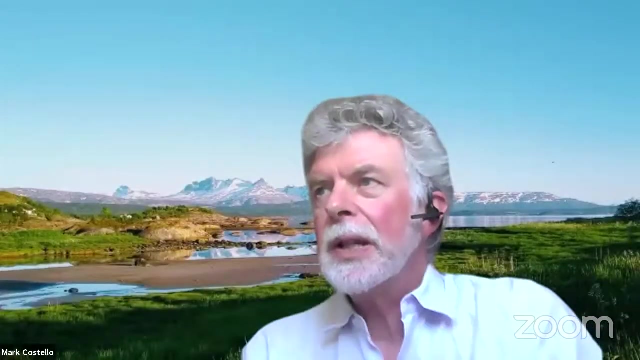 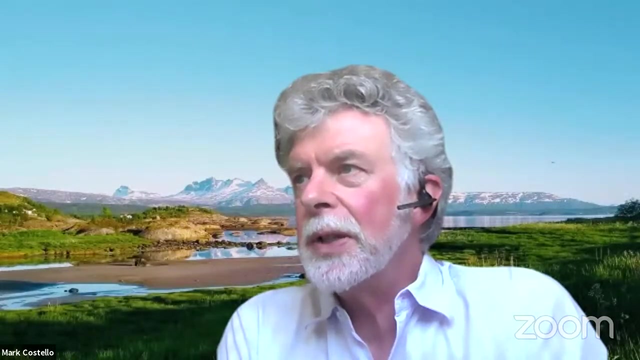 somewhere from the conference? Yeah, If we'll get an email on that. Yes, I will make them available for everyone. Yeah, Dan Leer has a question about the goal and the gaps around the coordinated creation, archiving and publication of data products. 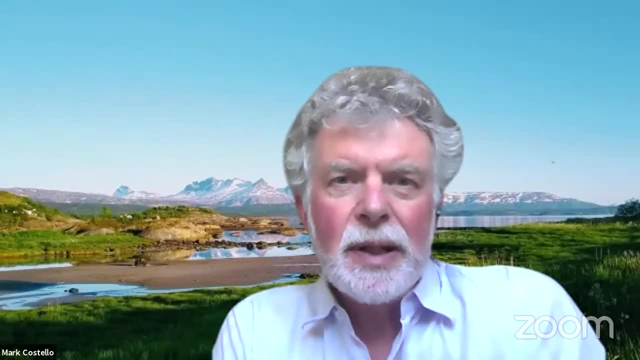 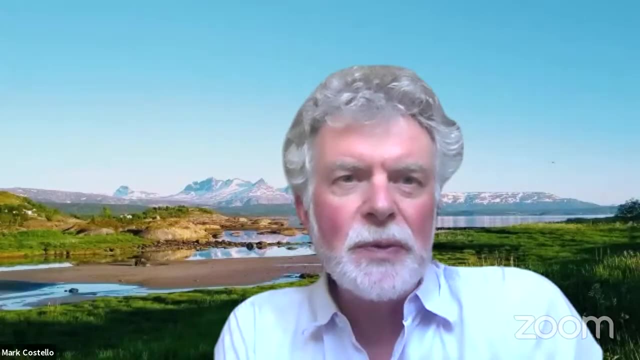 Yes, I guess that this touches on how comprehensive and representative the data is. This has been a discussion for many years And this is one of the things the EBVs and EOBs are aimed to: focus on particular key variables that should be measured. 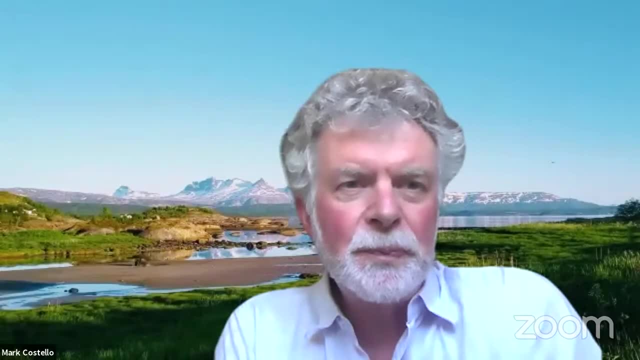 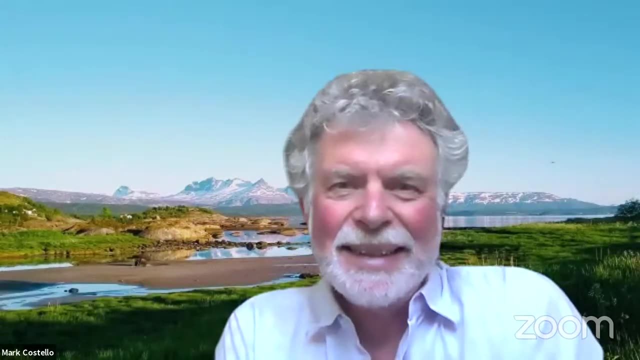 But I think in many cases other things have to be measured with them And I don't know how we address that. But I think it's important to address this problem of gaps If there's any solutions, No hands up or anything. 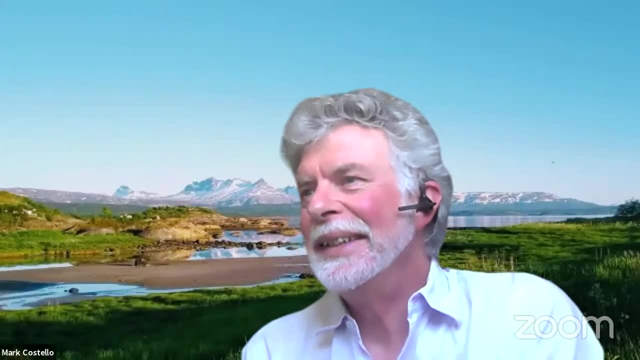 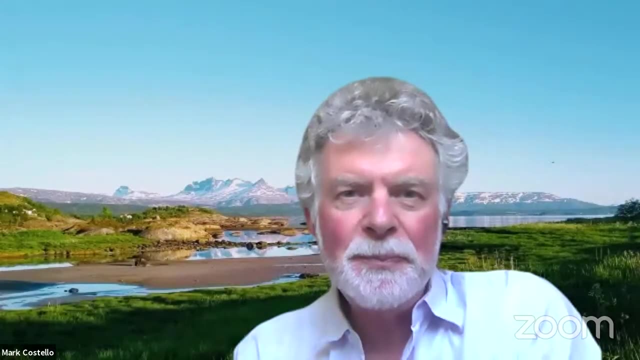 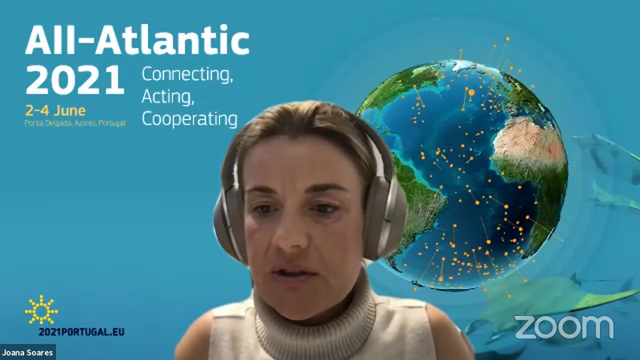 No, I think our time is up, isn't it, Joanna? We have to finish, bang on time. Well, if we have more questions, I think that we can go with the questions and skip to the next panel. I think we have a five minute break. 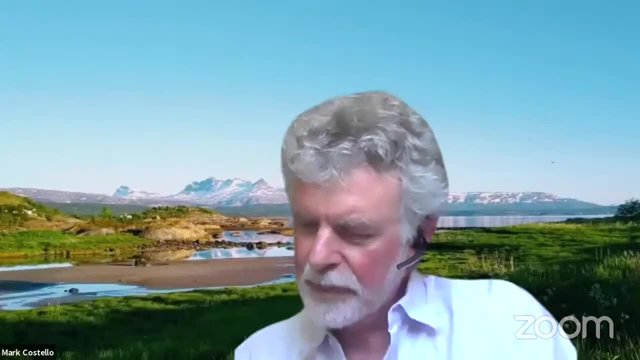 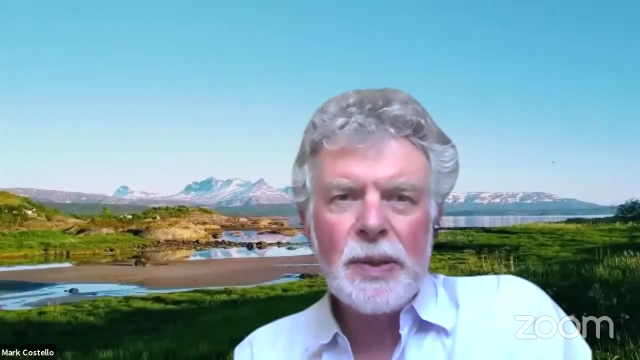 We have a five minute break. It was only five minutes. We have a five minute break. OK, Yeah, we'll start the second panel at 2.35.. OK, So some people might want to take a break, But we'll stay here if there are any questions. 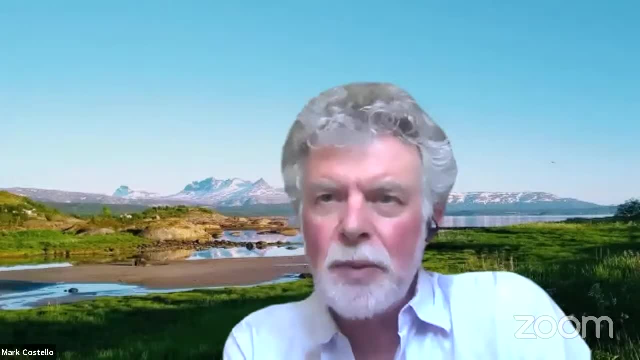 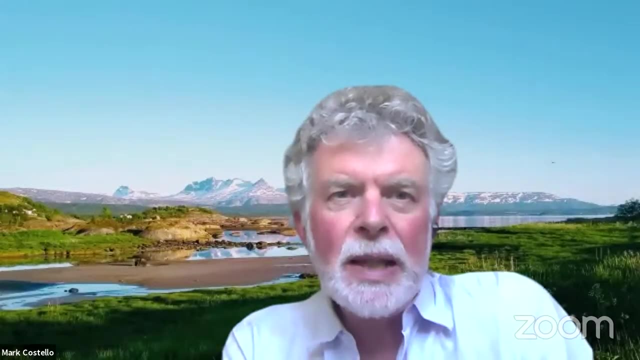 So I think people who have not been involved in MBON before you can register through the GeoBON website and then select MBON as your preferred grouping, And it's a conversation about how we collect data more efficiently and to collaborate with other people. 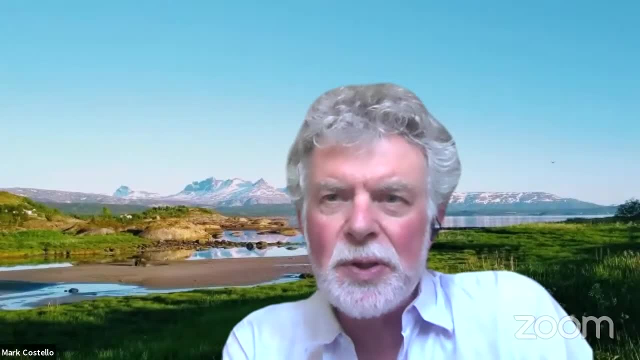 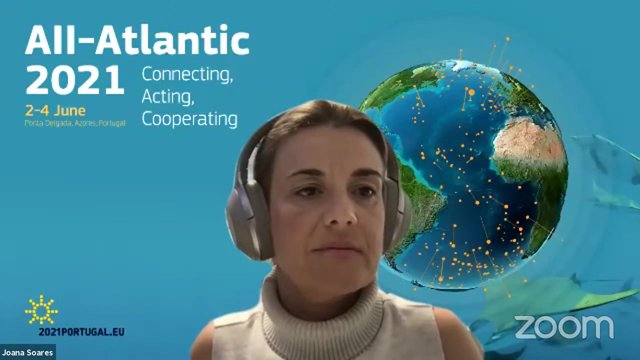 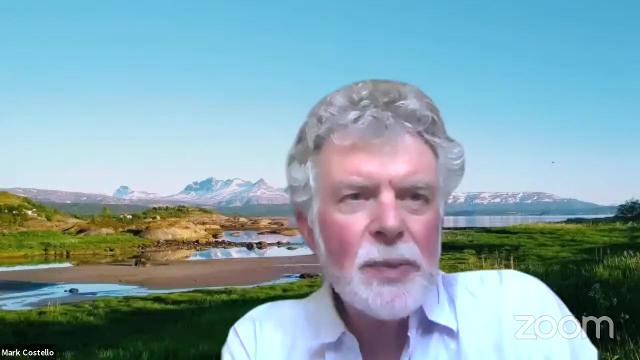 And we all have to gather our own resources and time to do this. unfortunately, MBON and GeoBON don't have their own core funding to give to members. OK, So I'll ask the four panelists If there's any comments you want to make. Isabel Emmet. 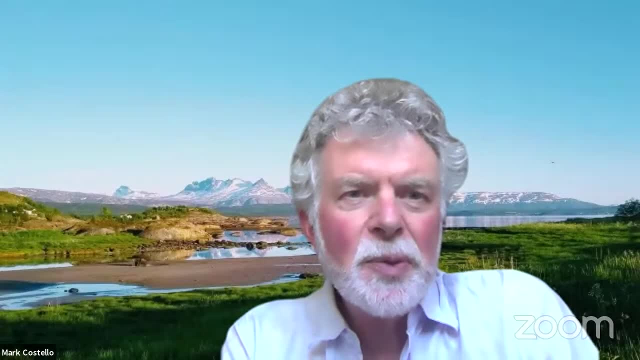 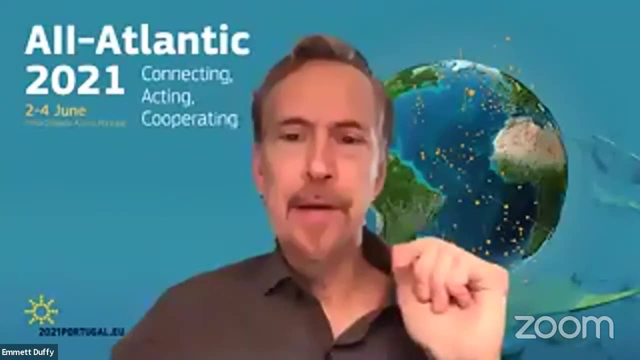 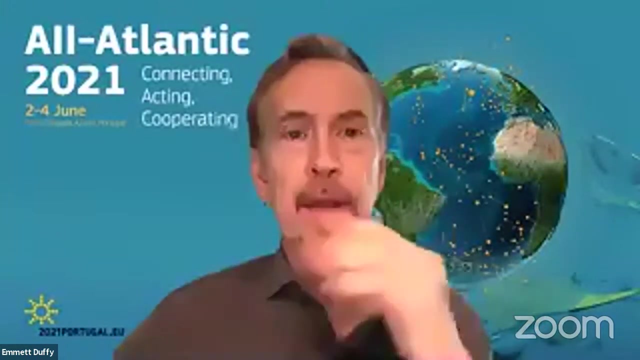 Enrique or Frank, if there's anything you want to add that you think, Emmet? yeah, Yes, there's just a question from Claude Nozarez about the barcode of life database and what role that might play What I have not mentioned in the Marine Life 2030 summary. 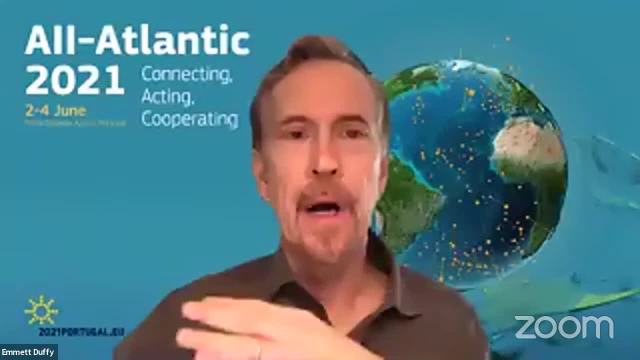 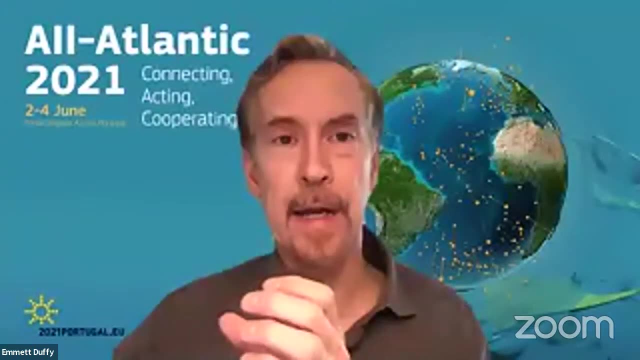 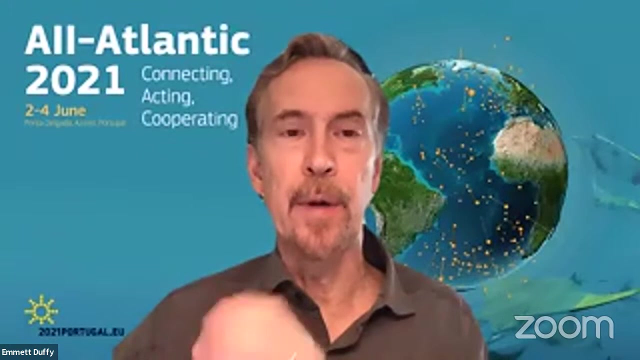 is that we see a very important aspect of again developing the capacity for this as developing the molecular sequence-based library of marine life. So that means developing barcodes that are connected to taxonomically vouchered specimens and images, and available And bold is the obvious place for those to live one of them. 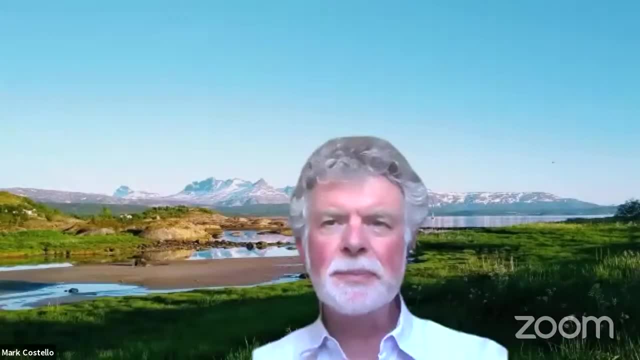 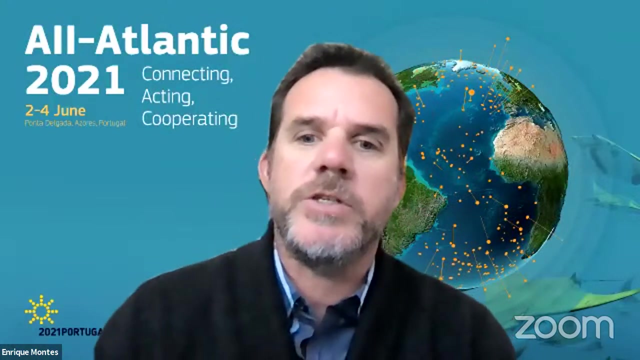 at least. Yeah, Thanks so much. Yeah, Isabel, did you have your hand up? No, Enrique, Very quickly. So, Mark, I'm going to type in the link to the website for the Poll to Poll, which is a sort of original demonstration. 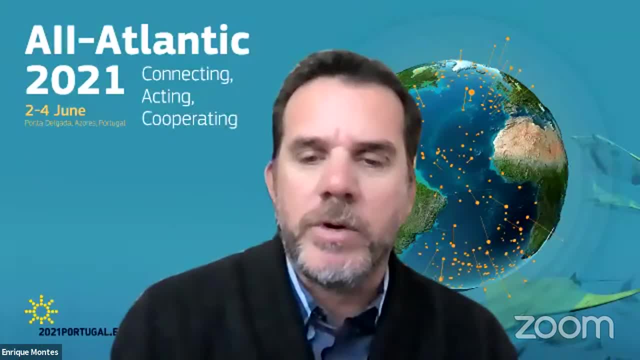 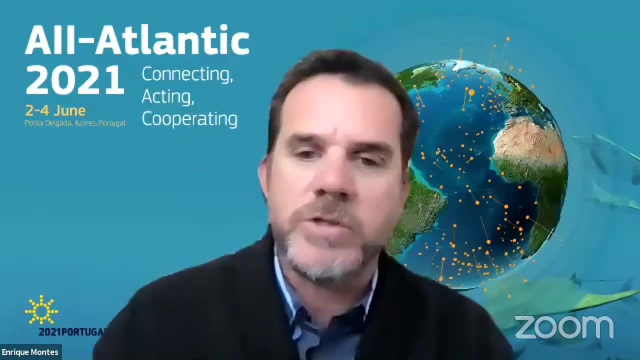 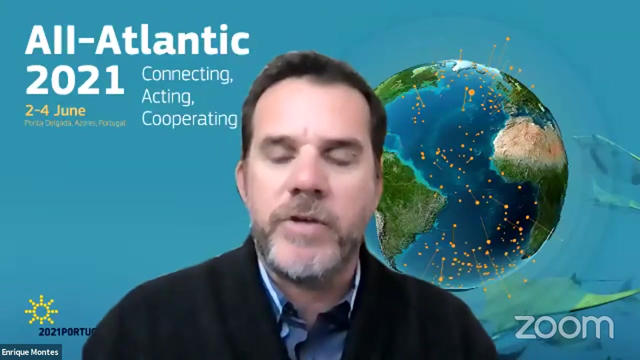 of an international program so that people can reach out to me or us and learn more about the program, And if anyone is interested in developing similar efforts in other parts of the world, like linking up Europe and Africa to develop a similar demonstration, I would be very interested in collaborating. 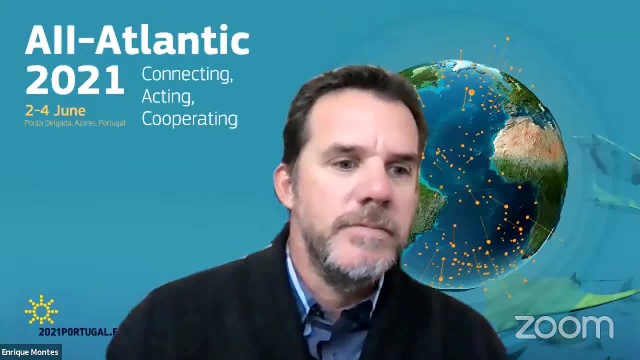 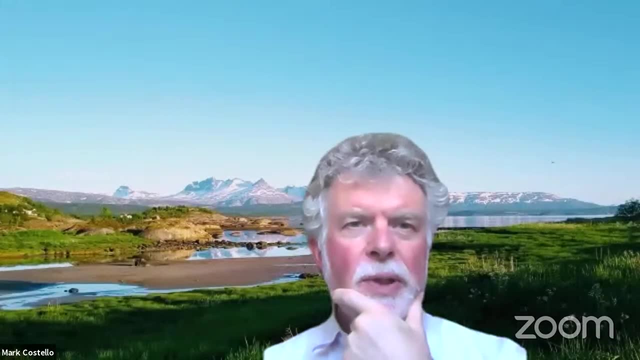 with you and working with you to achieve that. Thanks, Enrique. OK, I think we should take at least a two-minute break and everybody should do a stretch or your favorite dance, whatever you need to do before we settle down again. Thank you very much to all four speakers. 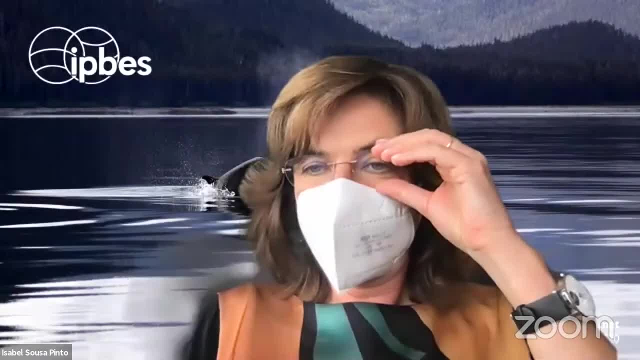 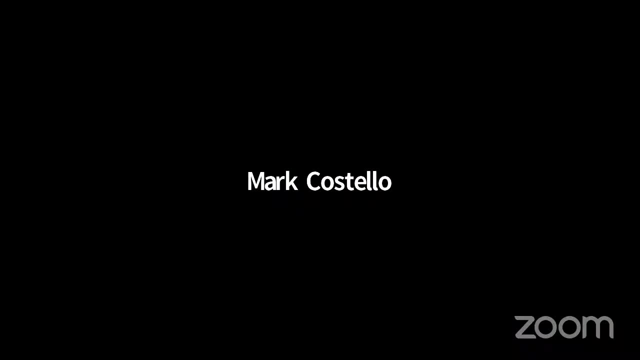 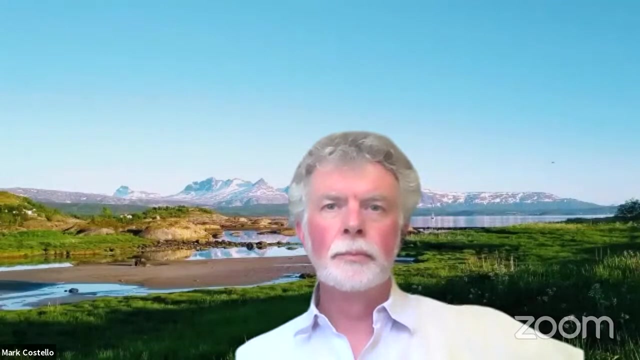 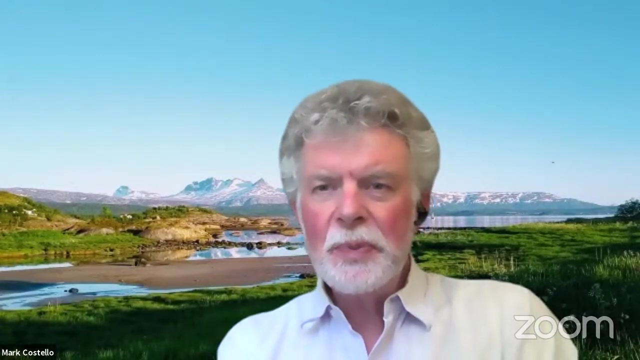 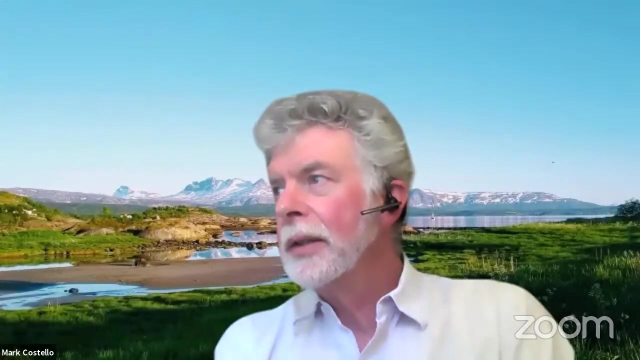 and the very good questions in the Q&A. Very good questions, Thank you, Thank you, Thank you You. Okay, I think we should get started. We have five minutes per speaker and then some minutes for discussion. Joanna, can you get the first slide ready? 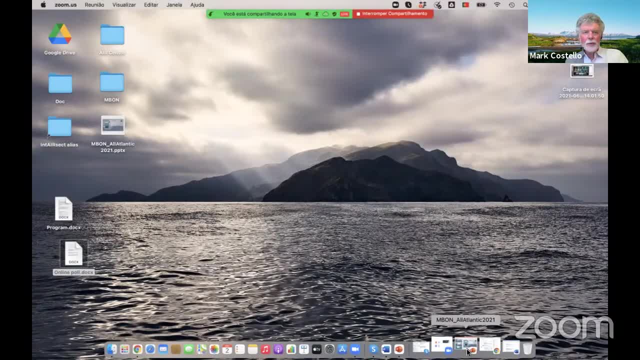 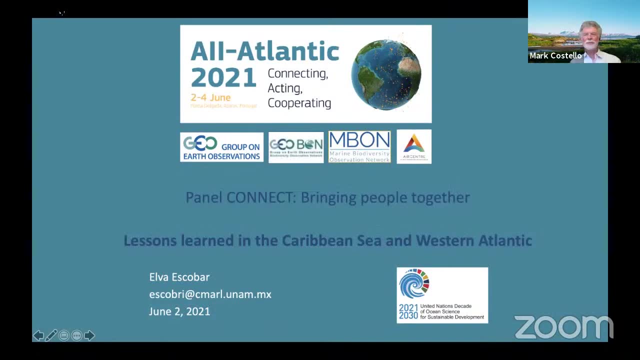 I think Elva is here. She's the first speaker. Yeah, I see Elva there now, Thank you. I'll start with a little paragraph in Spanish, which is: it's a paragraph from a poet, from Cuban poet, and when bringing people together, 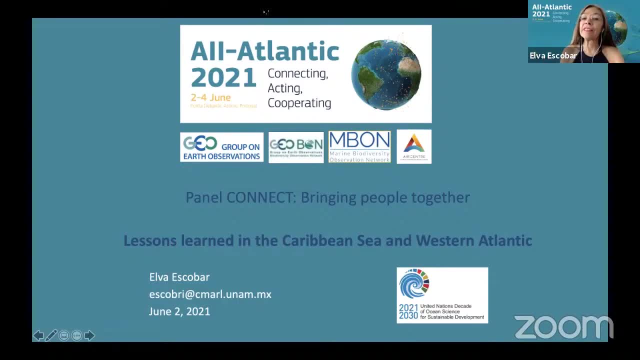 we take into account that the Caribbean Sea and the Western Atlantic seascape is 80 times larger than their land areas. for the sustainable use of this extended, warm, biodiversity rich ocean that contributes to economic growth and resilience. A Western tropical Atlantic region workshop for the UN Decade of Ocean Science for the 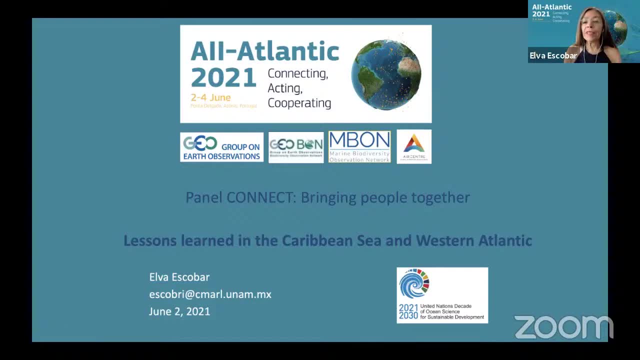 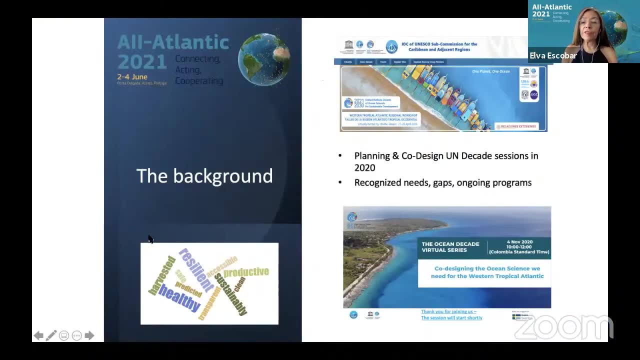 Sustainable Development 2021, 2030 took place. next, please, took place in April 2020, and a co-designed Western tropical Atlantic regional workshop in November 2020.. Next one, please. Results from the workshop: dialogue in the region. recognize that the Caribbean region. 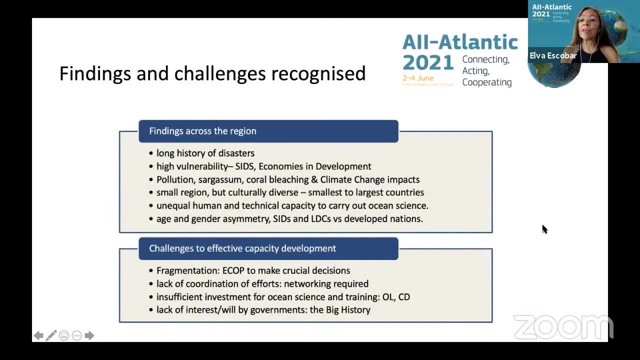 is among the world's most vulnerable to the impacts of climate change, recently highly impacted by sargassum, Massive beaching, harmful algal blooms and reduced fishery. There is an uneven distribution of ocean science capacity. Not all have access to the information, knowledge, technology or skills to make or implement. 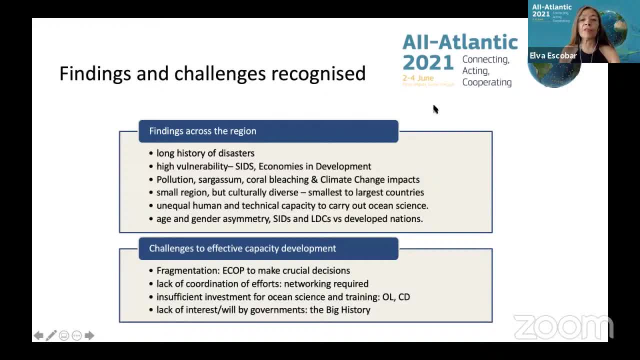 informed decisions regarding the ocean across the region. Age and gender asymmetry exists. Capacity building is urgently required When bringing people together. ocean data sharing and open access can ensure that the ocean is accessible. A variety of societal groups have access to data, products and services. 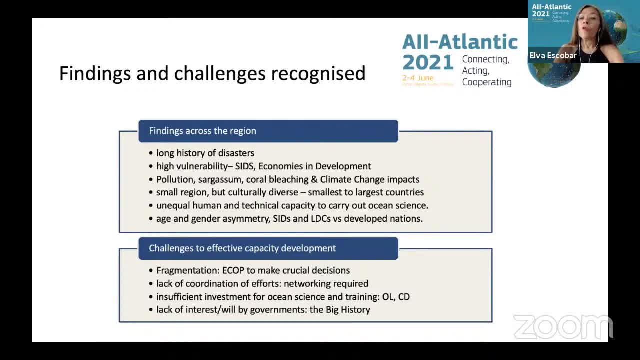 These are far from being open access in the region. Ocean science can connect sustainable development and management of ocean resources. Most nations in the region lack a specific strategy focusing on the ocean and SDG 14, its targets and indicators. Tourism is important in the region's prosperity and has severely impacted by the COVID lockdown. 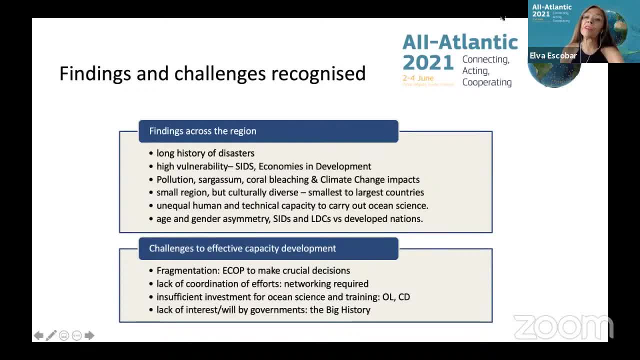 measures Declining And prioritizing job prospects, in particular, the women. Disasters such as hurricanes, flooding and erosion threaten lives, homes, jobs and infrastructure in the region shares global problems, including environmental degradation and marine pollution. Some small island developing states have considered enhancing tourism, fisheries and aquaculture. 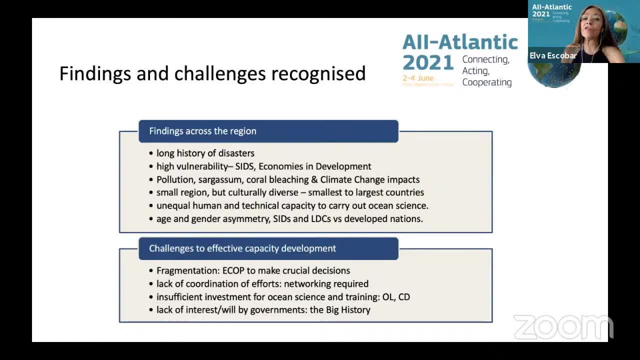 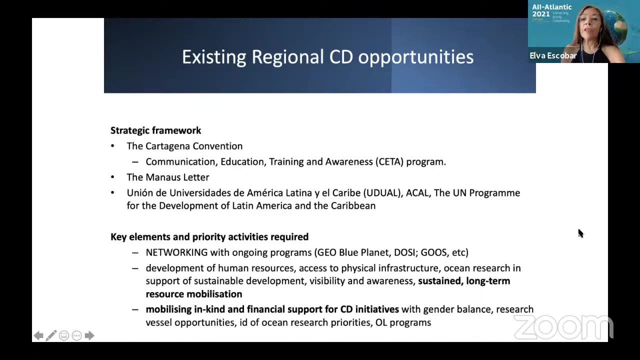 and waste management to boost economic recovery, help create jobs, to connect and bring people together, To help reduce, with science, the marine pollution And will allow them To a blue economy, sustainable portfolio. post-COVID-19 recovery Next, please. Solutions require partnerships, networking, investing in blue economy and robust science. 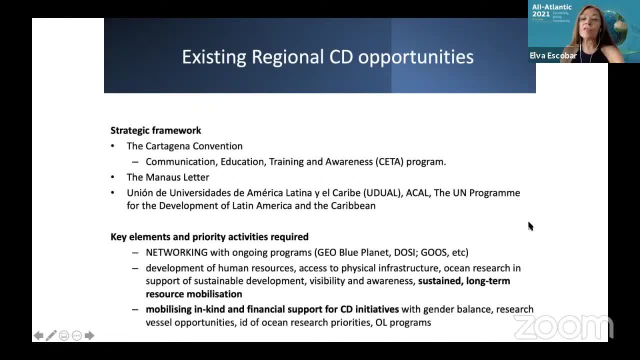 Regional capacity development opportunities exist in the region. Some are listed here. Among them the Cartagena Convention. No, I think We jumped one more. I would like to have the previous one. please, Let me see, I'm a little bit lost. 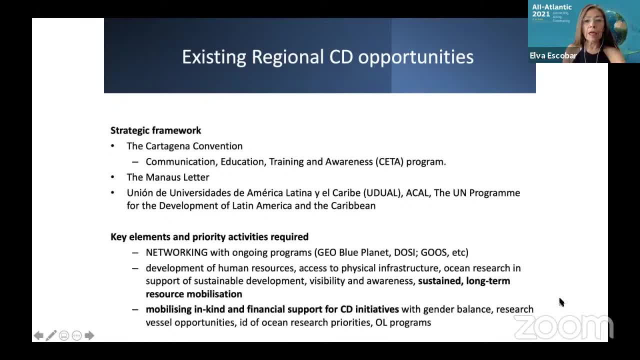 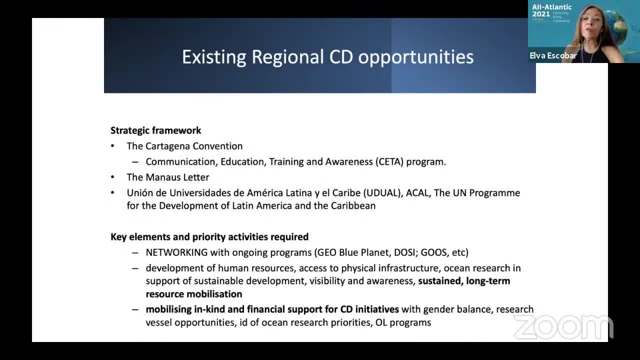 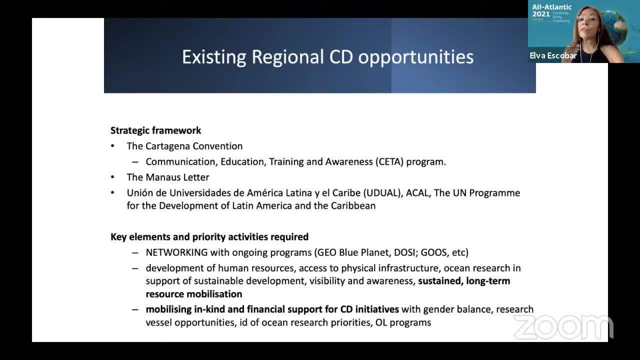 Can bring, bringing people together. The key element and approaches across the UN system include access to physical infrastructure, To ocean research and science, full context Sustained and with long-term resource mobilization. We recognize priority activities That should take place with inclusion and equity. 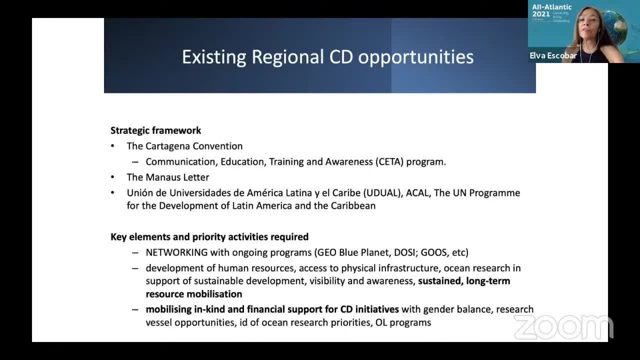 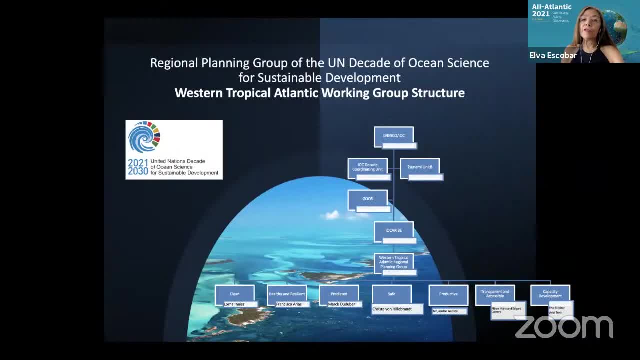 and that both the UN Decades of Ocean Sciences and Restoration can help impulse. Next one, please. To end, I would like to mention that we have the Regional Planning Group for the UN Decade of the Ocean Science for Sustainable Development for the Western Tropical Atlantic, with working group structure for the seven UN Decade outcomes. 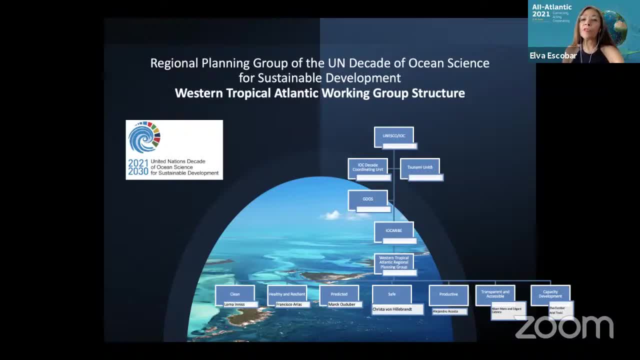 When bringing people together, we look forward to achieve, by 2030, new infrastructure, job creation that prevents future waterborne diseases. increasing water security enhances coastal water quality in the Caribbean Sea and the Western Atlantic. and for governments: listen to scientists and commit public funding to ocean sciences. 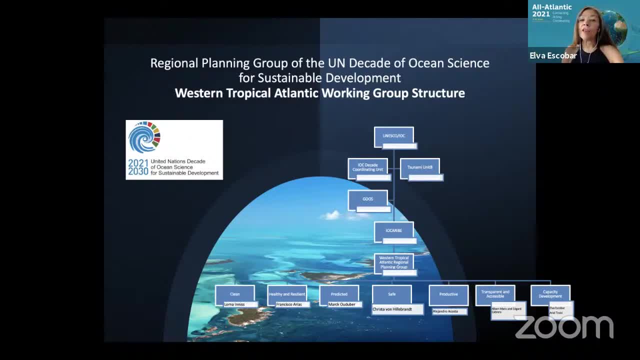 that help contribute to clean oceans, healthy oceans and other outcomes in the region, while promoting diversity and the services that diversity provide. I end up with an excerpt of Lorna Godison's poem that describes the region: Wet basalt back of whale passing 100 feet from the deck makes me call you to run from front gate to the seaside. 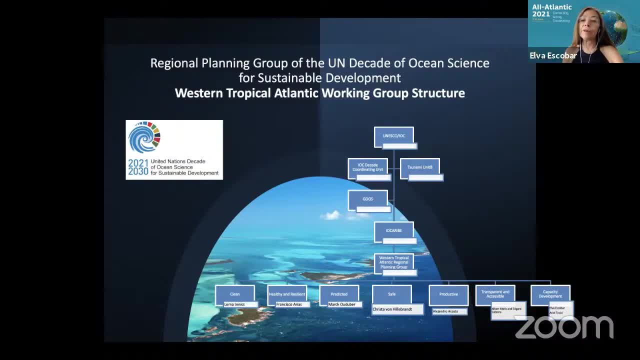 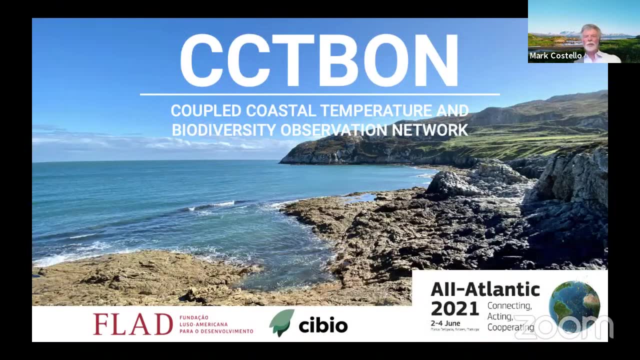 to watch this great token made manifest in the glassy March Sea. Thank you, Thank you very much, Alva, for that introduction to the experience in the Caribbean. Our next speaker is Rui, who will talk about wider Atlantic activities. 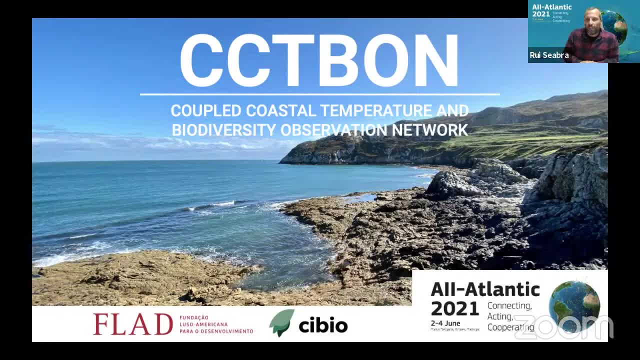 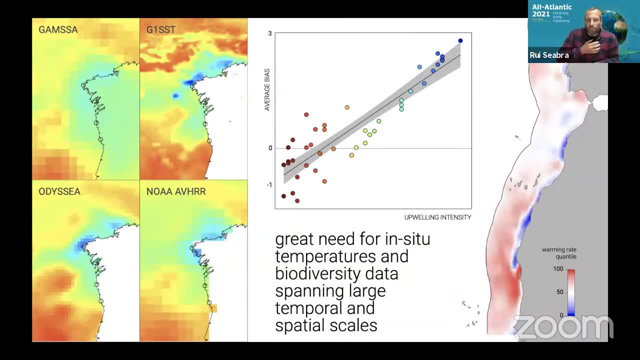 Thank you. So thank you for the opportunity to present the CCTBON network. So next slide, please. The network is a project that is starting, is developing as we speak. It is The underlying reason for its existence is the great need that. 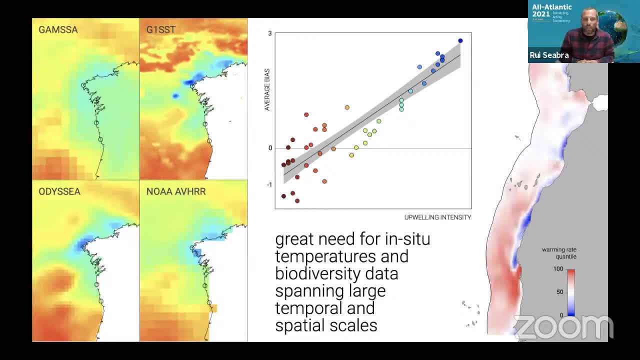 That is becoming increasingly evident in terms of in-situ temperatures and biodiversity from intertidal ecosystems that span large temporal and spatial scales, And this is because studies have shown that the bias between remotely sensed data and loggers deployed in the intertidal ecosystems is quite large. 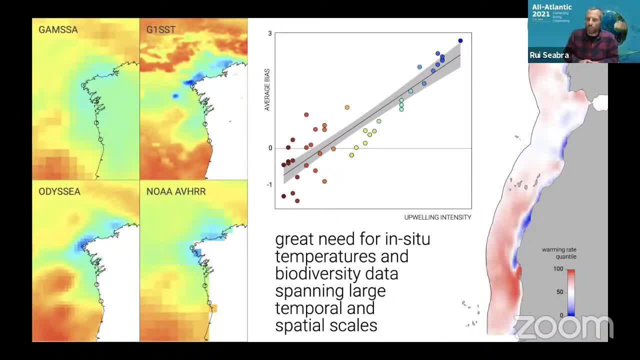 especially in upwelling, In the intertidal regions, And obviously as we face a warming climate. this raises many questions regarding the biogeographic patterns of species, and doing forecasts about the implications of these changes depends on the quality of data that we have that is very sparse in many locations of the ocean. 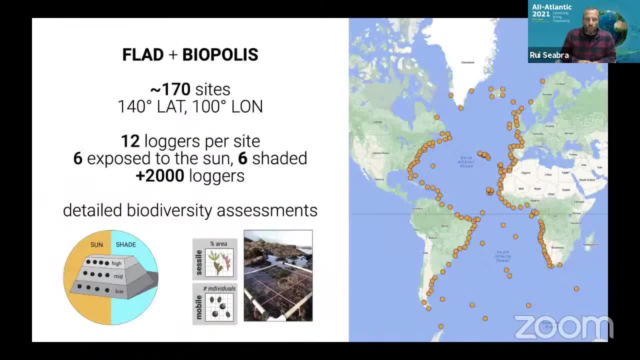 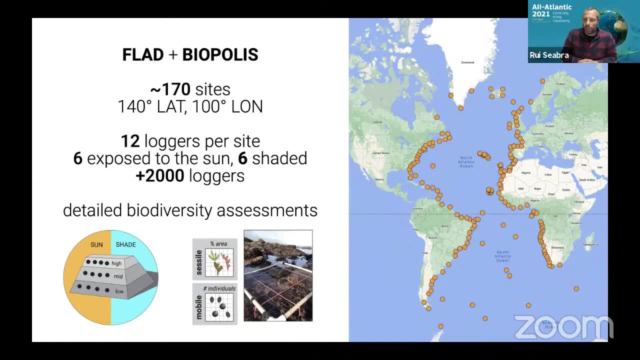 And it will establish around 170 sites across the entire Atlantic where we will deploy temperature loggers: 12 temperature loggers per site. We will cover micro-habitat exposure, so it will be very refined within each site. We will cover micro-habitat exposure, so it will be very refined within each site. 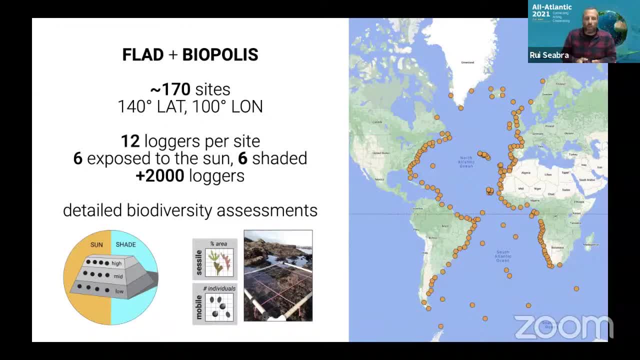 And it will total more than 2000 loggers. And it will total more than 2000 loggers And it will be coupled with detailed biodiversity assessments on each of these locations on varying timeframe depending on the remoteness of each location. Next slide, please. 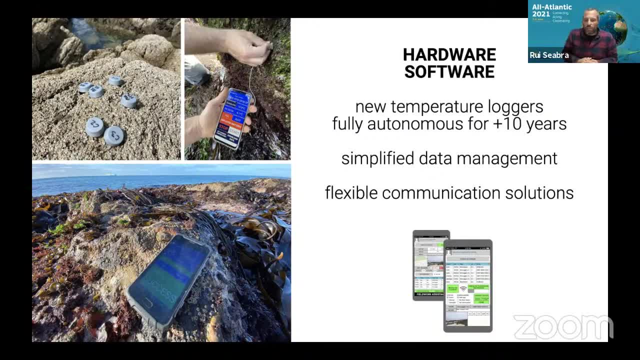 So, as we stand now, and I'm sure this is a concern that is shared by almost everyone, So, as we stand now, and I'm sure this is a concern that is shared by almost everyone, so, as we stand now, and I'm sure this is a concern that is shared by almost everyone- 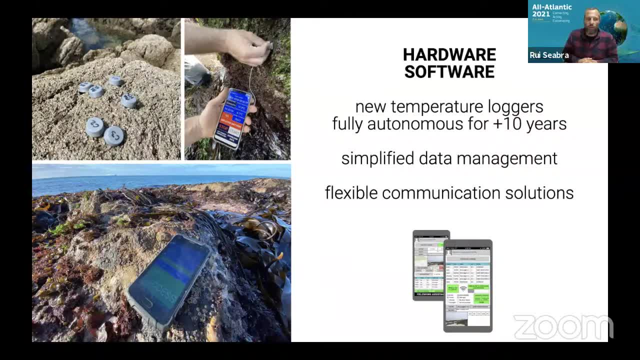 to the pandemics. everything is slowed down, but we have made significant progress nonetheless, especially on the hardware side and software side of the network, so as, in order to be able to collect all this data in a streamlined way and standardized way, we are developing our own temperature loggers, which we're now testing a version of them that can acquire 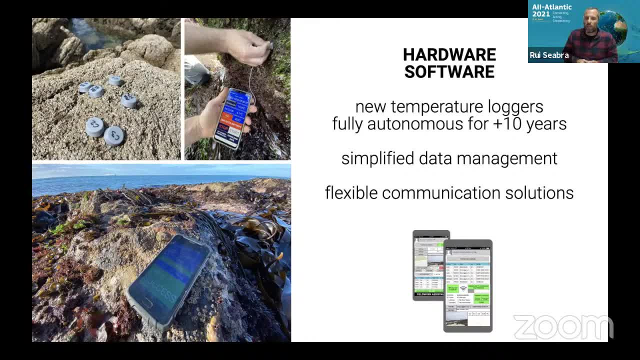 temperatures hourly for more than 10 than more than 10 years autonomously, and so this opens the the window to explore really remote locations where it's very hard to return to. we're also developing software applications for smartphones to manage the downloading of the data and relaying to servers, and also flexible communication solutions such as, for example, 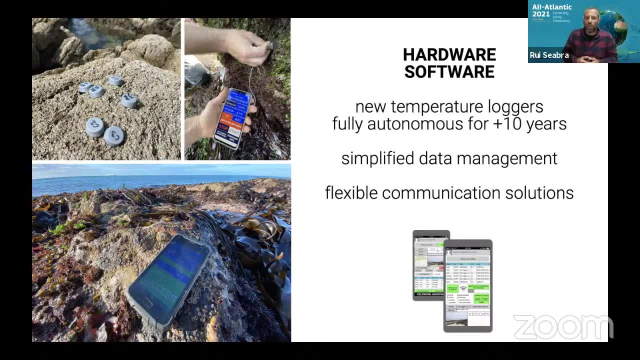 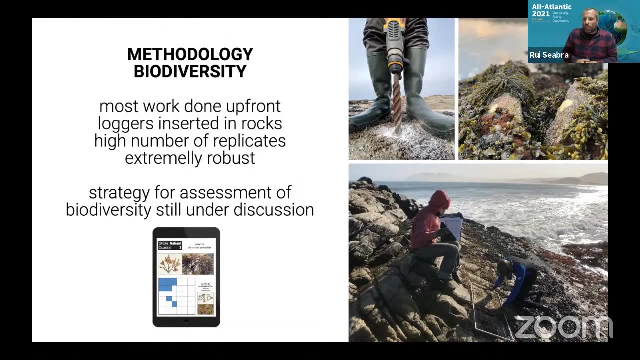 nfc extension cable that allows us an easier connection to the logger deployed on the rocks from the cell phone. next slide, please. regarding the methodology, we're still on with discussions with the some of our preferred collaborators, although this will be a very big venture with a lot of collaborators throughout. 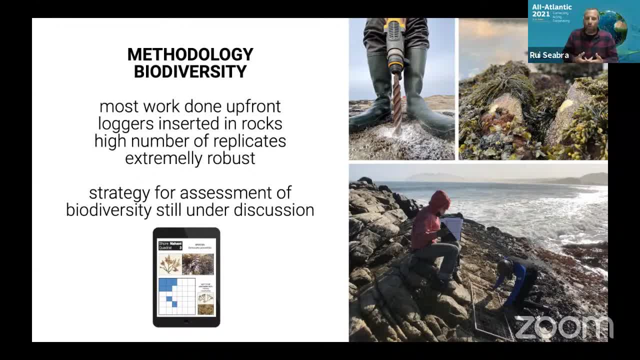 atlantic. there's a, an inner core with whom we're discussing the metal methodologies, uh before, but generally the certain, the strategy will be that most work is done up front. this is to mean that the deployment of the loggers and the first surveys will be the the bulk of the work, and then 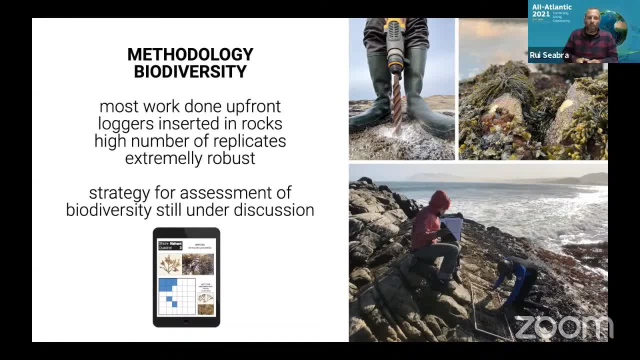 at each revisit, the work is done. work is much simpler than if the work was done throughout the time. Loggers will be inserted in rocks, and this is something that comes from our experience of monitoring temperatures for more than a decade. This really ensures that the loggers can survive for a very long time in the rocky shores. 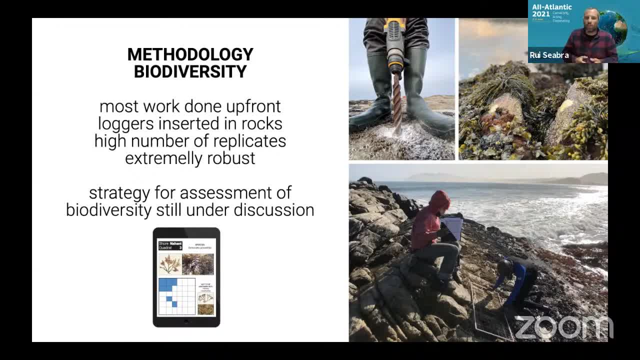 And we will also deploy a high number of replicates of loggers so that we can endure losses within a decade and still have valid data from most of the locations. The strategy for the assessment of the biodiversity is still being discussed, because we want to make decisions that ensure that we collect primarily standardised data from the entire 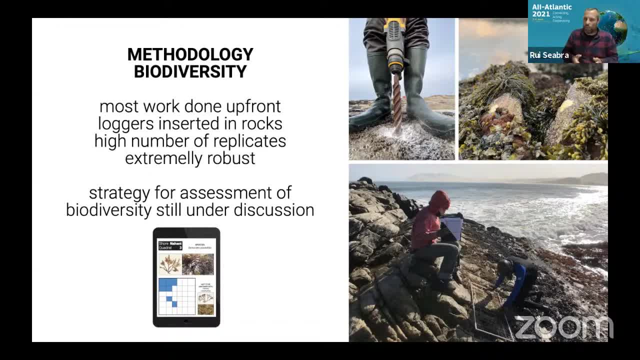 ocean, And this is something that is very important. I think that might pose questions, especially because there are differences in tidal regimes and other ecologically relevant factors that may complicate the issue, but we will strive to do the best. Next slide, please. 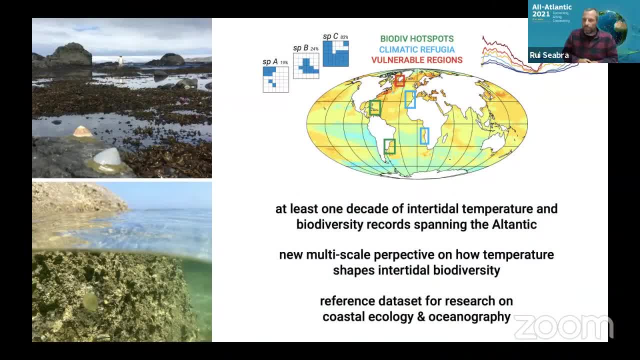 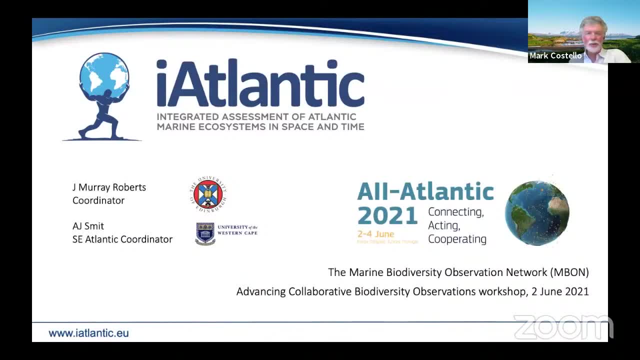 Thank you, Rui. I think we need to. That's it, basically. Thank you, Great, Okay, Thank you very much. It's very exciting, but I want to make sure that the next two talks have enough time. So is Murray or Ajay Smith are the next speakers. 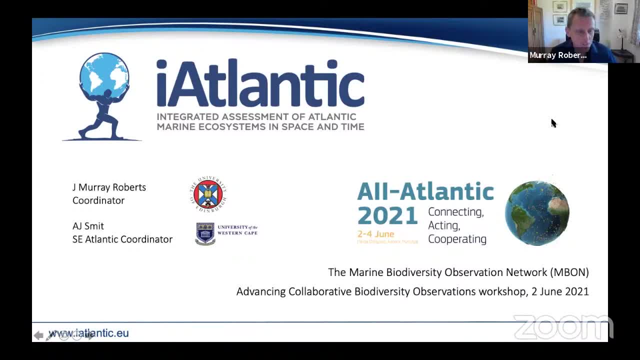 Is this a duet or will we have one speaker? It will be a duet, Mark, but Murray will go first. Okay, Okay, Five minutes. Thank you very much, Mark, And thanks everyone for the chance to speak to you today. 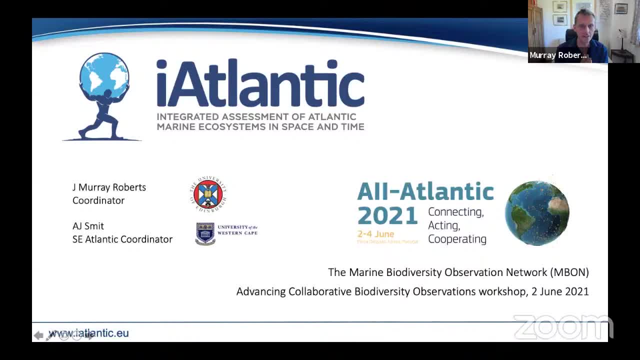 Ajay and I are going to give a quick overview of the iAtlantic project mission. It will speak to some of the questions from Juan and others in the chat about capacity building and enhancements across the Atlantic. Thank you, So if I could go to the next slide, please? 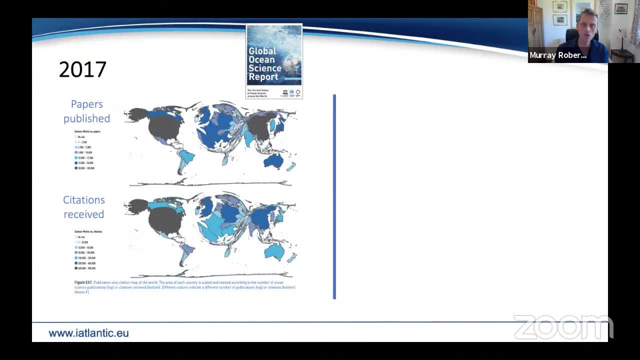 iAtlantic is a project that focuses on the deep and open ocean Atlantic. So from a marine biodiversity perspective, we deliberately focus on those areas of the Atlantic about which we know the least and from areas that we will very likely discover in new species, new habitats, and feed that information through to the scientific community. 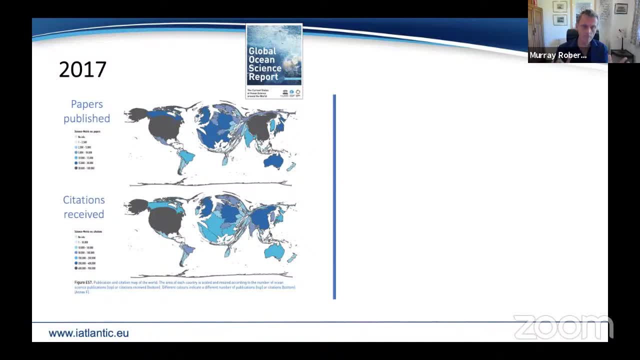 but critically to a wider policy audience as well, And by way of background, we built our project with this graphic. I think many people are very familiar with IOC's global ocean science report from 2017, and here we see cartograms where the world is scaled on the top by the numbers of papers. 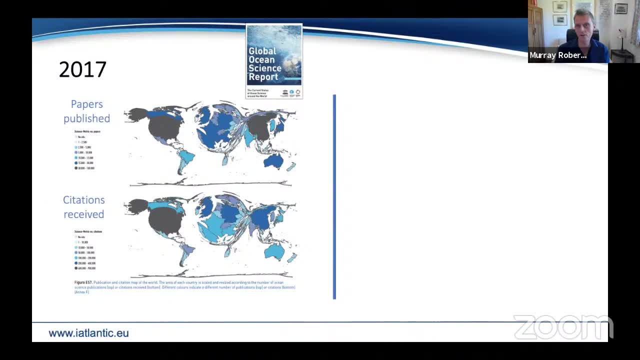 published and at the bottom the number of citations received. So it's a shocking graphic. It's a graphic that has great impact And in iAtlantic we built our plan in terms of enhancing human and technical capacities throughout the project. It's not siloed in any one place. 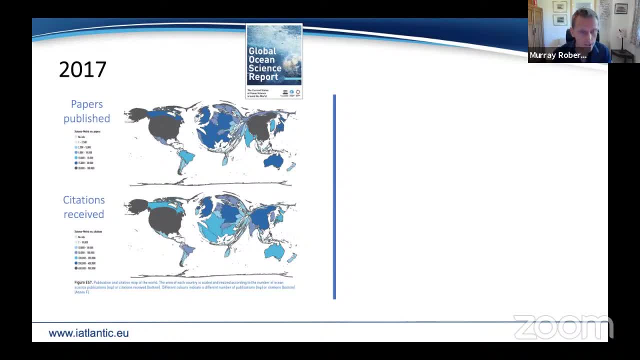 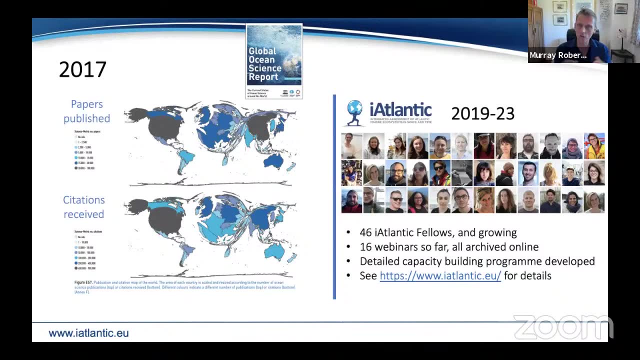 It's everywhere in everything that we do. Next slide, please, And to illustrate that, I've got a picture here of our fellowship scheme. These are the people in our project that are really making this happen. iAtlantic is a large project, so it has a good budget. 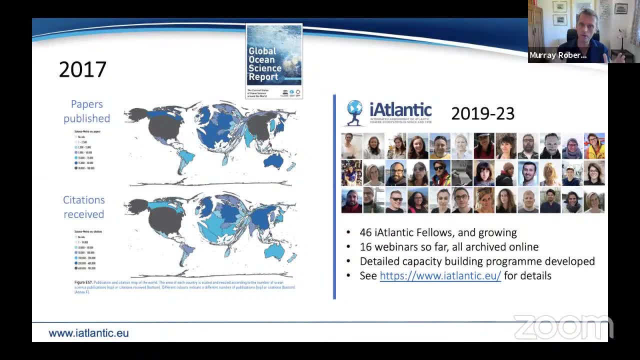 We can employ people, we can work with people and we can work with people across the Atlantic Basin with a mandate through the Belem Statement. We can send European funds to Argentina, Brazil, South Africa, and we've done so. The fellows come together as one example of how we build community. 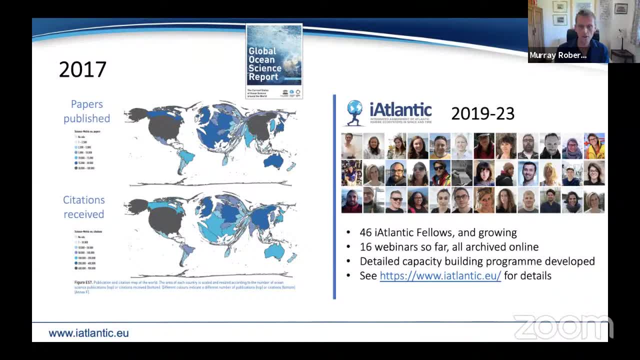 We have an active online presence. The fellows know each other very well by now and they're really leading our projects and leading the charge in terms of how we develop their careers and get the best science done in our project. If I could go to the next slide, please? 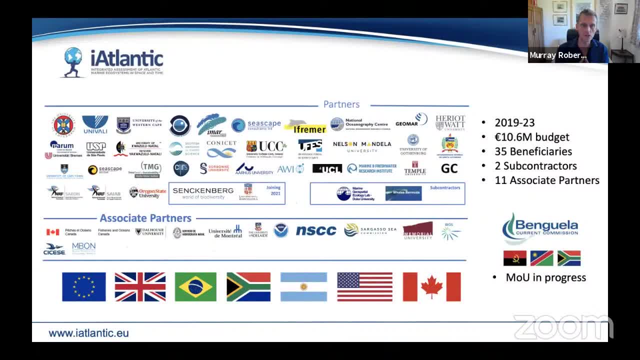 I want to tell you a little bit about how the project works, what it is that we're doing. It's built upon a partnership that you can see on the slide: A lot of organizations crisscrossing the Atlantic: north, south, east and west. 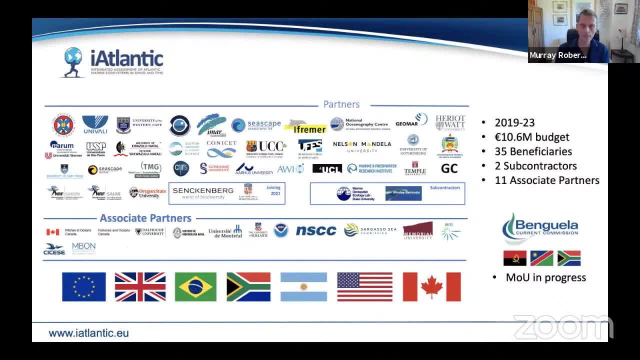 We're developing current projects. We're developing new projects. We're currently at the current commission and you can see a roll call of the nations and the EU partnerships that have developed to make this project happen. Enbon are one of our critical associate partners and we're working with Enbon in a number of 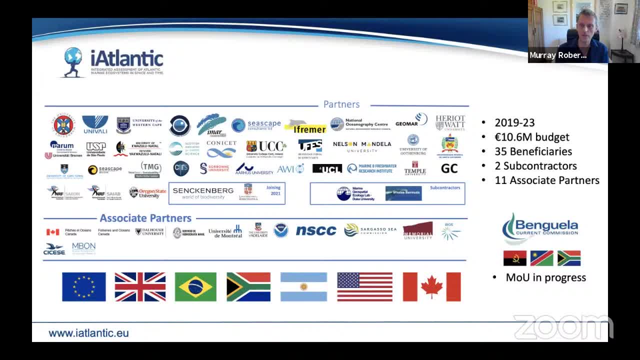 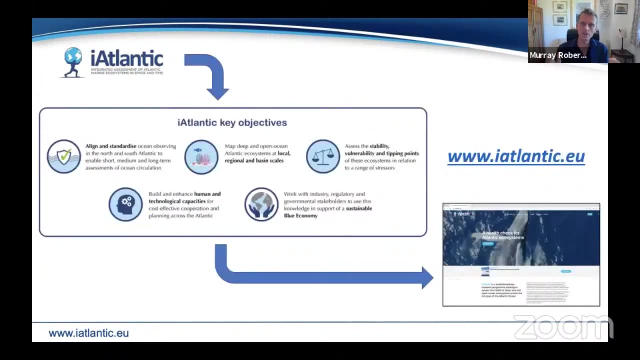 ways in a very practical sense, including some interesting ideas developing around best practice that we're focusing on at the moment. So iAtlantic is developing an integrated assessment of Atlantic marine ecosystems in space and time. If I could go to the next slide, We're doing that in a variety of ways. 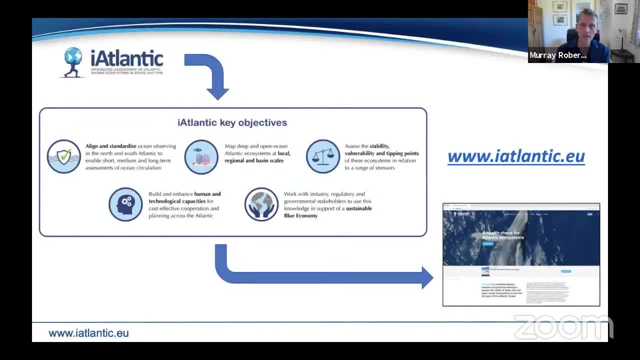 We use existing data heavily. We can't study all Atlantic ecosystems everywhere. We will use existing data and interrogate those data sets. In fact, one of our major capacity building workshops happens in two weeks' time in Capo Verde in cooperation with the Waskall Consortium, where we're training people from across the 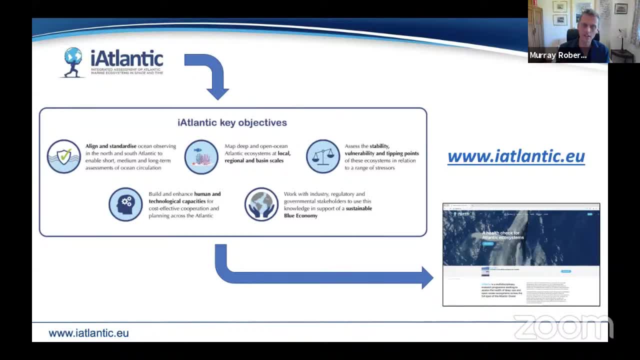 Atlantic basin in ecological time series. statistical analysis. That's one of the really important capacity building workshops. We're doing that in a variety of ways. We use existing data heavily. We can't study all Atlantic ecosystems in space and time series. We're doing that in a variety of ways. 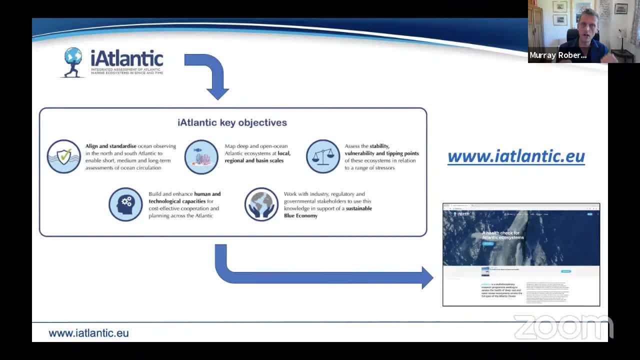 We're doing that in a variety of ways, But the capacity building goes every which way. in Atlantic We want to benefit from taxonomic expertise, for instance in places like Brazil, and bring that expertise across to our partners in Europe and elsewhere. 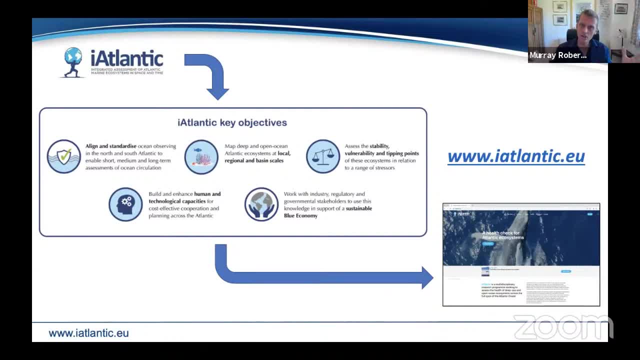 In terms of the objectives of the project. we have a foundation in a physical oceanography of the Atlantic, recognising the physical environment is changing very rapidly. We need to align and standardise these observations. in the North and the South, We're making practical interventions across different regions of the Atlantic. 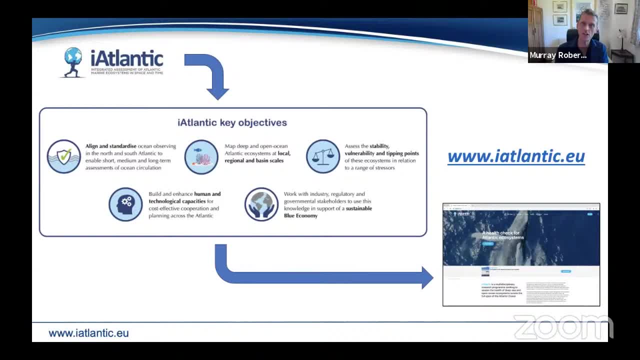 We need to use the data to make some clear comparisons, making practical means to enhance the capacities in the South Atlantic, For instance, by putting new instruments onto the arrays that cross from South America towards the middle of the Atlantic, the SAMOC and SAMBA array enhancements that we're funding. 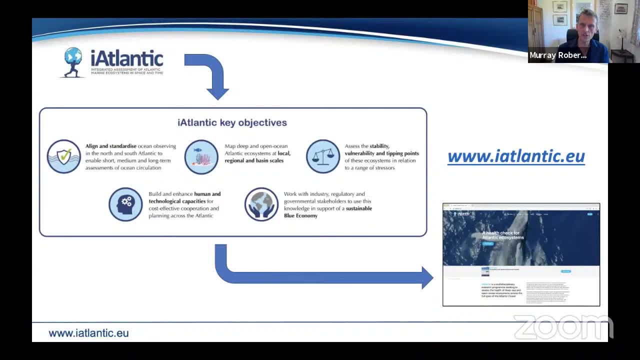 We have a large work package around mapping deep and open ocean ecosystems. Actually, a sister project is working on this as well, And both projects were at the CBET 2030 workshop that was running in parallel with our workshop. today, The spinal aspects of the project take place. 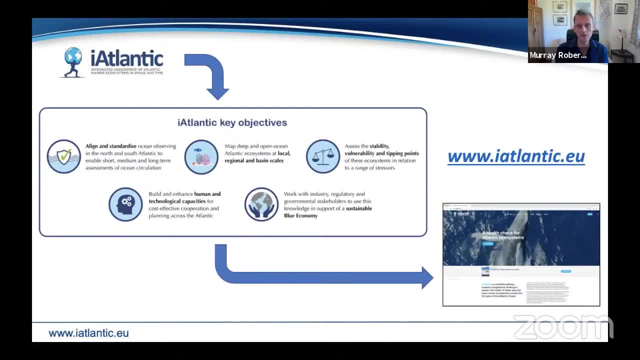 to assess the stability, vulnerability and tipping points of deep and open ocean ecosystems. So at the end of the project we want to identify which areas are experiencing the most rapid environmental change and within which we know ecosystems are showing signs of stress and pressures. 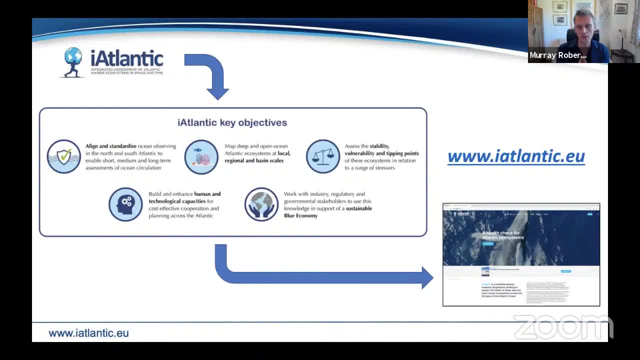 AJ will follow up with a couple of discrete examples from the South Atlantic after I finish. That's the real kind of heart of our project there in that third objective. There's one minute left for AJ. I will speed up Mark Build enhanced human and technical capacities. 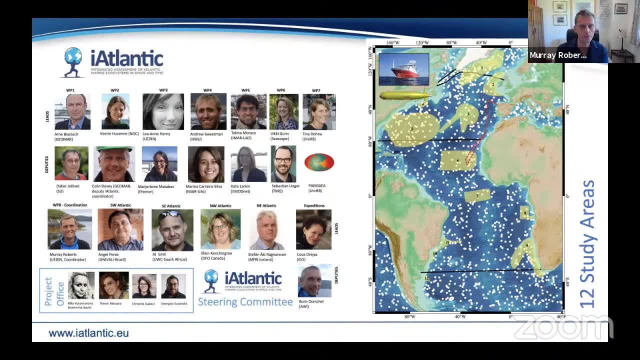 and then work with regulators and policy specialists across the Atlantic basin. This is the roll call of the team that lead the project, but I did want to note where we are working in the Atlantic. You can see the regional study areas: 12 across the Atlantic. 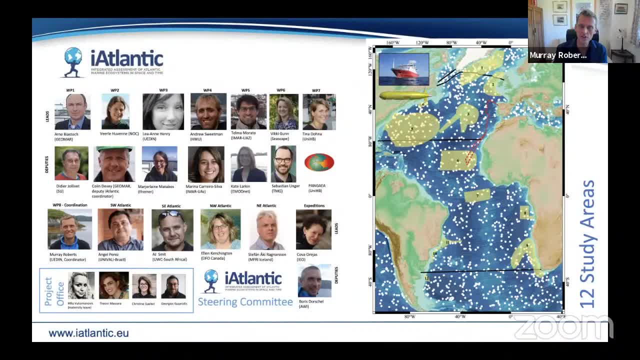 We're also working with the latest technology, including environmental DNA sampling, gathered autonomously from an AUV deployed from the Samyanto to Gamboa this summer. AJ, let me pass the mic to you. Thanks, Murray, Next slide, please. 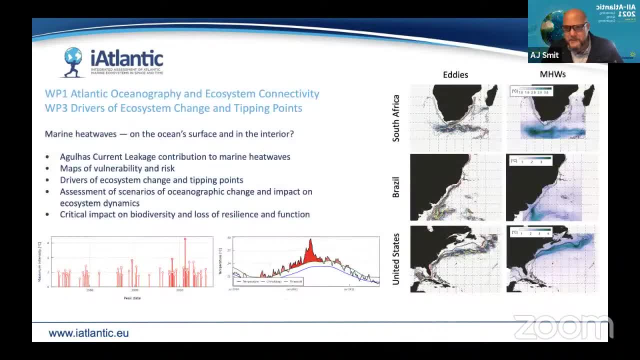 So one of the research questions that we're particularly interested in is the question of extreme events in the ocean. So to what extent are extreme phenomena, such as, in our instance, heatwaves, responsible for influencing the resilience of the deep ocean and the sensitivity of some of the very sensitive species? 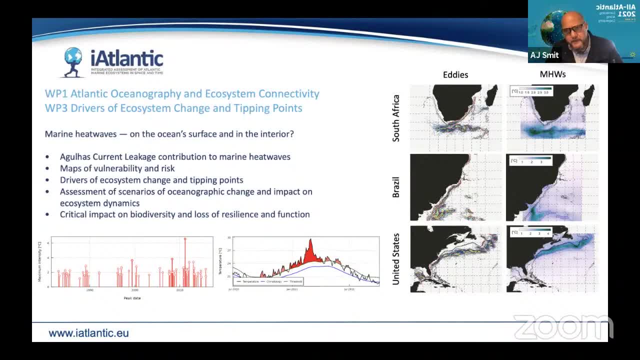 such as cold water corals. So one of our The Atlantic Fellows, in fact, is analyzing the output of ocean models to understand how stable the interior of the ocean is in terms of the thermal regime that the organisms experience there. If we can go to the next slide, please? 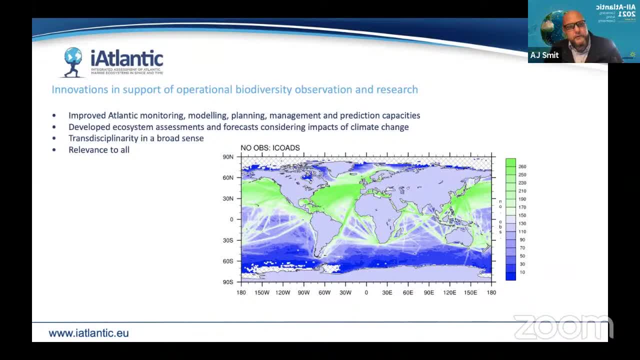 So the output of our research will then, of course, provide a broadened capability to monitor, model and plan the management of sensitive areas in the deep ocean, and to undertake and forecast the assessments of ecosystems in the deep ocean under the influence of climate change. 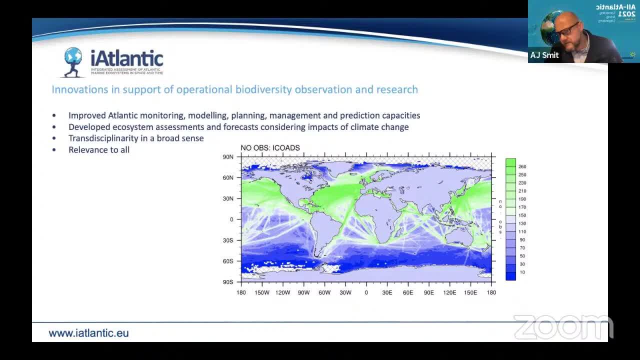 Of course, our work in South Africa has to be very much transdisciplinary. We have to make it relevant to everyone in the country. The central focus of our government in South Africa is the relevance to people. So in that sense we're very much transdisciplinary and we're going to, through public outreach programs and so on, of course, make it explain our outputs to the people that are impacted most by the changes that they are experiencing in the ocean. 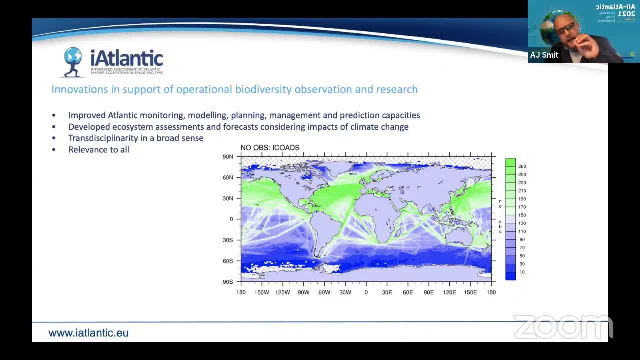 So, to this end, we are going to be filling in those unknown gaps in the Atlantic Ocean which are currently unexplored, as shown by the map of the ocean observations in the Atlantic Ocean. Thank you, And I'll stop there. 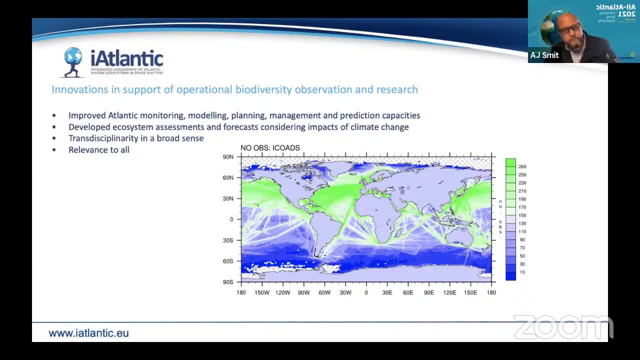 I know we're running out of time. Thank you very much. Thanks very much, Ajay and Maria. Very exciting project you've just started, Wow. And another very exciting development is ocean best practices, which is the topic for our next speaker, who is going to be Jordan. 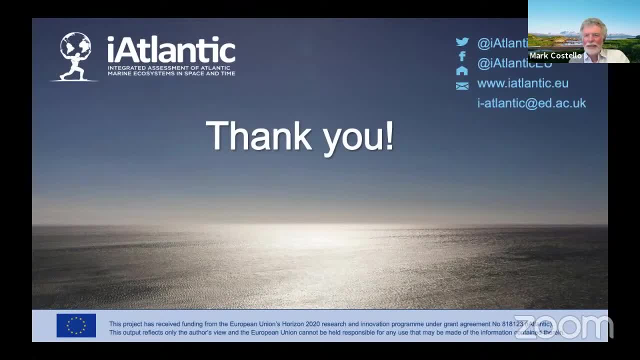 Okay, You're next, Jordan. Good day everyone. I am Jordan van Stavel And I'll be giving you a brief overview of what best practices are, as well as the ocean best practices system. Next slide, please, Thank you. 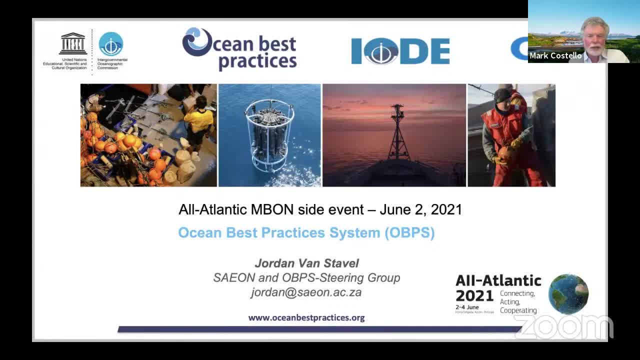 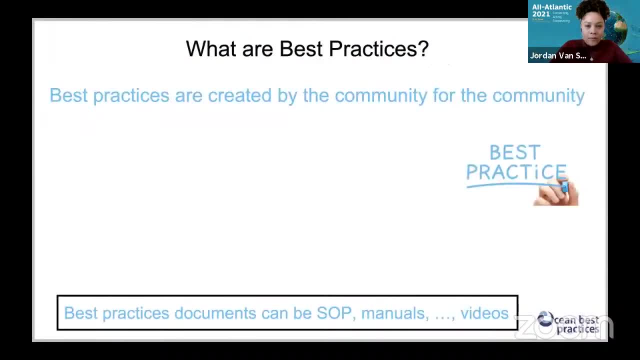 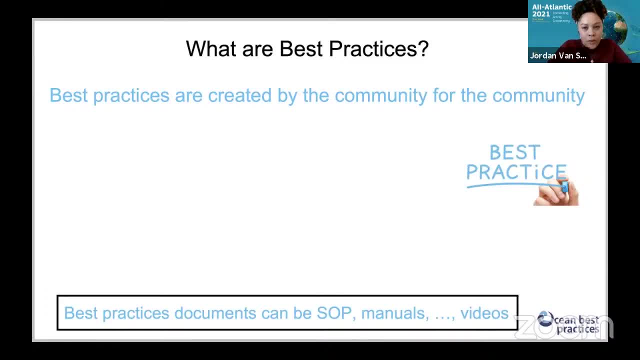 And best practices are created by the community for the community Next, please. So we define best practices as a methodology that is repeatedly produced superior results relative to other methodologies with the same objective, But sometimes best practices are used elsewhere. You see that. 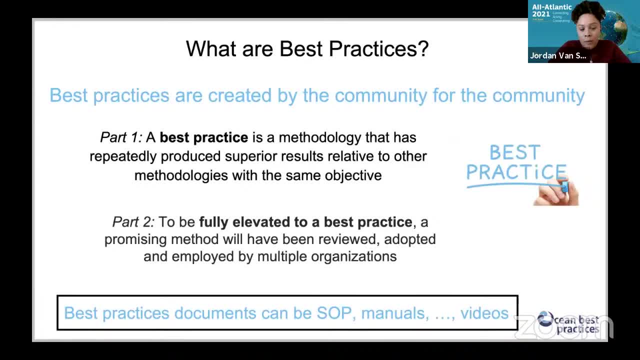 Sometimes the word best practices raises questions where people may say: I have a good method, but I don't know if it's the best or I've got many. there are many methods trying to achieve the same objective, but how do I know which one is best? 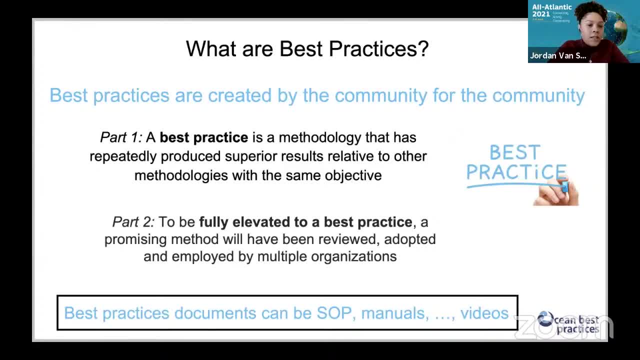 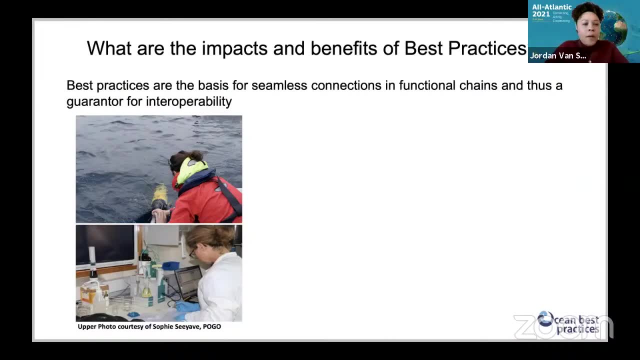 And this brings us to the second part of this definition, which states that, to be fully elevated to a best practice, a promising method will have been reviewed, adopted and employed by multiple organizations. Next, please. So some of the benefits and impacts of best practices. Best practices are the basis for seamless connections in functional chains and thus a guarantor for interoperability. Here we've listed a few. Next, please. 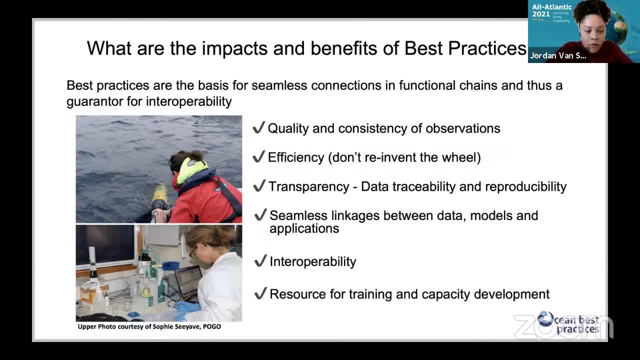 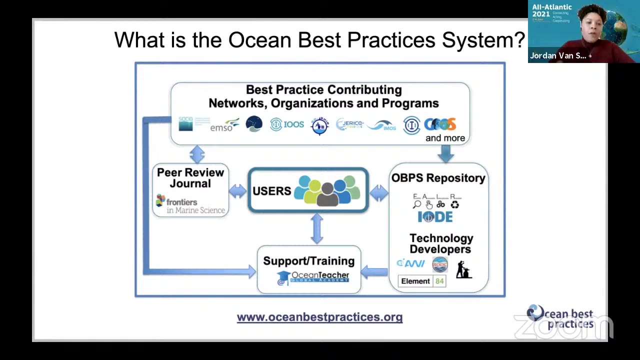 So, for example, it allows for quality and consistency of observations, efficiency, transparency through data traceability and the like. Next, please. So what is the Ocean Best Practices System? The OBPS is a global sustained system comprising of technological solutions and community approaches to enhance the management and support the development of ocean-based practices. 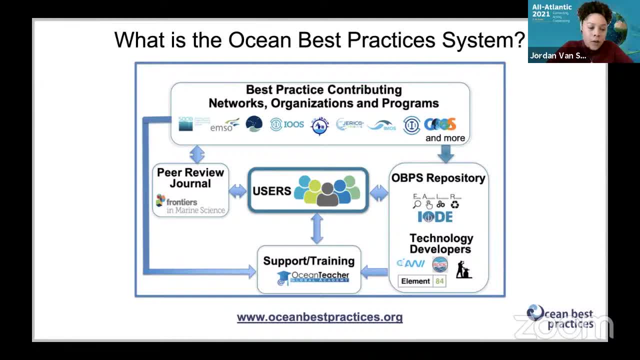 It consists of a number of components. So, firstly, the contributing networks, organizations and programs. a permanent repository which includes state-of-the-art semantic discovery and metadata indexing for the improved access to best practices. It also provides support and training by leveraging the Ocean Teacher Global Academy through web-based and in-person training. 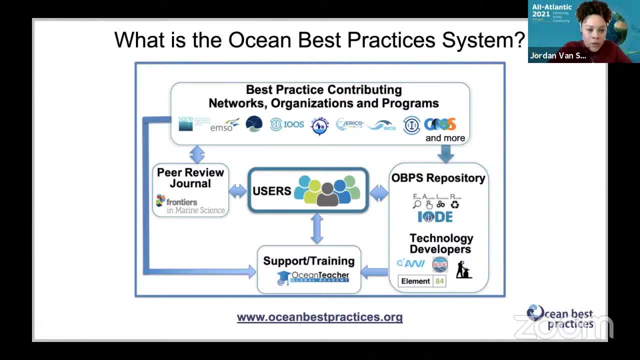 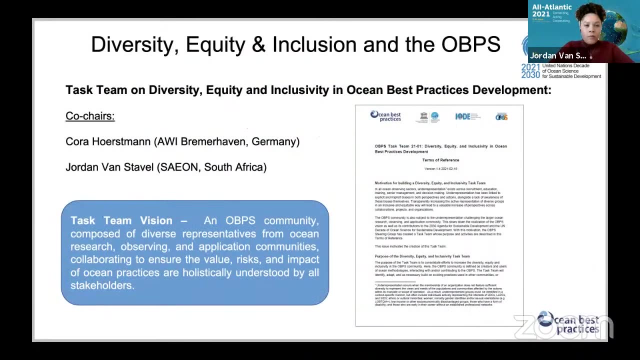 And then, lastly, it also has a research topic in peer-reviewed journal for Frontiers in Marine Science. User communities interact with each of these components, And I've also linked the best practice website below for more information Next, please. So the Ocean Best Practices System will play an integral role in the ocean decade. 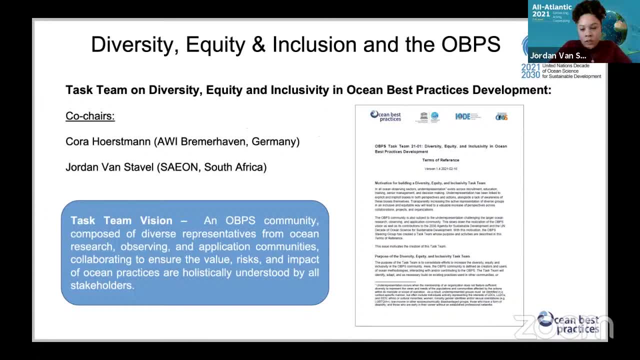 And it also recognizes that under-representation exists across the ocean observing sectors And as a contribution towards achieving the decade's actions and outcomes, we have also formed a task team to try and increase diversity, equity and inclusivity in ocean best practices development. My colleague Ms Cora Hortzman, and 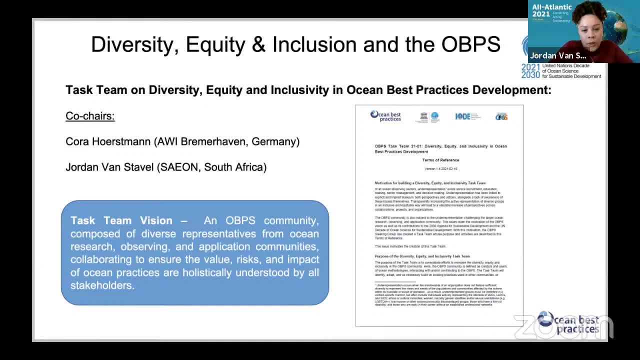 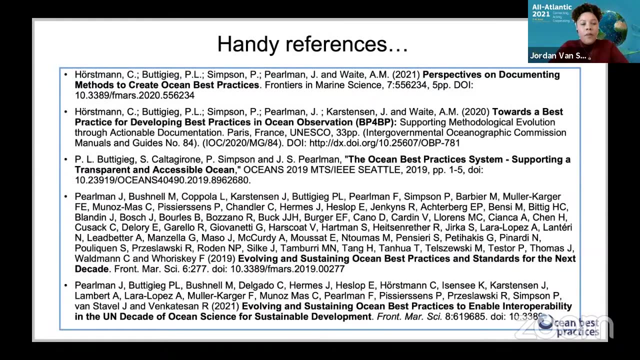 myself are the co-chairs of the STARS team, and we invite anybody who is eager to contribute or participate in the STARS team to please contact us. You can find more information on our terms and references on the ocean best practices website as well. Next, please, And then I've also just 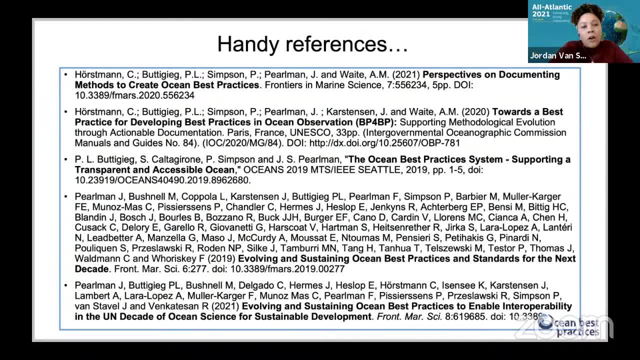 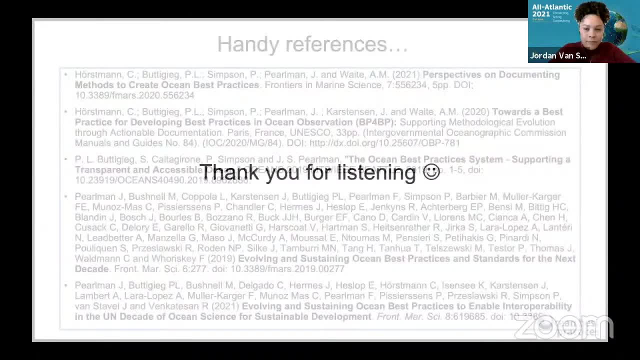 linked a few references for more information on the technologies behind the ocean best practices system- developing your own methods or best practices- and also more details on its contribution towards the ocean decade. Thank you so much. Thanks very much, Jordan. that was very timely. 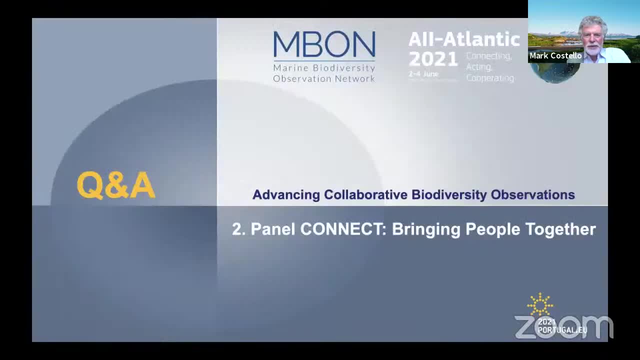 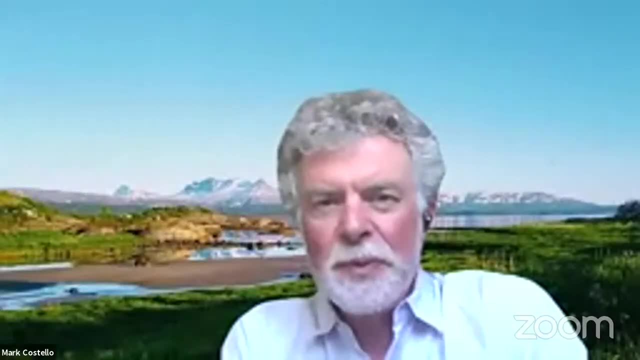 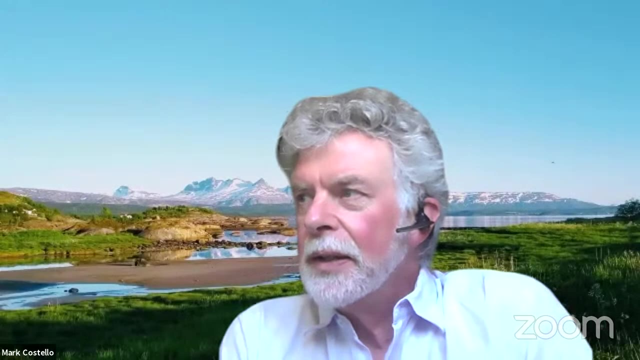 Do we have any questions for Jordan or the other speakers? Things are a bit quieter in the chat than they were the last time. Maybe we need a moment for people to get their questions out. If there are no hands up, I might ask the four speakers if there's anything they want to add. 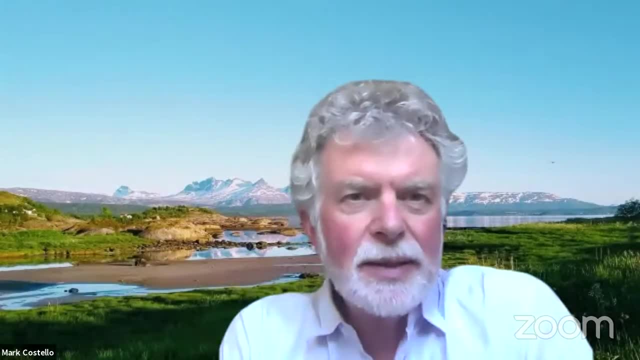 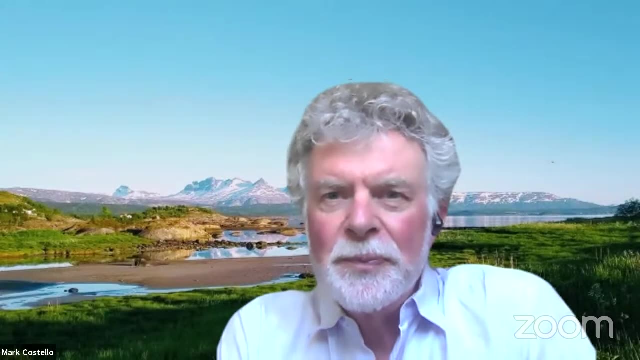 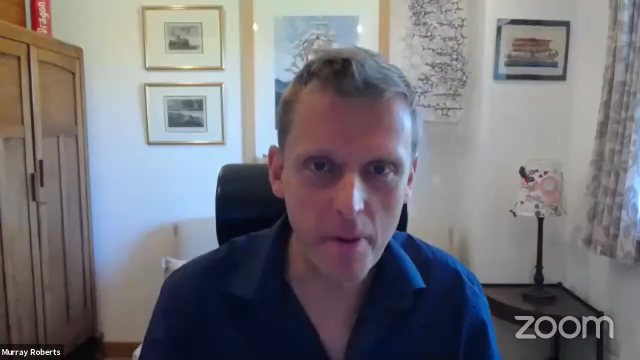 to their presentations or they think they might wish to add. Murray switched his microphone on. Do you want to say something, Murray? I was just preparing myself. You have two hands up, though, from Anthony and Frank. Oh, I do, Yes, Anthony, please. 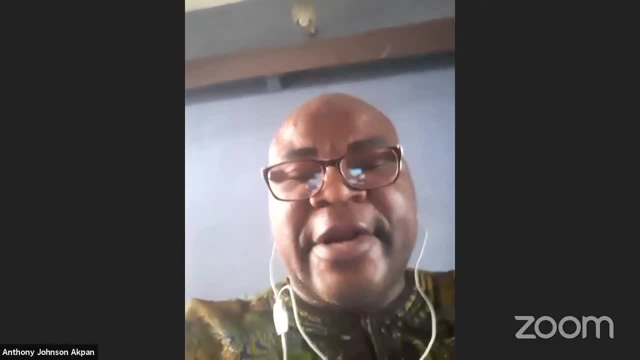 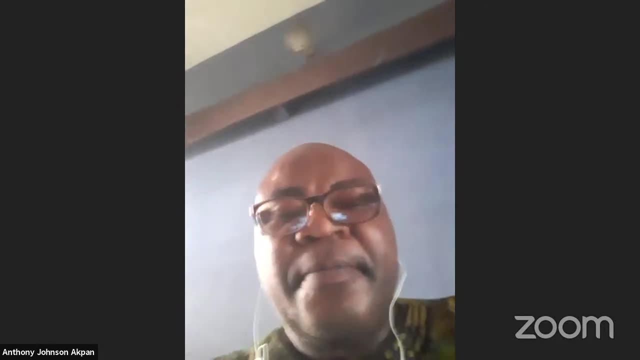 Okay, Murray, thanks so much for your presentation and idea. I just wanted to find out how do you connect the work you are doing with ocean literacy? Thank you, That's a great question. We take that on board. very, very much so, and so we do all we can to. 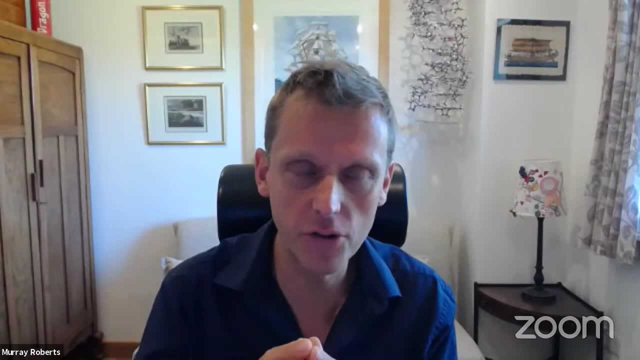 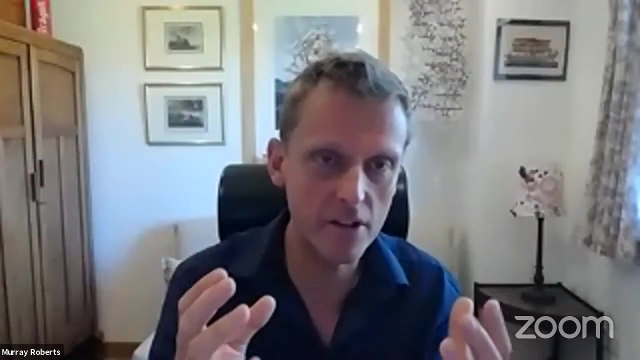 enhance ocean literacy. In fact, we just completed a project in the North Atlantic where we created a whole series of materials. We actually have a series of different sources that are available. I'll pop a note in the chat to point people to those resources. What we actually find is that somebody's been in a very lucky 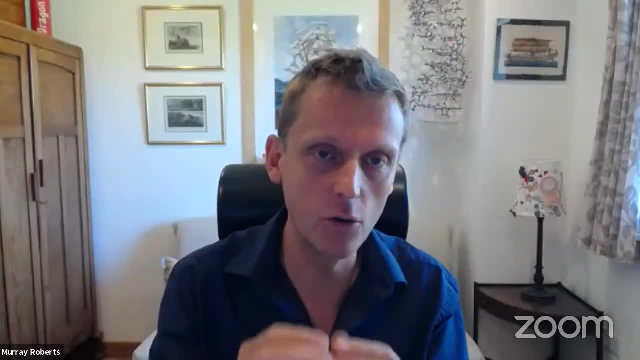 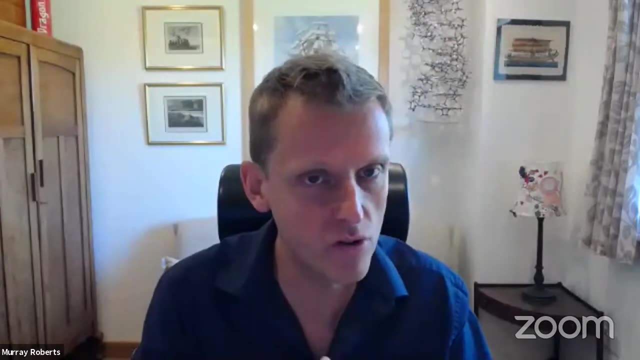 situation. People are fascinated by the deep and open ocean. There's a natural curiosity and we build upon that. The organisms are beautiful, The habitats are stunning and there's that also excitement around discovery science that we use. We work a lot with the mainstream media as and 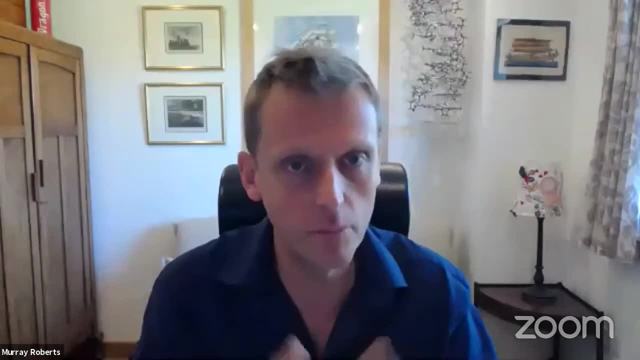 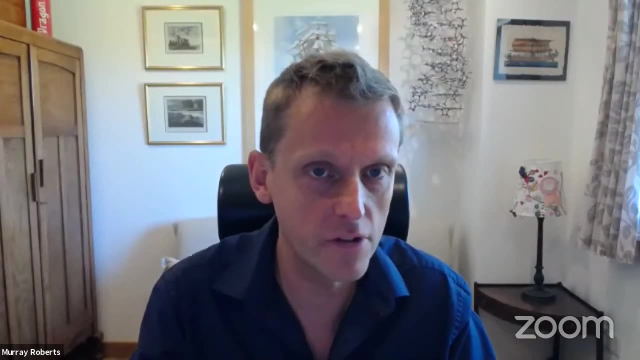 where appropriate as well, If a paper comes out, we'll work hard to secure appropriate publicity around that Sure Thank you or the voice of America, and so forth. So it's a great point and I think it's actually central to the discussion and the debate that we all have. 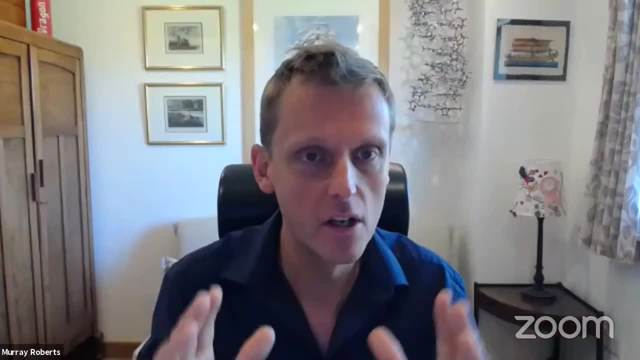 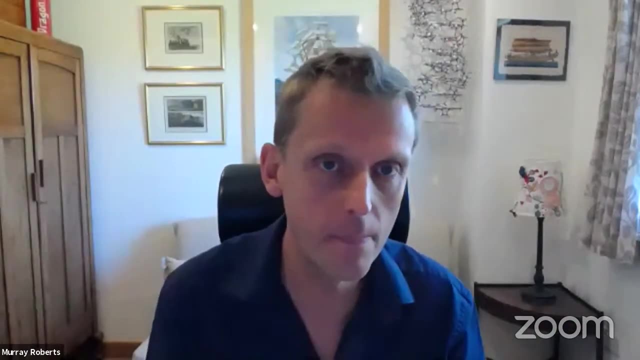 at meetings like this is that we know the issues on calls like this, but in wider society there's a huge lack of understanding of the importance of ocean ecosystems and the ocean in the climate system. They're good examples, Frank, you have your hand up. 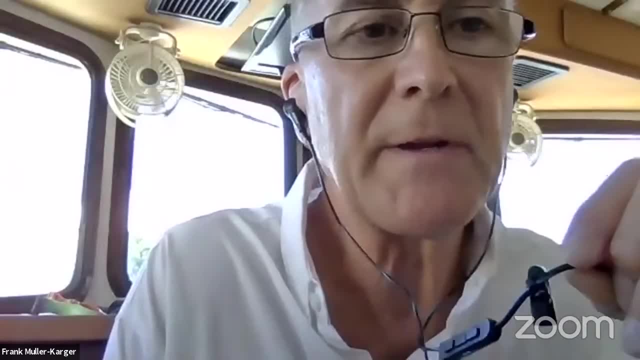 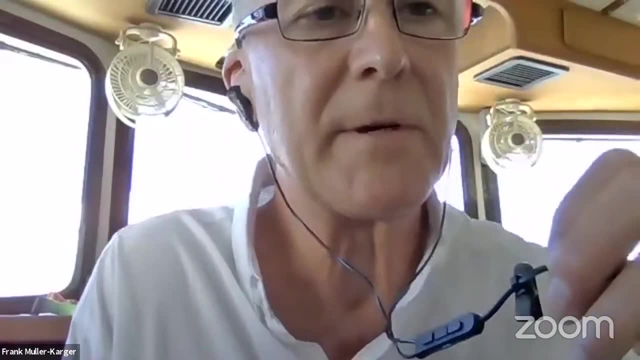 Yeah, thanks. I want to emphasize that the reason we're having meetings like this is to engage everyone in addressing these kinds of questions. How do you develop standards? How do we do ocean literacy around these concepts? How do we do more advanced training? 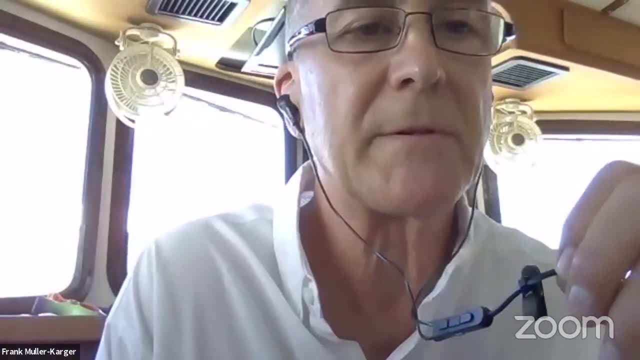 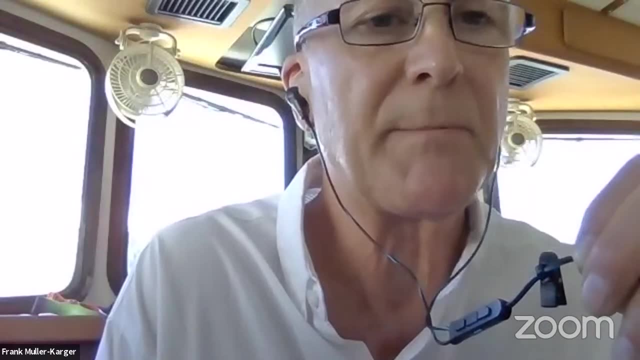 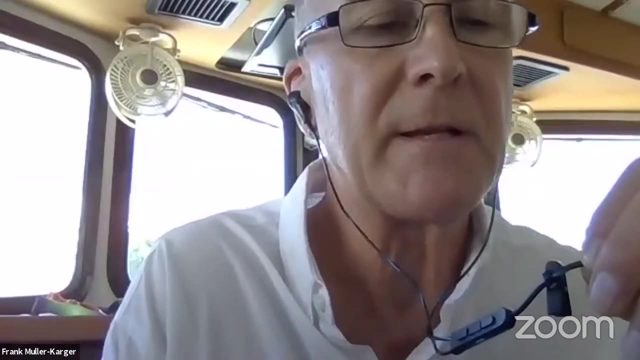 on the essential ocean variables or the need for standards or data management or data collection or publications. This is something that takes a lot of people around the world and that's why we're creating these frameworks. We're trying to engage with a decade. 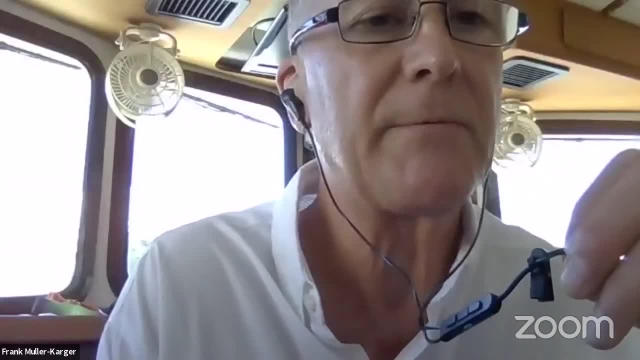 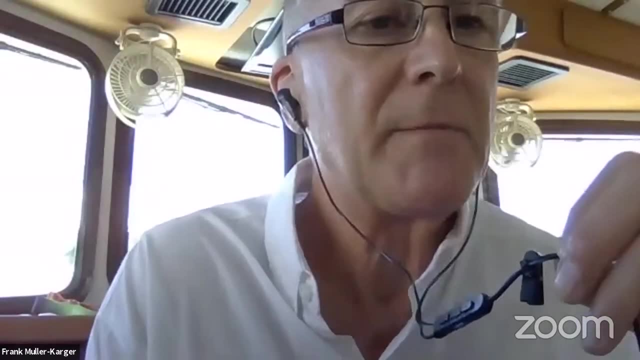 So Elva mentioned a regional group. There's many regional conversations happening under the umbrella of the ocean decade. It's a wonderful opportunity to get engaged. We don't have all the solutions, We certainly don't have the money, but if we work together, 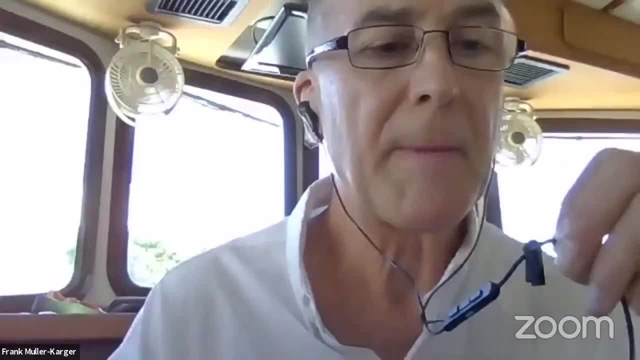 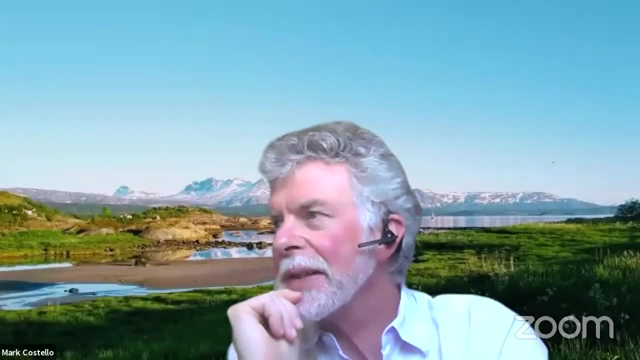 we can try to address these issues. Okay, yes, I didn't see citizen science mentioned in any of the talks, but I think it's a great question. I've seen a lot of talks so far, although it might be in the next session. 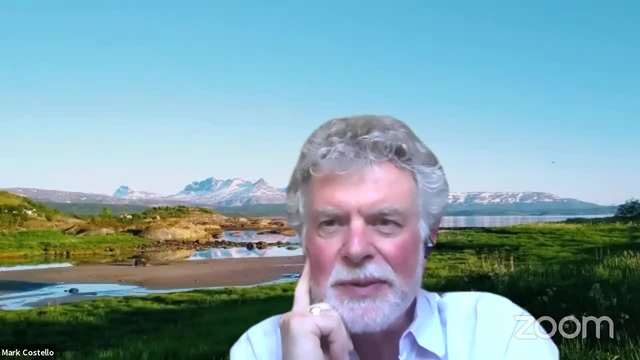 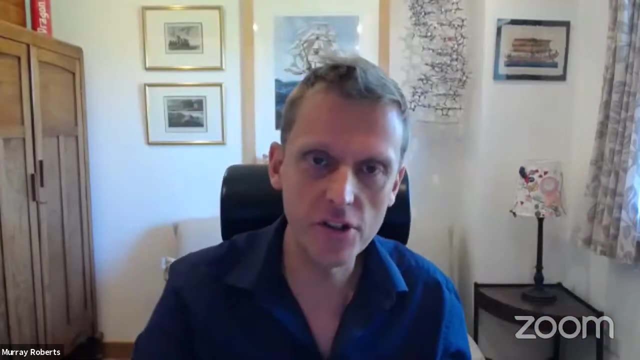 So maybe I shouldn't mention it. Murray has his hand up. Is citizen science involved, Murray? It is, and something we're super proud of, actually, because you'd have thought focused in deep sea and open ocean systems, there wouldn't be as much opportunity for citizen science. 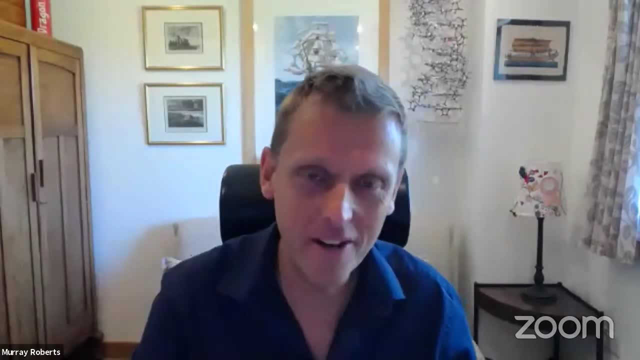 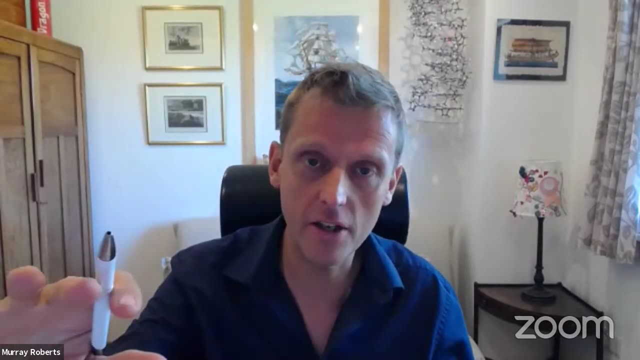 But one concrete example- we work on my slide- of our partnerships. We had Wales- Bermuda and Wales Bermuda established by somebody who's passionate about the humpback whales that migrate through the Sargasso Sea And for 15 years has generated a unique time series. 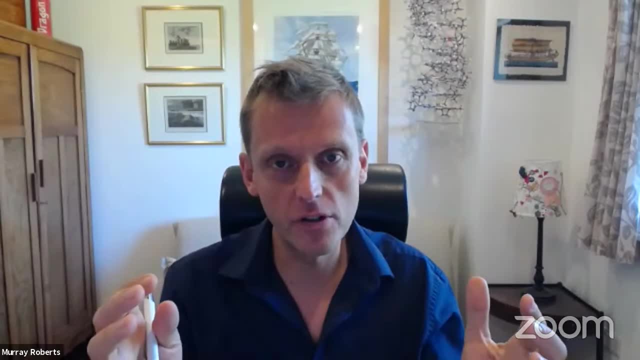 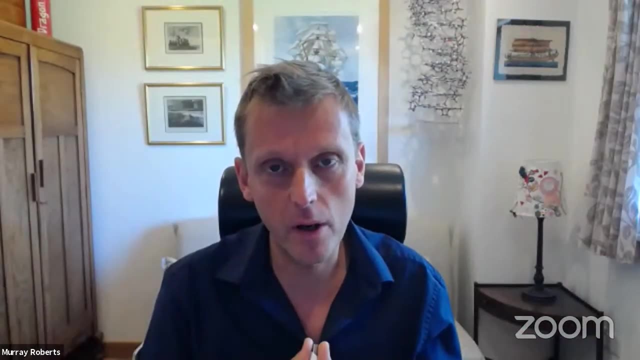 data set. So we're using mark recapture statistical approaches at the University of Edinburgh to then interrogate this citizen science data set and reconstruct the population migratory flows of those humpback whales. There's more information on this actually on our website, if people are interested. 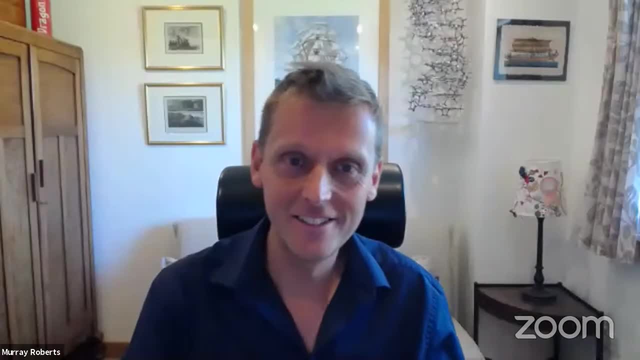 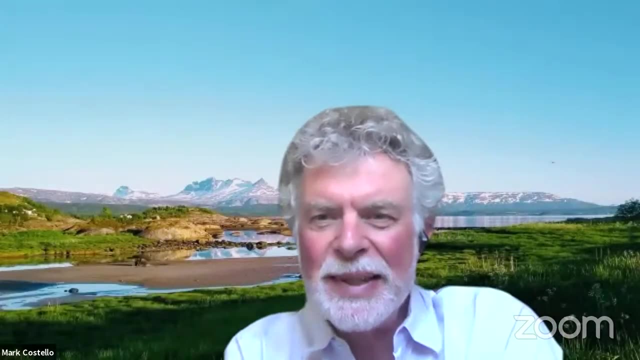 and some of Andrew Stevenson's amazing imagery as well, And I saw Amos put his hand up and then he took it down again. So I don't know if he means to put it up or down, but his microphone is off so he must be quiet. 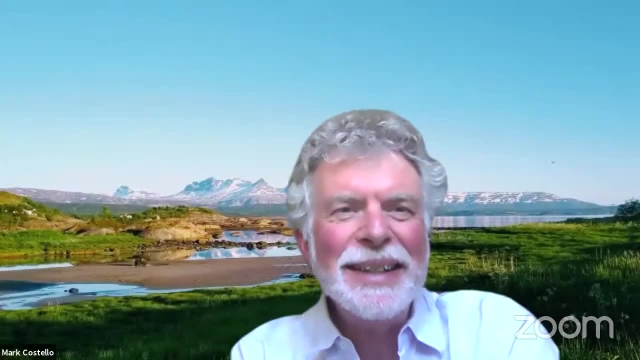 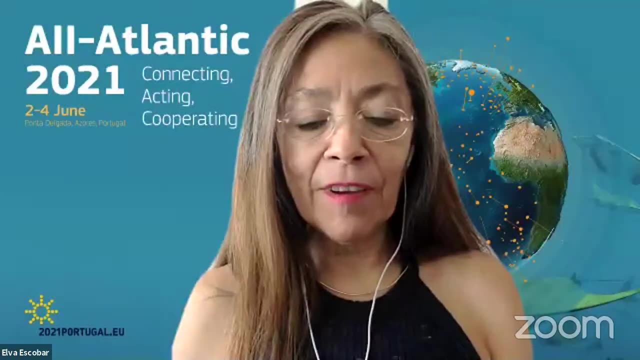 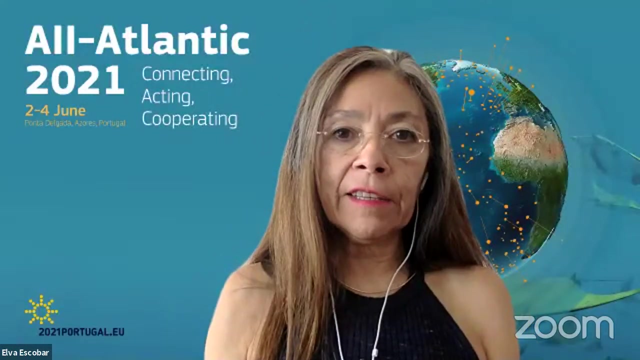 No, he's back. I'll answer in the chat, Thank you, Okay, thanks, Alba. did you want to answer or add? Actually, in ocean literacy and some of the citizen science programs, Relato recently held a very large five-day session. 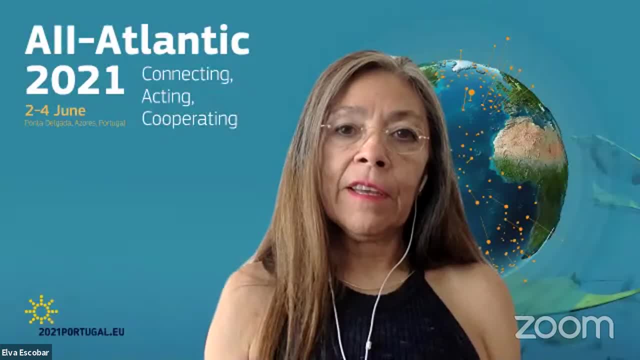 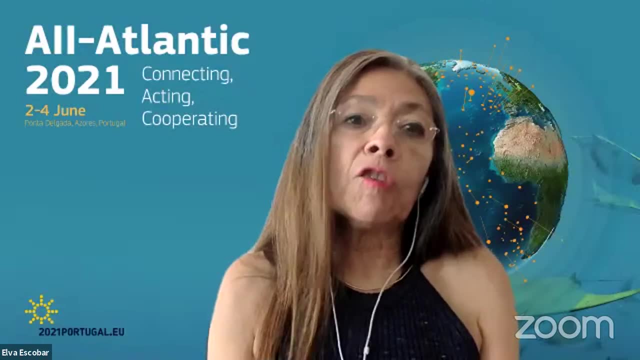 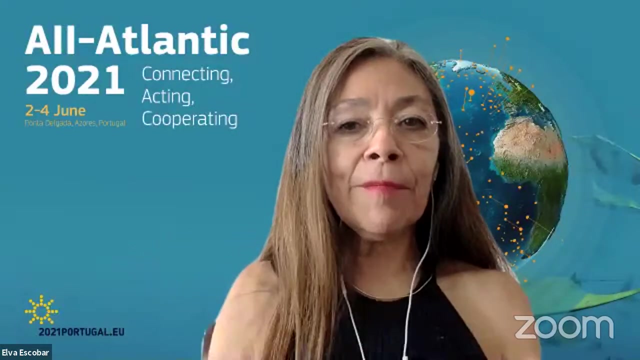 to understand what happens in the Caribbean and in Latin America, And there were a lot of programs and projects presented that are very useful. We just simply don't know them. They seem to be set up in a different area and we have to merge them and try to dialogue with them. 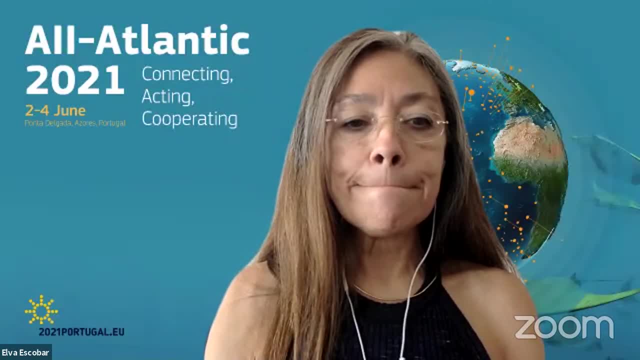 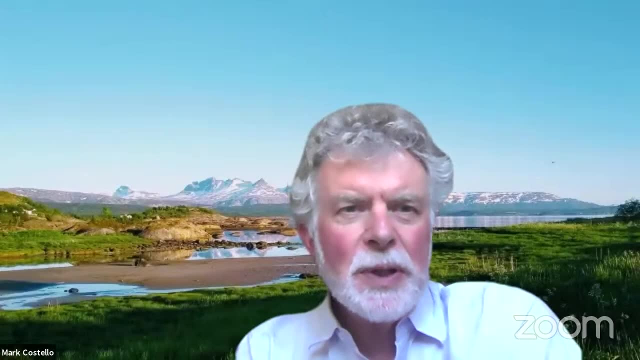 to bring them together to this program. Thanks, Alba. We've just about a minute left here, so we can break now, if you like, and we come back at a quarter past the hour for the next session, So I have an opportunity to make coffee. 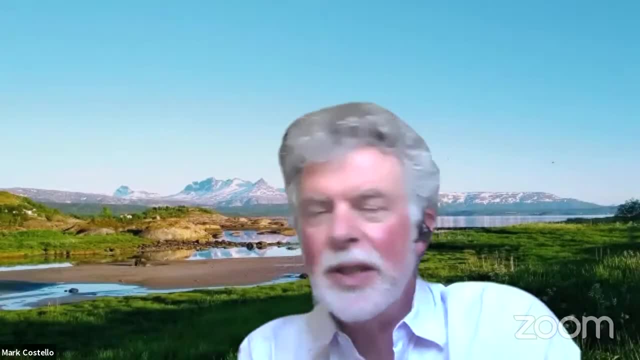 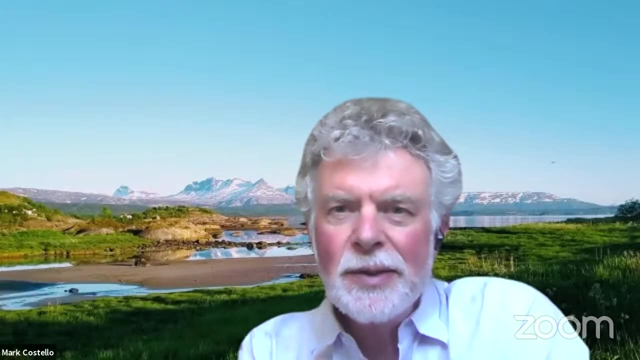 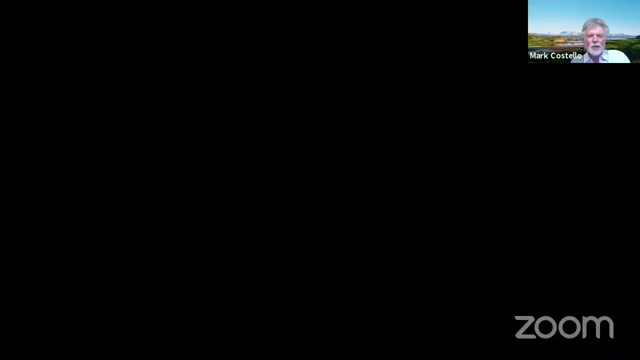 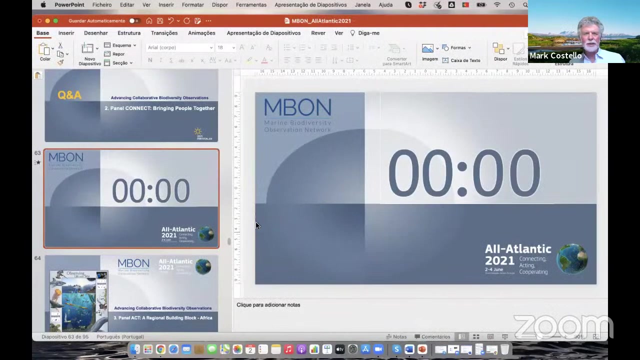 Get a glass of water and keep answering the messages in the chat. So unless anybody wants to say anything now, I think we'll take a break, But it's nice that the chat keeps continuing. Thank you, See you in 10 minutes time. 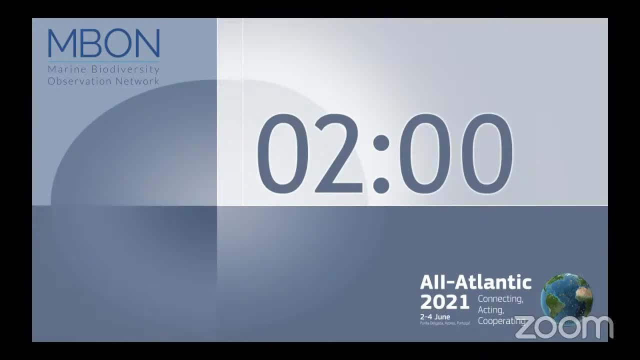 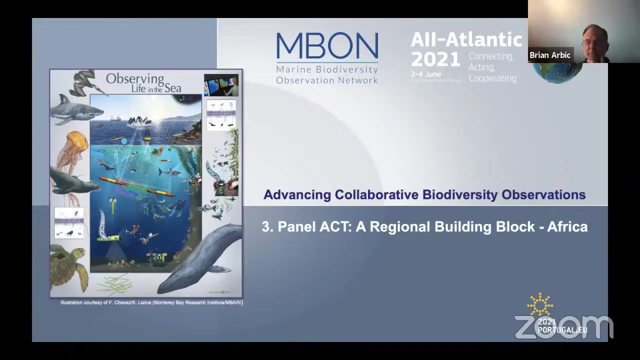 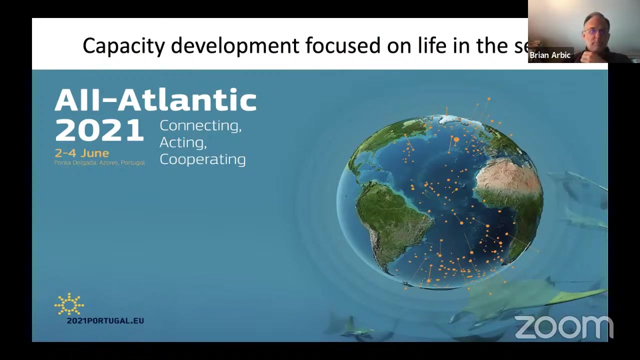 Thank you, Thank you, Thank you. So I think Brian Arbick will be the next speaker. Brian, if you want to turn your camera on, Hi, I'm here, Great, So welcome back everybody. And for this third act, it's actually called the Panel Act, which is kind of interesting. 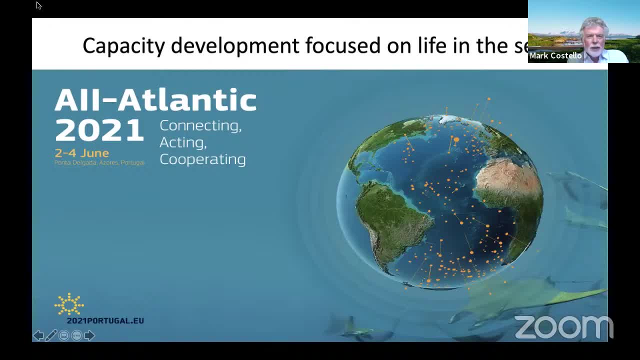 The Regional Building Block for Africa, And our first speaker is Brian Arbeck. Brian, you have the floor. Thanks, Can everyone hear me? Yep, Okay, great. So I'm going to talk about capacity development focused on life in the sea. 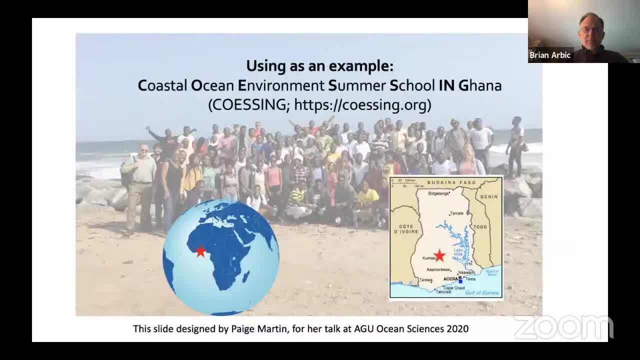 Next slide, please, And I'll be using as an example the Coastal Development Program for Africa: Coastal Ocean Environment Summer School in Ghana, or COSING, a website given there, which is a program that we've run in Ghana for one week every year in August since 2015,. 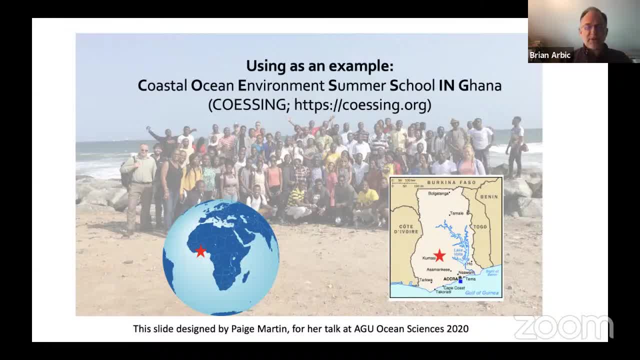 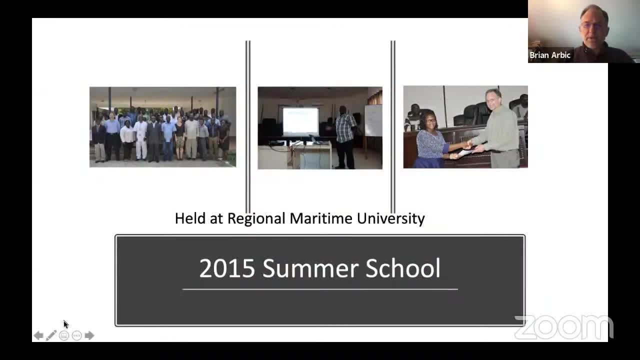 with support from the US National Science Foundation and others Next. So the school alternates between the Regional Maritime University, which trains people for maritime careers- you know, shipping ports, things like that- and the University of Ghana, which has a marine science department. 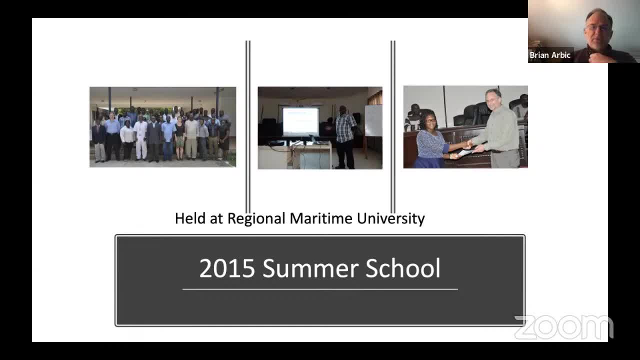 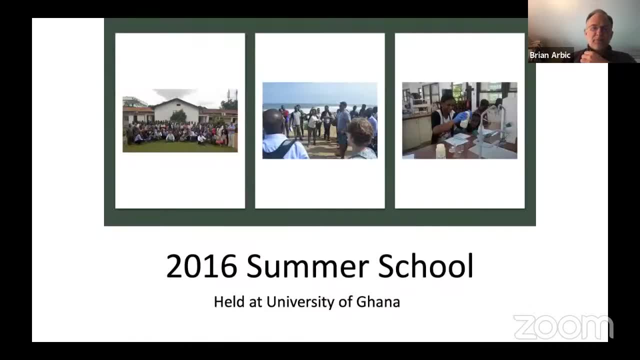 So the first year that we held it at RMU, it was fairly small, as you can see, and we only had lectures. Next, From 2016 onwards, we've had about 100 to 120 or so participants every year. 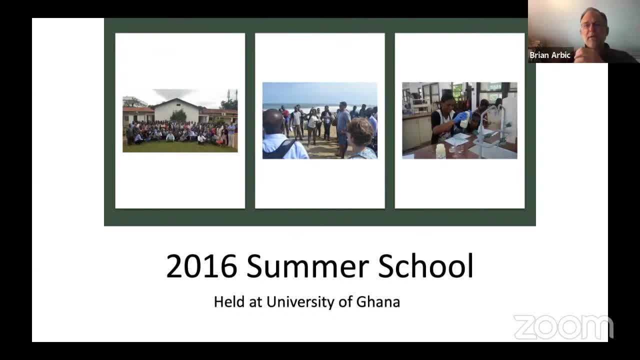 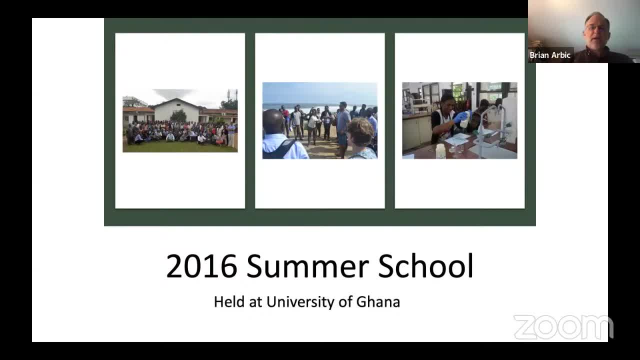 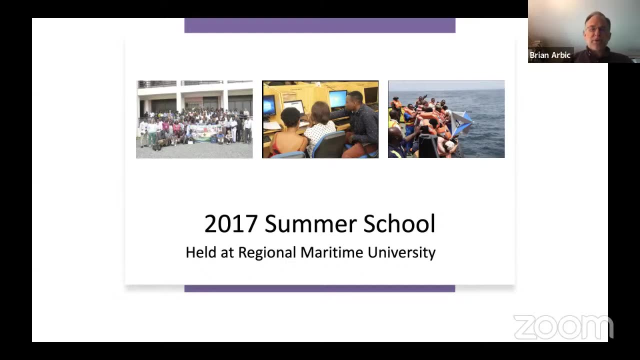 We have extra energy and ideas. We've done more things like trips: field trips to the beach, as shown in the middle, and labs, as shown on the right. Next, And we keep adding new things every year- In 2017, we added boat trips, where participants deployed instruments. 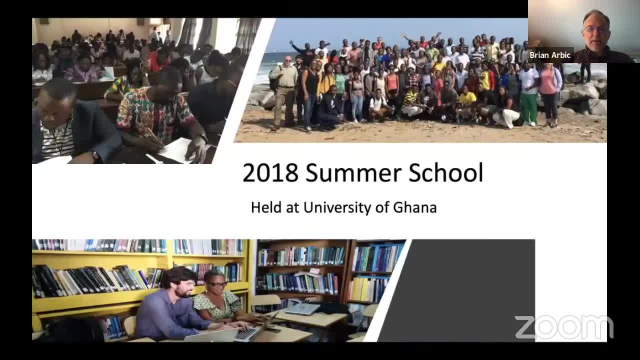 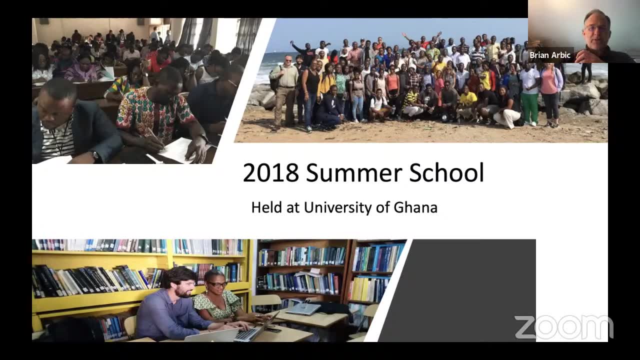 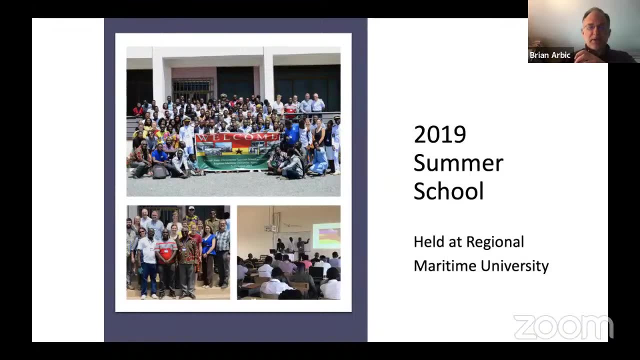 Next. In 2018, we had, as shown on the bottom, people working in small groups to do research. Next projects Next And then in 2019, the research projects was a larger component. Many people did projects and presented them in PowerPoint. Some of them said that this is the first time they'd. 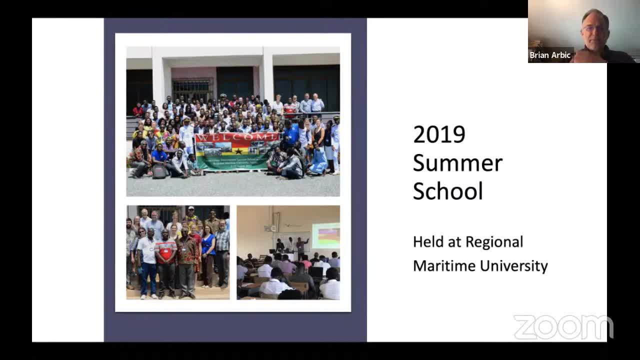 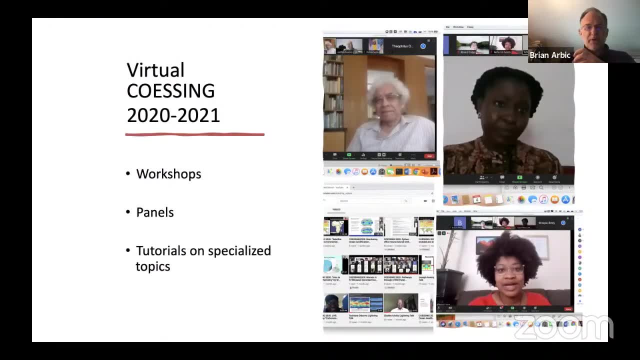 done something like that And that is shown in the bottom right. Next, So in 2020 and 2021,. of course, we've had to go virtual because of COVID, So we've had panels and workshops via Zoom, also tutorials on specialized projects, The panels: 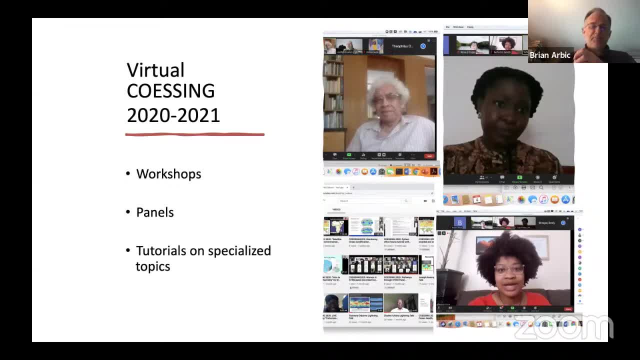 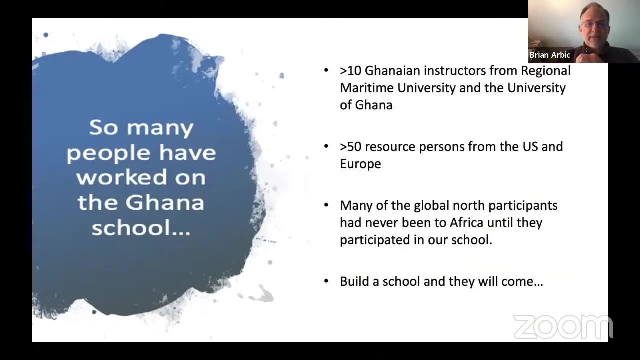 tend to be on things like women in STEM, STEM careers, topics like that, And the tutorials are a little more specialized, like: how do you analyze tie gauge data, or something like that. Next, So many people have worked on the Ghana School. There's just 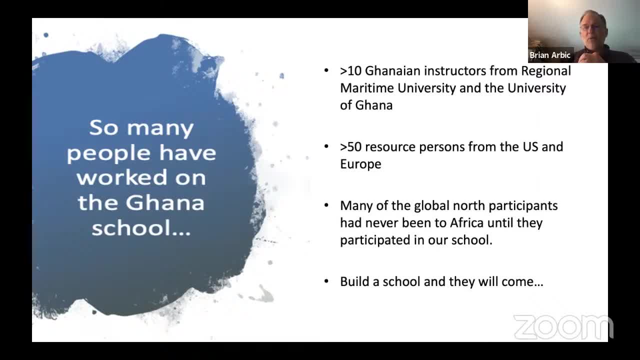 so many people I have to thank for this. We've had more than 10 Ghanaian instructors from the two universities that we work with, most of whom participate more than one. you know have participated more than one year, So in other words, return instructors, And we've had more than 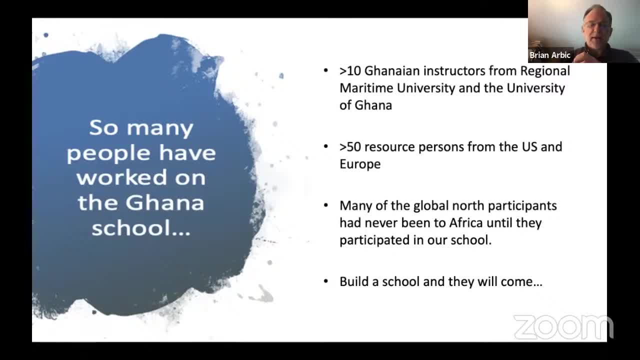 50 resource persons, all the way from undergraduates to faculty, coming from the US and Europe. And again, many of them are return participants. Many of the Global North participants had never been to Africa until they were in the US and Europe. So we've had more than 50 resource persons all the 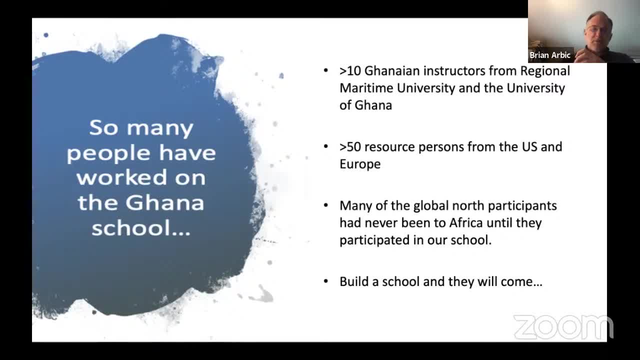 year And again, many of them have participated in our school, And some of those folks are now passionate advocates for capacity development, have taken Africans as PhD students or set up collaborations with African scientists. So the point is that if you do the hard work of setting 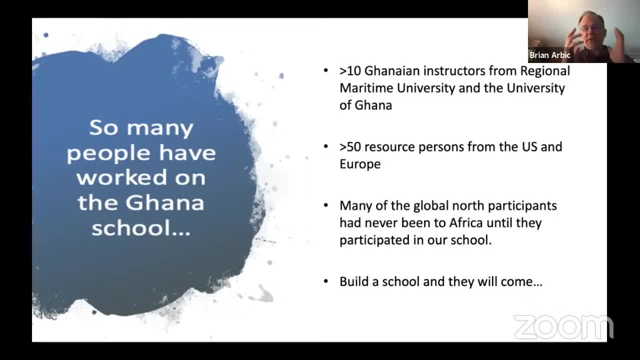 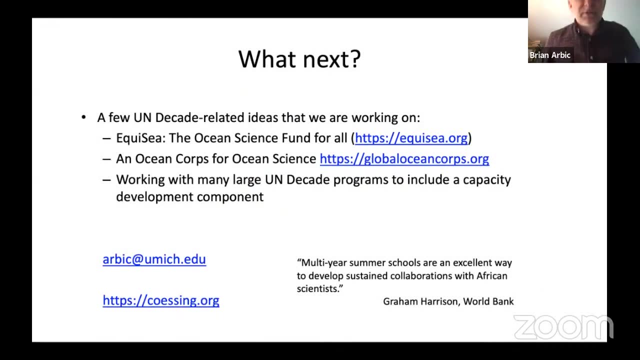 up a school, people will join you And it is a good way, I think, to get a lot more people from the US and Europe, for instance, working in Africa. And the next slide is the last one. The UN Decade, of course, presents a great opportunity to work on capacity development. 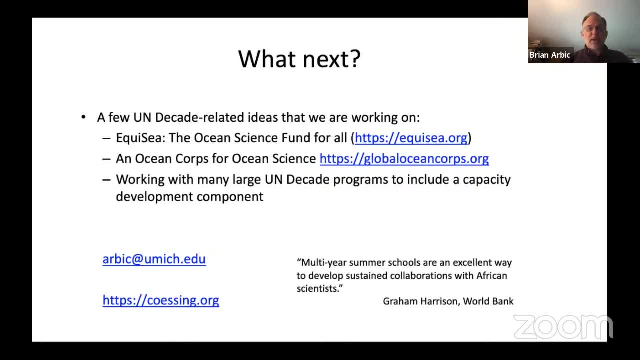 Here are a few UN Decade-related ideas we're working on. So I'm a co-lead of something called the Ocean Science Fund for All, which is going to be run well, probably mostly at the Ocean Foundation, And the idea there is that, as we all know, it's hard for scientists and under-resourced nations to get funds to do projects or host workshops or all kind of new initiatives of research, And the plan will be to have plans on the UN Decadeверful manager of thechet report in 2020.. And then other due to that, But I'm proud to say I'm very proud. 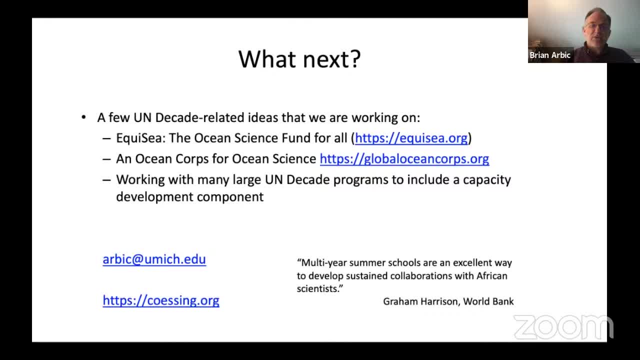 that we have allowed that qui do so and attended this climate impact conference, or the unfathomable US submission on the худural research project. We'll definitely send in like five to ten kinds of things, And so there should be a fund for scientists to apply to for exciting capacity. 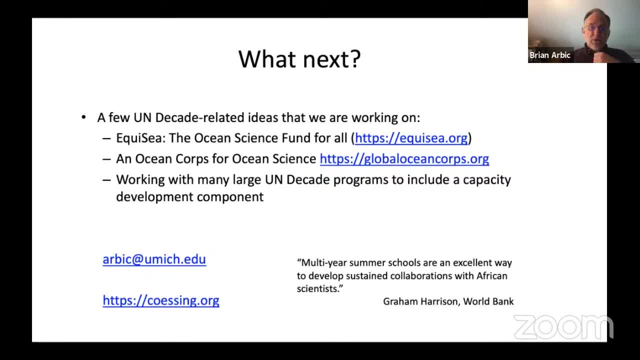 development projects. That's the idea there, And Ocean Corps for Ocean Science has also been submitted as an idea for the decade, And so the idea there is that inspired by what we're doing in Ghana and also by the Peace Corps- I was a Peace Corps volunteer myself years ago, I think. 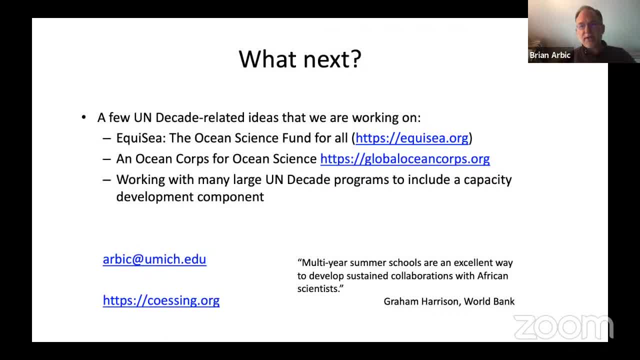 that there should be many, many schools, like what we're doing in Ghana, around the world, And that's the idea of an Ocean Corps that you know, if you have the infrastructure, you get young people excited. you know, go abroad and start collaborating around the world. It will work If you have the 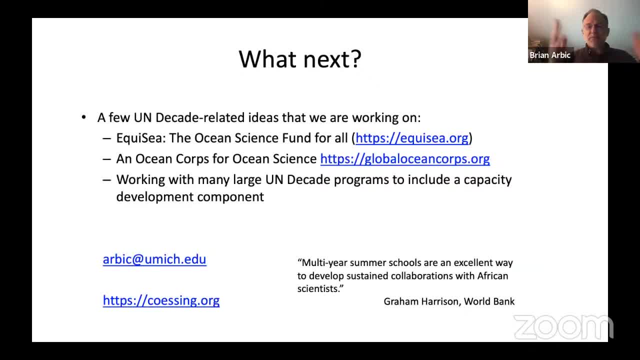 money, it will work. I mean, I talk about this idea to many. I was at Scripps a few months ago talking about with collaborators. young people especially are super excited. They want to do this kind of thing. We're working with many large UN decade programs, including NBON, to you know. we talk about these. 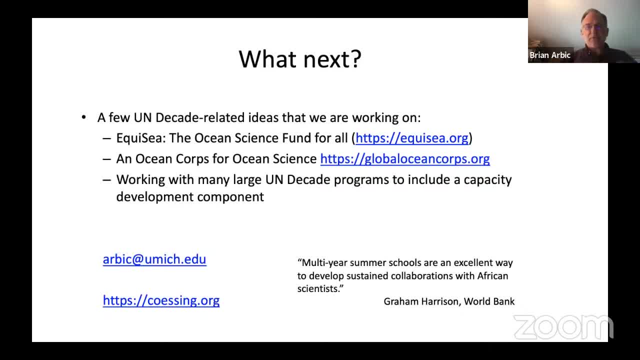 ideas. If all these things were implemented, we would love to, just, you know, go full bore and expand this kind of stuff. And I'll close with two things. I can see a few of our participants are from previous schools, are on the attendees list, And I'll just mention Michelle Clotty. 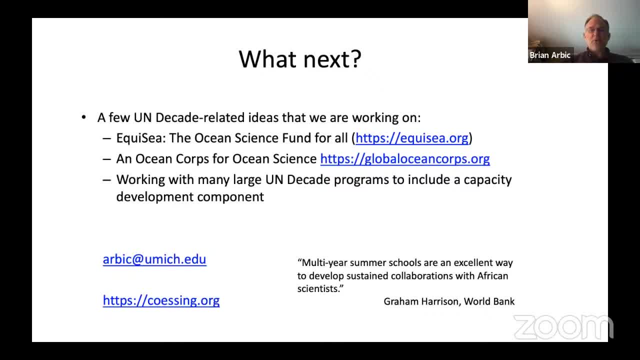 is a fishery researcher. She's a fishery researcher. She's a fishery researcher. She's a fishery scientist in Ghana. She participated in our school at least once, maybe more than once, and learned how to use satellite data to monitor sea surface temperature, which is, of course. 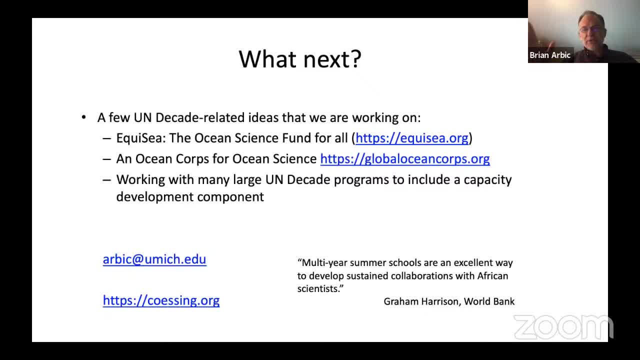 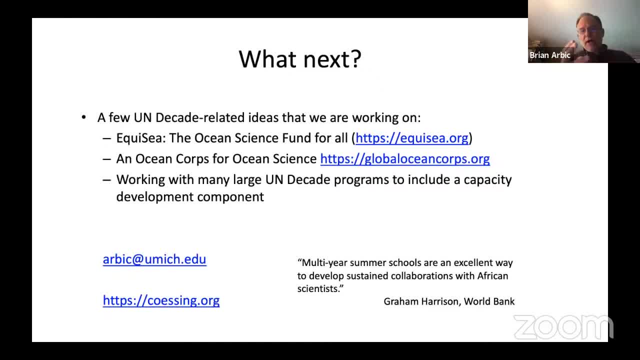 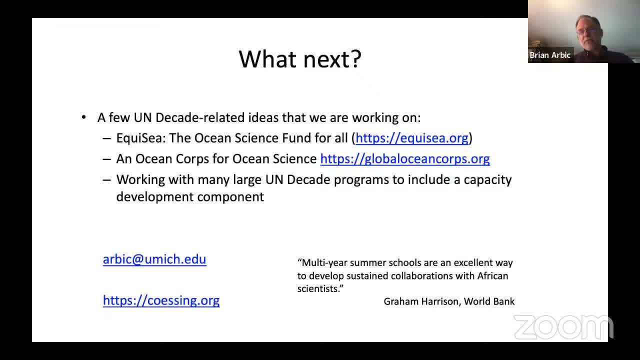 but many of them can commit for one week every year And so if you have a school every year and you go there for one week, you can sustain something like this and grow lots of collaborations. So I think if you had a lot of funding for this kind of stuff, you could have schools focused on 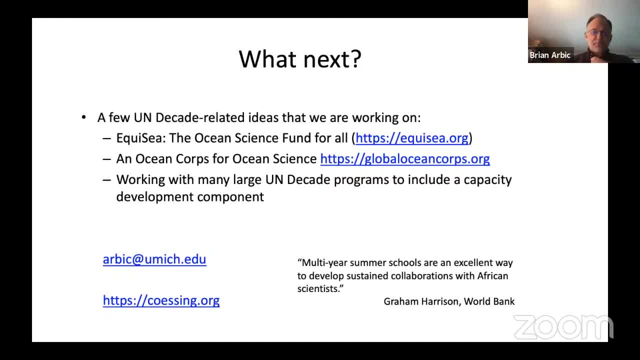 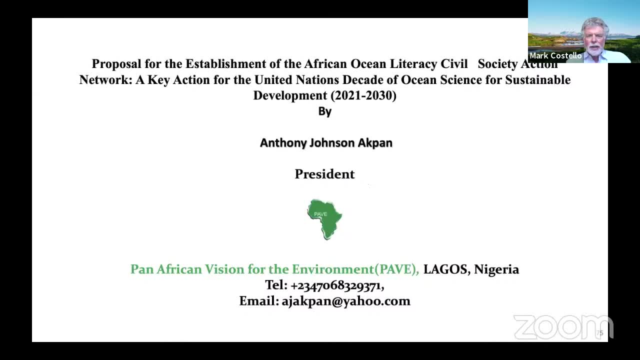 life in the sea issues. Thank you very much. Thanks very much, Brian. It's a very exciting initiative. I'm getting lots of positive feedback in the chat, So our next speaker is Anthony Johnson-Akpan. Anthony, you have the floor. 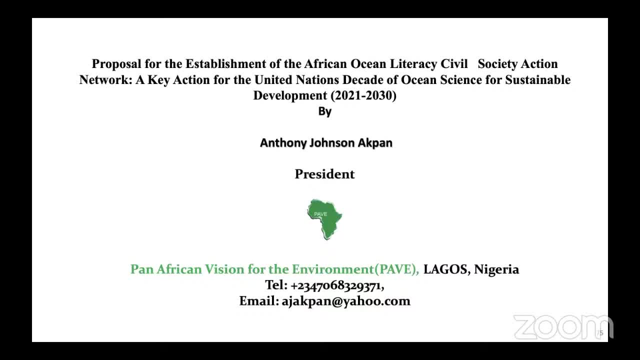 I don't hear Anthony yet, but we can turn your video on. Yeah, my video is on. Thank you so much and welcome everybody. My presentation is basically about our proposal to the ocean decade And we basically have noticed that in Africa generally there is very little knowledge and appreciation about the 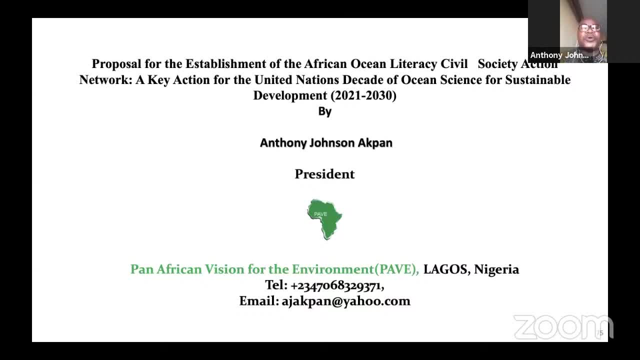 ocean. Hence the need to begin to build capacity and increase ocean literacy on the continent. Hence our proposal, which we have submitted to the decade action, to establish an African Ocean Literacy Civil Society Network, which we believe will be a key action for the United Nations Decade of Ocean Science for Sustainable Development. 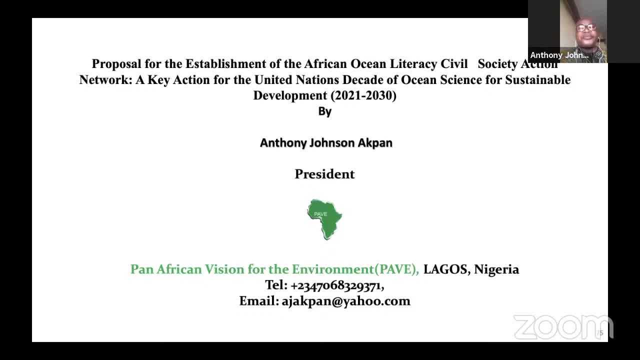 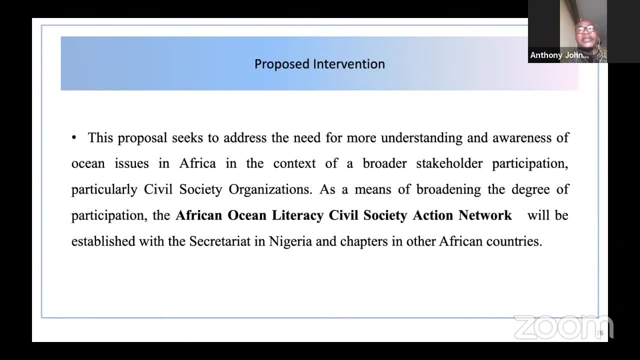 2021-2023.. Next slide, please. This proposal basically seeks to address the need for more understanding and awareness of ocean issues in Africa in the context of the broader stakeholder participation, particularly civil society organizations, As a means of broadening the degree of participation. 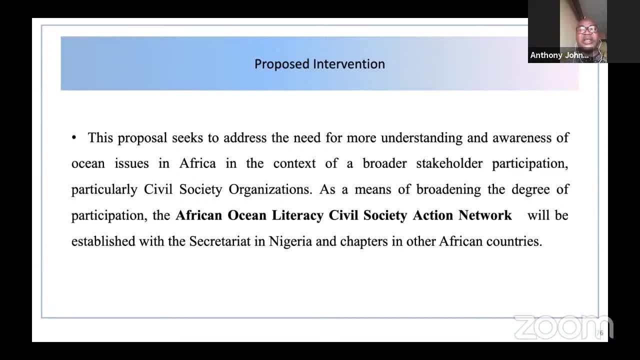 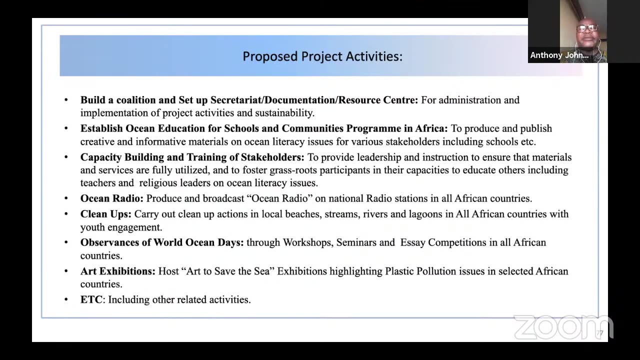 the African Ocean Literacy Civil Society Action Network will be established, with the Secretariat in Nigeria. We also hope to have chapters in other African countries. Next slide, please. So, basically, some of the things that we're going to be discussing today will be related to the 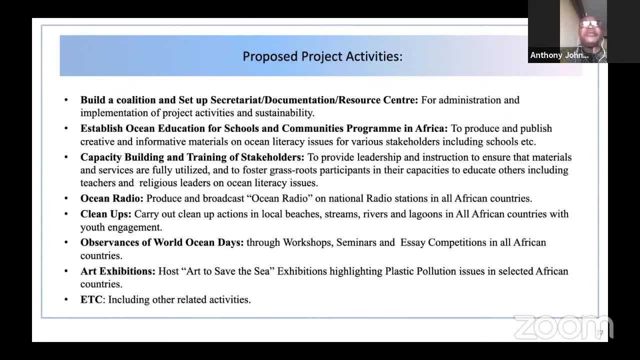 project. Some of the proposed activities that we anticipate that this proposed network will begin to carry out to build capacity. it's not conclusive, but some of them will be to build a coalition and a set of secretariat or, more or less, a documentation centre for 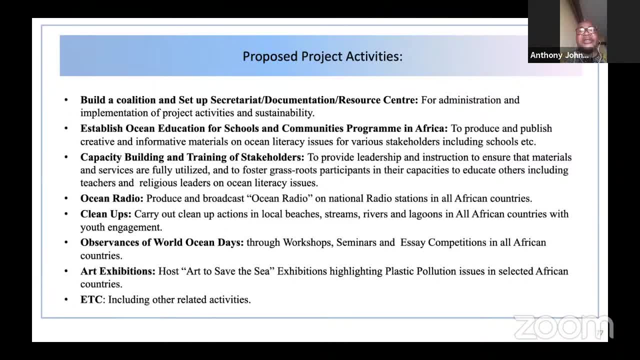 administration and implementation of the project activities and for sustainability. Some other activities will include establish ocean education and development programs, education for schools and communities program in Africa. we believe it is important to begin to have this ocean literacy knowledge even at the grassroots level, at the primary level. 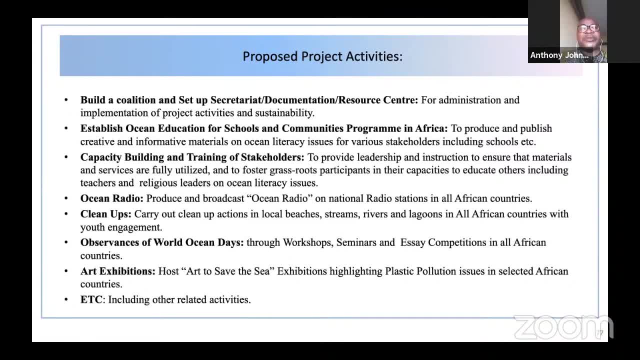 so that the children, as they grow up, starting to use, begin to appreciate what the ocean is and how they can contribute to its protection. another, capacity building and training of various stakeholders, including the civil society, the media, government and all key stakeholders, the maritime sector, you know, to really understand what role they have to play to safeguard the. 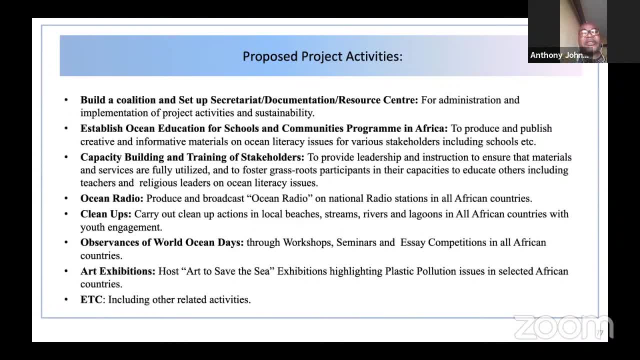 ocean. we're also looking at the establishing ocean radio program in various countries. when we're touching this program where we're educating the general public about ocean issues, we are still looking at um organizing, particularly getting youth involvement in ocean cleanups, and look at beaches, streams and rivers and lagoons in all countries and we think, engaging. 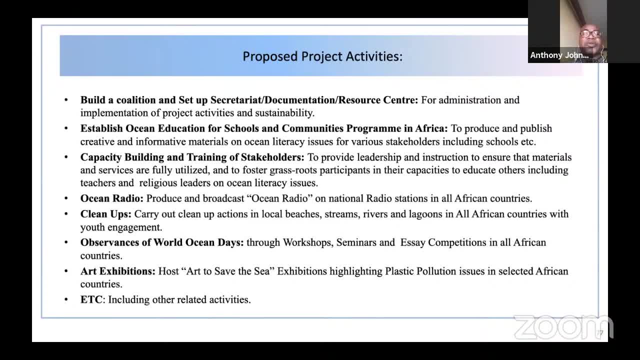 youth is critical and also we are looking at the observances of the world ocean days and also the African day. we see and uh ocean also through workshops, uh seminars and essay competitions in all African countries countries and, more interestingly, we're also looking at using art exhibition to 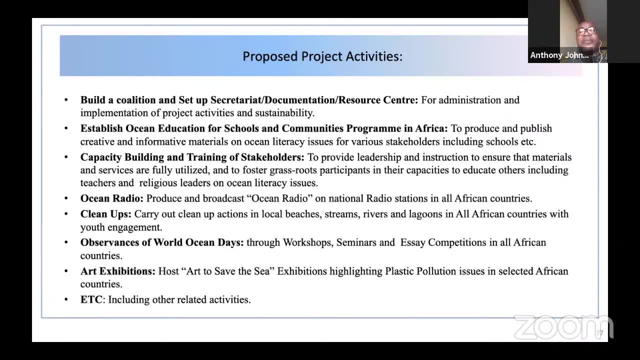 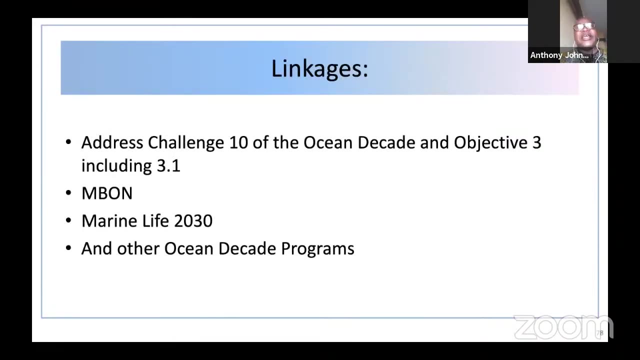 host art to save the sea exhibition highlighting plastic pollution issues in selected african countries. so these are just some of the activities that we think the proposals can bring to bear. next slide, please, so we see linkages like the, the, the question i posed to murray and age, i mean. 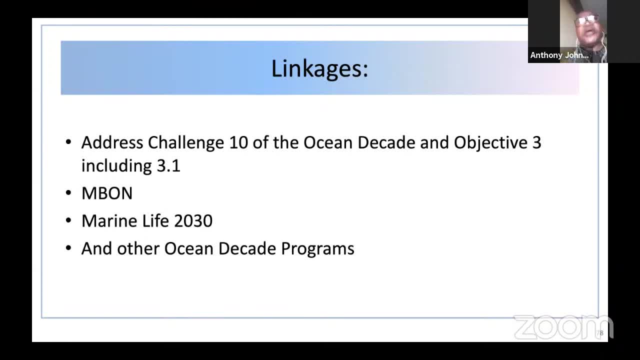 ocean literacy is key. so, whatever you're doing with observation or remote sensing or whatever, it has to be a linkage that people can really now understand from the technicality of the information you are generating. and how does that really apply um physically to to their lives and to things they can relate with. 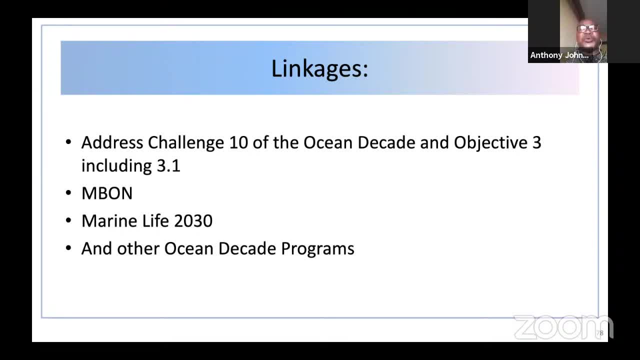 so we think we see linkages uh to, particularly to address talent 10 of the ocean decade and objective three and objective uh 3.1 and um the more projects i've just been spoken about, and then the marine life project and other related ocean decade programs such as the. 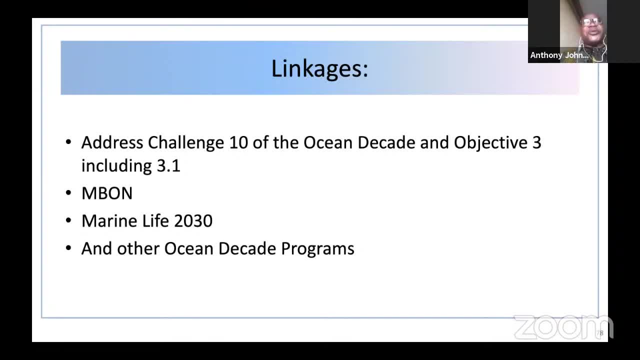 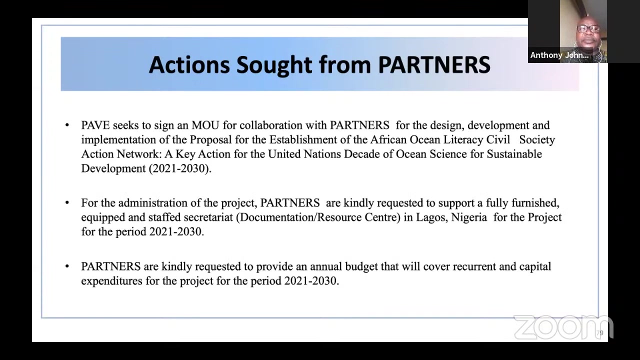 high atlantic and all of that. i mean we can integrate and use our ocean literacy skill to vibrate and also encourage the, the, the, the product coming up from your, from your various projects and researches, and enhance people: comprehensive knowledge next slide. so basically, uh, we are, we are still at the proposal stage and we are, we are calling. 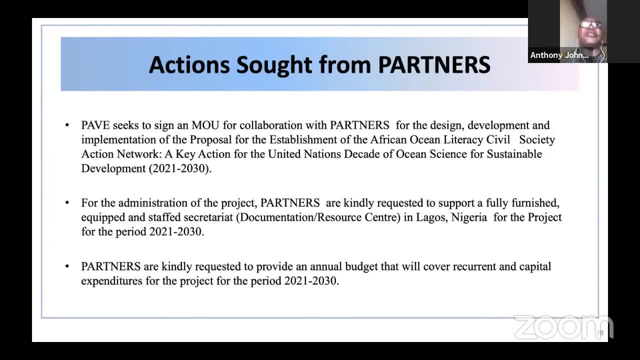 for partners um to partner with us to make this um proposal a reality, because we see it's really key, is a great necessity and um and the knowledge of the ocean on all other continents is high up there and on the african continent we see that it's very low and that we also see the number of 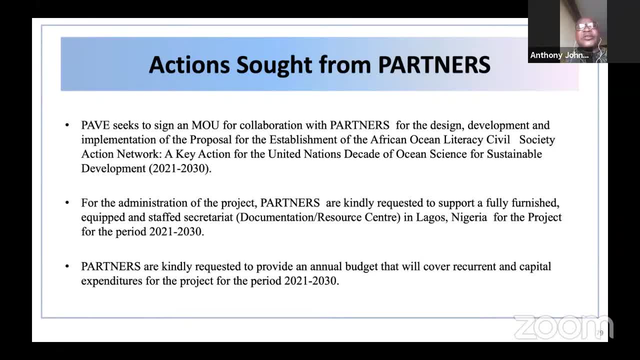 scientists, ocean related scientists that are coming out from the continent. so we think by the time we are able to raise awareness among stakeholders about the importance of the ocean and its related activities, then more ocean scientists will be coming out from africa. so in that context, to follow up our big um, our big uh project on the continent, we seek the mou. 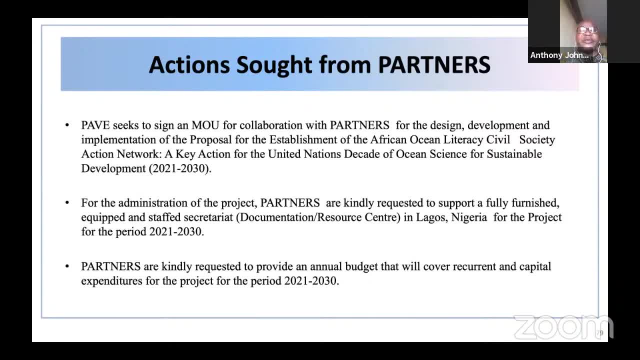 collaboration with potential partners in the design and information of the project. um there's nothing you can can do without um money, so we also establish a secretariat for the project to run and create um possible funding support from potential projects and partners. that are where we share. 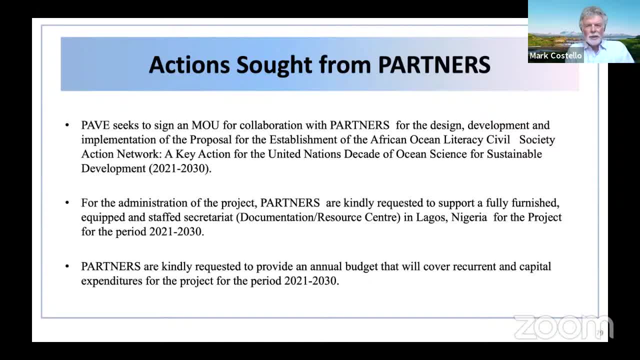 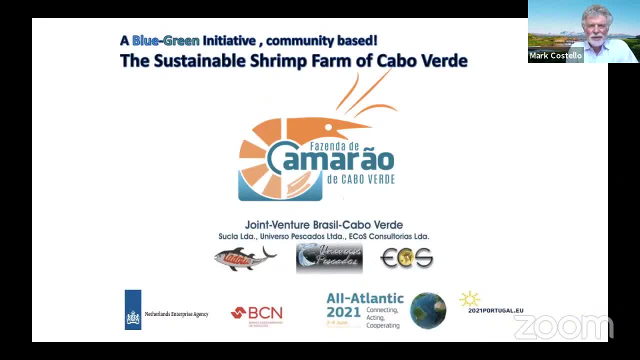 similar aims, thank you. thank you, anthony. i think we're running out of time. i just finished as well. thank you, that's great. that's a very another, very exciting and excellent idea. so the next talk is a little bit different, on sustainable shrimp farming. um so, tatiana, i think, is the speaker. yes, okay. 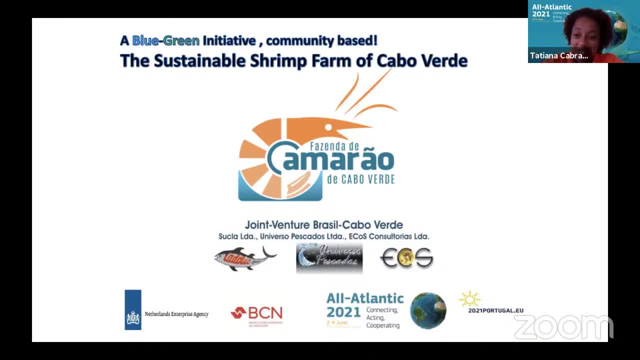 and welcome everybody. um, i am tatiana. i work at fazenda. come around the cup of earth. uh. it's a joint venture, uh, between brazil and capo verde. it started the idea of the project started in 2008, uh, but overcoming the challenges like accessing the financial loans, fund findings. 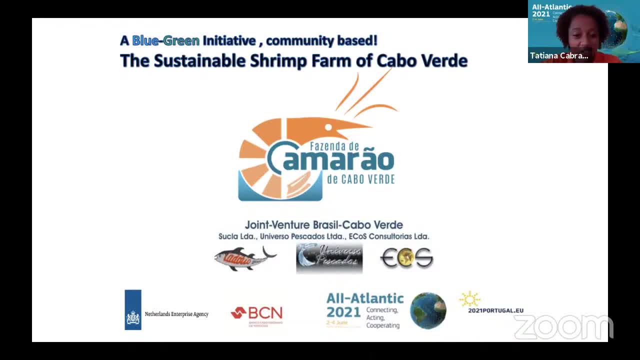 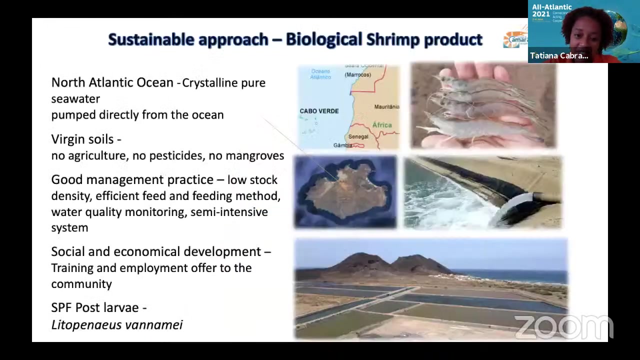 techno, technology, know-how transfer, logistics and all these. um, so we started the production in 2018, so we're very new in the market. um, it's uh, the project. it's a community based uh, so, uh, we are the first, uh- shrimp farm of the country of capo verde. next, please, next slide, please. so we located. 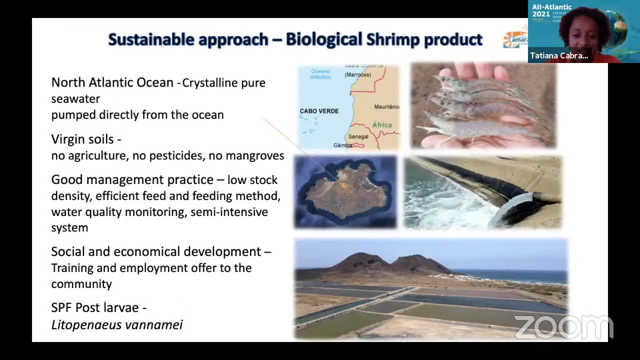 um in the island of san vicente, one of the islands of cabo verde, in the uh caliao, which is a small fishing village, and so the isolation is an advantage for us. it brings advantages and disadvantage. uh, one of the advantages: that we are free from heavy industrial pollution, so we have crystalline, pure sea water. 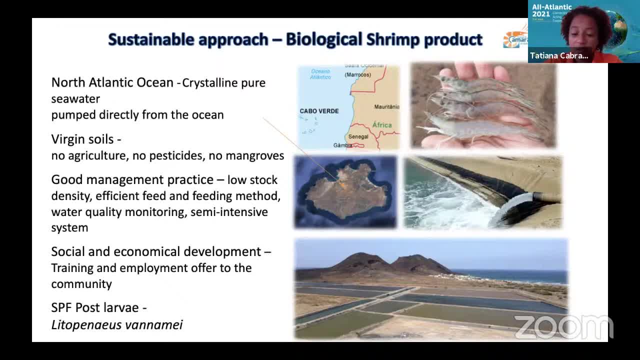 we pumped it directly from the ocean. uh the farm was built, uh in under virgin soil, so there was no agriculture, no pesticides, no mangroves, so there was no. nothing was destroyed to start, uh the farm. so we have a lot of environmental impact. so we use all that to our advantage, and so we practice. 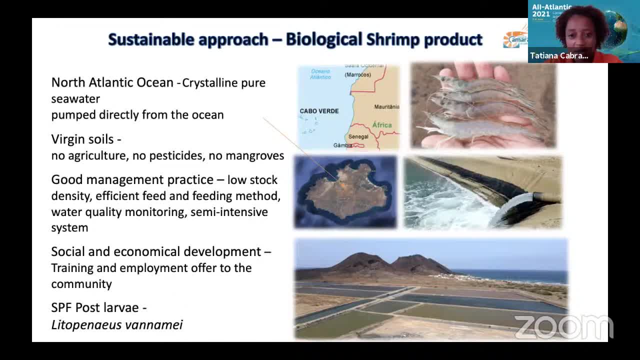 good management so we have low stock density. uh. so when you have a low stock density, you don't have to introduce chemical products. we use all the our natural resources, we monitor our water and, uh, as i said, we are based in a community so we invest a lot in training uh. 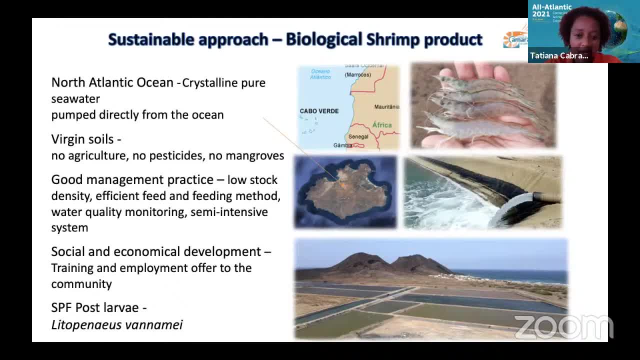 we have a lot of people who are from cali and we employ mostly people from uh caliao and uh to to. to continue with and the advantage we have of being isolated and to have the sustainable approach. we imported the post larvae we start- we started first with uh importing post larvae. 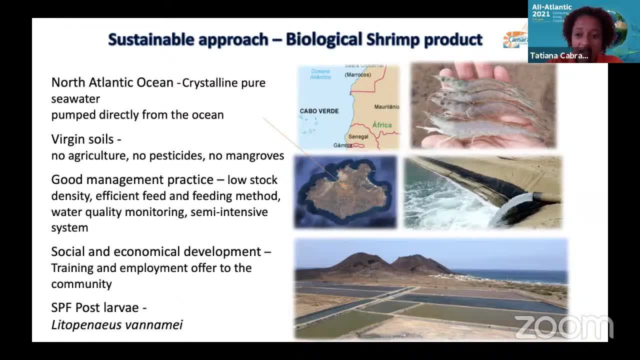 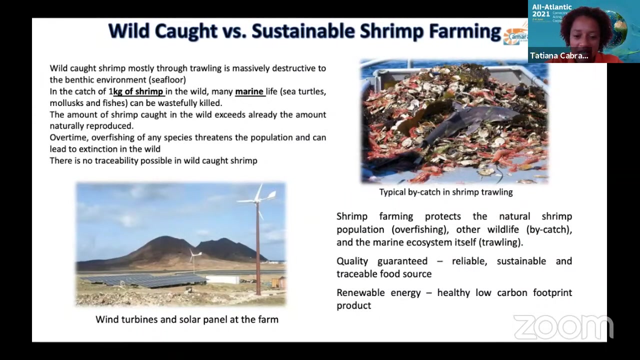 uh specific free, pathogenic free, so we maintain our environment free of uh any pathogen we use. i will tell you our products: um, they, they are more skeptical and they're and, and when you talk about wild-caught shrimp, for example, it's more acceptable, uh, but when you talk about ocean sustainability, you have. 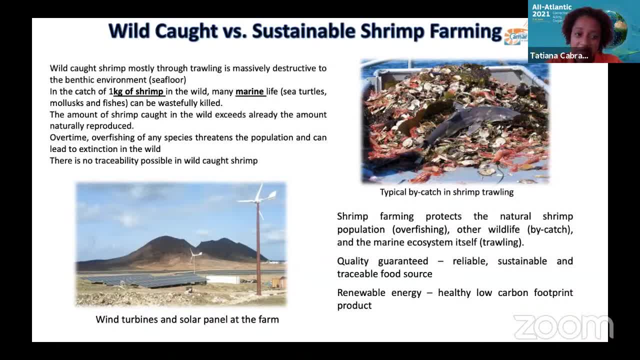 to think of the traceability of the product and you have to think how it was caught. so, for example, uh shrimp, a lot of the shrimp is they use a trolling uh method which is massively destructive to our benthic environment of the seam floor. so, um, people need to be aware of that, so they know. 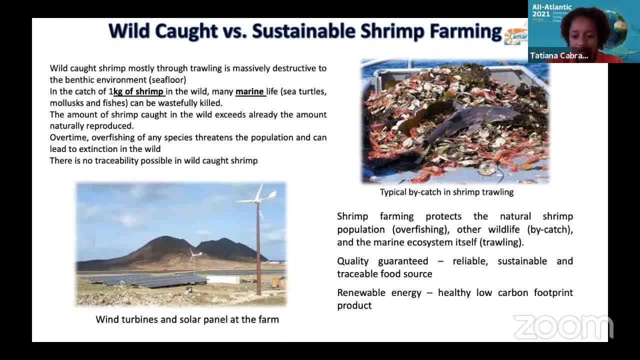 uh about the sustainability and uh also uh, compare that with a sustainable shrimp farm where you you can trace your product, you know where it comes from, and uh, you and also in the farm we use renewable energy to reduce our carbon footprint, so we have a biodegradable. 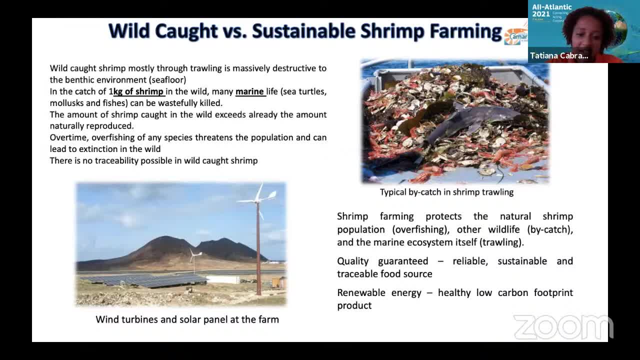 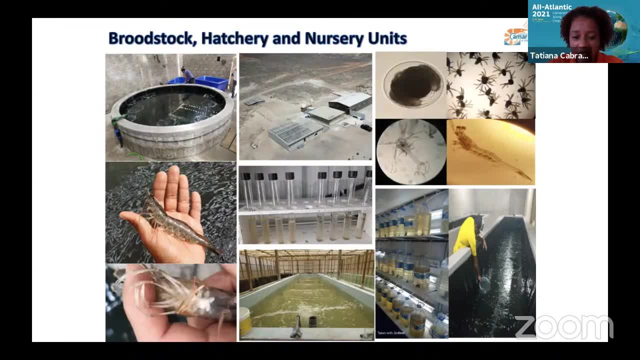 biological product next, please, uh, the next slides are just to show a little bit of our work. uh, so first we started importing the post larvae, but due to the logistics of transport, because being isolated it's, it's good, uh, it has advantages. but also when it comes to the logistics, uh, there's. 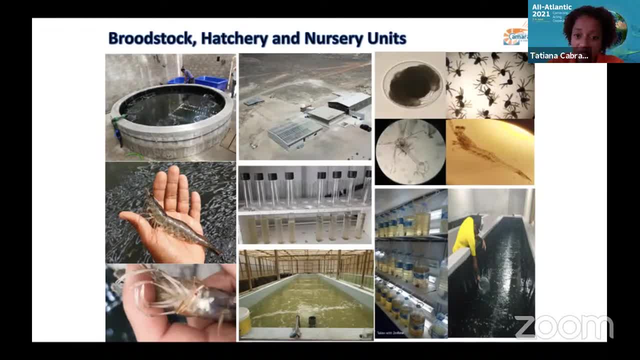 a lot of difficulties. so we had to start our one post larvae production. so right now we have our own hatchery and we do any everything from the start. so we have our own breeders and we produce our own microalgees in the farm and so we go from the hatchery, which is the first. 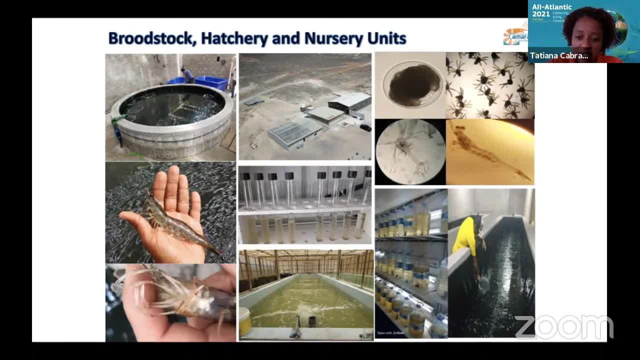 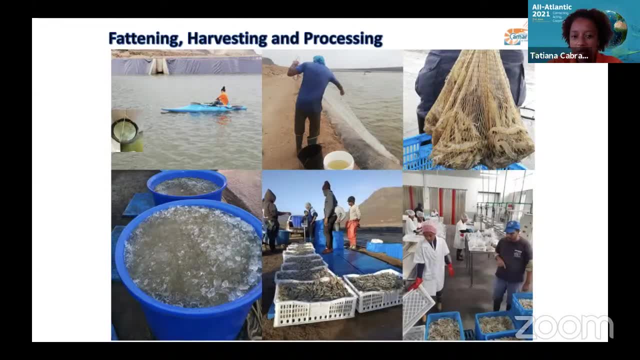 production: the first larvae stage all the way to the nursery units and then the next slide, i ll please- and to the grow out ponds, where you grow them to the uh commercial size, which is 12 grams. um, um. Here in the picture we have an example of how we do our feeding. 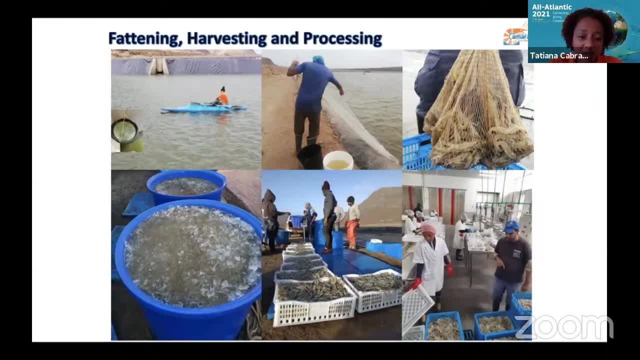 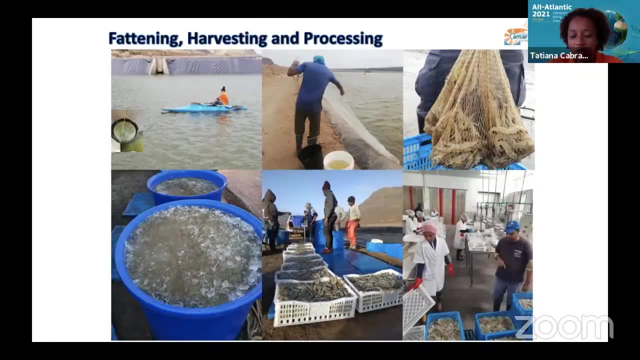 So we use feeding trays to monitor our waste and also if there's a mortality, and to better to maintain your water quality. We do biological sampling, So we weigh and we analyze our shrimp every week, And here we have an example of how we do our processing. Next, please, 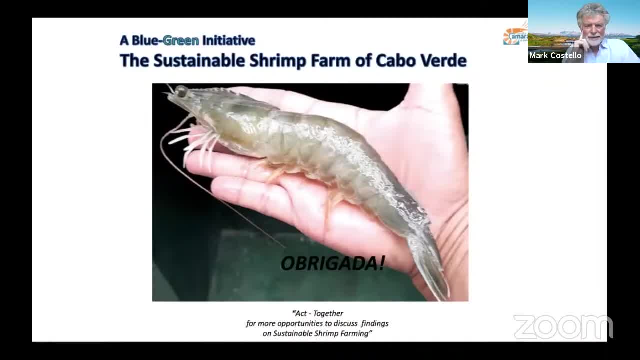 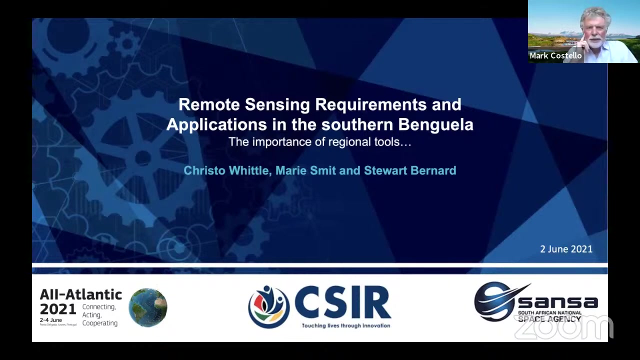 So we need to wrap up: Yes And it's thank you, And together we will come up for more opportunities to discuss findings on sustainable shrimp farming. Thank you very much, Satyana. Sounds like a dream place to be farming. Our next speaker is on something completely different: on remote sensing by Christo Whittle. 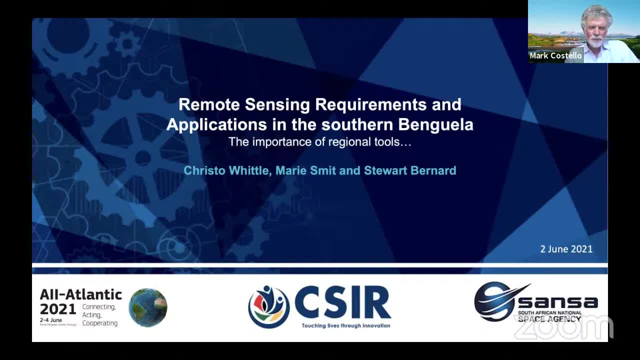 Thank you, Christo. You can turn on your video, Christo, and start speaking. As ever, I forget to turn on my video and my mic. Good afternoon, fellow delegates. Thank you for providing me with the opportunity to showcase some of the observation, research and development conducted at the CSR South Africa. 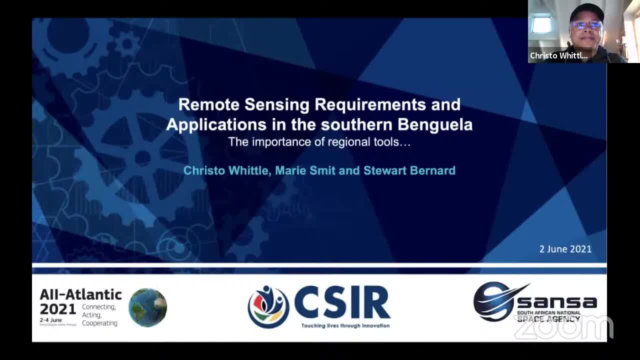 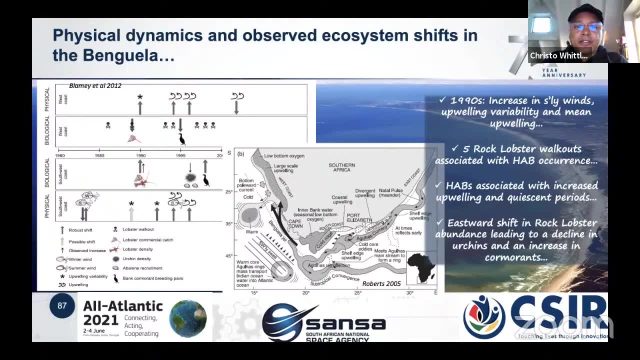 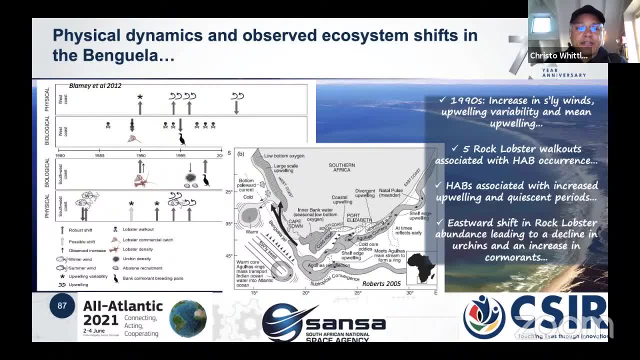 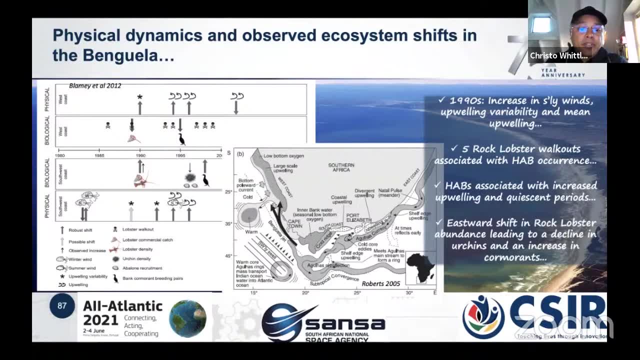 cells that form impressive cold plumes from Cape Columbine to Cape Recife all around the coast, sustaining a nutrient-rich, productive environment that supports lucrative fishing grounds On the broader shelf south of the current, the Gullis Current, south of South Africa. 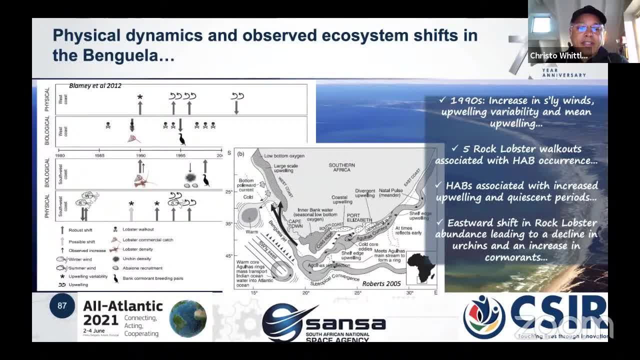 the Gullis Current has a varying influence throughout the year, intermittently injecting plumes of oligotrophic water towards the coast, So it's a complicated environment. The schematic on the left illustrates an ecosystem shift in the southern Manguela during the 1990s. 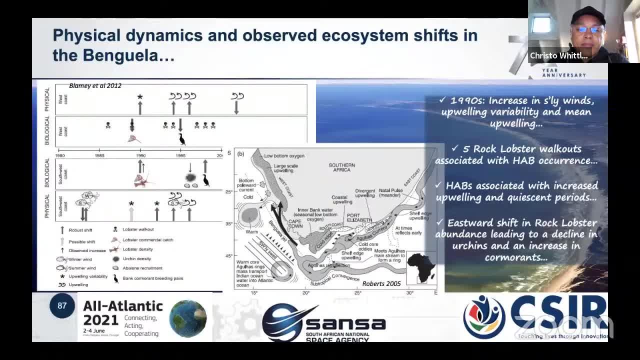 when southerly winds mean upwelling, and upwelling variability increased in comparison to the previous decade, particularly between Cape Columbine and Cape Gullis. Increased upwelling and quiescent periods are closely linked to an increase of dense dinoflagellate plumes. 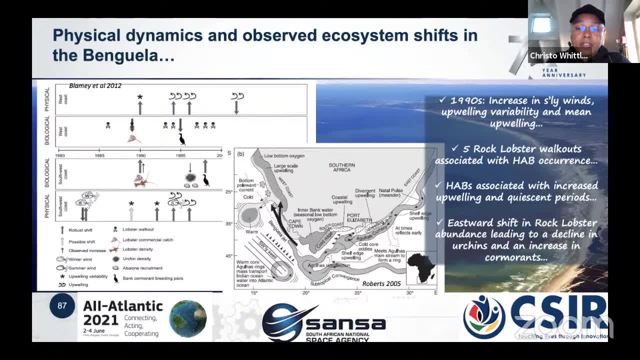 Subsequently, an eastward shift in rock lobster abundance was observed, with this shift also being reflected in the increase of rock lobster predators and the decrease in rock lobster prey and associated species, Also known as rare types. these algal blooms could have wide-ranging harmful effects, including the depletion of. 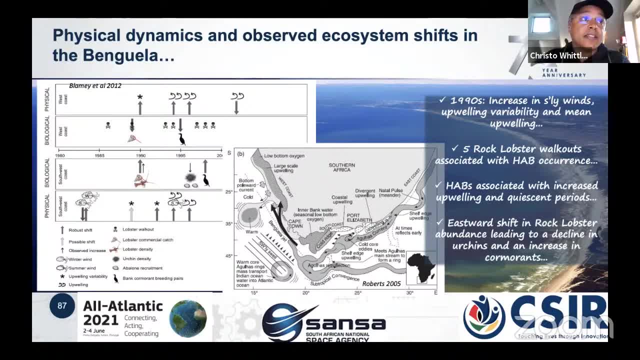 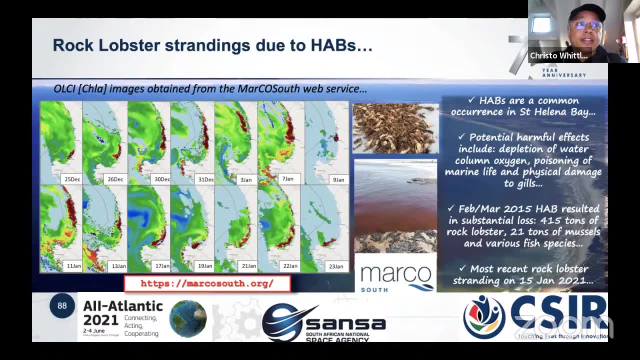 water column, oxygen poisoning of marine life and physical damage to gills. Next slide, please. So large marine mortality resulted in the removal of 415 tons of rock lobster, which is a significant shift in the natural habitat life of the rock lobster. 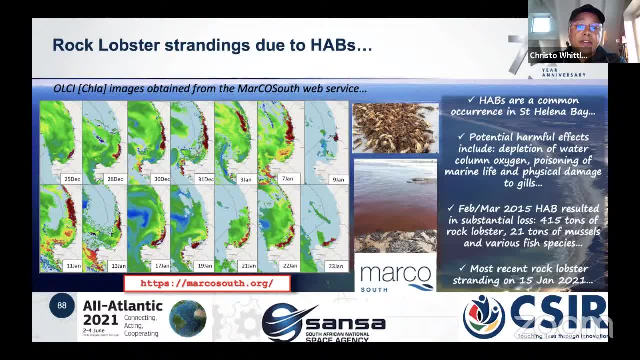 The next slide shows a picture of a large rock lobster- 21 tons of mussels and various fish species from the beaches within the Centralina Bay area during the February- March 2015.. As recently as January 21, a less severe rock lobster stranding occurred in Centralina Bay. This is illustrated in the sequence of images on the slide. The red blob and the accompanying chlorophyll-A images are indicative of a harmful algal bloom growing and translating in this retention zone. 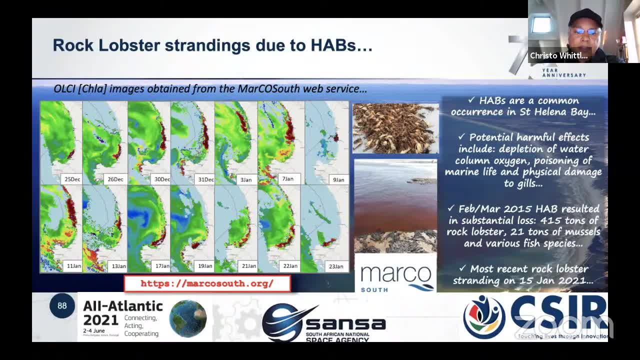 Its presence eventually resulted in rock lobster stranding in the southern part of the Bay on 15 January 2020.. The rock lobsters are present throughout the entire Bay Area, including the northern part of the Bay. information is still being released. The rock lobsters that are present in this region are the most common and are commonly found in the Centralina Bay area. 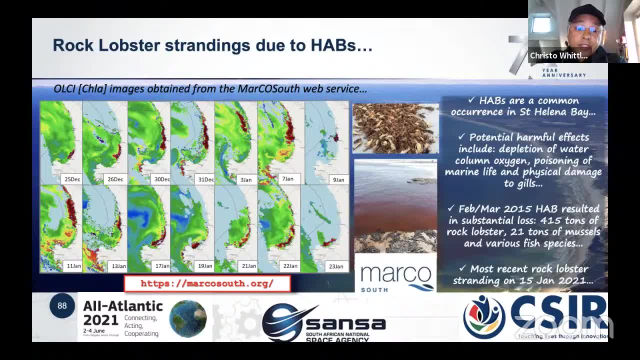 the band 15 january 2021. we are, of course, on the hunt for reliable earth observatory ecosystem indicators that can be monitored and form part of an early warning system. possible shifts in the southern meguel inshore region, particularly factors that promote the increase of hypercurrents. 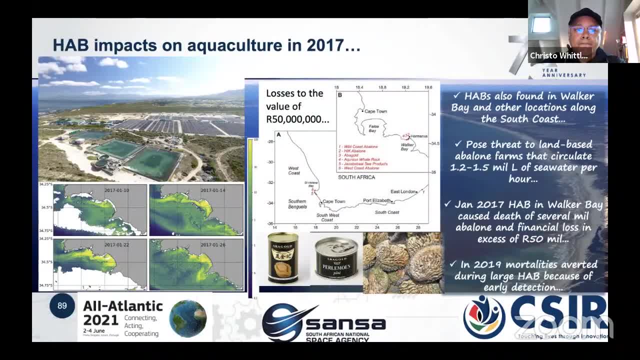 next slide, please. land-based abalone farms circulate about 1.2 to 1.5 million liters of seawater per hour, and one of the biggest threats to production is posed by harmful algal blooms in the adjacent marine environment. in january 27, walker bay was inundated by a large red tide that impacted three 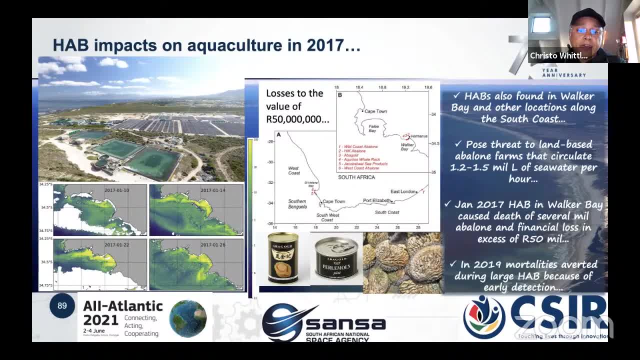 land-based abalone farms, causing the death of several million abalone and financial losses in excess of 50 million rats. land-based abalone farms circulate about 1.2 to 1.5 million liters of seawater per hour. all the aquaculture industries are to some extent susceptible to the negative impact of red tides. 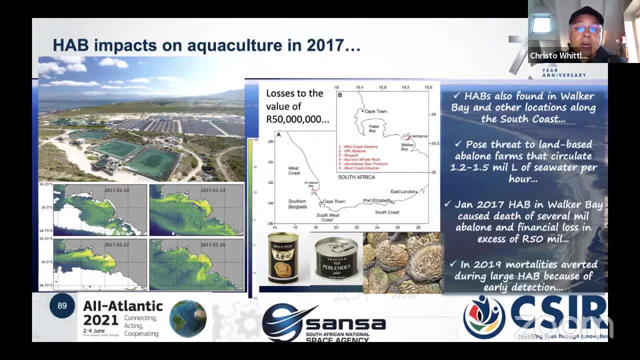 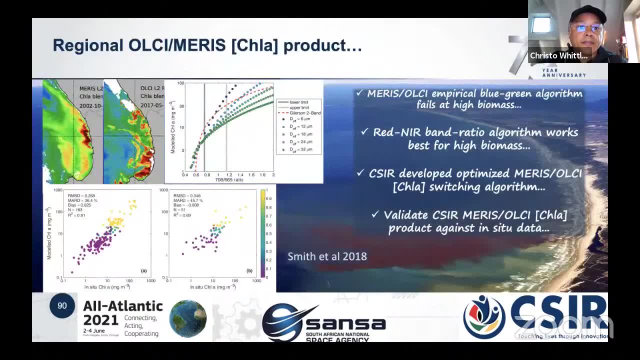 whether directly through the simulation of toxins, mechanical damage, or indirectly through the anoxia from bloom collapse. next slide, please. so we need to be able to identify, monitor high biomass blooms. however, empirical blue-green algorithms used to retrieve chlorophyll, a concentration for the mirrors and ultrasensors. 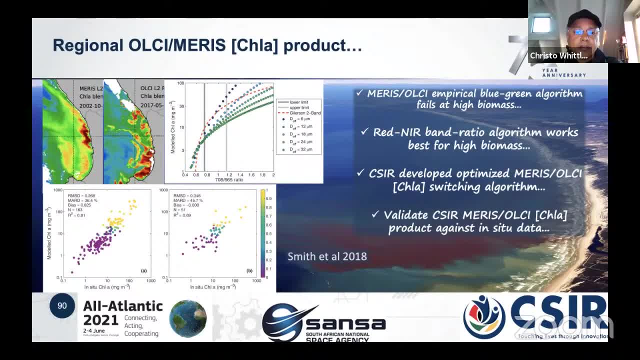 present with accurate and accurate results, with accuracy issues when high biomass pixels are encountered. under most conditions, a new water leaving radiance contribution in the near infrared is considered as radiance contributed by aerosols and subsequently removed from the empirical. green. blue-green chlorophyll, a concentration product. 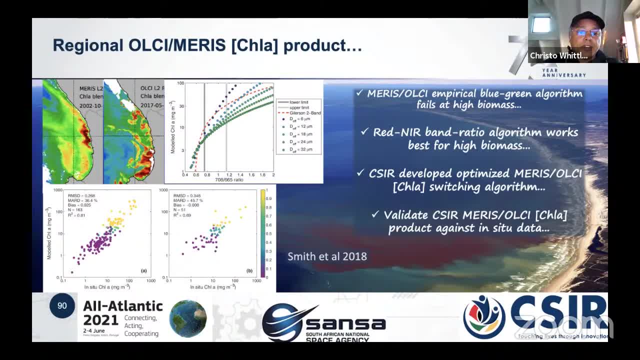 this assumption holds except in coastal environments with large reflective contributions from surface sediments or very high biomass biological blooms such as the benguela. the csrr other observation group developed by the university of san francisco and the university of san francisco developed a novel technique to apply and blend two different chlorophyll a concentration algorithms. 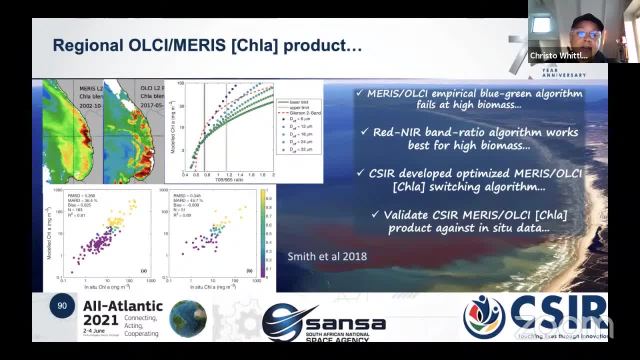 an empirical blue-green algorithm for low to moderate biomass and a red near infrared band ratio algorithm for moderate to high biomass. this optimized maris olchi switching algorithm showed superior performance in the southern megawilla compared to any single algorithm when compared to nc2 data. next slide, please. 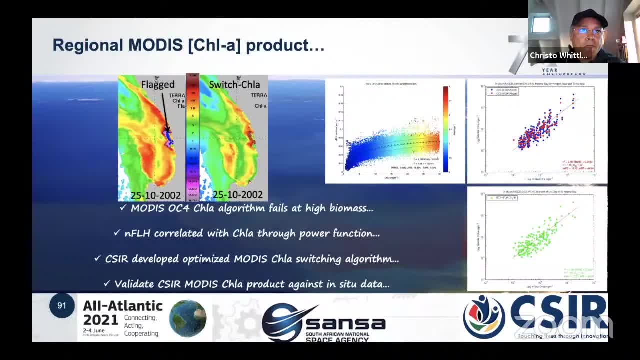 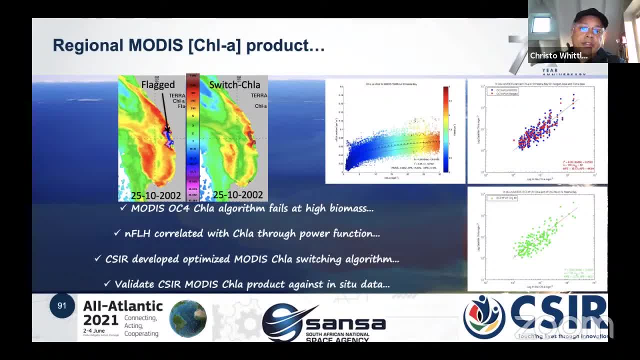 the gap and increase the time series inter�� cada inter��QUE interервQ inter��QUE inter �� the forest and chlorophyll values or power functions at higher chlorophyll values. Our research group derived chlorophyll A from the MODIS fluorescence linite product using a power function and used the result 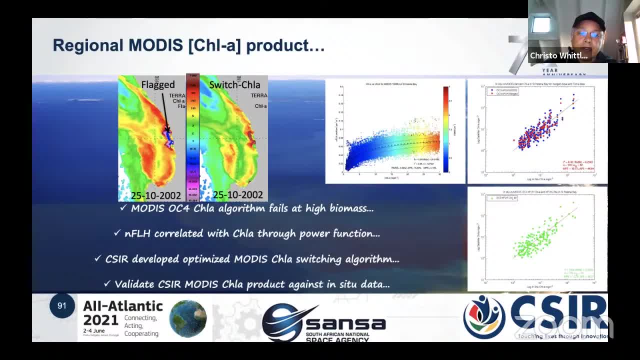 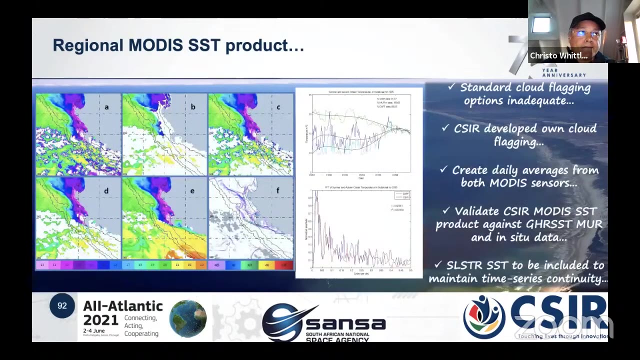 to develop a switching algorithm for MODIS to accurately track high biomass values associated with HABS. This optimized MODIS chlorophyll A product showed increased pixel retrieval and an improved correlation with higher biomass values in comparison to the OC4 algorithm when validated against in-situ data. Next slide, please Just one minute. Since active upwelling and subsequent 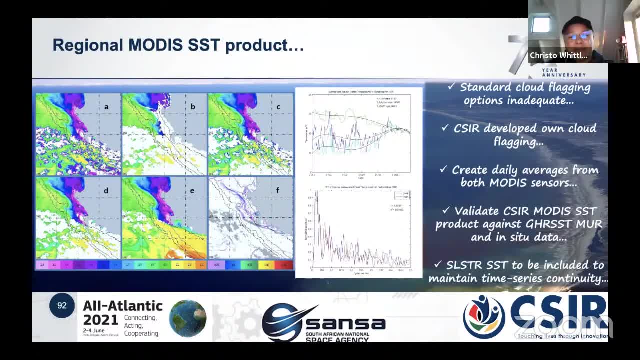 periods are precursors to HABS development. we want to be able to accurately monitor SST and available satellite winds. Standard cloud flagging options for MODIS SST either removes too many valid pixels or retains the pixels represented. We developed an SST cloud flagging procedure that reduces the impact of cloud edge pixels on single 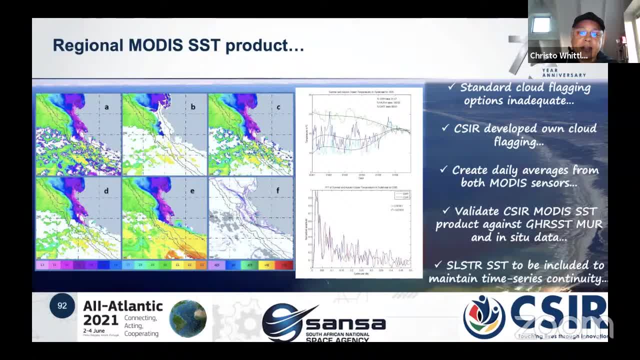 overpasses and further reduce cloud influence by generating daily averages of the cloud single overpass scenes from both MODIS sensors, using daytime and nighttime data. The final product retains more SST pixels and accurately represents the physical phenomena in the southern best BCLME, while retaining the strong gradients associated with the edge of upwelling plumes. 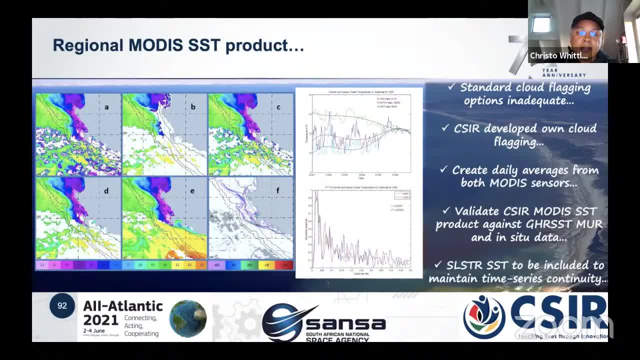 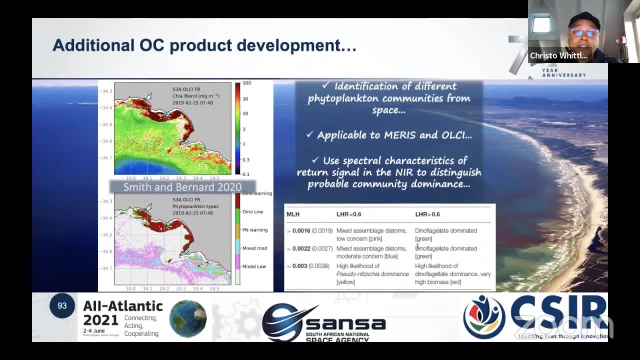 and the good object current. This optimized SST was validated against the CURST MUR v4 SST product and in-situ data. Next slide, please. Once we have identified the presence of a bloom, it would be useful to determine the level of threat. 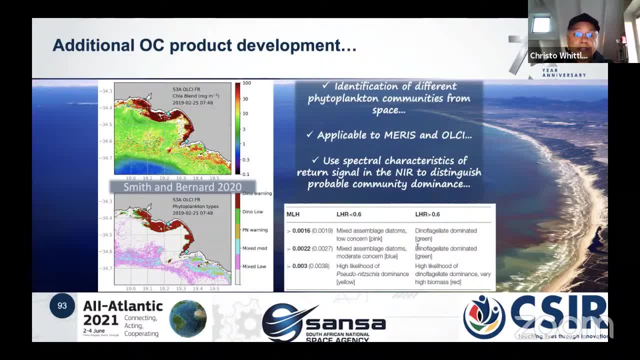 pose. To that end, a recently published algorithm presents the possibility for the identification of different phytoplankton communities from space using the spectral characteristics of the recorded signal in the near-environment. This is an example of the presence of a bloom in the lower part of the. 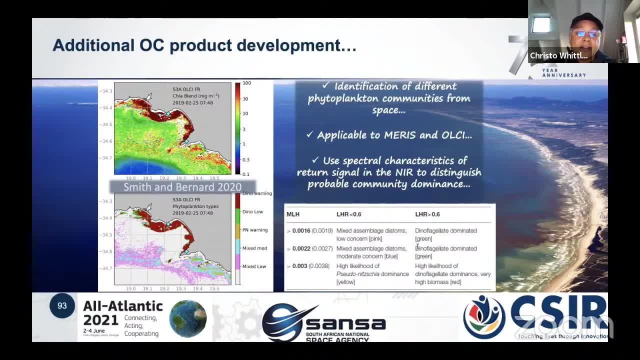 infrared to distinguish probable community dominance. The CSR algorithms described in this talk reduce spatial temporal error associated with limitations inheriting earth observation algorithms that were not intended for detecting the extremes associated with the southern Vecrila large marine ecosystem. Thank you for your attention. 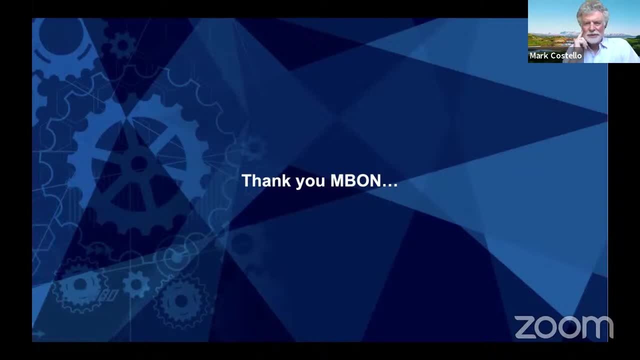 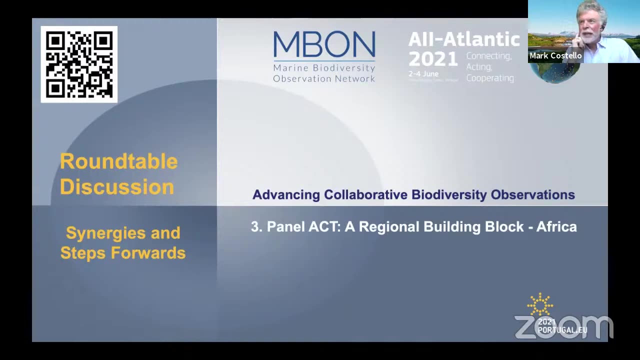 Thank you very much, Christo, and thank you all the speakers for very clear and nice short talks. It's hard to give a good five-minute talk when we have so much to speak about. I noticed that there's a couple of questions for Tatiana about the waste from. 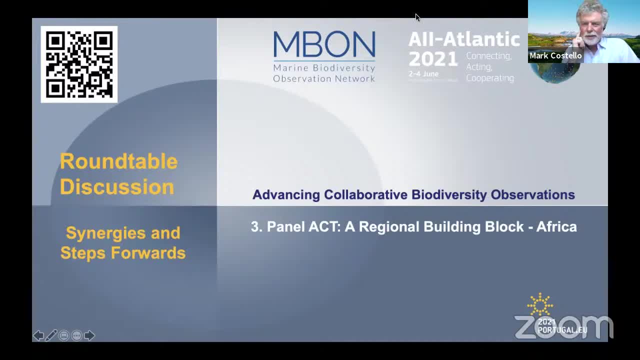 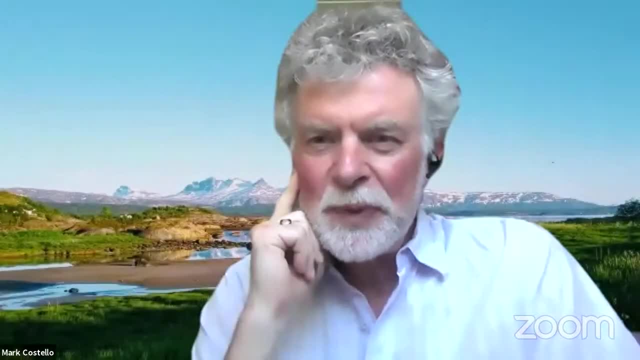 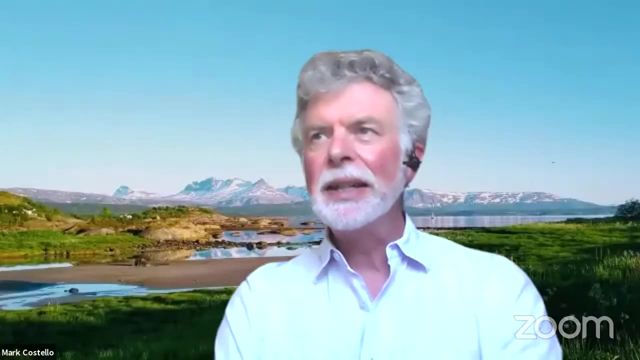 the shrimp farm and if they're considering to grow algae in it, seaweeds in particular? We have some Isabelle likes seaweeds, so maybe Tatiana would like to speak to multi-trophic aquaculture, if you're considering it. And then there's a second question from 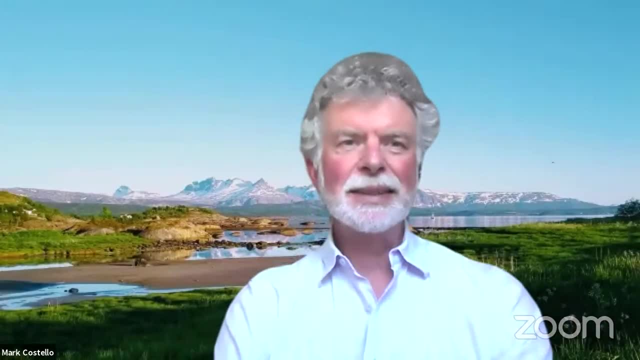 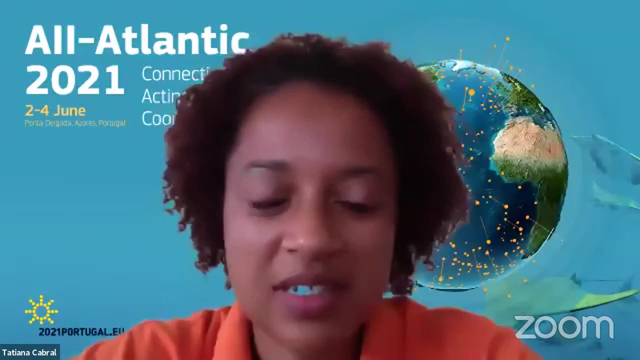 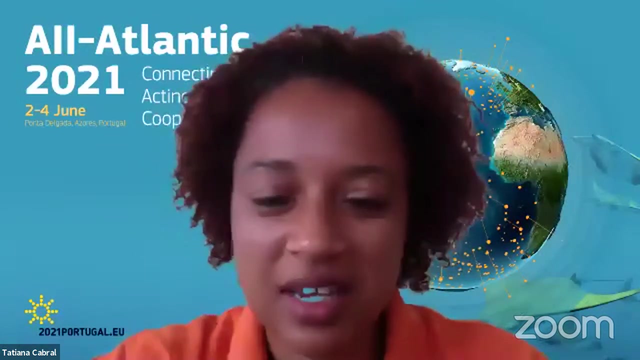 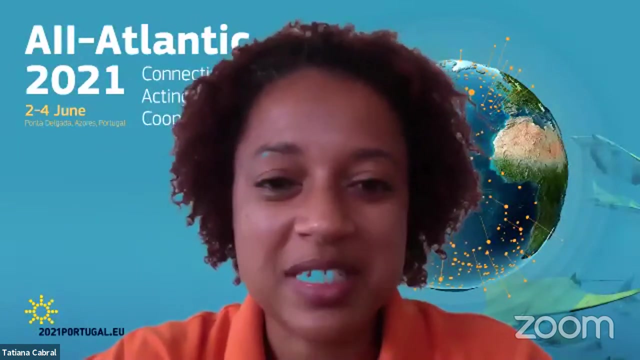 Daniel, I'll get back to as well after this. So about the waste? What we do is we have a sedimentation lagoon where all the wastewater goes to, and then it's treated, and in order for us to release it in the sea, it has to be in the same parameters, except for the salinity, that will be high. 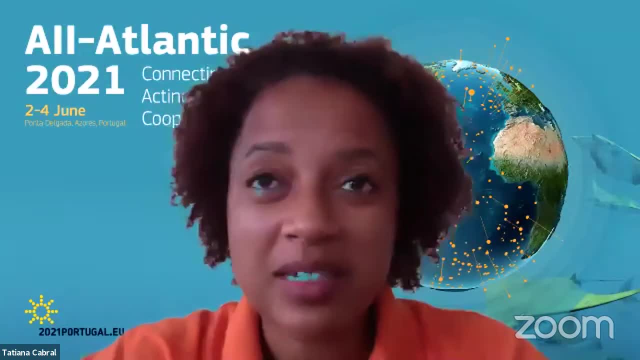 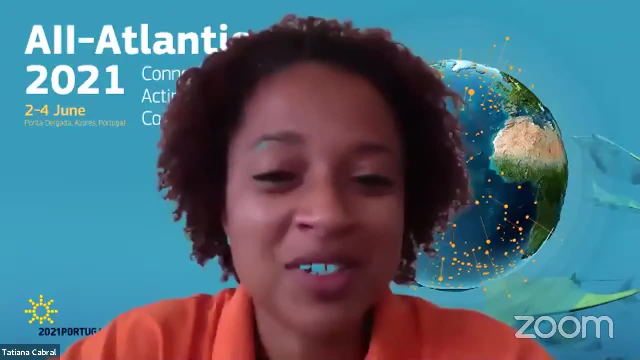 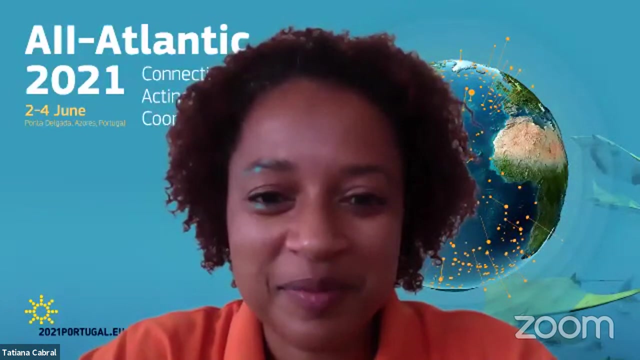 And in terms of of the seaweed, it's something we haven't thought about yet there, but there's still- like I said, we are still new- and there's a lot of projects that could be done together and lots of studies. great thanks, Tatiana. Isabel is dying to talk about seaweeds. I know she. 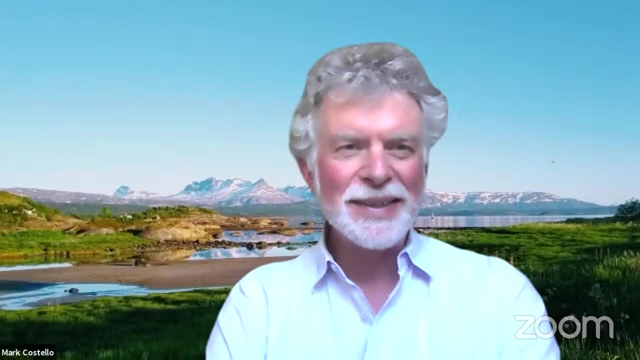 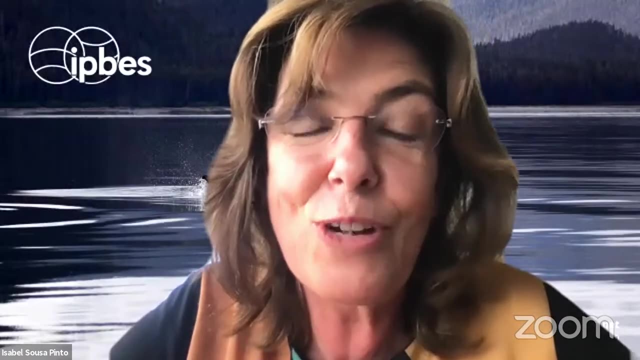 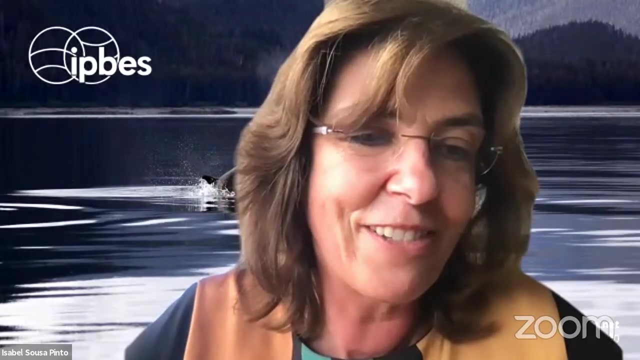 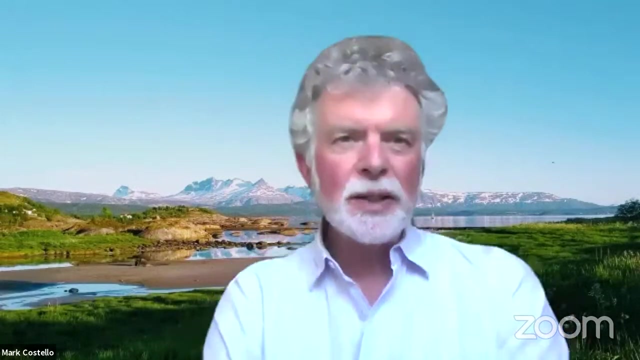 she has her hand up so I better let her speak on seaweed. no, just to say that you are really throwing away a lot of resources because you know with that you can really get a lot of biomass. I talk then: yeah, thank you. Daniel raised an interesting question which has been partly 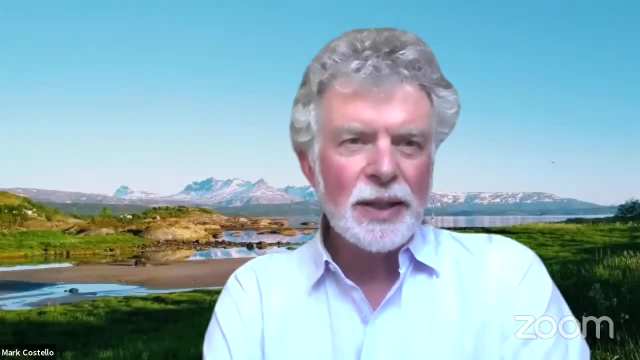 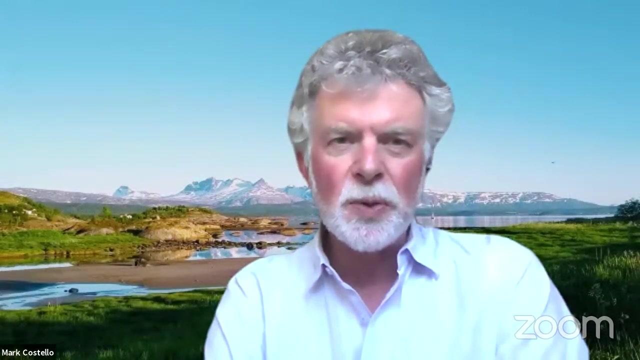 addressed but I think is core to these problems is how do we get data out more quickly, how do we collect data more efficiently and make it available more quickly? and this is really at the heart of the big issue that MBON is trying to solve. Frank has shown graphs of five more years delay before data. 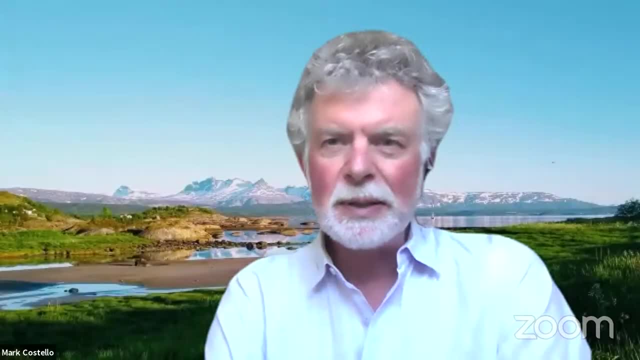 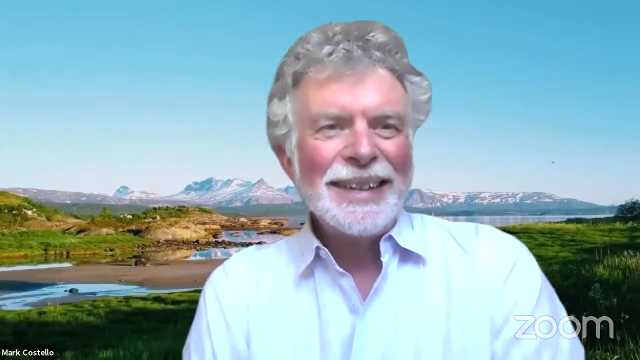 gets into OBIS and the scientists were not very good at this. the citizen scientists are perhaps much better, but if anybody wants to put a hand up as to possible solutions- how we accelerate timely publication of data and collection, Frank, you have an answer. I have more questions than answers, but I think that this 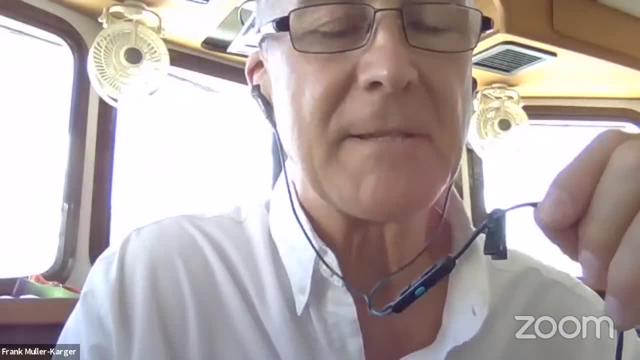 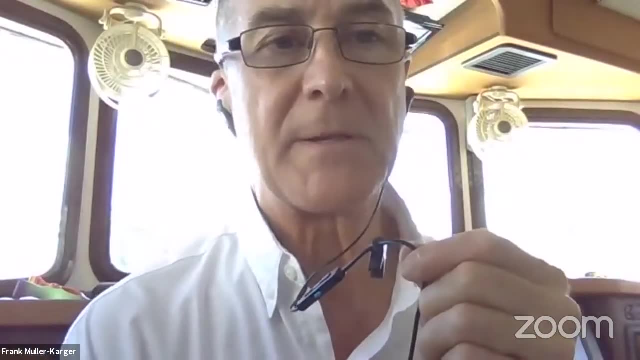 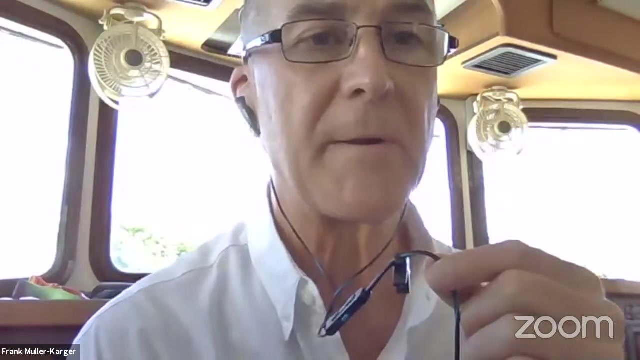 is something that we can learn. so it's not all scientists that are that are causing this delay in the delivery of data, for example, meteorologists, you know. they listen to society's needs and they said: well, we need to find a way to harmonize data, put it out and, in a GTS stream, share it around the. 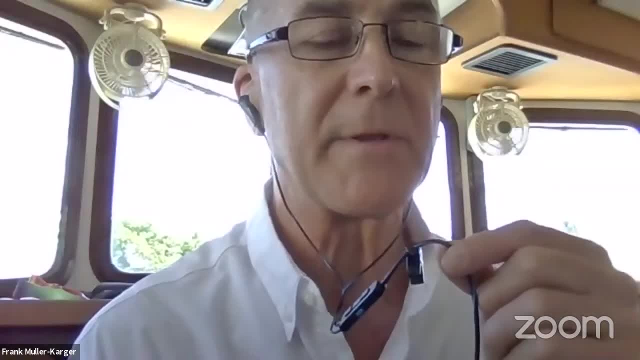 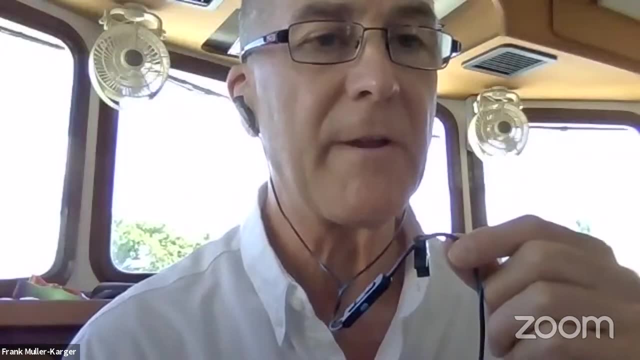 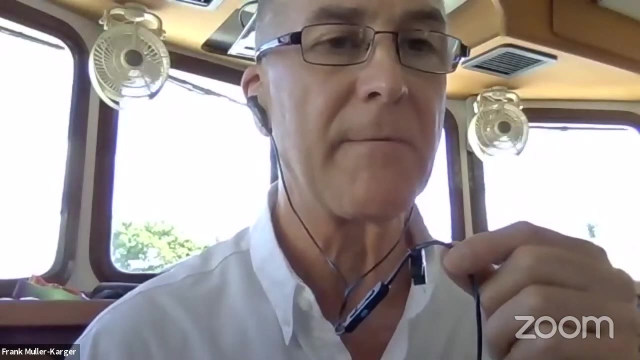 world, and everybody agreed that there's some key- not everything, but there's some key measurements like wind speed direction and wind speed direction and wind speed direction and wind speed direction, humidity, insulation. you know some very fundamental measurements that have to be shared so that you can forecast the weather, and so this is the kind of thing that we can learn from if the meteorologists 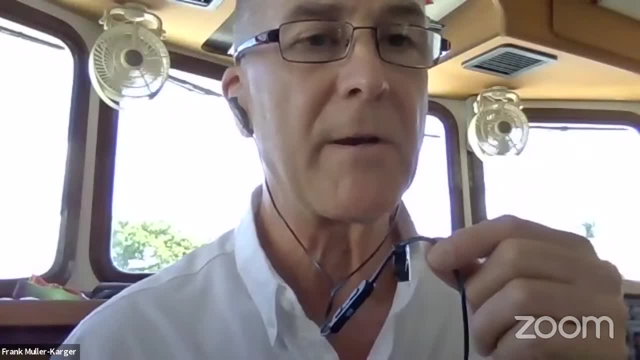 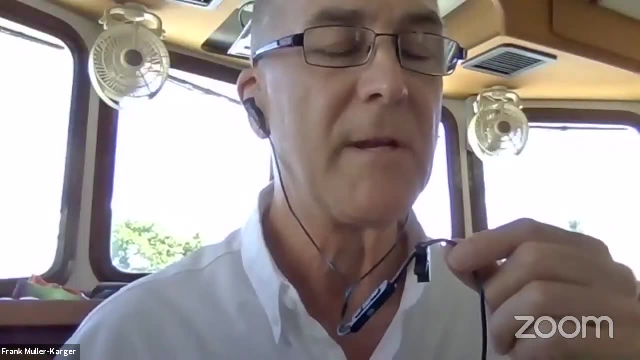 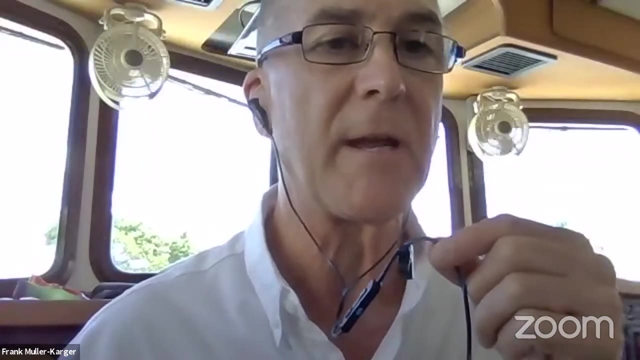 can do it, and they did it 50 years ago. why can't biologists do this? and so we have been very attached to our data. you know it cost money. students and principal investigators have to publish, and yet I think that the argument that we're making is that we don't need to share. 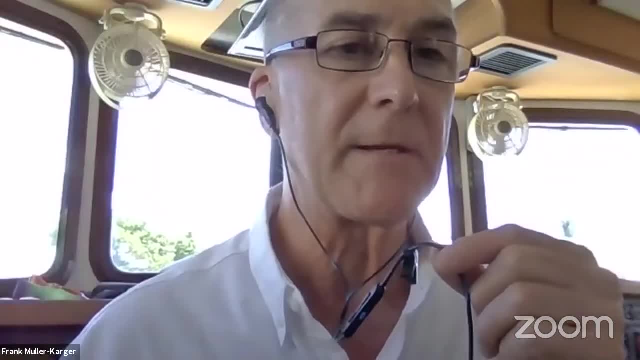 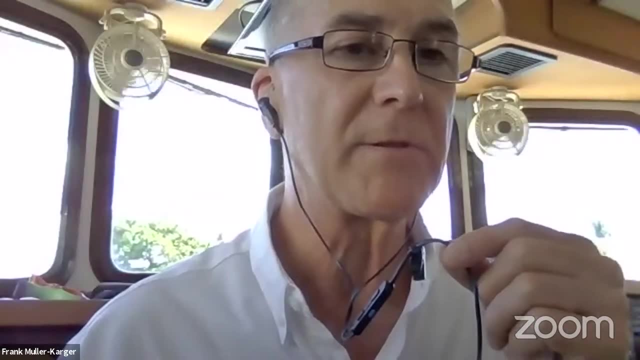 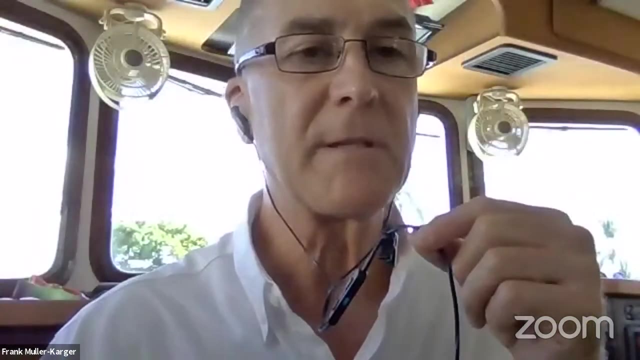 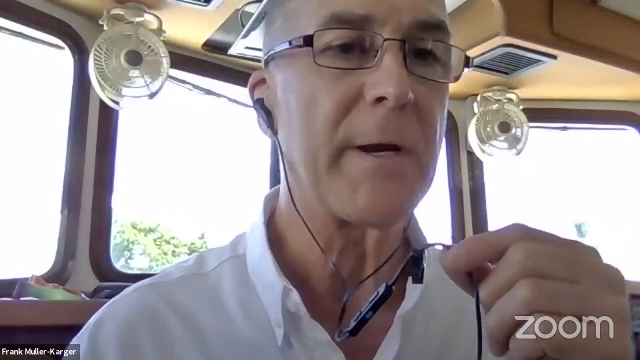 everything that we do, but there may be some fundamental observations that we can collect locally for our own investigations that complement everything else that we're doing that can inform society locally but also help us understand what is happening at a global scale. and that's the key is: how do we get to that point where we can agree? what is it that we can measure together about? 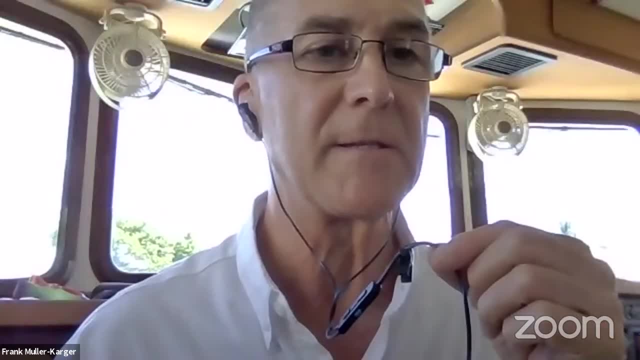 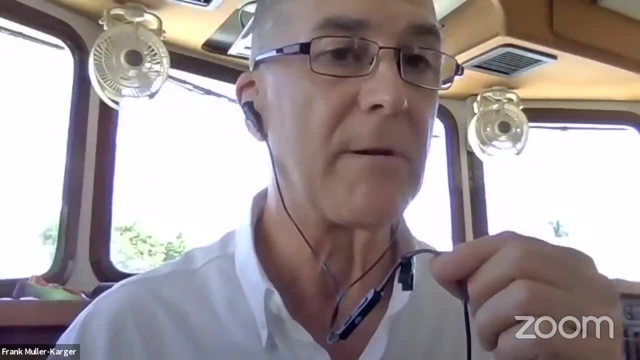 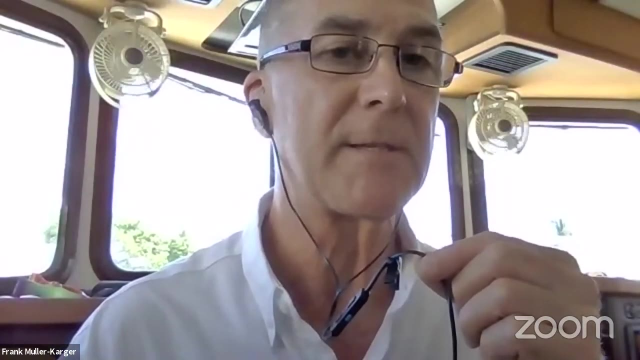 biology, so we can understand how the life of the sea is changing, and that's that's not a simple question, and we have to overcome a cultural, uh- obstacle also in how we share the information. so there's no question about that, but that's what we would like to accomplish during this decade. that's right, Frank. so other people have done it. 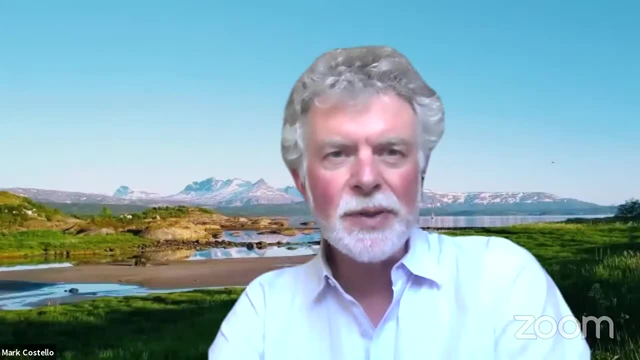 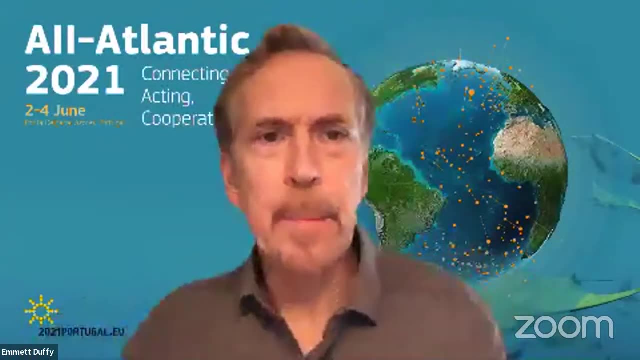 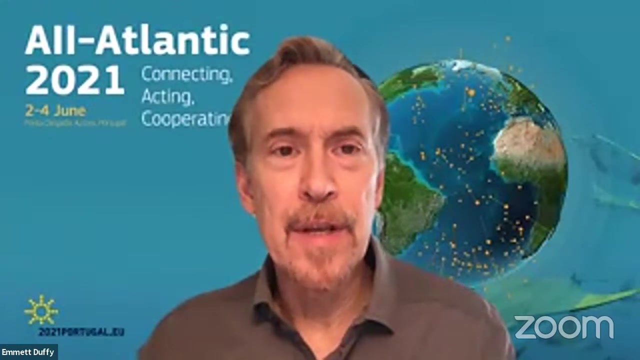 so why can't we as biologists- and I think Emmett and then Murray have some responses. Emmett, yes, uh, I think Frank made made good points. I I would add two things about that time scale. one which is in some ways the elephant in the room here, that we 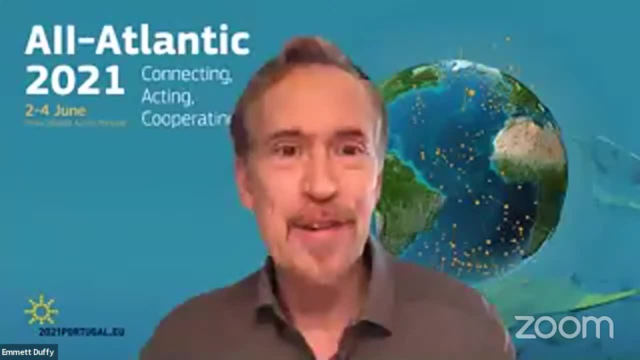 haven't mentioned yet is that biodiversity is hard. it's a lot harder than temperature. um, generally speaking, it requires, uh, you know, intensive sort of human um uh, knowledge, uh, as opposed to simply being able to measure it with an instrument. we hope that that will change with time. there's a lot of progress in that direction, but that that's one of. 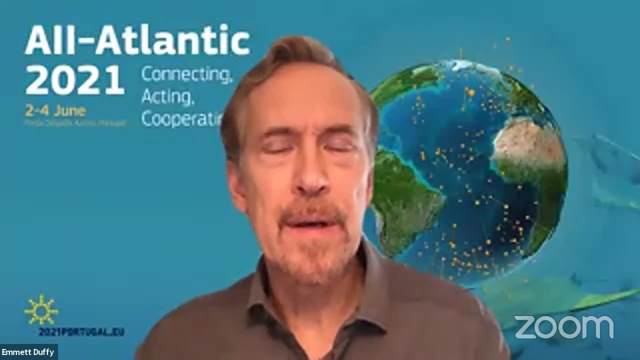 the things that I will move it the. the second point- I think that that speaks to to what Frank was saying also- is that, because of the fact that there's so much human effort in doing this, I think there has to be a strong emphasis on incentives to data providers for providing the data. you know what? 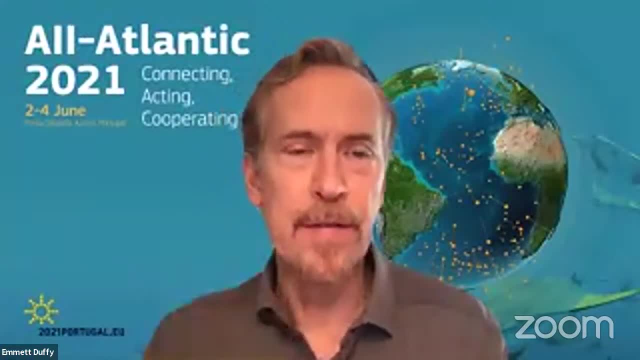 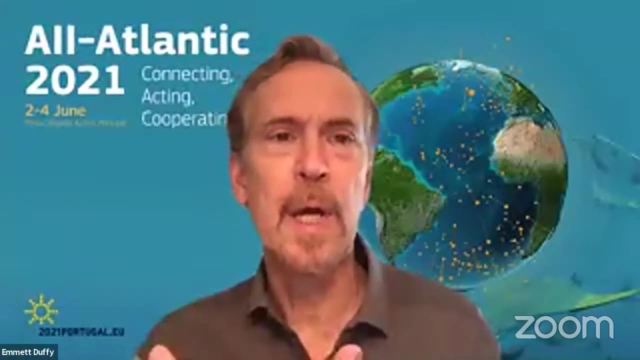 what do you get out of this? for putting your data into a system and you know, in Smithsonian Rangio we are primarily working with other scientists who are interested in in publications and that that's a strong and attentive but of course that won't work for. 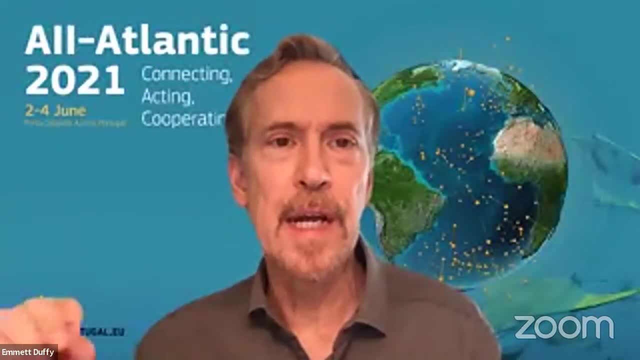 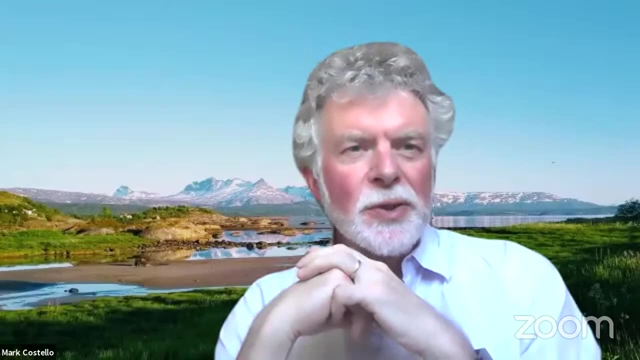 all of these kind of situations. so I think that just thinking about the incentives to data providers is going to be an important aspect of this. I I have wondered about that, Emma. I used to say that. but if we look at Citizen scientists, who expect their data to be made freely available, and our 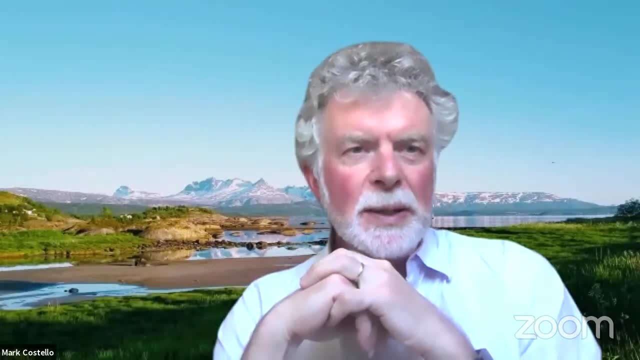 naturalist does this every month so, and they're doing it for free. so why can't scientists who've been paid by the tax pair be obliged to make their data free if we sit down here and report a similar obliged to make their data free available a bit more promptly? It's a little bit, I wonder what. 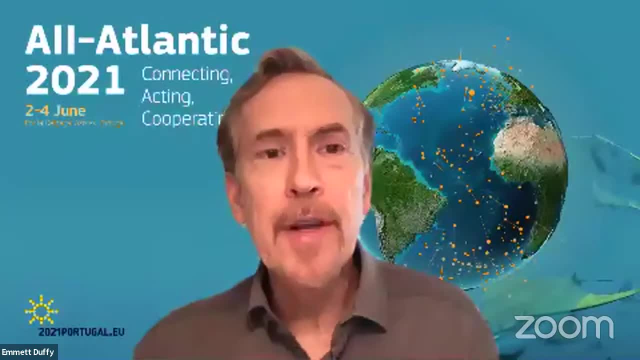 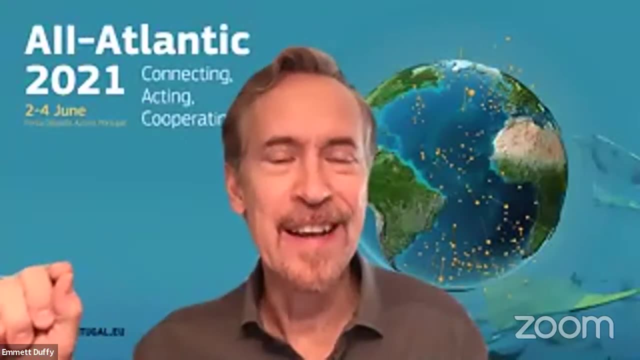 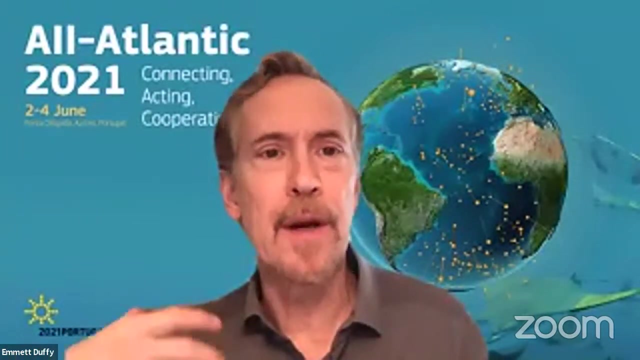 the public would say about this, Mark. I actually think that is a strong example of what I was talking about. There is an incentive on iNaturalist because you get immediate gratification. you know oftentimes very rapid, you know interaction with the community. There are a 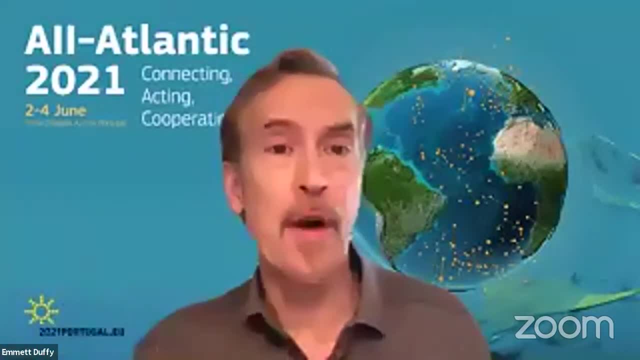 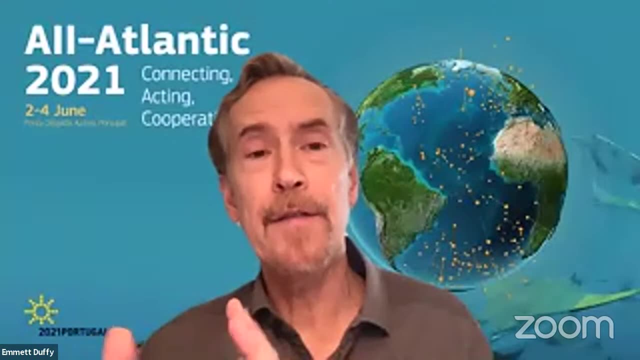 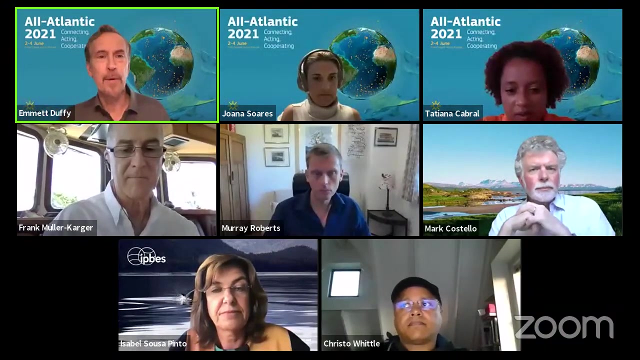 lot of people that look at it and can help you identify things. There's an artificial intelligence algorithm that can identify species. So I think that you know to the you know if that kind of approach could be incorporated in some way, you know, into marine biodiversity. 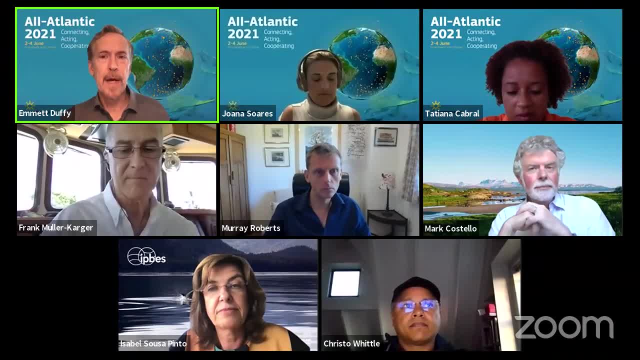 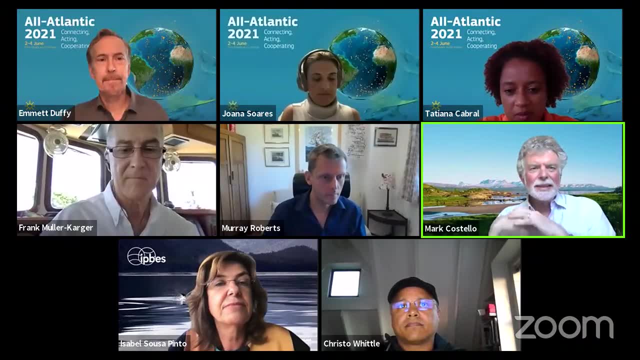 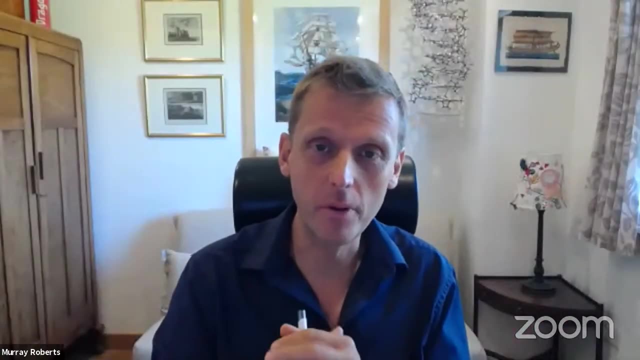 observing generally. that would make a significant difference, I think. Good Thanks, Marty. Thank you, Mark. Yeah, I was kind of going to speak to the point around the scale of the problem and accessing data from different sources, And I'm thinking in particular. 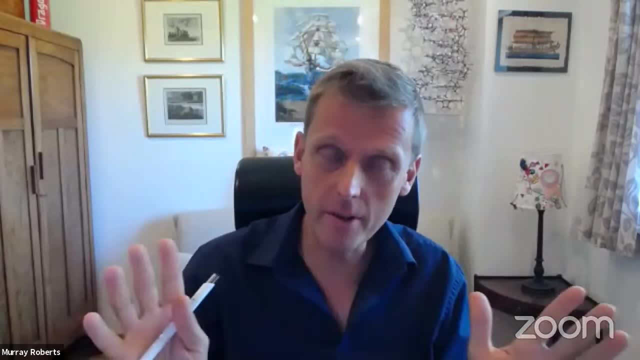 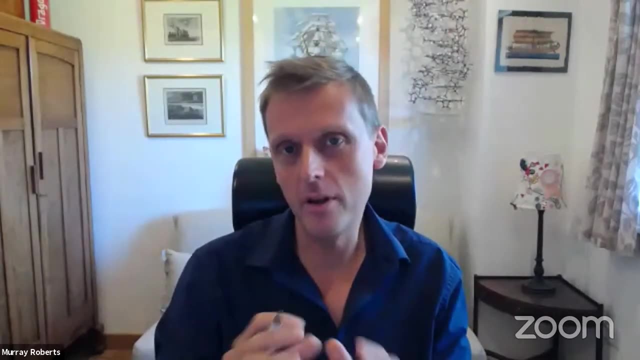 here actually of industrial data sets which are often off limits to academic science. They're hidden behind many layers of confidentiality and non-disclosure And I think typically we ignore them, We don't go for them. We're aware of them, but it's just too hard to get there. 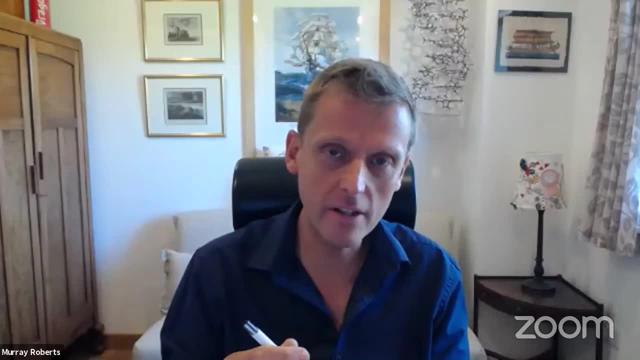 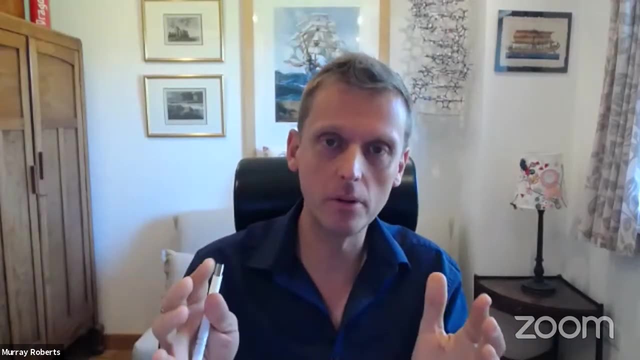 So in iAtlantic and other projects we've really worked at that really hard and developed the partnerships that have opened those repositories. And that takes a lot of time, It's an effort, but they're incredible, They're to a very high standard, They're major, as we know. 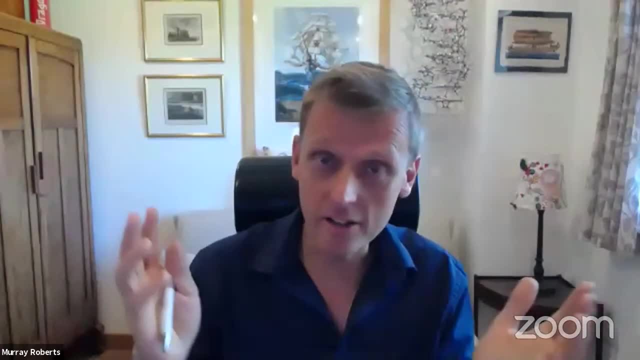 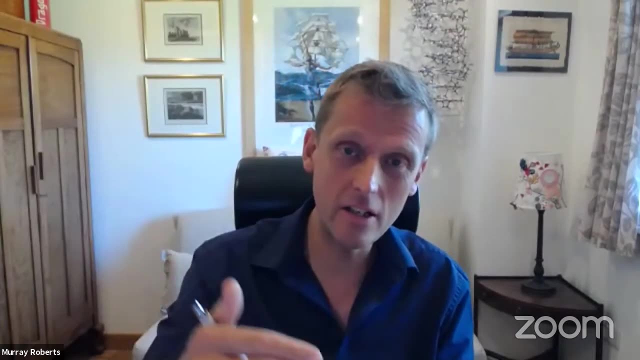 major, major industries working in the deep and open ocean, in the Atlantic and elsewhere, And they have incredibly high quality data sets, including biodiversity data sets. They're at the leading edge of eDNA testing and implementation in the field And, in fact, often these data are. 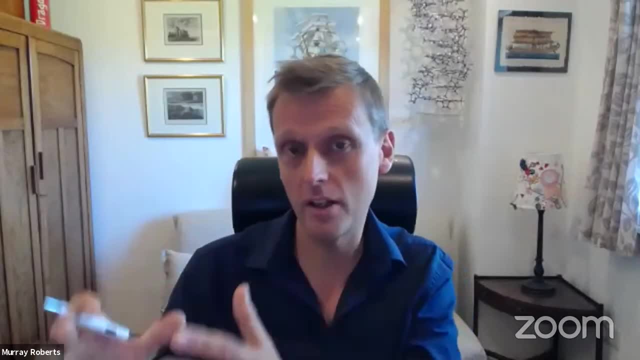 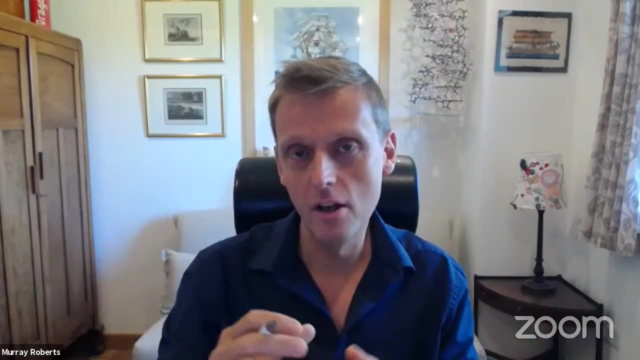 not very commercially confidential, And with the right negotiation and discussion we can access these. It's only going to increase when we look at the upscaling of renewable energy, for instance, This marine sprawl, this industrialization of large areas of marine. 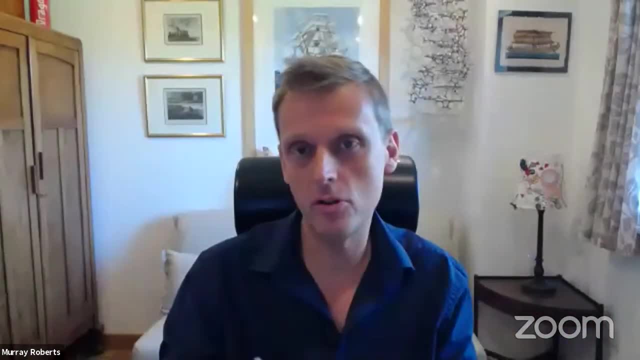 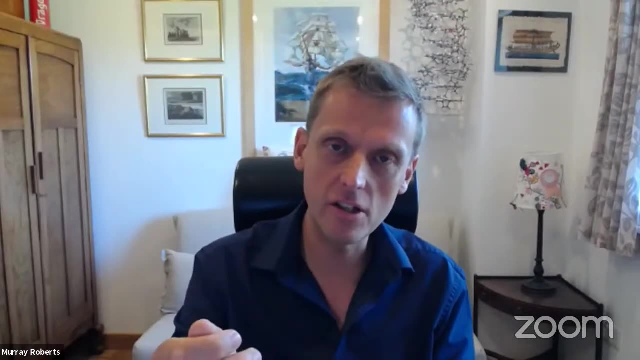 space. whether we like it or not, it is happening And there are huge opportunities around that, But it does mean engaging right at the coalface with those sectors. From iAtlantic, we've just secured a data set that Brazilian partners have been trying to access for maybe five to 10 years. 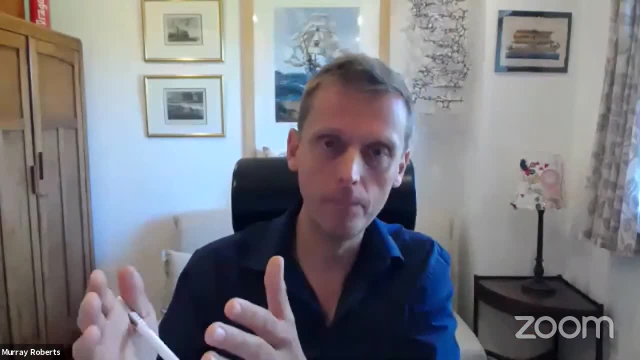 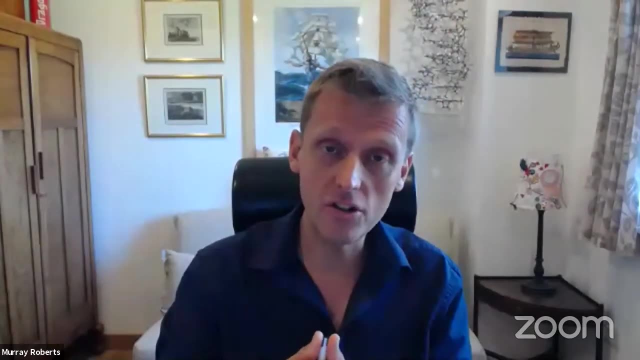 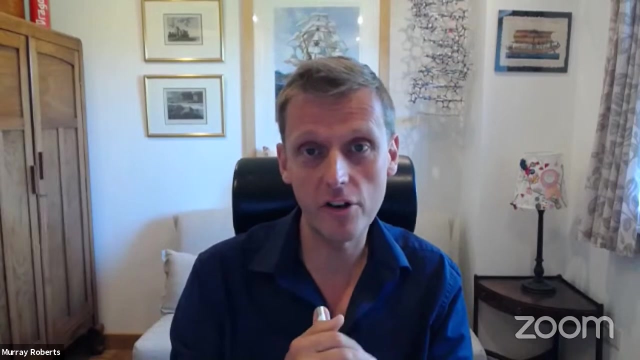 But the convening power and application through global industry bodies allowed access for the other Brazilian partners to these data sets, including very commercially interesting data sets- multi-beam bathymetry included alongside species data as well. So I think that's a kind of key opportunity for us as a community to look at really seriously. 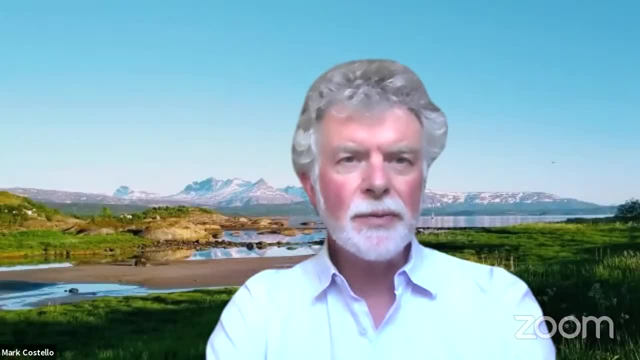 That's a very good point, Murray. It's often it's good to talk to industry. I've discovered that industry are really pleased if somebody wants to publish their data and make it available, because it gives them actually visibility and shows they're being a good citizen. So that's a very good idea. 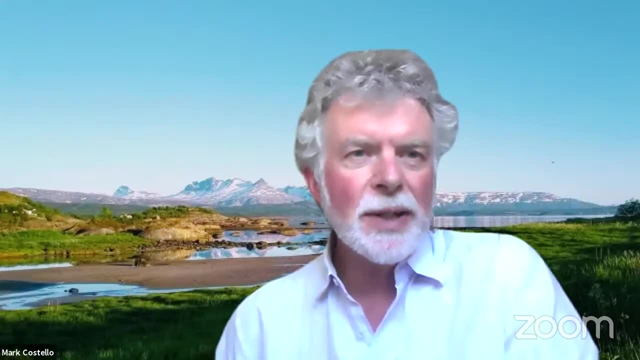 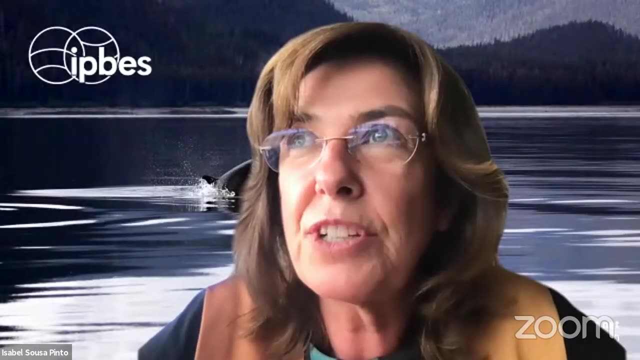 You need to talk to the industry. Isabel has her hand up, Isabel. Yeah, actually we are discussing this in IPPES and the data knowledge task force And we are creating the system that can really identify how many times your data, your data. 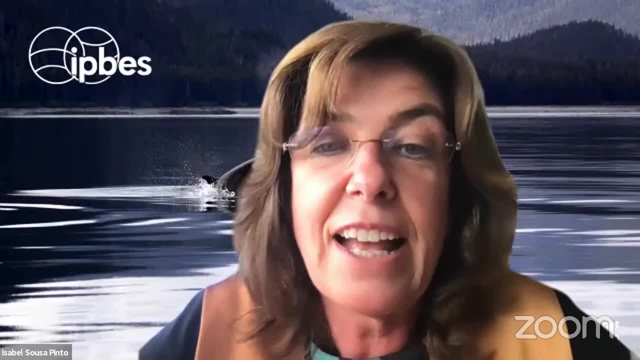 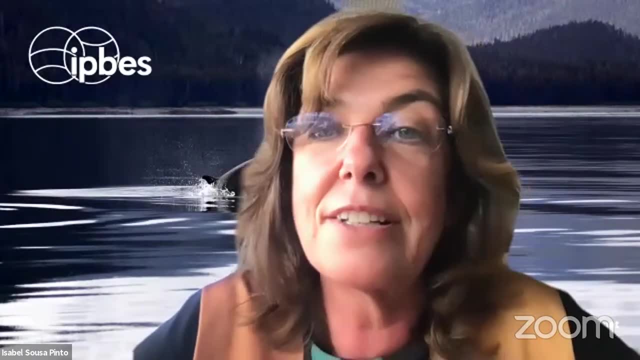 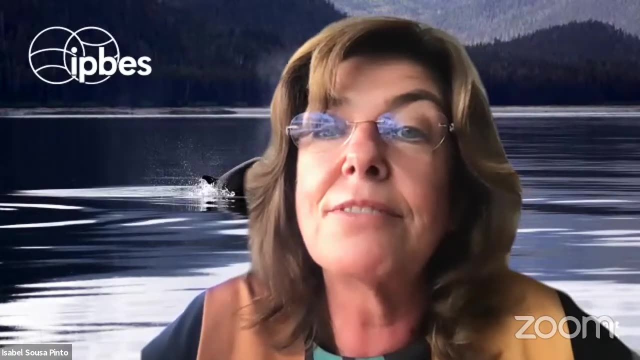 has been used, for instance, in IPPES reports, And I think if we can really manage to have a system like this, this could be really something that scientists appreciate and could really show the impact of their data, of their data sets, on important reports. 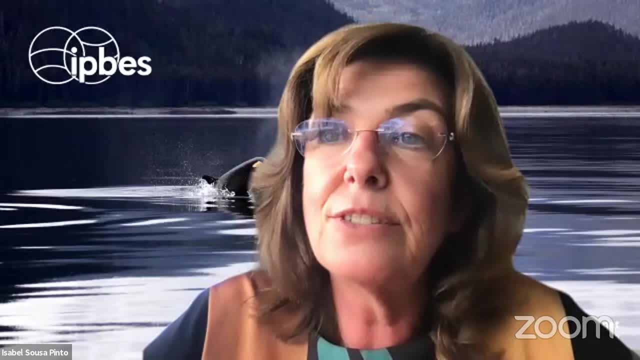 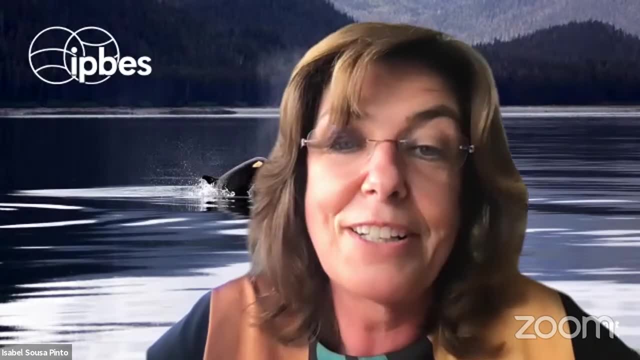 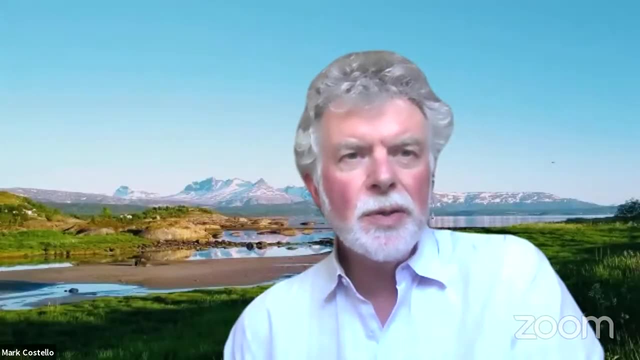 And I think this is I really believe we need to work on the reward system for making these data available, because it's still a lot of work to do this. Yeah, and GBIF and DOBIS have developed tools to do that, but I don't know if they've been followed through. 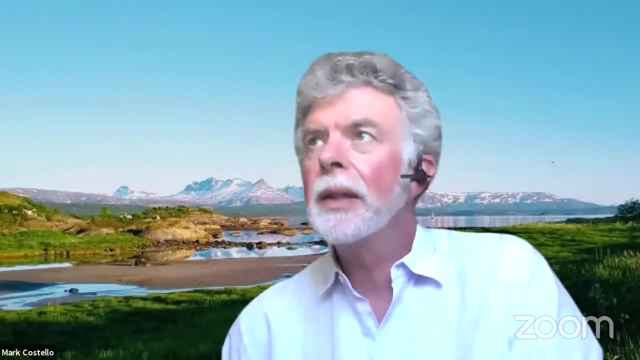 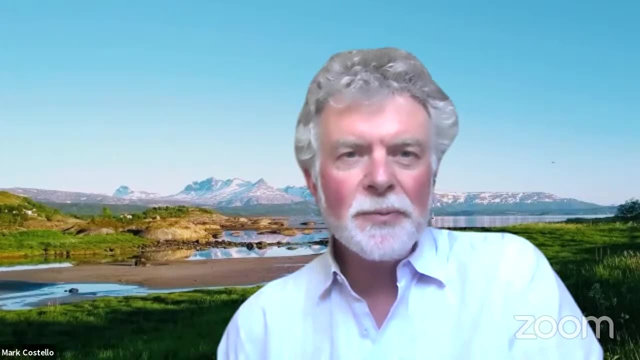 completely and made visible. it's a good point, And I noticed another unanswered question in the Q&A- which is of the many questions that hasn't been answered because it's very hard to answer- by Vahab, And he asks how to validate old biodiversity data. 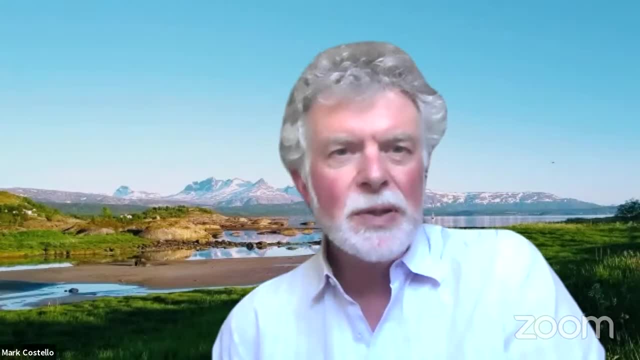 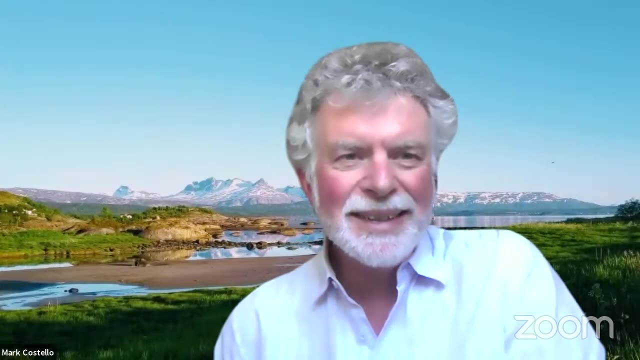 So the older data gets, how do you know is the species, what the species is now and these other issues? So I don't know if anybody has an answer to the problem with looking at old data, it's coordinates and these other issues. Is it a matter of being a marine detective? 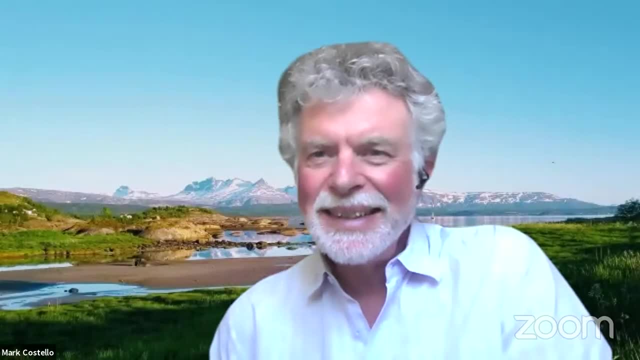 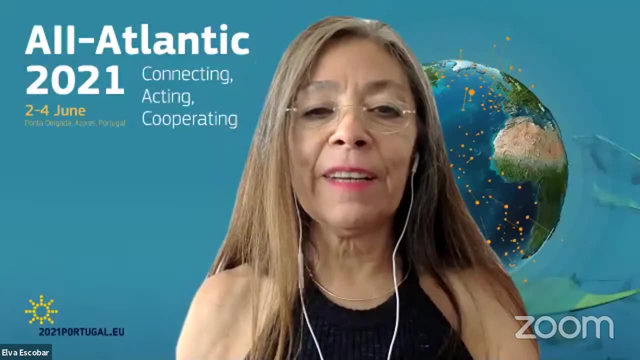 Yes, nobody can answer. Elba has an answer to it. Okay, Oh sorry, Isabel, you're speaking. No, no, no, no, You go first, Elba. Actually, I think it can compliment with whatever Isabel will say. 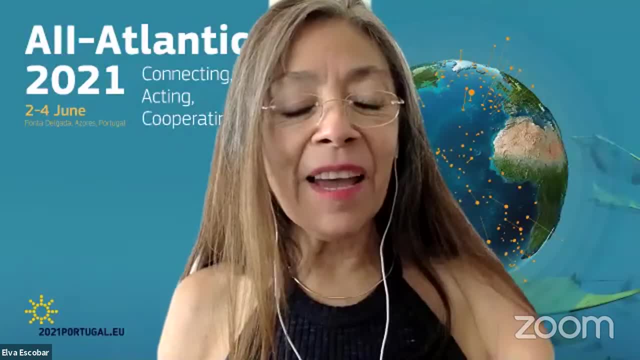 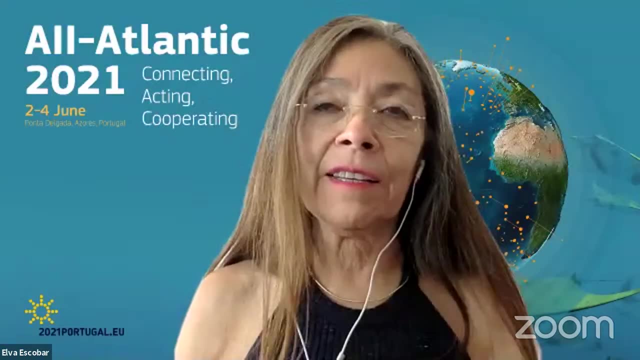 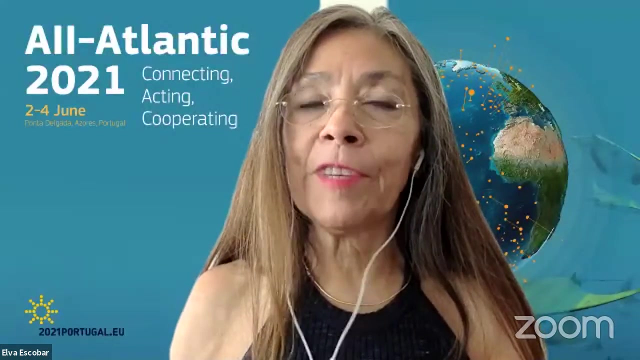 which will be probably more wiser than myself, And actually what I think is that we cannot consider that older data are wrong. They were done with a different technology, They were obtained with different initiatives and objectives in mind, but they are useful at the end. 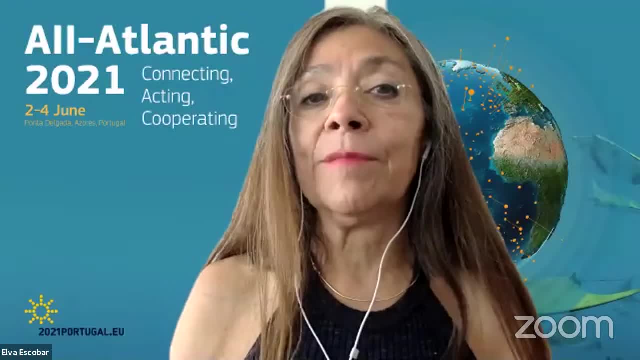 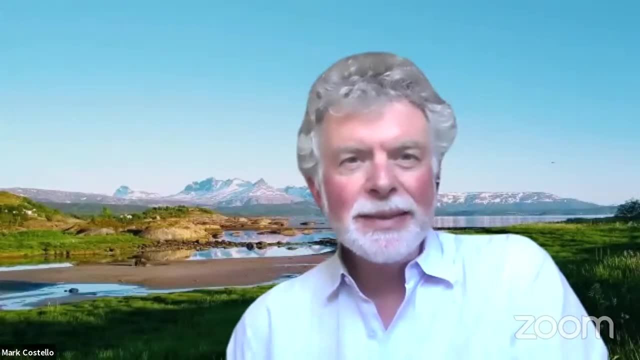 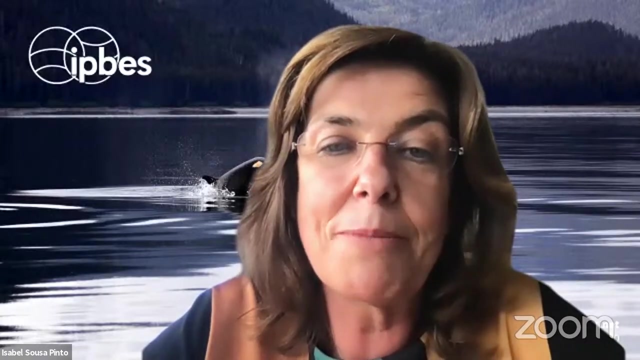 And if they were done with good practices then we can trust them. Yeah, The older I guess, the more I agree with that, Isabel. But I think I remember, for a sense of marine life they had a really interesting program of ocean. 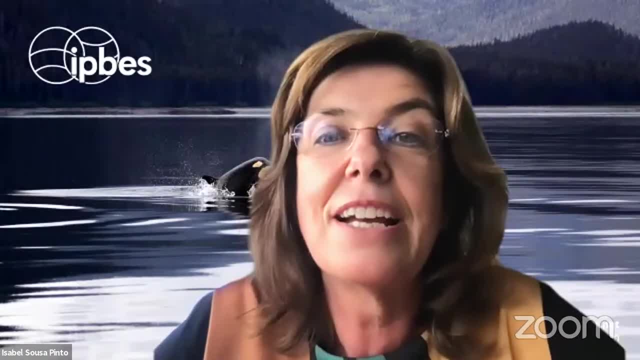 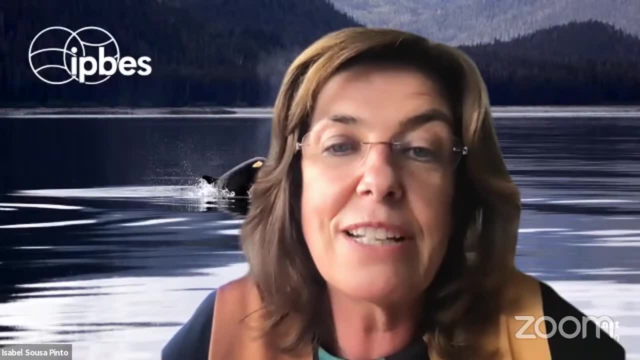 past or something like that that really went to documents. So I think, yeah, you need, for maybe you need some more work, really this detective work you're talking about- to really for some data that is not complete, but if it's worthwhile. 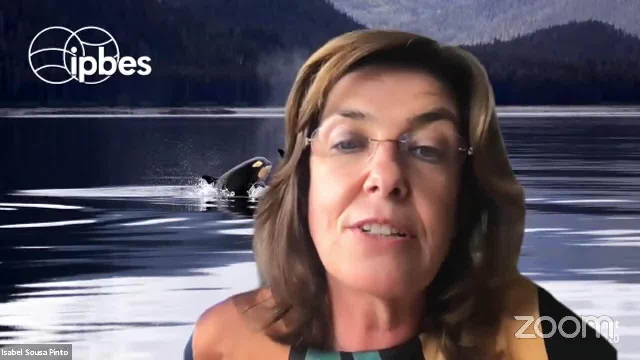 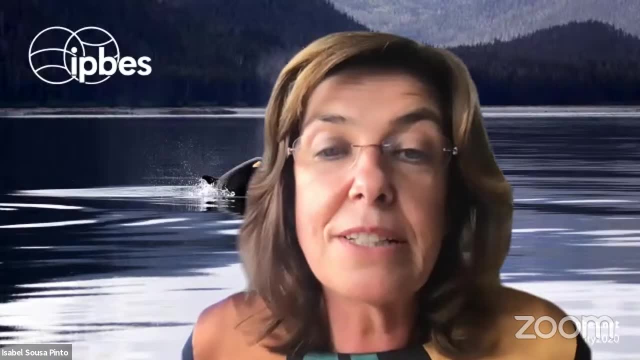 if it's from places where we really lack information or we want to have older data. I think this is very important: to try to use this data and really try to complete as much as possible what is missing. Of course, depth can be important. 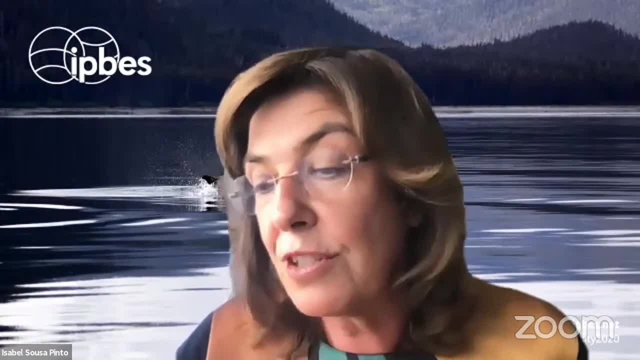 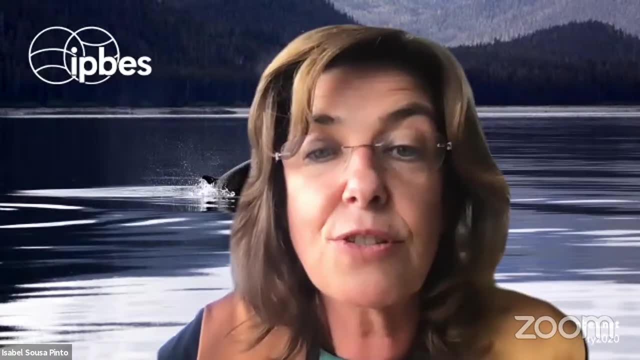 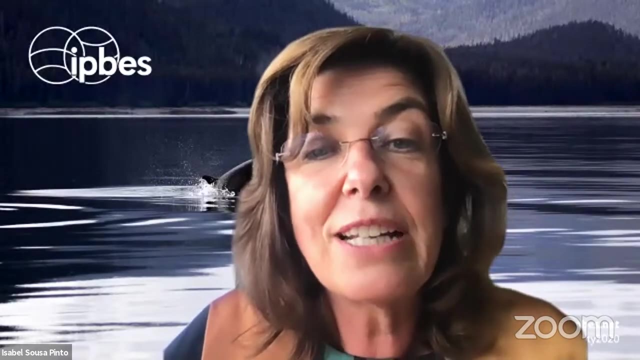 but try to really use, of course, more. do some work- And I was really. I think there was incredible results just going to old books and things like that- I mean this was really old, hundreds of years old- to really try to have data how marine life was then. 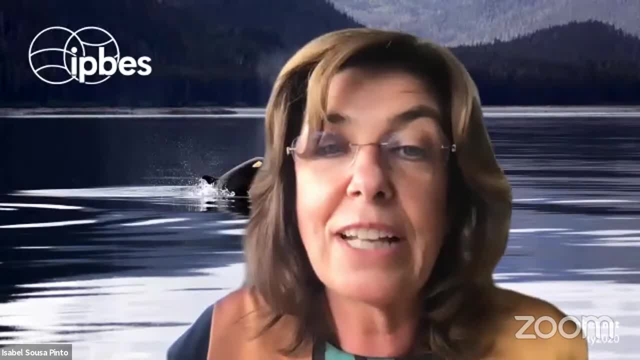 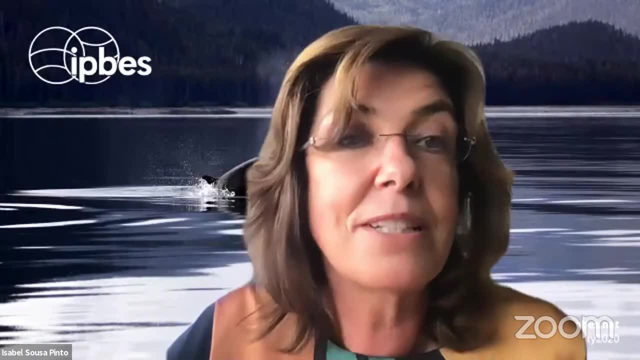 So I think if you could do that, we can also use older data, And that was not has not everything that we all the metadata that we would like to have but maybe still can use. Thanks, Isabel, Is that an old hand you have up, Murray? 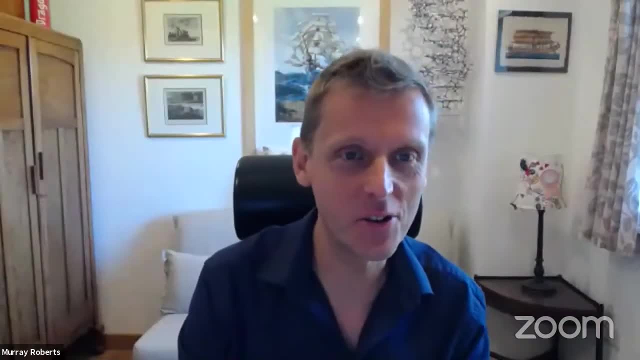 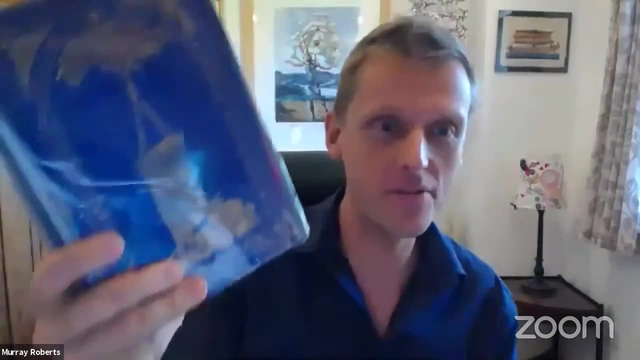 or is that a new hand? It's a new hand, but actually Mark Isabel has already trailed what I was going to say, So here's something I wanted to show you all, since we have cameras. This is the depths of the sea. 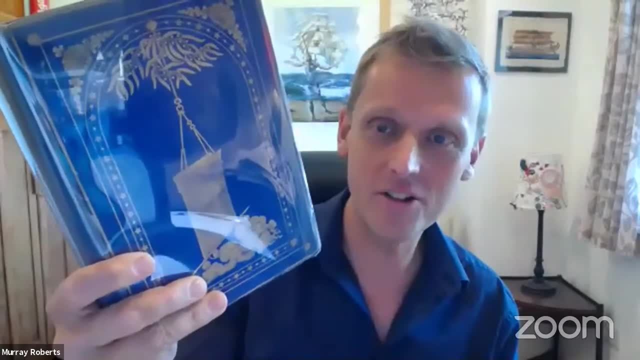 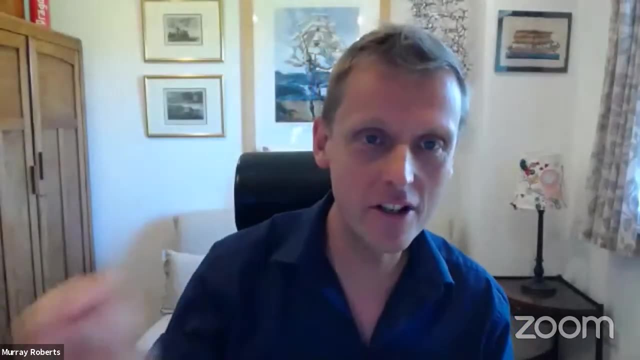 Who knows this book by Charles Wivel Thompson who led the Challenger expedition And he was a professor in Edinburgh? this is a fantastic book And in this book Wivel Thompson talks about stony copses of deep sea corals covering many miles between the Faroe Islands. 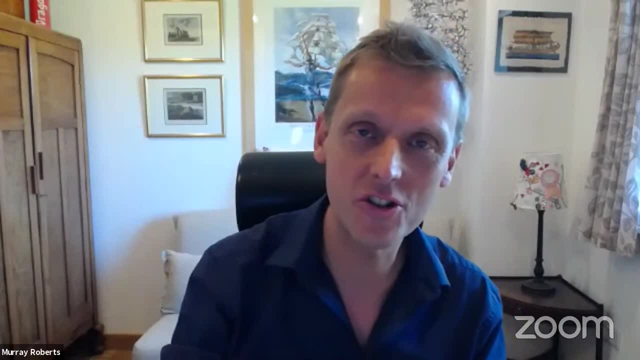 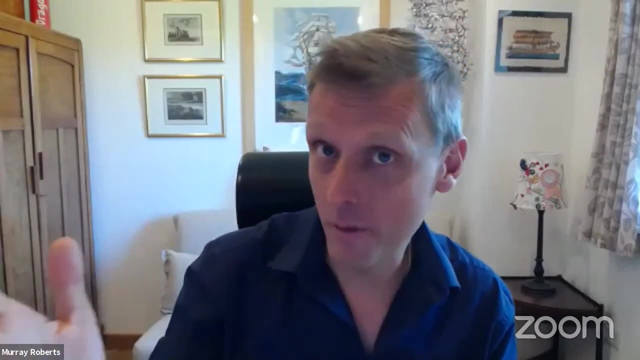 and the Shetland Islands. Well, I remember going there on my first research cruise in 1997.. We couldn't find those stony copses. They weren't there. They've all been trawled up, I would argue. 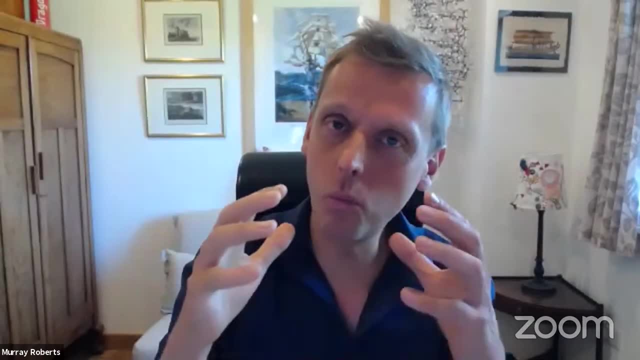 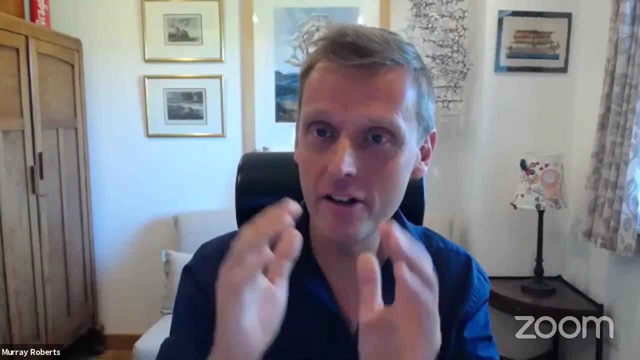 So this point that Isabel makes is absolutely right. It depends what we're trying to get. The old information is incredibly valuable, It gives us that context, but otherwise it's entirely lost, And there is a really nice discipline, of course, of historical ecologists that are busy pursuing that. 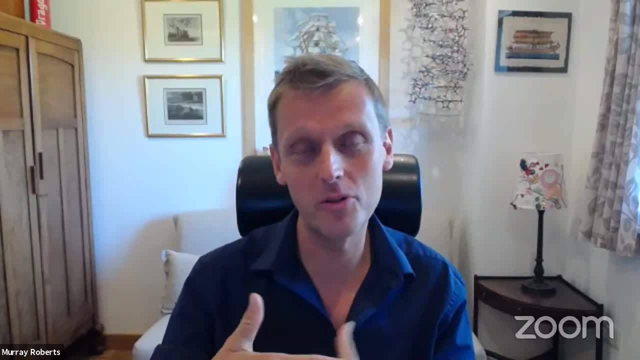 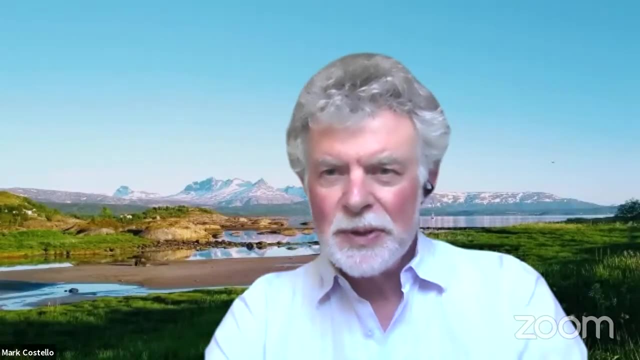 I think there's a lot more that can be done. I think it's absolutely fascinating and a huge opportunity. Thanks very much. We've just five minutes, so I'd like to give the floor to the people who haven't spoken. Yes, there's Brian Anthony Jordan, AJ Rui Alice. 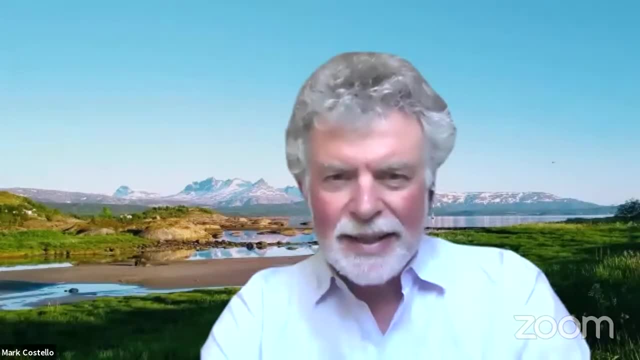 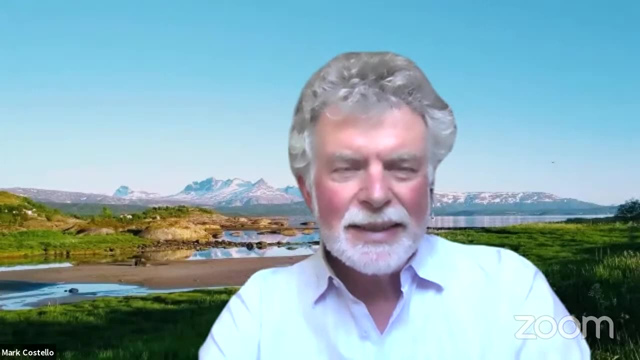 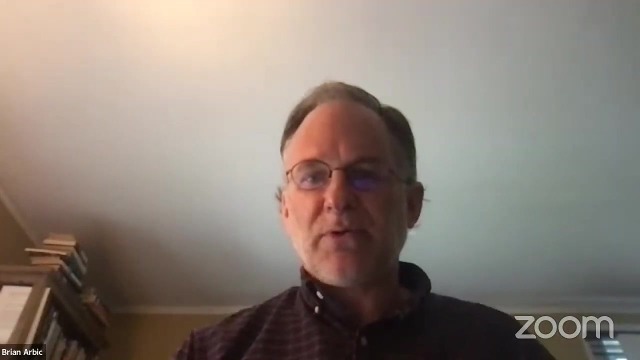 Oh no, Alice is supporting And, Katerina, if there's any comments you want to make on the session. so far, I mean, I'll just say again, I think we all agree, capacity development is really important. I think someone- I don't know if it's from the audience- 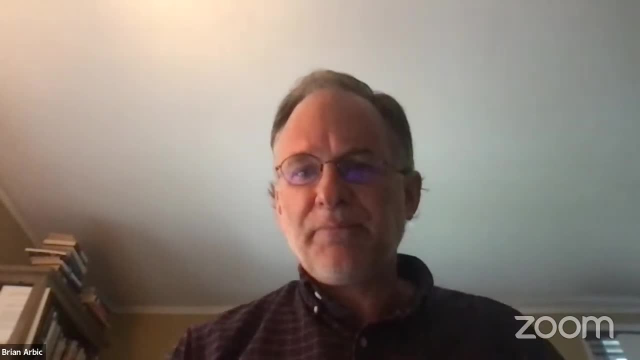 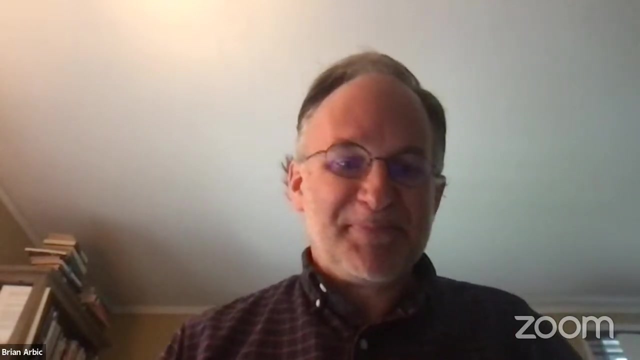 or the panel pointed out that human resources in under-resourced nations there just aren't many oceanographers. So I just think it's really important to increase the number of oceanographers in places like Africa and elsewhere, not just Africa. So I think everyone would probably agree with that right. 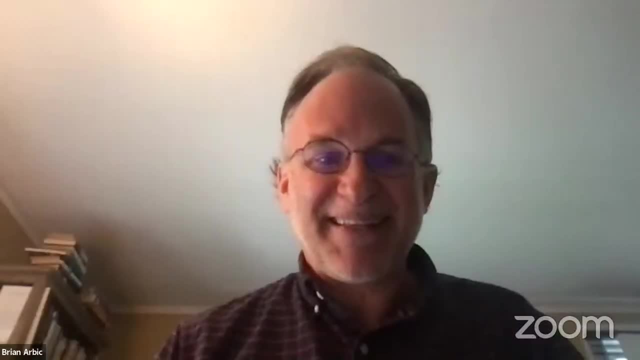 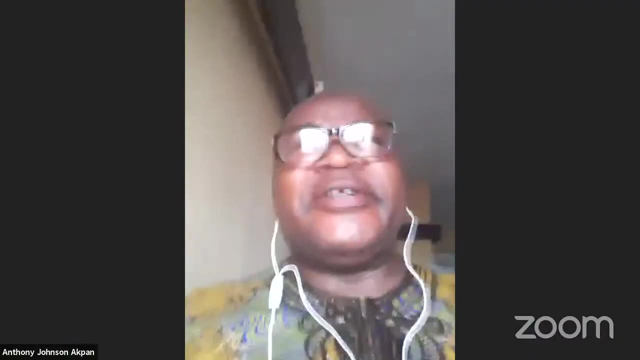 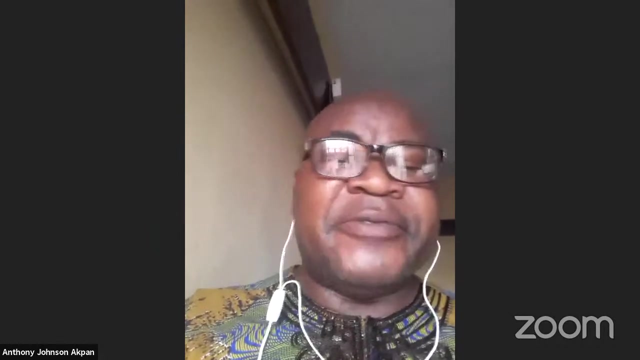 You must be an oceanographer. Yeah, Can I come in, Anthony? sorry, Yeah, I mean just like you said. I mean you cannot over-encise the importance of people to understand their impact on the ocean and our impact on the ocean and what the ocean means to it. 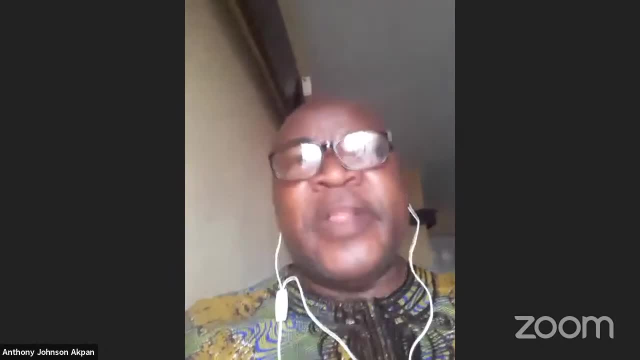 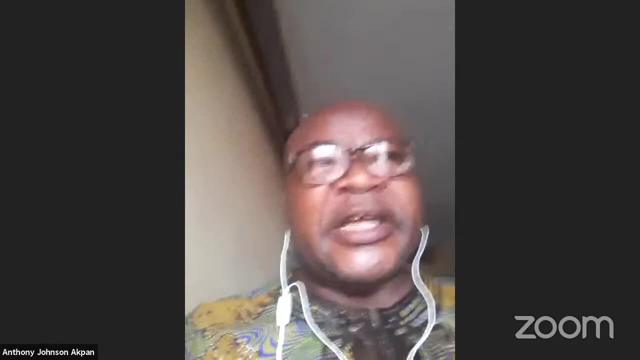 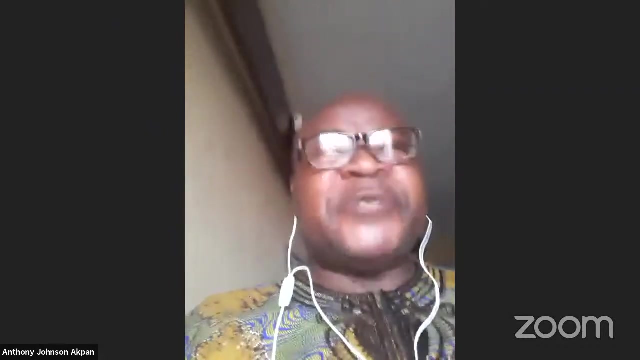 So, particularly like I mentioned in my presentation, Africa is really backward in ocean-related science and understanding and some of these efforts we are trying to do is to boost this capacity and all of that. So we really call on various existing projects that have experience to really support us and to enable us. 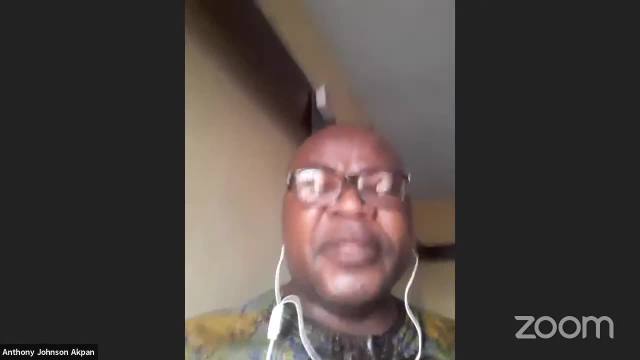 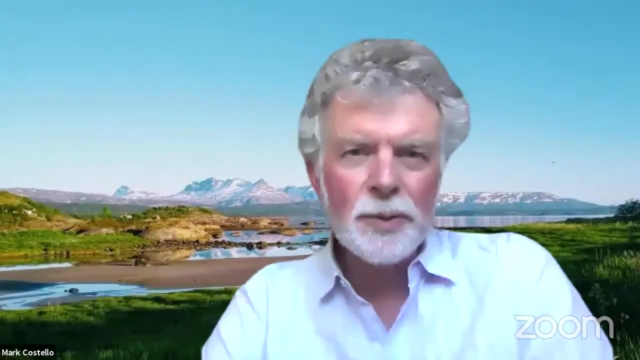 to put this proposed action at the implementation. Thank you, Yeah, it's fundamental because in my parents' generation in Ireland, where I grew up, they never did marine science. Yeah, Yeah, Yeah, Yeah, Yeah, I mean the question of marine science in school. 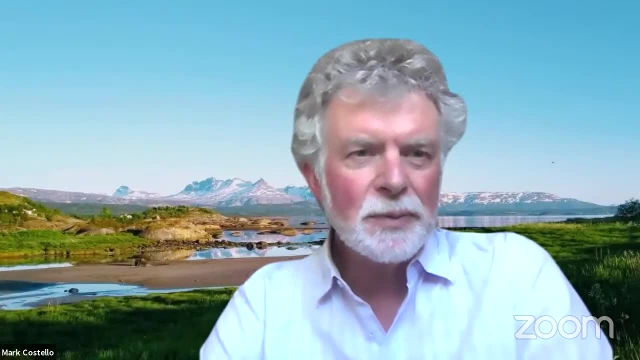 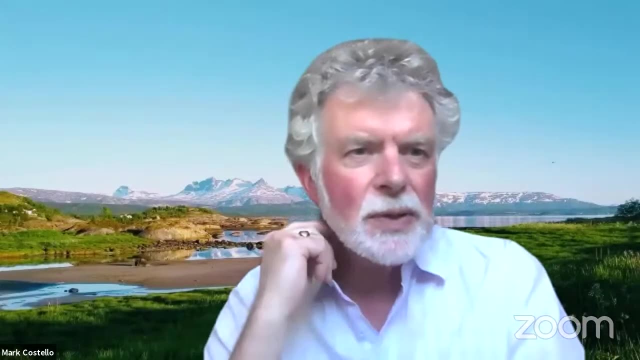 it was never mentioned. It's only in the last few decades that marine science has even been in schools around the world, So it's really important to have an informed society. Any of the other speakers, Christo or Jordan? I have a quick comment, Mark. 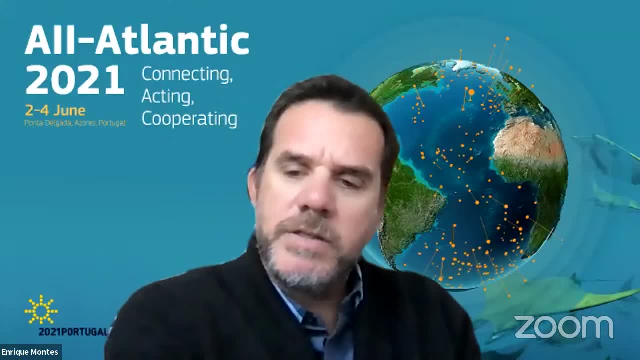 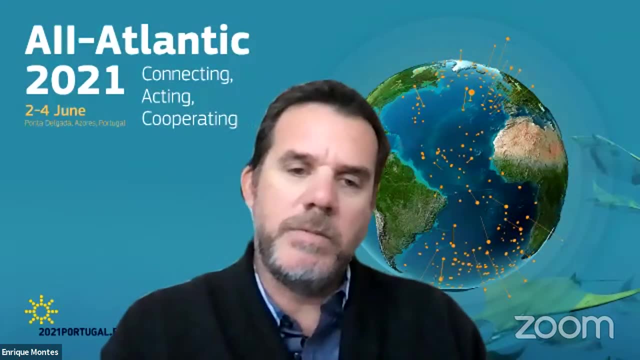 Just to complement what Brian and Anthony were saying. it's, you know, solving the issue of biodiversity data becoming available to the community and being useful- useful for all of the applications that we talked about. It's very important to focus on capacity building. 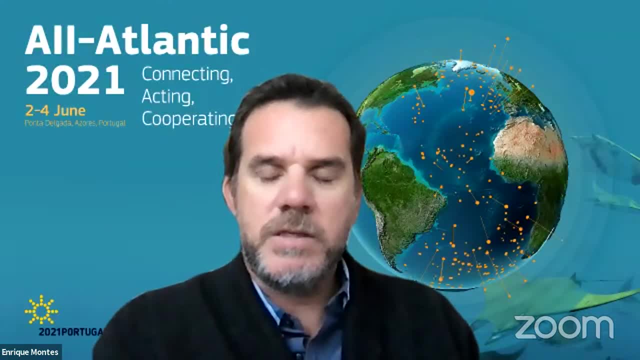 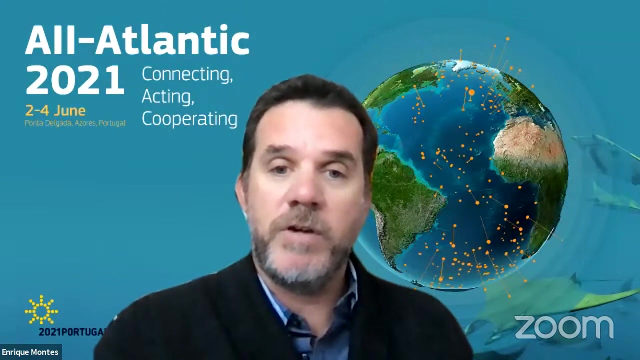 investing in capacity building as a priority. This has the benefit of providing people with the tools needed to implement biodiversity monitoring, but it has the synergistic effect of building a network: People that start talking to each other from very different places that otherwise would have not been able to meet and learn from each other. 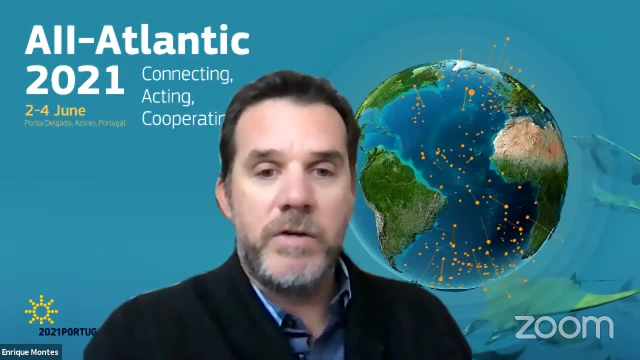 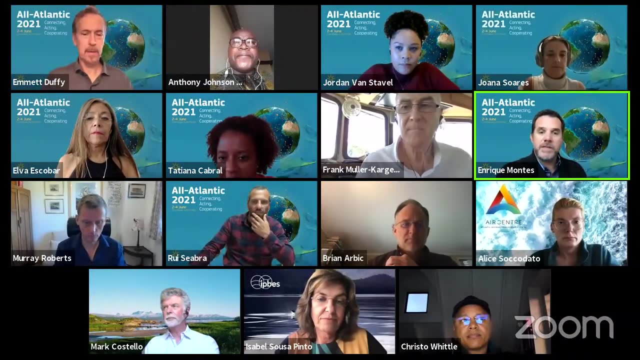 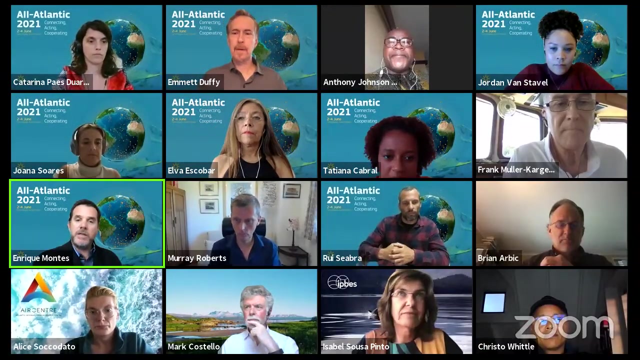 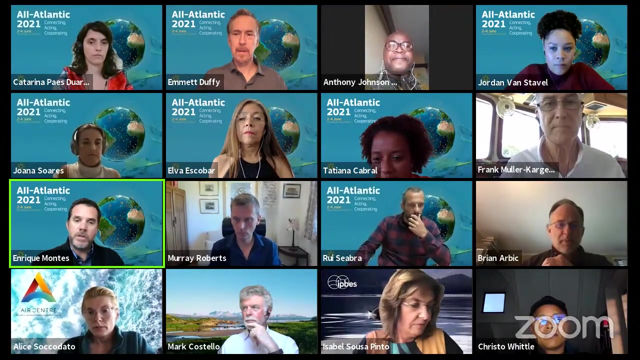 So, and in addition to that, I think it's also very important that these marine ecologists, and maybe managers, interact more heavily with the data science communities to really close the gap between the ability to collect data and share the data. through these open archives, We've noticed that there is an important limitation. 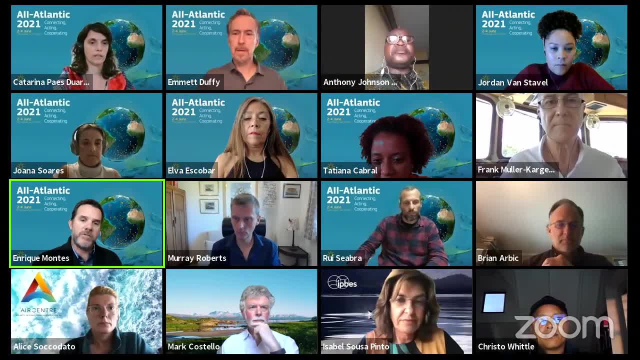 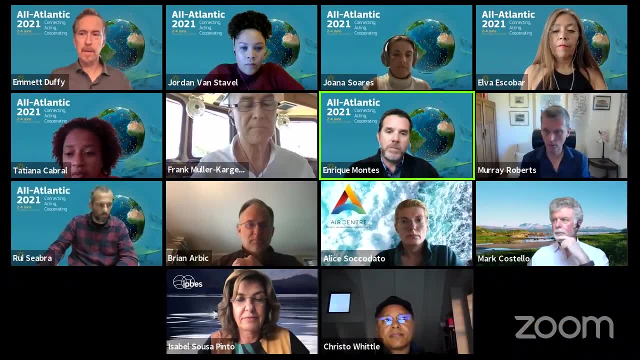 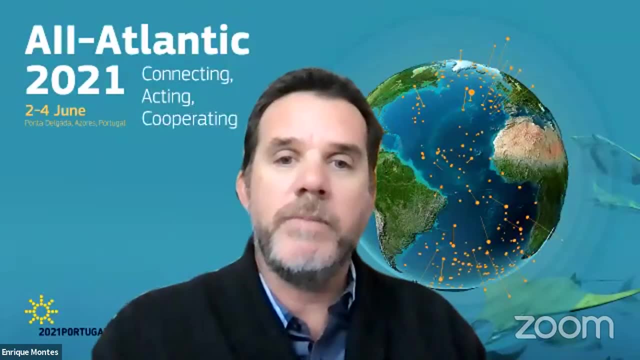 technical limitation. people doing that because it requires a lot of time to learn how to use these different applications for data schema transformations and sharing, And so it's very important that we also invest in developing computing tools, software and code that will facilitate the process for people to share data. 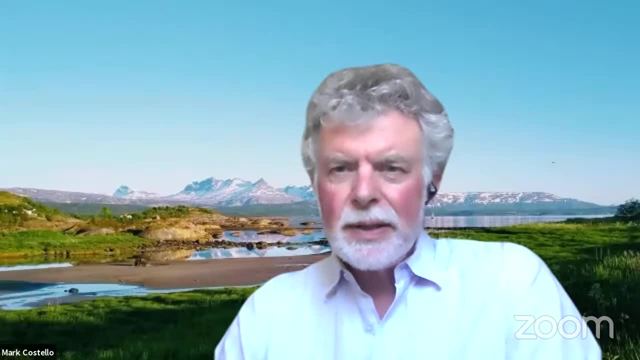 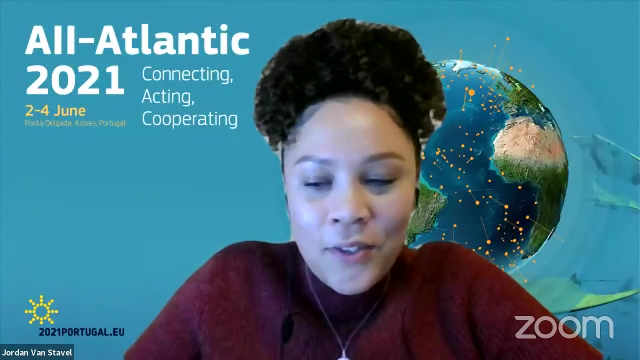 Thanks, Enrique. We're just about at the end. Did Jordan or anybody want to say anything, Are you OK? Yeah, I'll just add one comment. So I just wanted to thank everyone for the really wonderful presentations And then also just adding on to what Anthony mentioned. 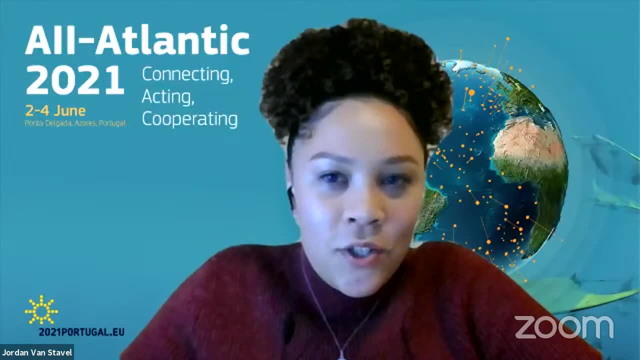 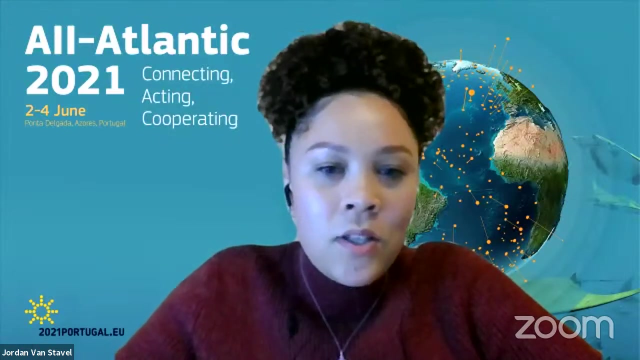 that ocean literacy is so important And I think bringing the message across of how the ocean can actually, how the ocean could be important to say, for instance, people who are living in landlocked countries. just bringing that across and getting that the value of the ocean to those people, the message, 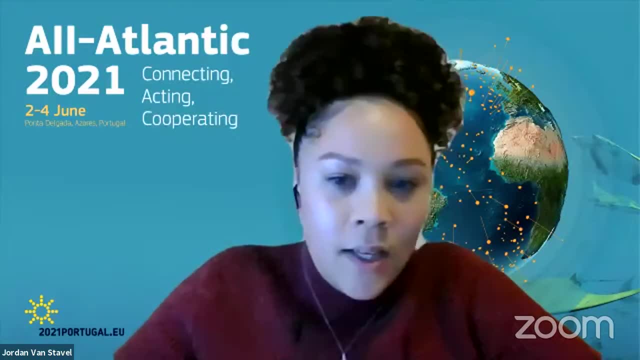 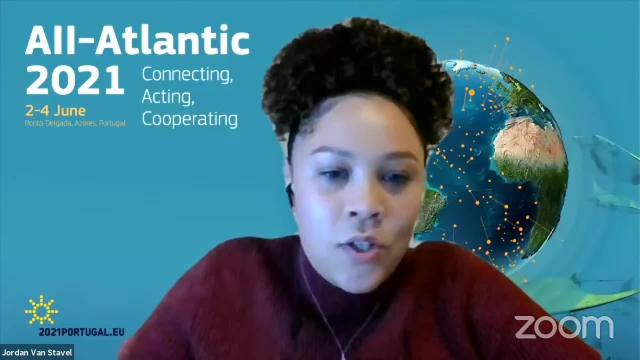 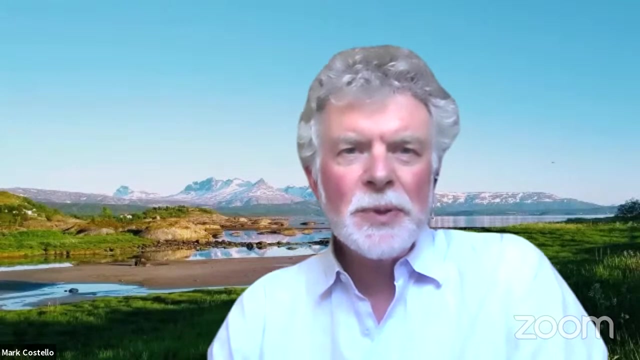 is so important for them to understand And how it actually affects their daily lives and how important it is to get involved and to try and make a difference towards the decade and just towards a sustainable ocean in general. Thanks, Thanks, Jordan, And Christo has his hand up. 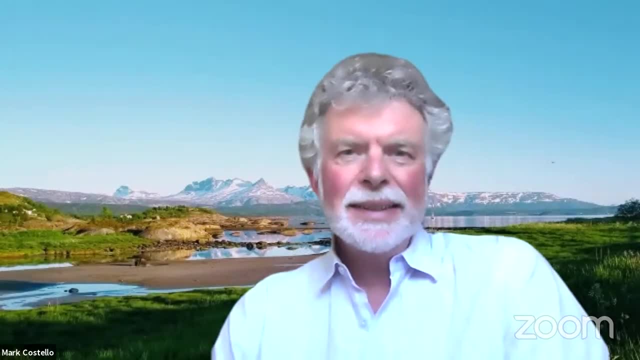 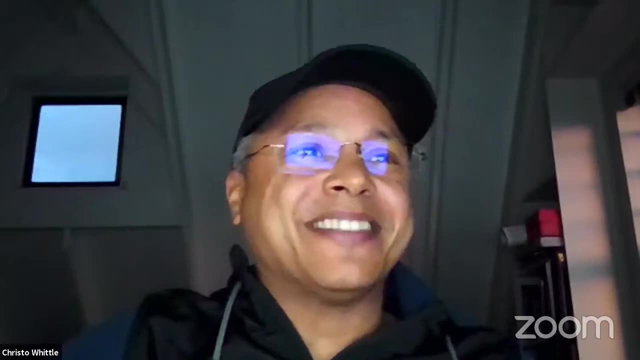 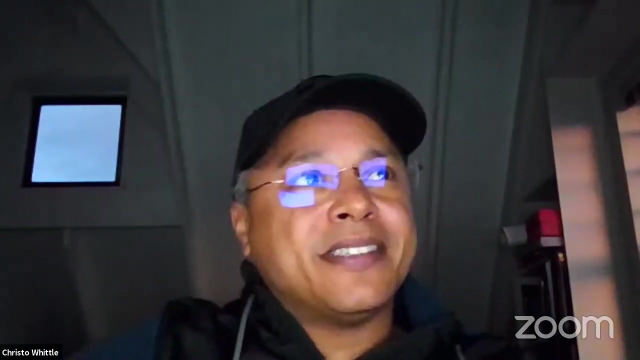 Christo and then Frank, Thanks. Also thank you for inviting me to speak. I kind of come in at the end and feel like an outsider in the physical perspective, all the biology talk- But when it comes to the education, I think target audience is really a big deal in terms. 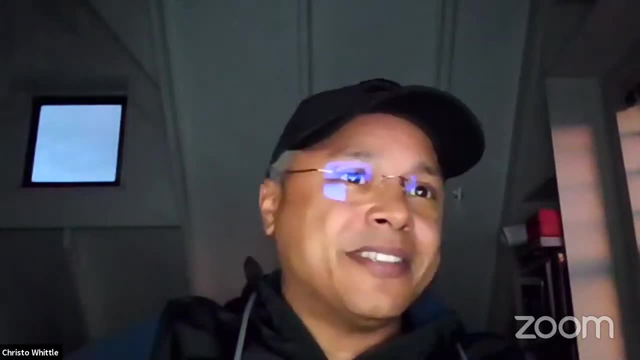 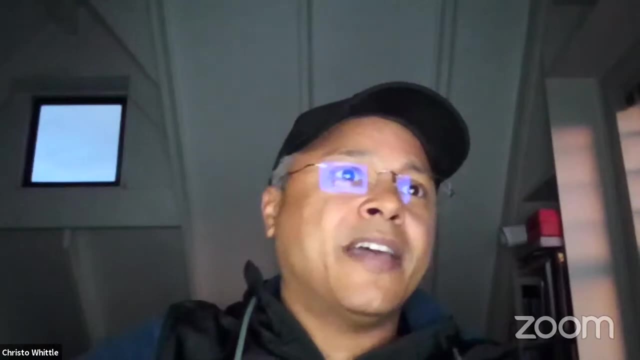 of where we are talking, the level that we are talking at. Our target audience is clear: scientists- And when we're talking about data and data sharing, but if you want to talk about levels of education, aiming it at postgraduate or graduate schools. 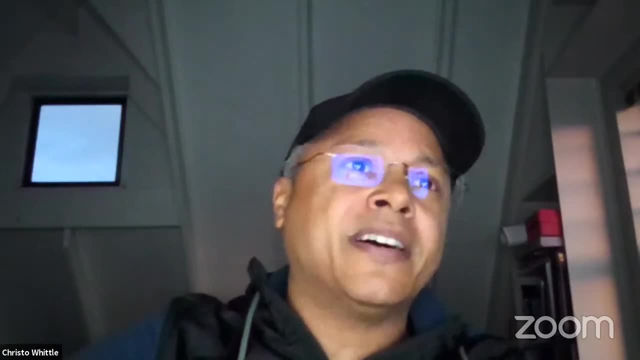 already too high. We should be thinking about engaging in social media at levels that are accessible to the people. who's going to matter next? So, if you want to talk about something more popular, what's happening or even memes- And I'm just thinking about my kids now- 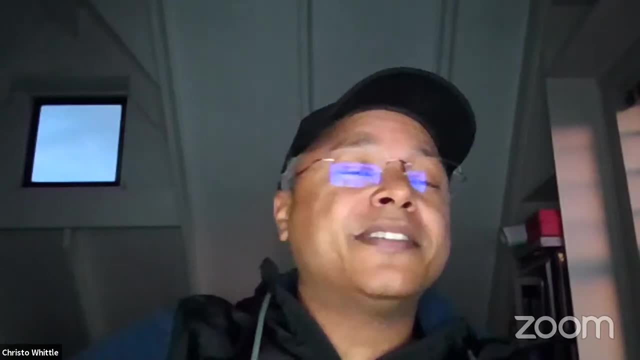 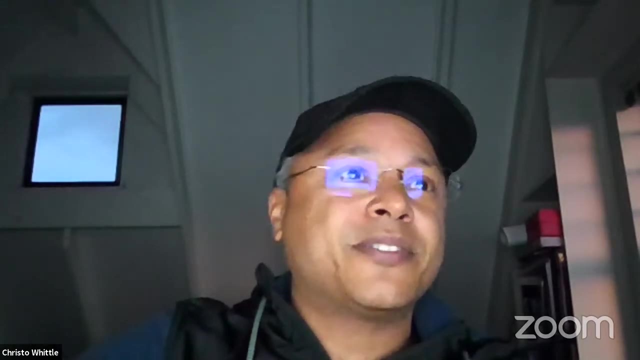 Memes and TikTok, those kinds of things, But this is what the kids are paying attention to, and also YouTube. They learn a lot from YouTube. Whenever they need to go and research something, that's where they start. So that is if we want to create a profile for our science. 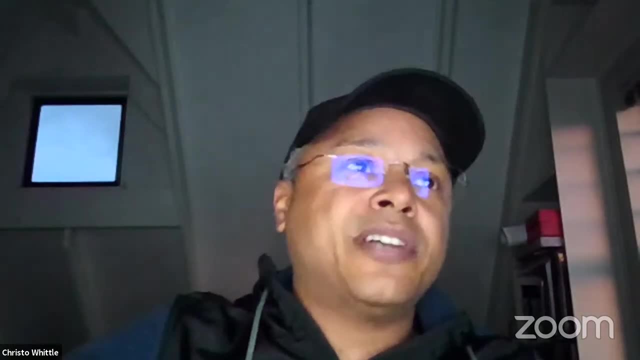 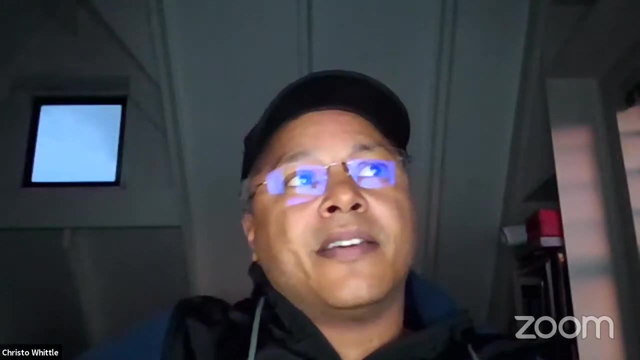 and engage the impact that my octopus teacher had. everybody had to watch that It was just being bandied around socially. This is the kind of thing I think we should be looking at. I mean, we're already doing the other education. 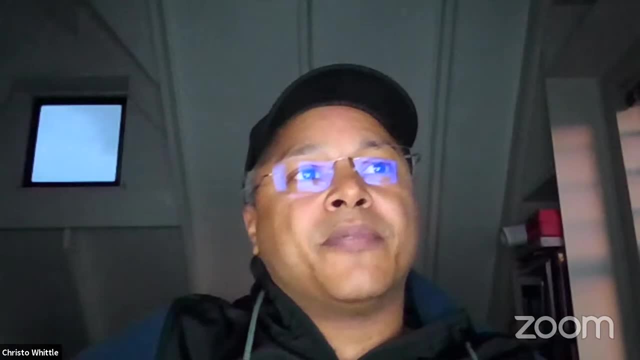 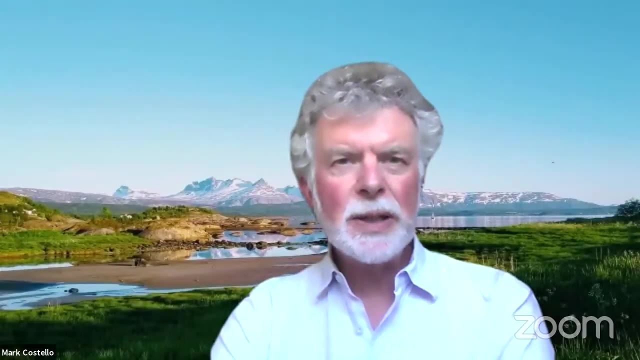 at the tertiary level. It is what's happening below that, where we are eating the snack, I think. Thanks, Thanks, Christo. I'll give the final word to Frank, but I want to make a personal word of thanks to Joanna Suarez, who's hidden in the background somewhere. 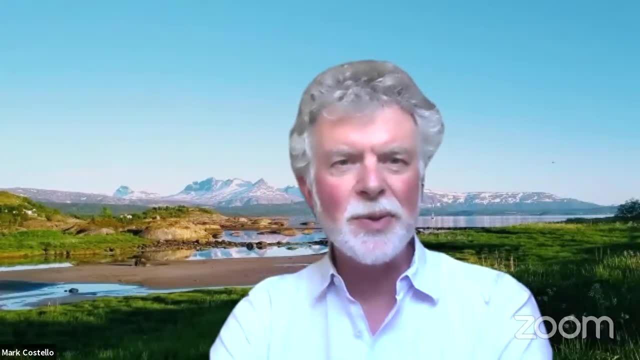 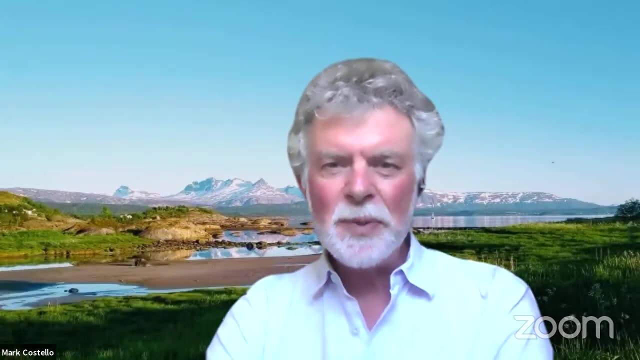 But she's organized all of this event, put all your slides together, sent you all the reminders and reminders again and coached us all to have a very successful session. And if you all want to turn your cards, your cameras on, she might want to take a little photograph. 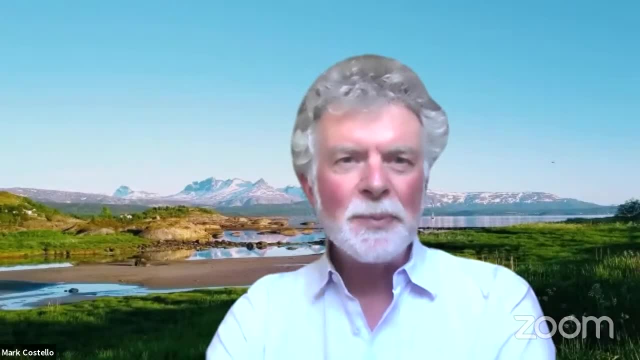 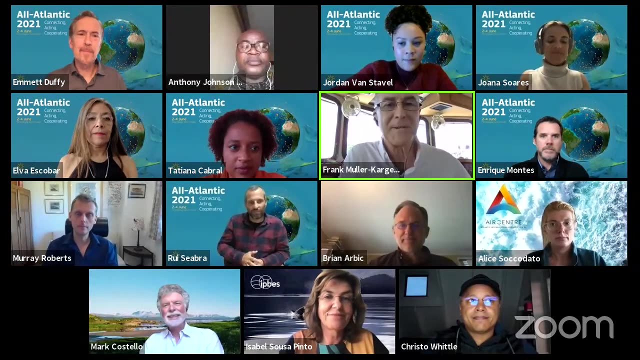 of everybody a screenshot before we finish. So, Frank is one of the two co-chairs of MBON. Do you want to have the last word? Yes, Mark, I wanted to also thank Joanna and Alice and the team at the Air Center for organizing this. 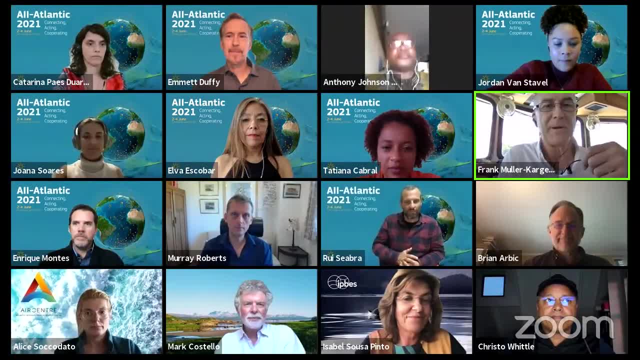 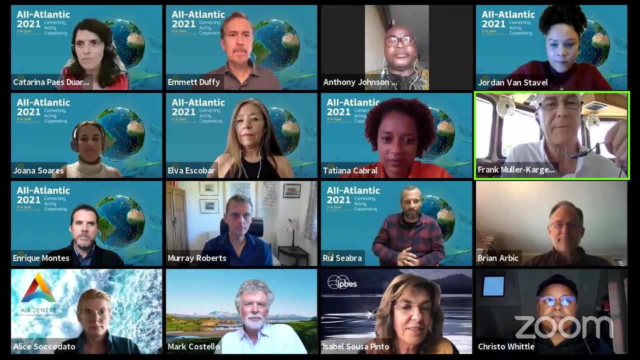 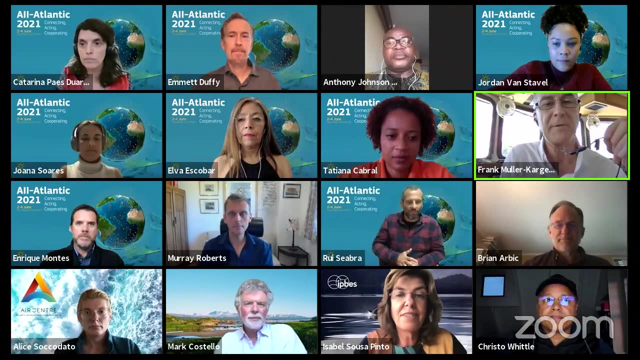 and for all the speakers And you, Mark, for helping moderate this. I want to remind people that we have a digital session session on the microbiome of the And also one on the contributions of the Atlantic to global observing. So the presentations continue.